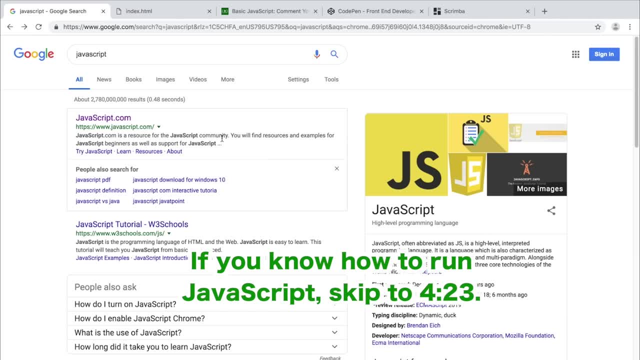 all web browsers can run JavaScript, which is great because a lot of devices have Web browsers on them. So when you write something with JavaScript, it will run on all sorts of devices and operating systems. So you have a few options for writing JavaScript. Let 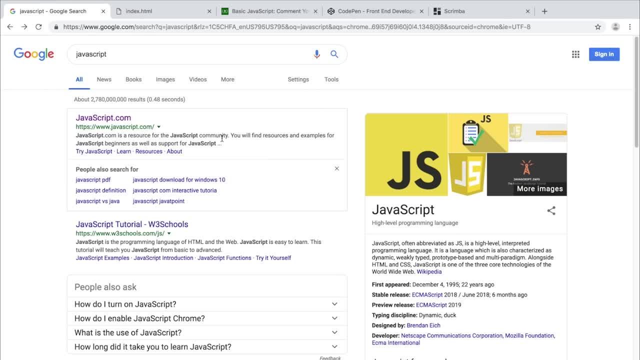 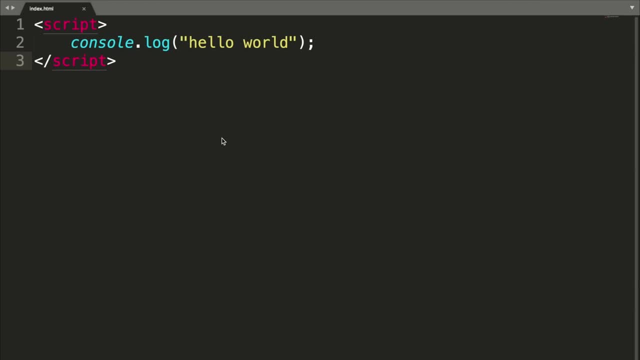 me show you a few things you can do to follow along with this course. you could download a code editor Here. I have sublime text. you could also use Visual Studio Code or Adam or any code editor, And I've created an HTML file, because HTML files can be open in. 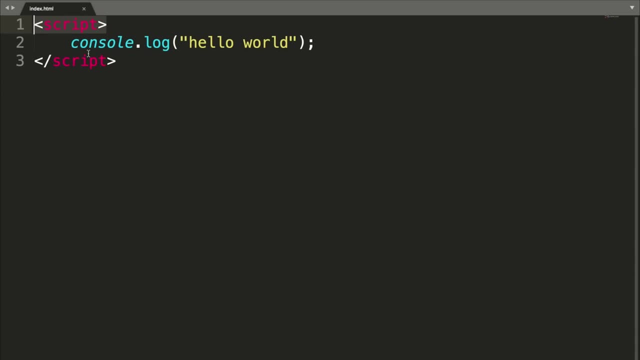 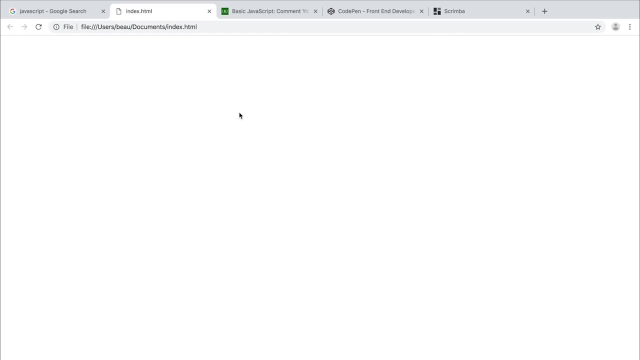 web browsers And I have these script tags. These are HTML tags, But within our script tags we have our JavaScript. So if I open up this file in a web browser, it looks like this: Well, I can open up my JavaScript console And then in the console you can see it says Hello world. That's right. 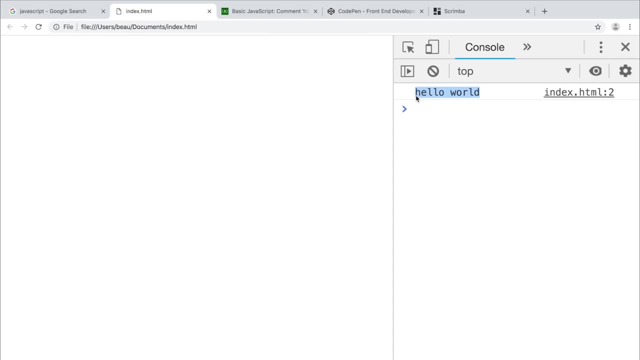 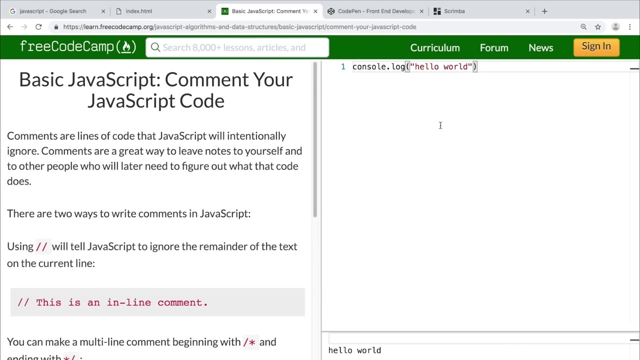 from my JavaScript program. So whenever you do console dot log it's going to show in the console. here You could also just use the code editor that's included. on free code camporg. Like I mentioned, this course follows along with the JavaScript curriculum on free code camporg. 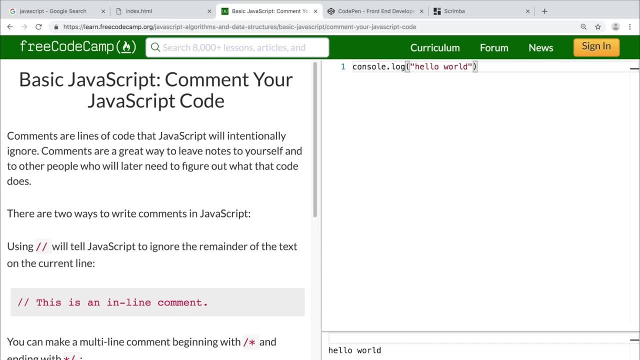 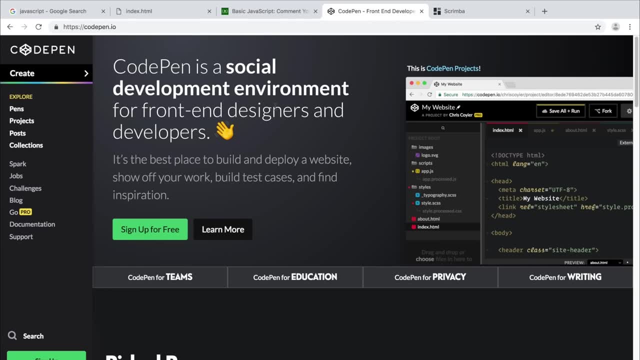 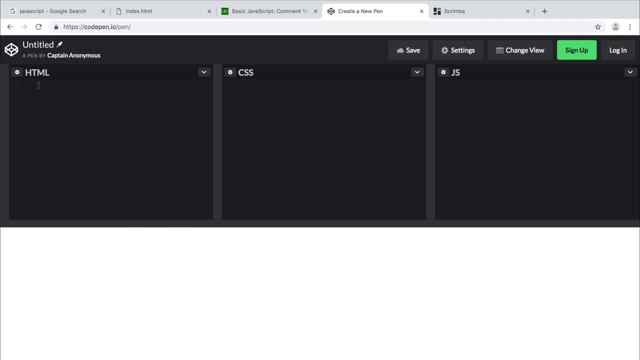 And there's a built in JavaScript editor right in here And then it shows you the console down here. Another option would be to use CodePen. If you go to CodePenio going to go to create pen, And then there's going to be three windows: HTML, CSS and JavaScript. Well, 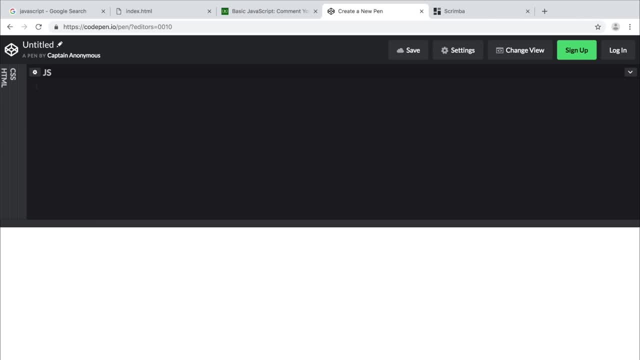 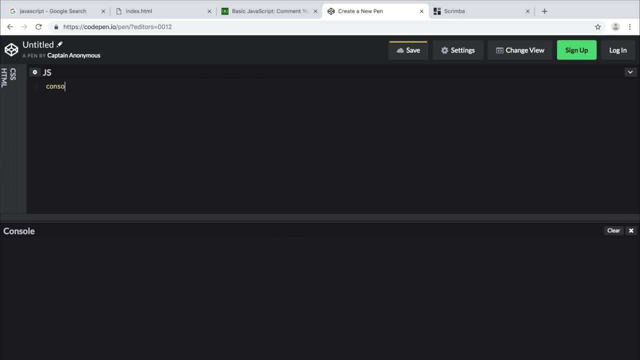 we just care about the JavaScript And in this course we're not going to be doing anything with HTML and CSS. we just need the JavaScript and the JavaScript console. So if I do console dot log and then do Hello world, then we can see right in the console Hello world. the final thing you could do would be: 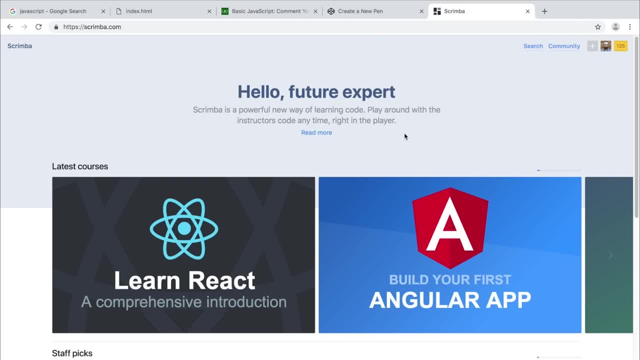 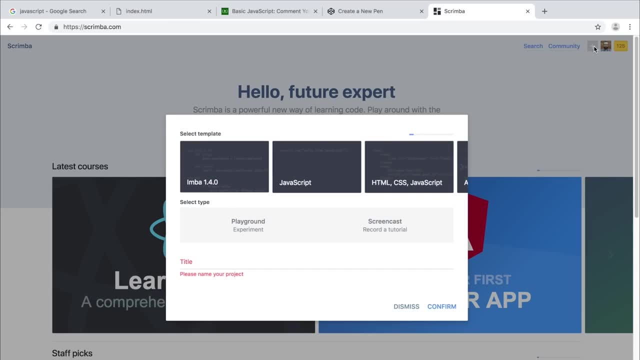 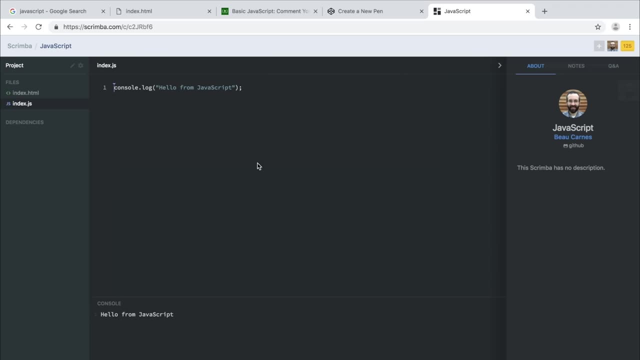 use scrim, But most of the course I actually recorded using scrim dot com. So if you want, you can use scrim dot com to follow along. Once you log in, just click the plus button and do JavaScript playground and then confirm And it's going to open up a new JavaScript window. Now I can increase. 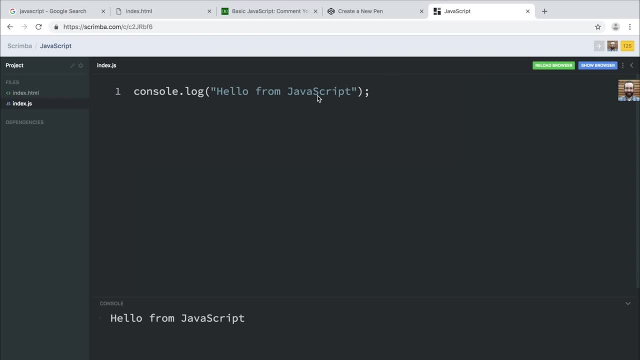 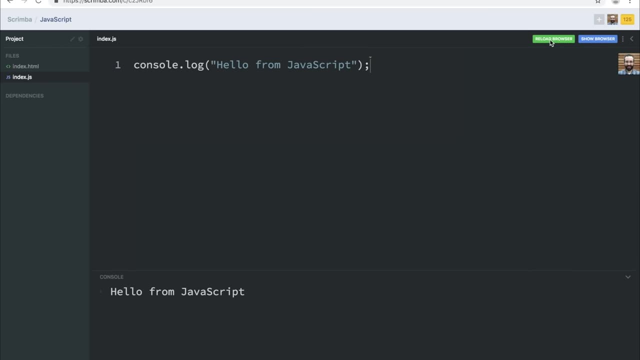 the font size here And it already has console dot log. Hello from JavaScript and you can see in the console right here: Hello from JavaScript. Also, if you hit reload, it reloads everything and you'll see this pop up. Hello from. 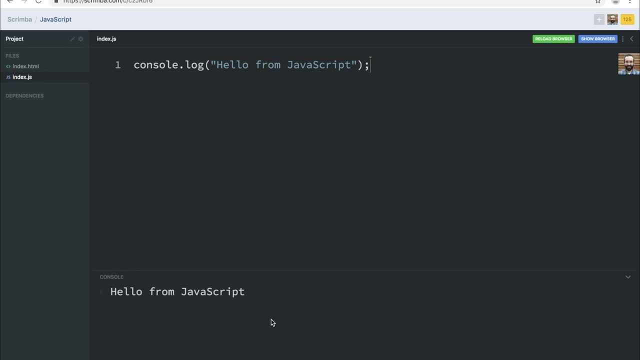 JavaScript. So that's something interesting about scrimba is that it has two ways of logging in the console. we have the pop up and then we have the console. here you'll see that in this course to the two different ways of logging to the console. 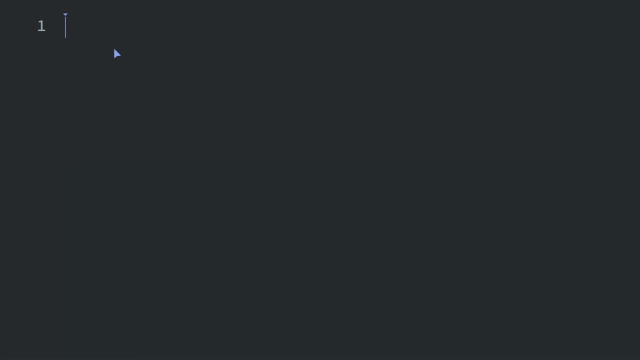 The first thing we'll talk about in JavaScript is comments. Comments are lines of code that JavaScript will intentionally ignore. They don't do anything. They're just used to create notes for yourself and others about what the code does. So if you do slash, slash, you can make an inline. 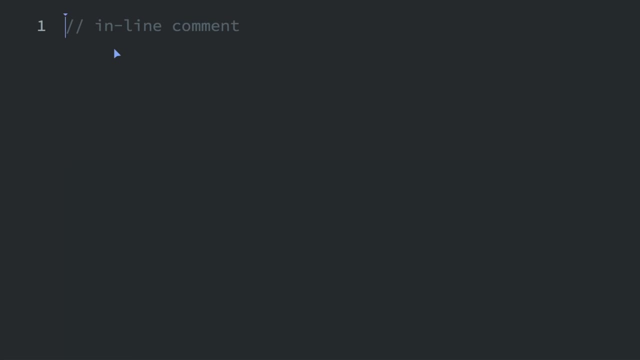 comment. An inline comment means it's at the end of a line of code. For instance, I can put: var: number equals five. that's a way to declare a variable And we'll talk more about that later, But right now we're just talking about comments. you can see that this code is in color because the code editor knows. 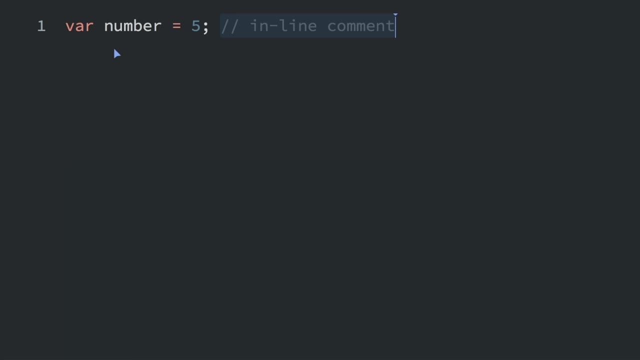 that that's code, that's going to run And the comment is automatically grayed out because it's not going to run. We can also do an inline comment, or I mean a multi line comment. If we do a slash star and I 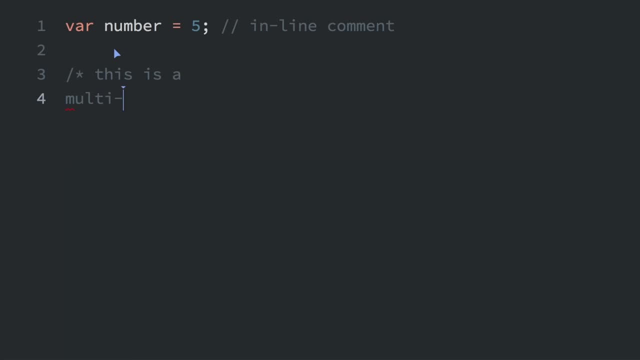 can put: this is a, and then I can put multi line comment And I'm going to end with a star slash. So it begins with a slash star and end with a star slash, And you can put as much text as you want in between these And you can see: this is all. 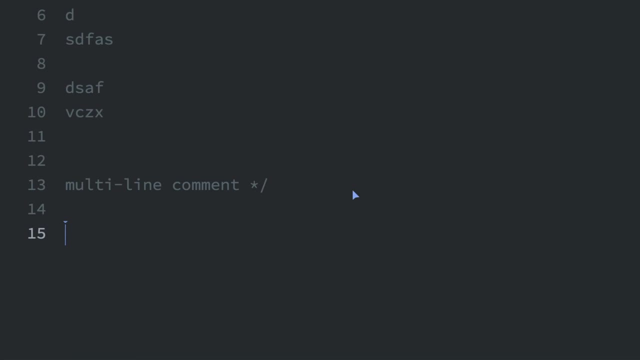 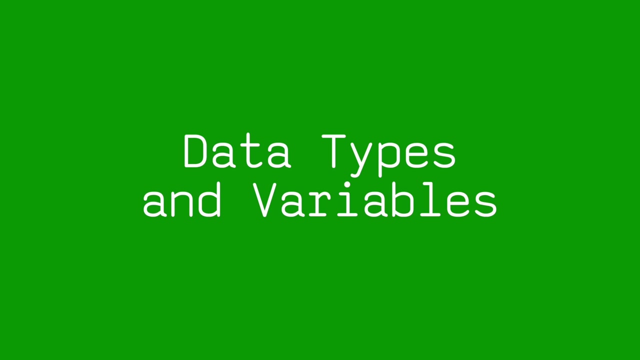 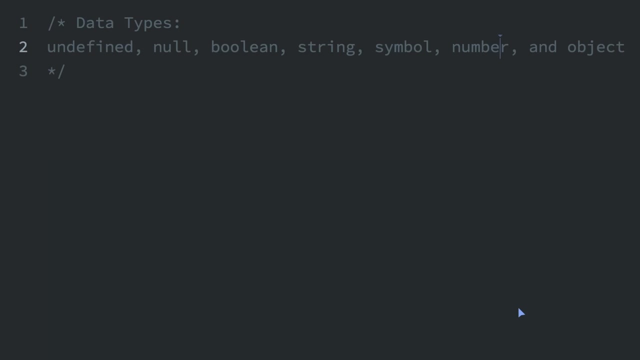 grayed out because it's all a comment, And then afterwards I can put number equals it. I can put number equals nine and you can see it will be in color again because it's no longer commented out. Okay, now we're going to talk about data types and variables. In computer science, data is anything. 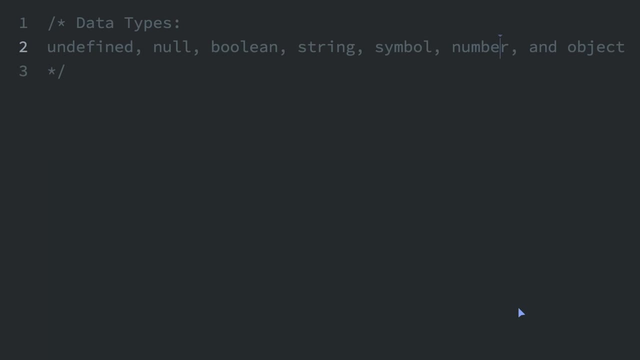 that is meaningful to the computer, And JavaScript provides seven different data types that you can use within JavaScript. Now, some of the more obvious and most common are strings and numbers. a string is just any sort of text. a number is a number. Now let's go from the top So undefined. 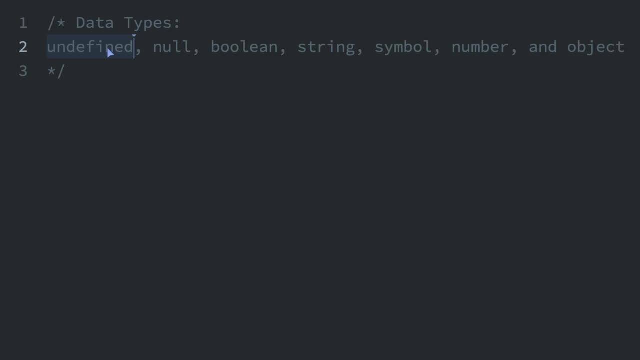 is something that is a string, and a number is a text, And a string is a text And a number is a thing that hasn't been defined. you may have a variable that you haven't set to be anything yet. Null means nothing, So you've set it to be something, And that thing is nothing, So you can. 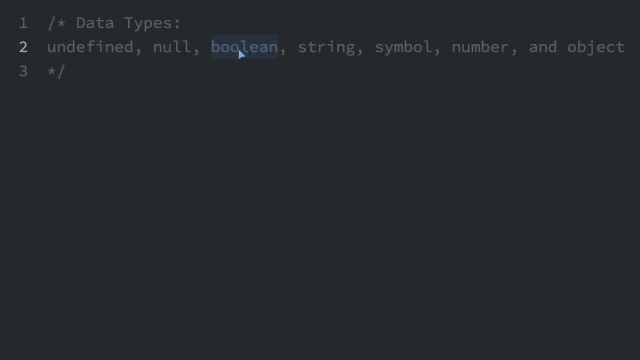 say this is null or nothing. A Boolean means true or false. We talked about string. A symbol is an immutable primitive value that is unique. Now we'll talk more about those later Numbers. a number and an object can be a string And a number is a number And an object can be a string And a number is a. 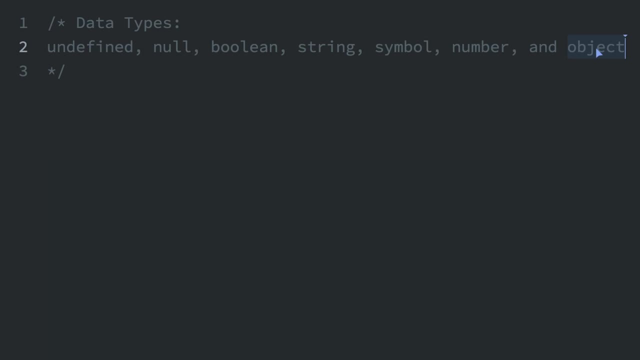 string And a number is a number And a number is a pair And a number is a value. So these are different key value pairs. Again, we'll talk more about those later. Now you're, you are often going to set data into a variable. A variable allows computers to store and manipulate data and in a 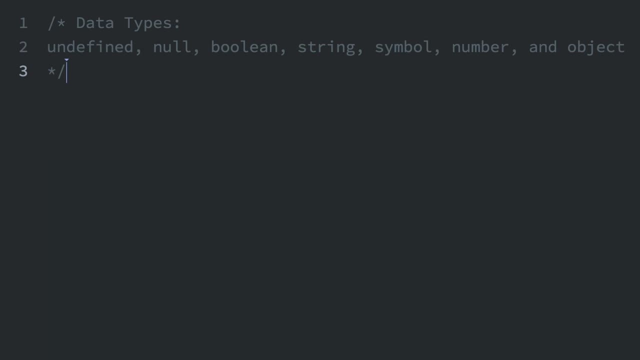 dynamic fashion. It's basically a label to point to the data. A variable is almost like a box and you can fill it with anything. you'll fill with the data that you want. So to declare a variable, one way is to use the var keyboard keyword. var stands for variable And I can say my name. 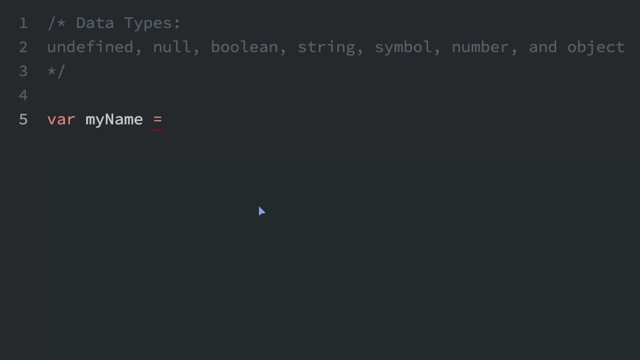 I can put set this to anything. it can be any of the data types above, But it's common to set something to a string. So I can set my name to be bow Now. later you can set to be something else. 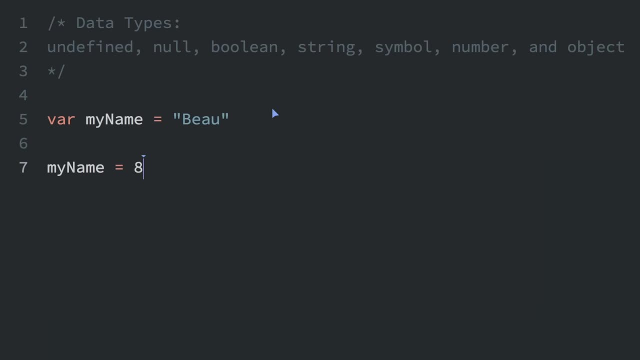 I can say my name equals eight And you can just set to other data types later. Now there are actually three ways to declare a variable in JavaScript. So var is one of them, And for a while that was the only way, But there are other ways to. there's a way called let. 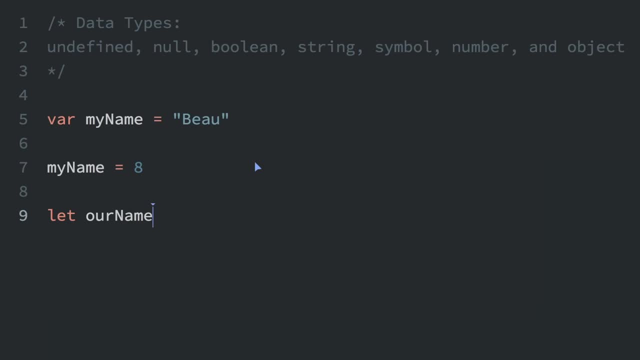 so I can say let, our name, and then I can say equals free code camp, And then the other thing would be const. So I could do a sit do: const pi equals and 3.14.. Now the difference between var, let and const var is going to be able to be used throughout your whole. 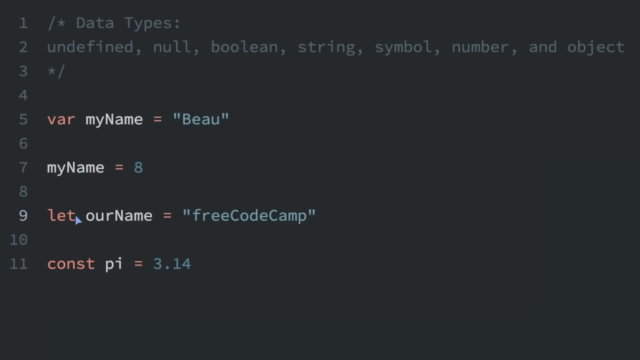 program Let will only be used within the scope of where you declare that. Now we're going to be talking about letting const more later, So I'm just giving you a brief overview of what that they are. now. Const is a variable that should never change. it can never change, So like right. 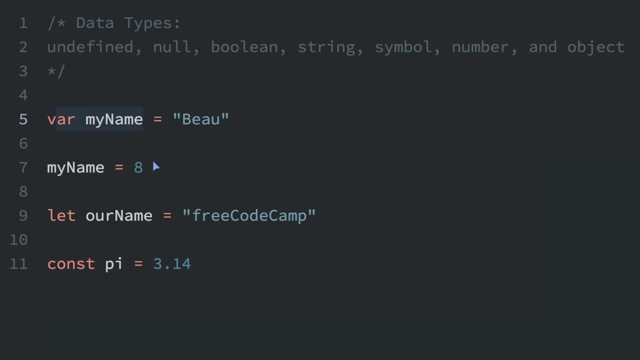 up here I declared my name, but then we changed it here, So it started out to be bow and we change it to eight a const, you can never change it. If you do try to change it, you'll get an error, Okay. 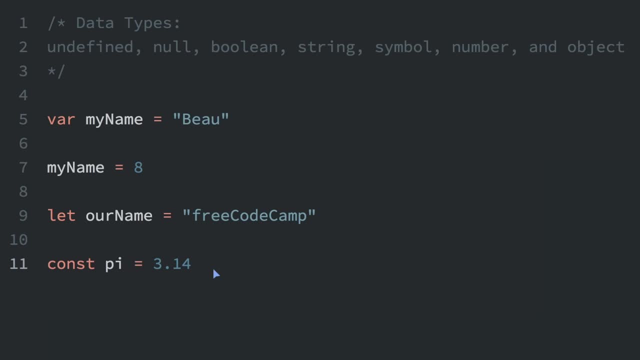 that's all for now, But, like I said, we'll be talking more about the different types of variables later. There's a difference between declaring variables and assigning variables. Here's how you assign a variable: var a, and then the semicolon. I didn't mention this earlier, but you end all lines in. 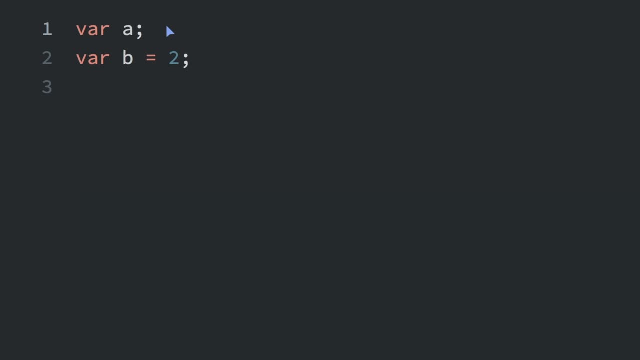 JavaScript with a semicolon. Well, it's not actually required. you can actually just skip the semicolons completely, But most people recommend that you put a semicolon, just so it's obvious where the end of the line is. So here: 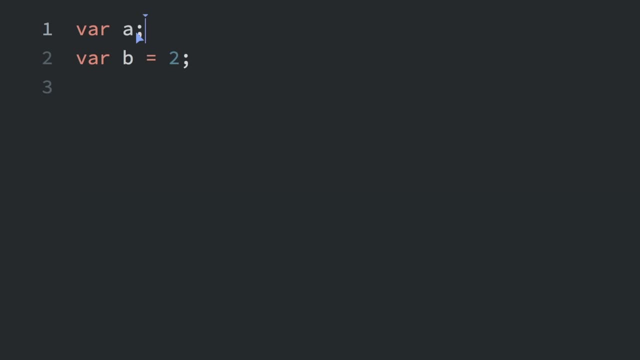 we are just declaring a variable to be called a, And then here we are assigning a variable. we're declaring and assigning in one line, So we're declaring it var B And then the equal sign is the assignment operator. It means that two is being assigned to B. we're not checking if B equals. 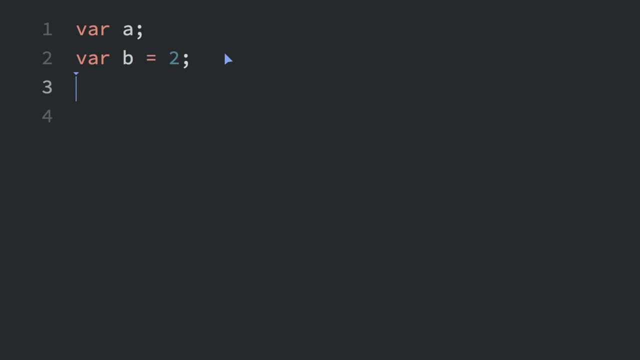 two, though we're just assigning two to B, So after that we can actually assign other things. So I can say: a equals seven. So now I've just assigned seven to a. I didn't have to declare a because it was. 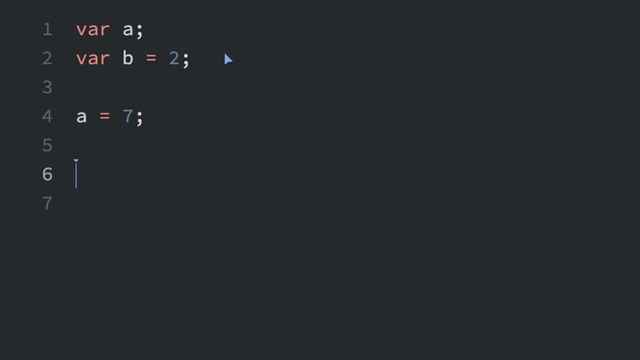 already declared, And I can also say that B equals a. So I've now assigned the contents of a to B. I'll put the semicolon there. One thing I want to tell you about is console dot log. console dot log allows you to see things in the console. So I'm going to console dot log a. And if I load this here, 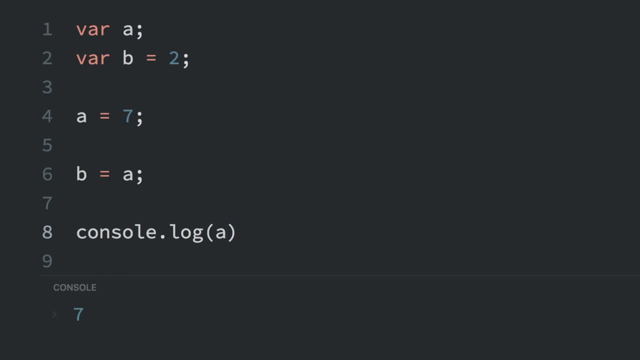 you can see down here in the console it shows seven. So right now we've assigned a to be seven or and so we, when we console dot log a, it shows seven down there. If we put another console dot log right here, This will allow us to show what a was up here and then down there. So console 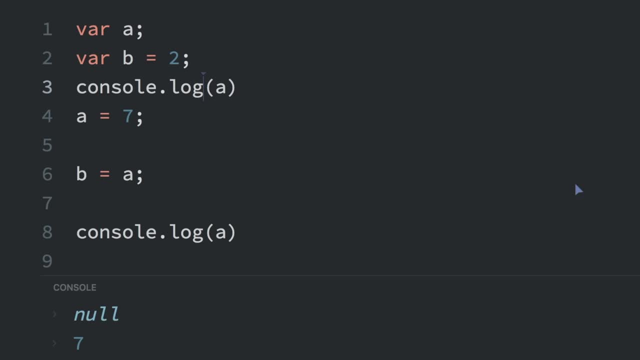 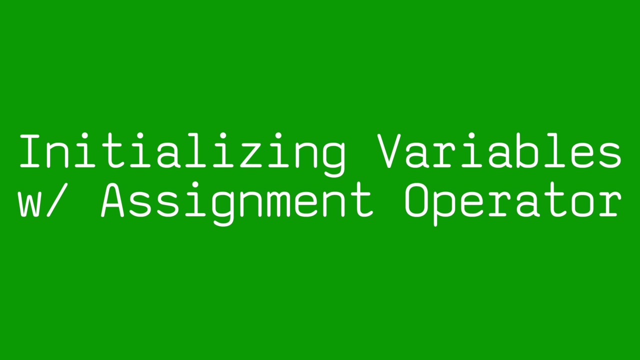 dot log. Now if I run that, we can now see at first a was null and then now it's seven. So here was this non seven down here, So you can check what variables are at various points in your program. Now I'll show you another example of initializing a variable to an initial. 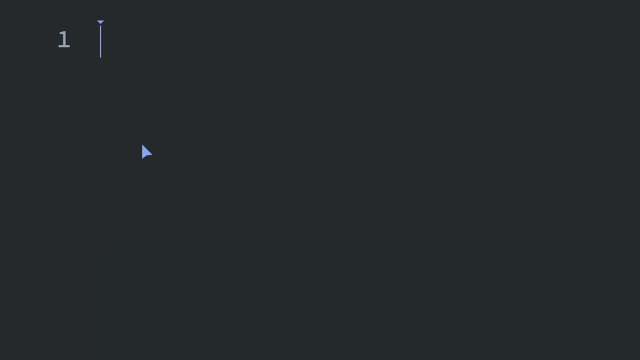 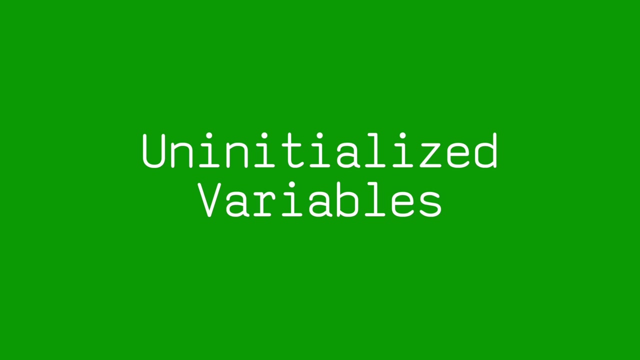 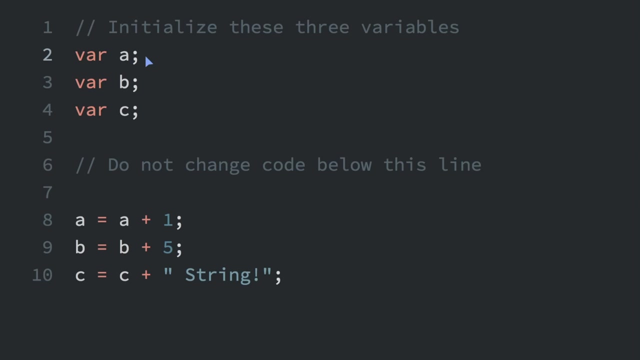 value at the same time it's declared. So I'm going to say var a equals nine. So the var A is declaring it in the equals nine is initializing it with that, the assignment operator, which is the equal sign. Before we do anything to these variables, they are uninstrollable. 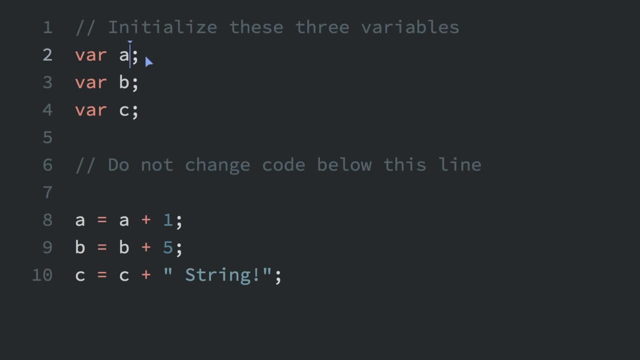 That means their value is undefined. We have not set them to anything, But it's simple to fix that. I'll just set this to five. I'll set B to 10. And then we can set C to a string. it's going to be. I am a string we always have to put in quotation. 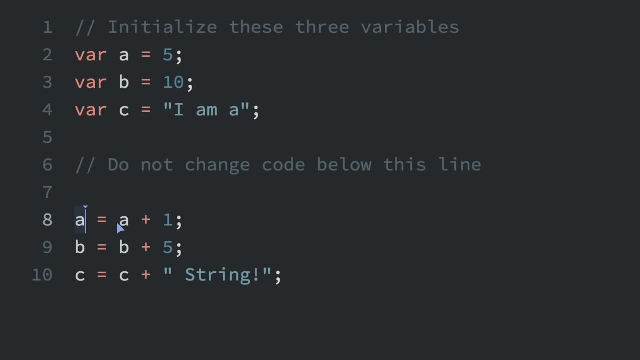 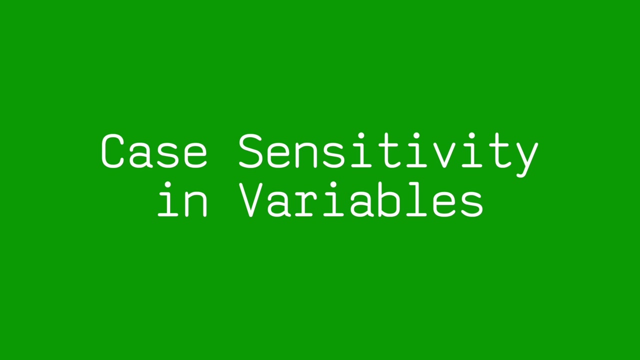 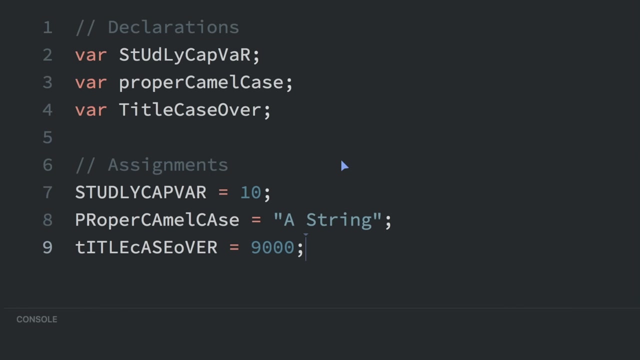 marks like that, So you can see: a A plus one is going to equal six. five plus one equals six B equals B plus five, that's gonna be 15.. And then C is now going to say: I am a string. variable names and function names in JavaScript are case sensitive. That means the capitalization matters. 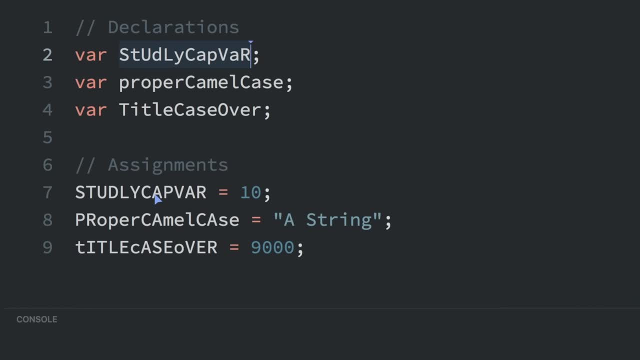 So this declaration here is not the same as this assignment. Even though the letters are the same, the capitalization is not the same. So it's not going to assign correctly And in here you'll see there's an error if we try to run it, because this has not been defined, it has not been declared. 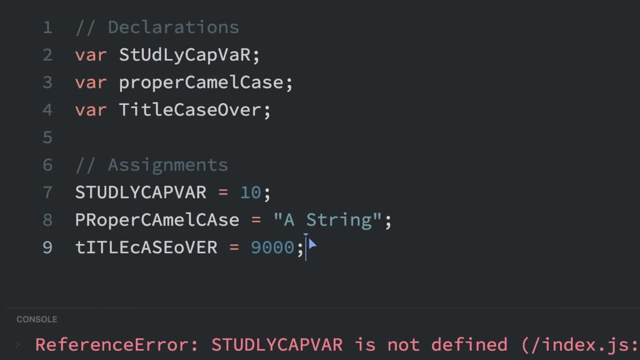 It's generally common practice This to use camel case. So let me show you how we do that. Instead of studly cap var, it's gonna be stud Lee cap var, So the first letter is always going to be lowercase, And anytime you have a new 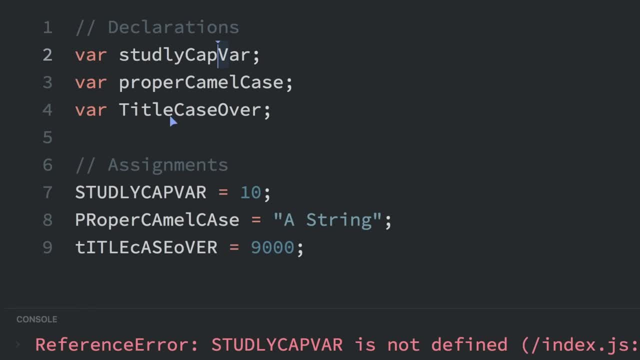 word or new section of a word. you just capitalize the first letter And so we can change this. this one's correct. So now we just go down here studly, cap, var, And then we just do proper camel case and then title case over. So now all these should be defined, So we declare them. 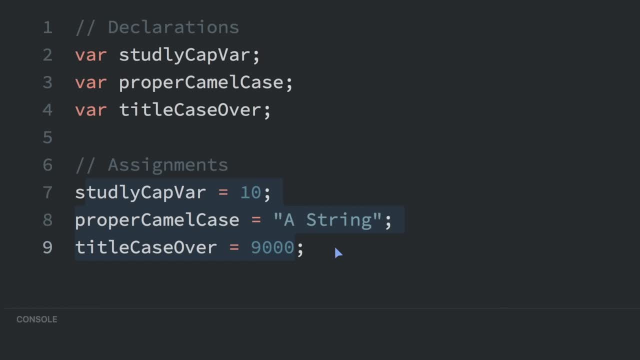 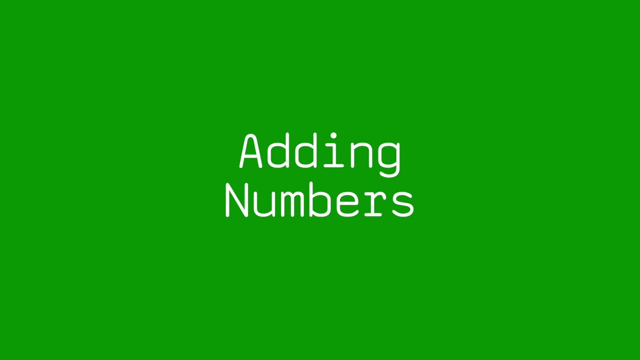 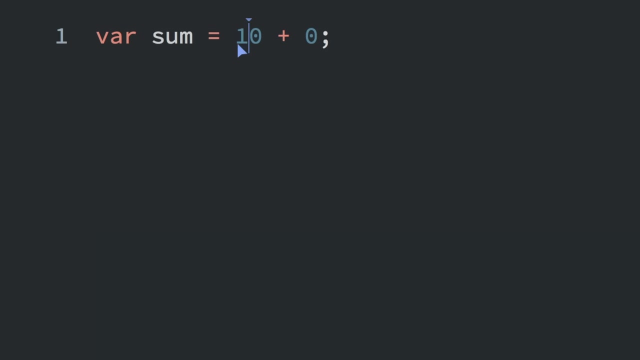 up here. we assign them right here, And then this is not going to give us any errors, it's going to behave exactly how we want it to behave. Adding two numbers in JavaScript is pretty straightforward. You just use the plus um. so this says: 10 plus zero, which equals 10.. We can also do 10 plus 10, which is going to equal. 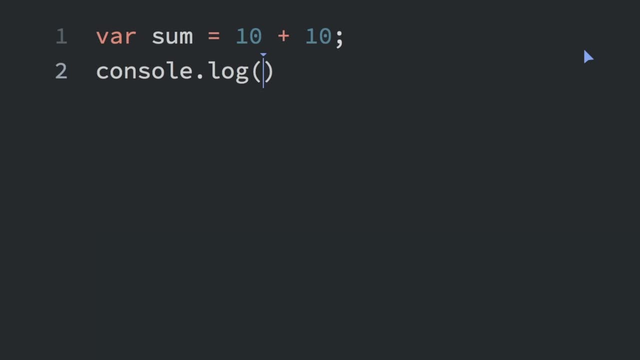 20. If we do a console dot log and I can put some here and then you'll be able to see that the answer is 20.. Right in the console. 10 plus 10 is 20. And subtraction is also what you would. 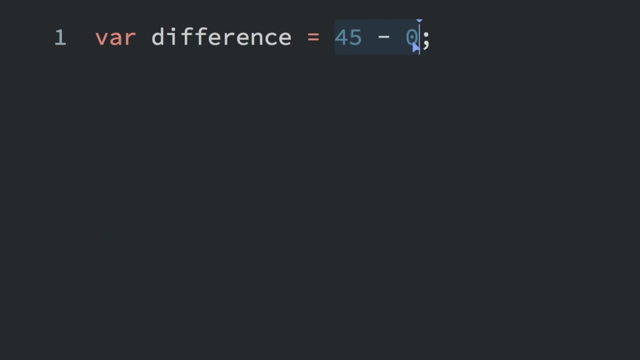 expect. we have the subtraction sign here. this says 45 minus zero. we can also do 45 minus 33. And then that would equal 12. So the difference variable equals 12.. Now multiplication in JavaScript uses this asterisk or star symbol here. So this says eight times zero. 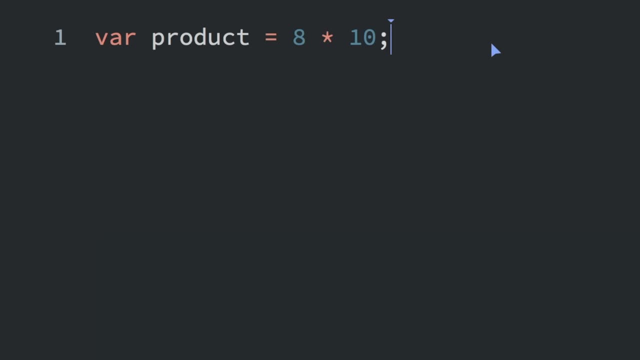 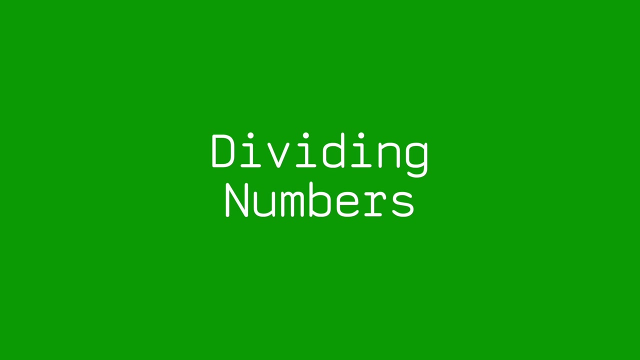 which is zero, or we can change it to eight times 10,, which is 80. So now the product variable is zero, And then we can also do subtraction. So we can also do subtraction, So the variable equals 80.. You can divide in JavaScript with this slash symbol, So this: 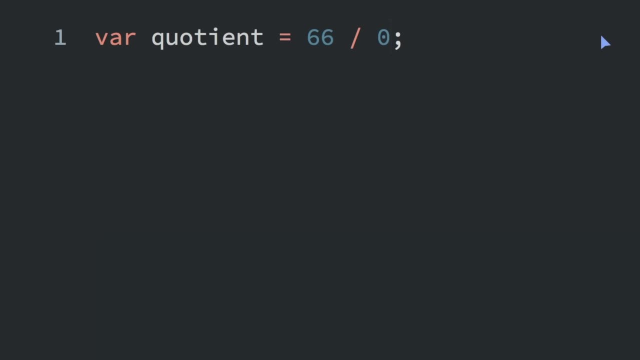 says 66 divided by zero. we can change this to 33.. So now, 66 divided by 33 is two. quotient equals two. To increment a number means to add one to it. So here we're incrementing my var And by one, so it starts at 8787 plus one is 88.. There is a quicker way to increment a number Instead of 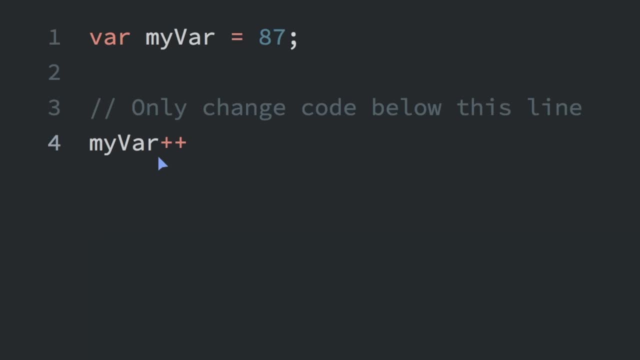 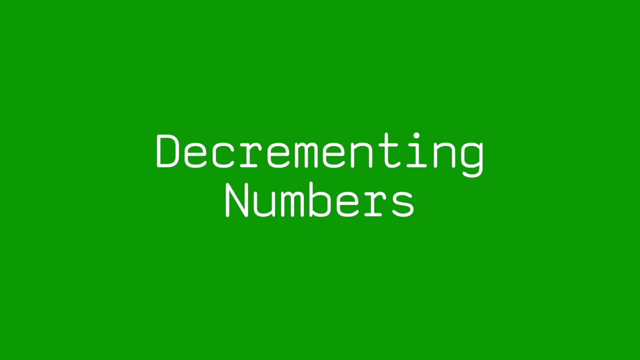 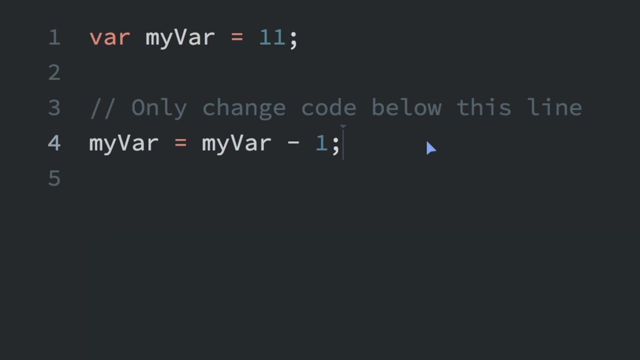 doing this. we can just do my var plus plus. I have our plus plus now. we have incremented my var from 87 to 88.. We learned about incrementing a number with plus plus. you can also decrement a number with minus minus. that means subtracting one, So we can increment a number with minus, minus that. 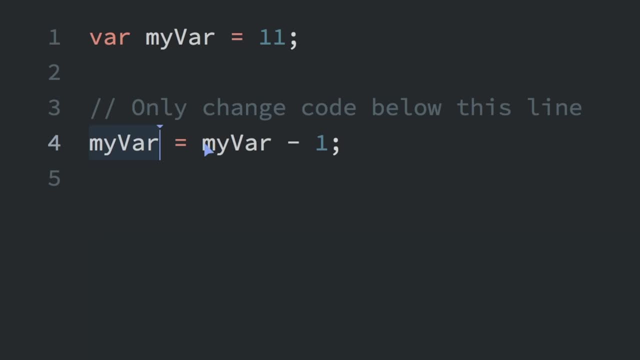 means subtracting one. So we can also increment a number with minus minus. that means subtracting one. So right now my var is gonna equal 1011 minus one equals 10.. We can do the same thing with the minus minus operator. So now my var still equals 10.. We can also create decimal numbers with: 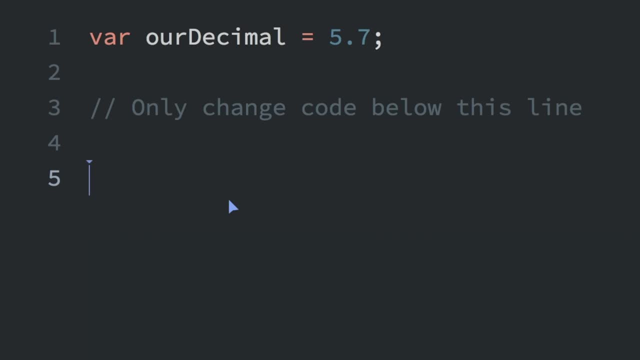 JavaScript. These are sometimes referred to as floating point numbers or floats. You can see this is one here, 5.7.. It can be anything. I'm going to make one called my decimal And then I'm going to store as 0.009.. Anything that has a decimal point in it is a decimal point number. 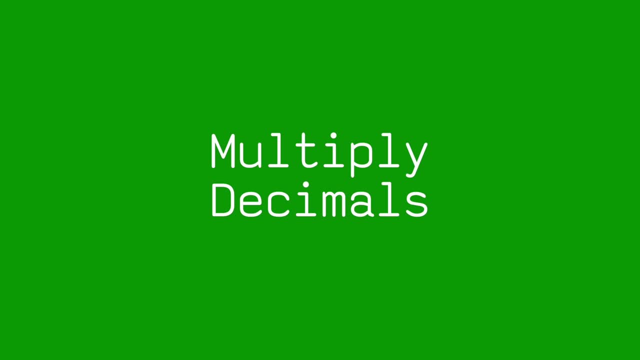 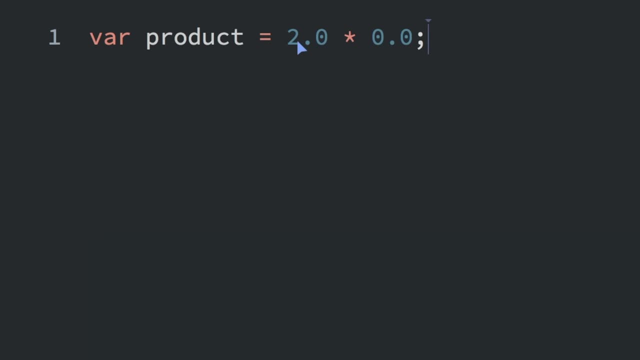 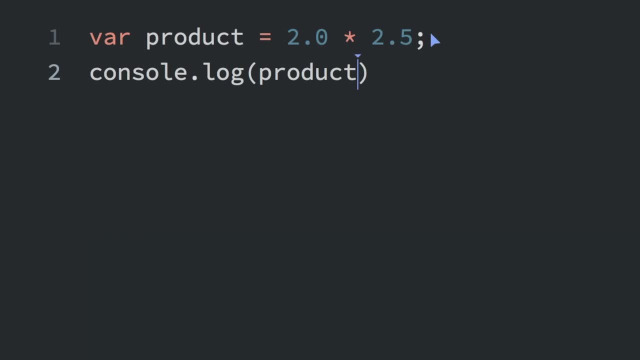 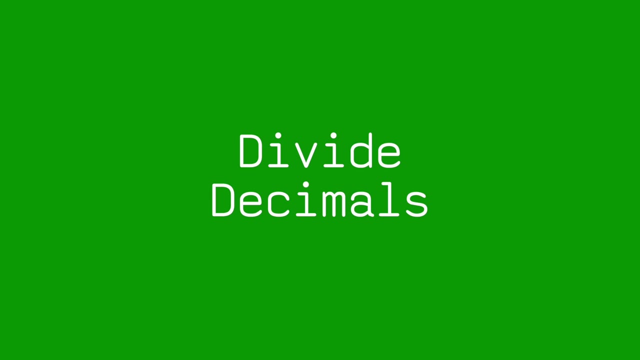 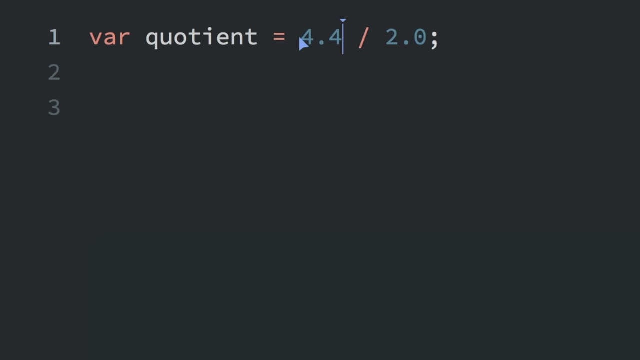 So you can see, if I just put product And if we do the browser here, you'll see that the answer is five. You can also divide decimal point numbers, So in this case I'm going to change this to 4.4.. 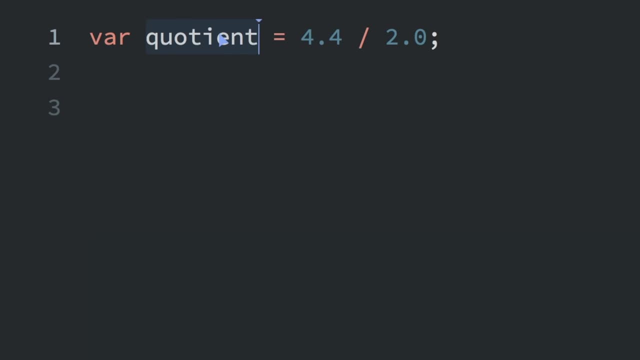 So now the answer to quotient is 2.2. quotient equals 2.2.. The remainder operator looks like a percent sign and it gives the remainder of the division of two numbers. So for in, for instance, if I want to find out the remainder of 11, divided by three, I can do remainder. 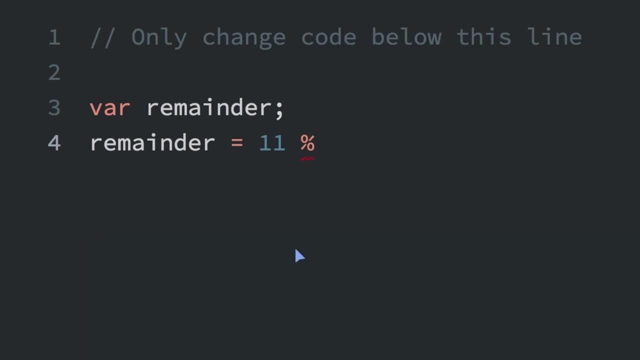 equals 11.. And then I'm gonna put the percent sign which is the remainder operator. three and 11 divided by three is 911 minus nine is two. So the remainder is going to be two: 11, remainder three is two. 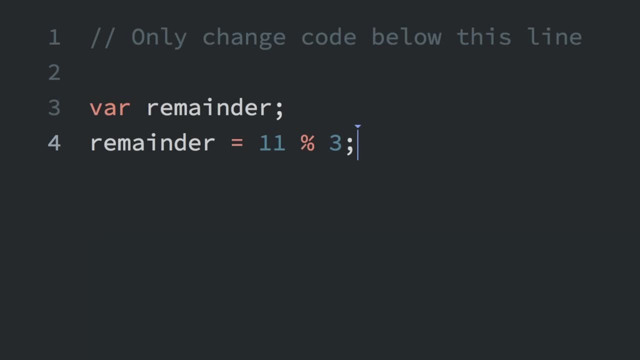 the remainder operators often used to determine if a number is even or odd. If you can divide a number by two and the remainder is zero, that means the number is even. It's common to want to add a number to a variable like this: the A equals a plus 12.. Well, a starts. 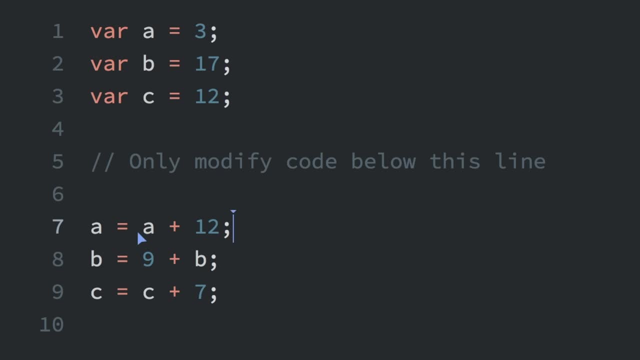 at three plus 12 is 15.. So just adding 12 to whatever a is here, we're adding nine to whatever B is here, we're adding seven to whatever C is. this is such a common pattern that there's a shortcut to do the same thing. It's the plus equals operator, So instead. 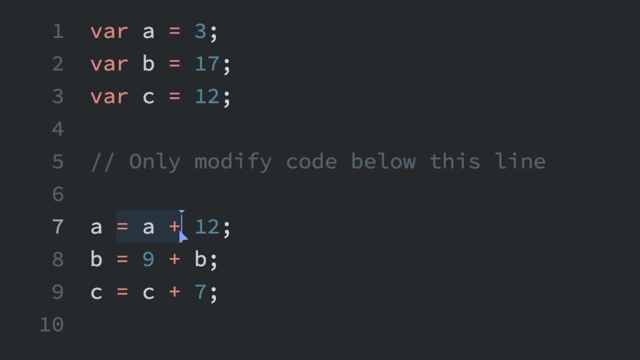 of a equals A plus 12,. we can do a plus equals 12.. So this equals the same thing. So instead of B equals nine plus B, we can do B plus equals nine. So now we're adding the value to the variable and assigning the answer to that variable. So again here we. 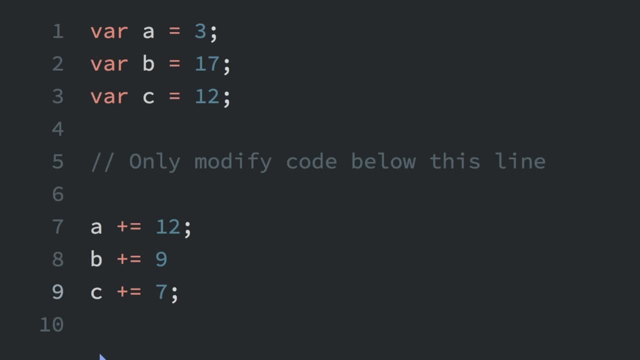 can do plus equal seven. So that's just a shortcut. Previously we learned about plus equals. well, minus equals does the same thing, but subtracting. So this says a equals a minus six. we started at 11, minus six is going to be five, So the new a is going to be five, But we can shorten that instead. 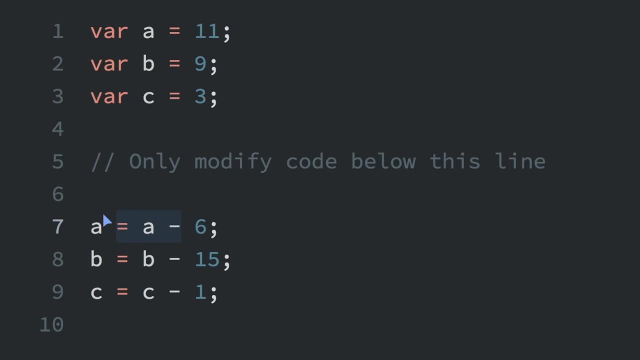 of a equals a minus six. we can do minus equals. This is just a shortcut that JavaScript has. that means the same thing. That means a equals a minus six, but it's just shortened Same here, So we can do minus equals 15.. C equals C minus one. we can do C minus one. we can do C minus one. So 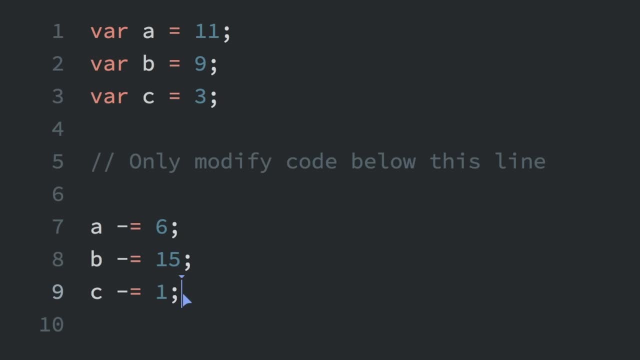 it just subtracts the number from the original value and then assigns that new value to the variable. Here we have a equals a times five. Well, we can do the same thing as before. we can shorten this to a times equals five. So that means the same thing. Here we can do a. 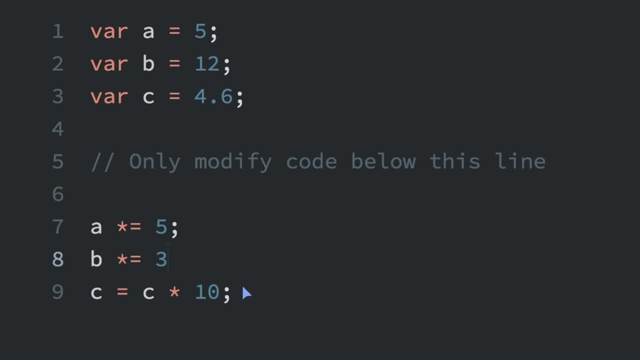 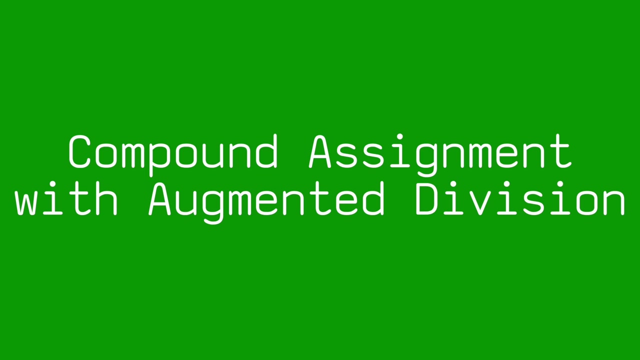 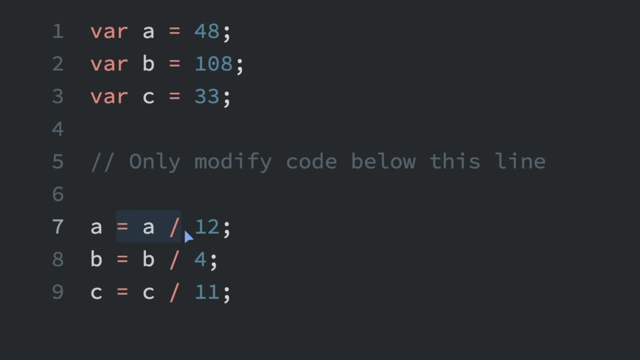 times equals three, And then C equals C times 10, we can shorten this to C times equal 10.. And that's another shortcut for JavaScript. And there's also divide equal, so A equals A divided by 12.. We can do a divided by equal 12.. Then here we can just do: 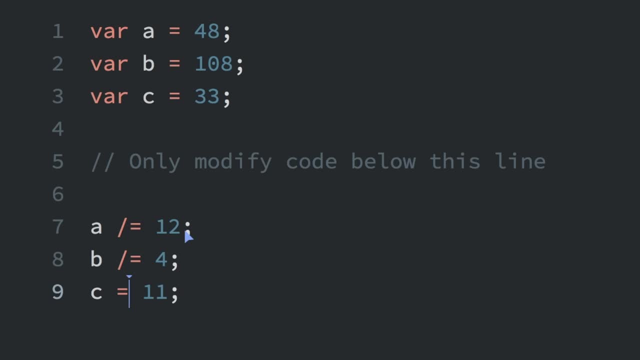 divided by equal four or divided by equal 11.. So another way of just dividing the variable by a new number and assigning that answer to the variable. We've already mentioned strings a little bit, But anytime you have some characters surrounded by quotation marks, they can either be single quotation marks, double quotation marks. 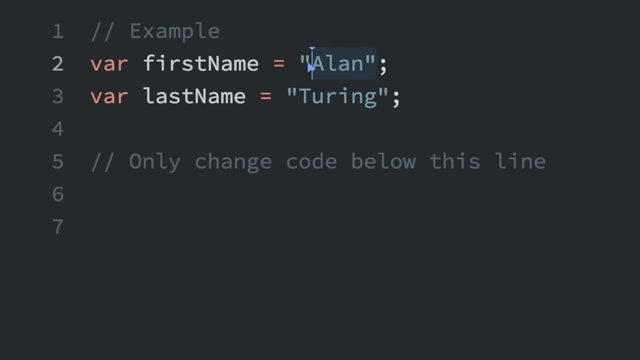 or backticks. It's a string. These are called string literals And you can create them just like you see above. I'm going to do a few more. So var, my first name, equals bow, And var, my last name, equals Carnes. So that's how you create a string in JavaScript. 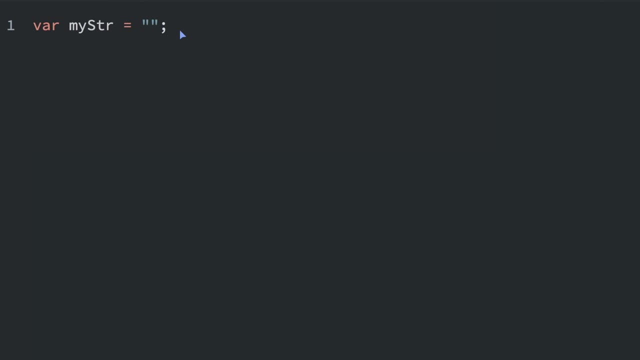 Sometimes your string contains the quote symbol. Now, normally the quotes identify the beginning and the ending of the string. But what if you have something like this? I am a double quoted, spring inside double quotes, So I'm actually trying to use these quotes, right. 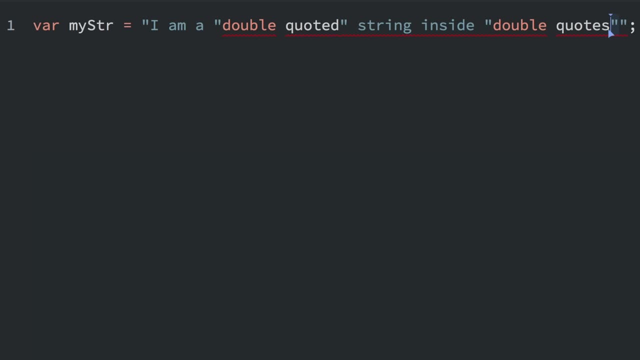 inside the string, But the JavaScript doesn't know what to do about it. It thinks that this is the things, that this is the whole string. When it sees the first quote inside the string, it thinks we're at the end of the string, So there's something called an escape character. 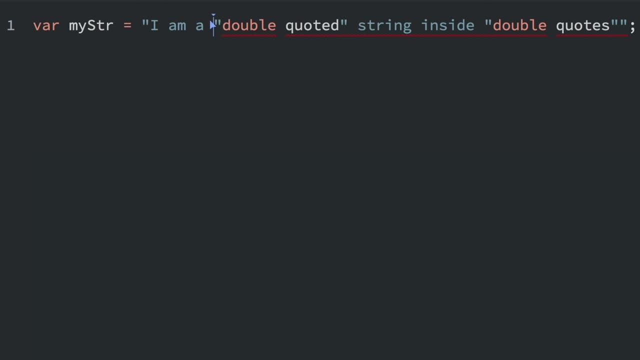 So if you want to escape a quote, that means it will no longer be considered the end of the string, I'm going to put a backslash. So if I put a backsplash, a backslash, before each of these quotation marks, JavaScript no longer interprets it as being the. 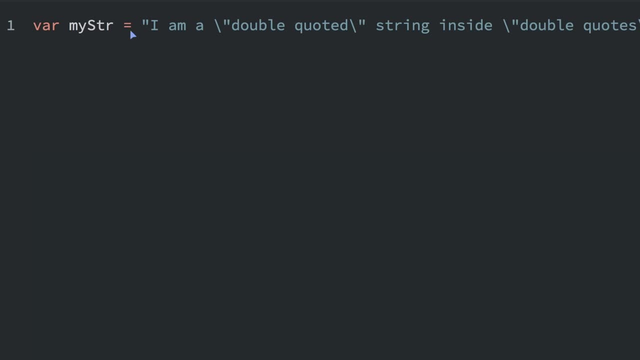 last character in the string. So now you can see this is a full string. And then if I log this out- console dot log- and I put my string, you'll see that it's not going to show the quotation marks. So I mean it's not going to show the slash. the backslash is it shows the. 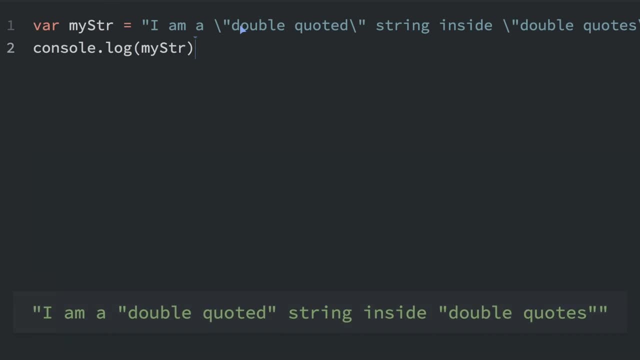 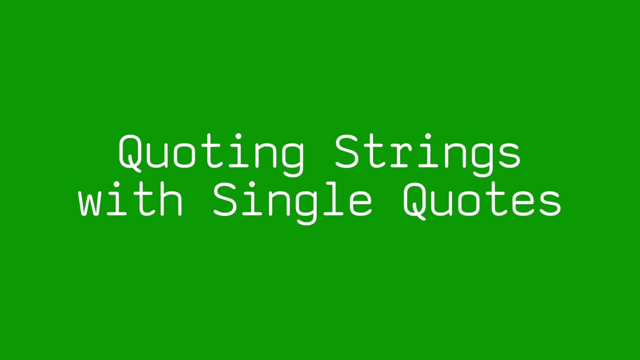 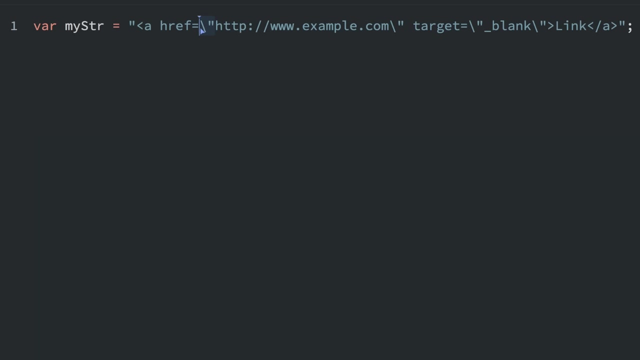 quotation marks. So it's not going to show the slash. the backslash is: it shows the quotation marks without the backslash is because when we put backslash quotation mark, JavaScript knows that this should just mean a quotation mark. We talked about escaping a quote character like this, where you put a backslash before. 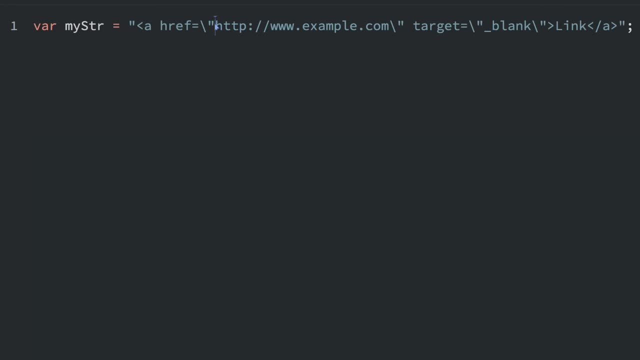 the quote character, So JavaScript knows that this is supposed to be a literal quote character inside the string. However, you're not going to have to escape quote characters very often, because there are other methods of accomplishing the same thing, of having a quote character within. 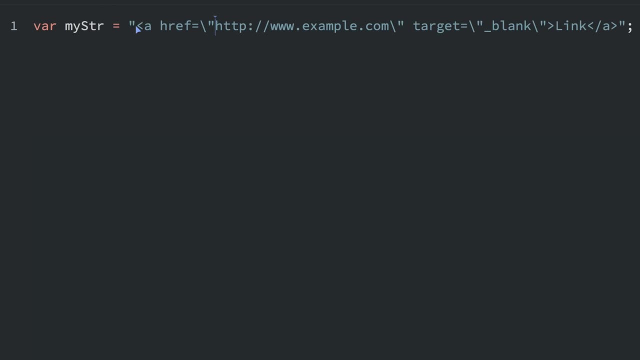 a string. So a common way is to use: instead of having your string start with double quotes, have it start with a single quote. So a string can either be surrounded by single quotes or double quotes. So this time we're just going to have single quotes And now I can remove all of. 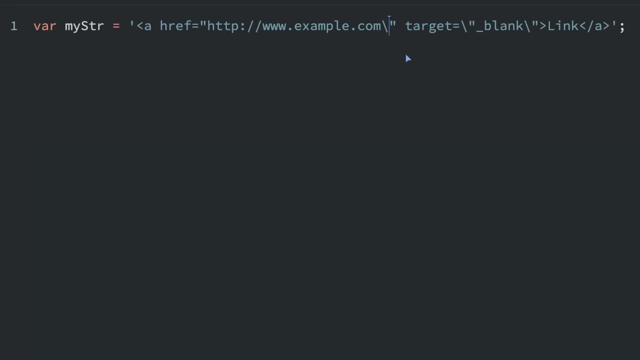 these escape characters from inside the string here. Okay, so now you can see that JavaScript still knows that, knows that this is a string, even though it has these double quotes inside. An additional thing you could do is use backticks. So if I put a backticks before, 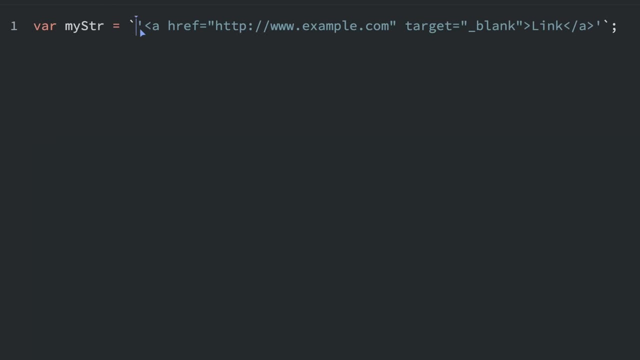 at the beginning of the end of the string. now I actually can use single quotes and double quotes both within the string, But right now I'm just going to focus on showing you the double quotes or the single quotes with the double quotes inside. We talked about escaping a double quote character by using the backslash. 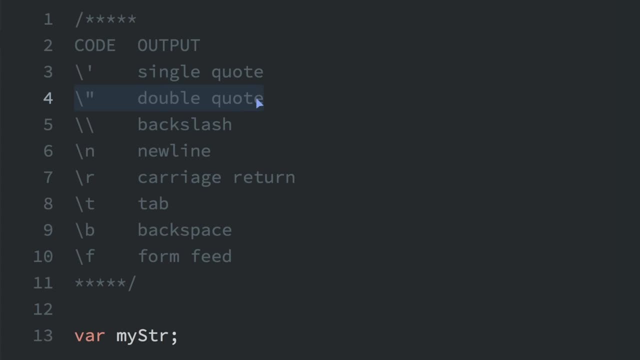 before the double quote, there's actually quite a few other things you can escape out. you can escape out a single quote character, you can escape out a backslash. In fact, anytime you're going to use a backslash, you're going to have to put two backslashes. So the 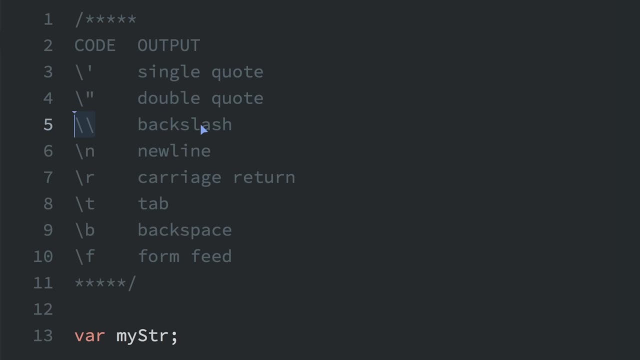 JavaScript knows that you're not trying to escape a character. You can also add a new line character or a carriage, return a tab, a backspace or a form feed, all with doing a slash and the corresponding letter here. So let me show you an example. I'm going to put var, my string equals and we're. 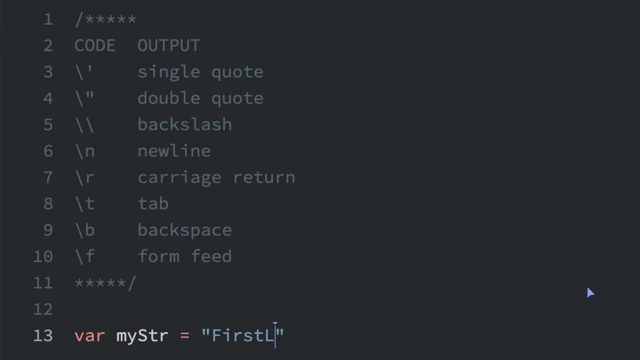 going to make a multi line string. So we're going to have the first line And now I'm going to put backslash in to add a, a second line, and then I'm going to put a tab. So backslash T for the. 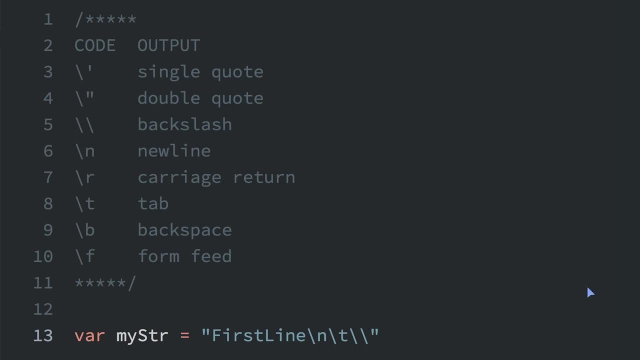 tab and backslash, backslash, to add a backslash. Now it's going to say second line, Now I'll do backslash, And then I'll just say third line. And if I were able to log out all of that, you would. 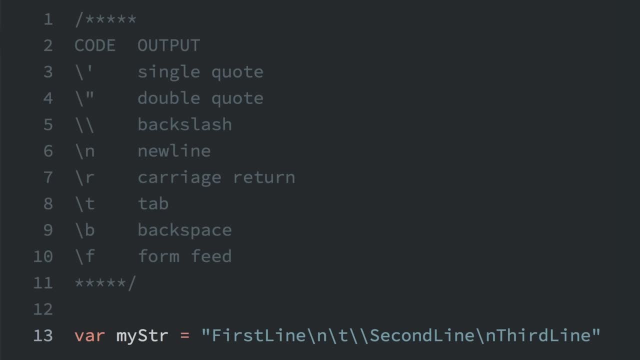 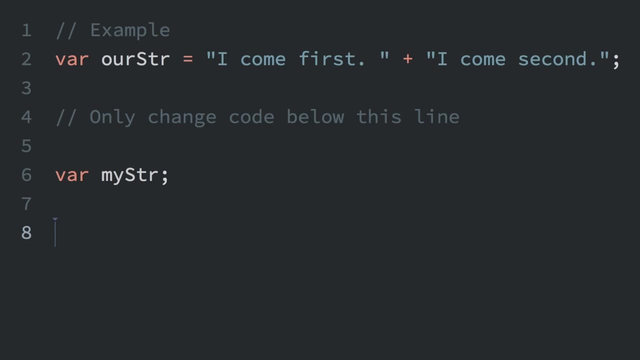 see three different lines And you would see the tab and then the backslash character. You can concatenate strings with the plus operation. You can see here that we have two strings: I come first and I come second. they've been added together or concatenated with this. So the r str, our string, is now one long string that says I come. 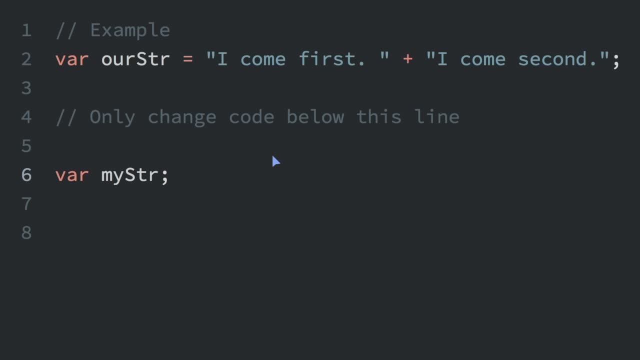 first, I come second. I'll give you another example here, So we can say: my string equals. this is the start, And then I'm going to put a space before the in quotation mark, because when these get concatenated together, we want there to be a space between these two sentences And I'll say: this is the end. Now, 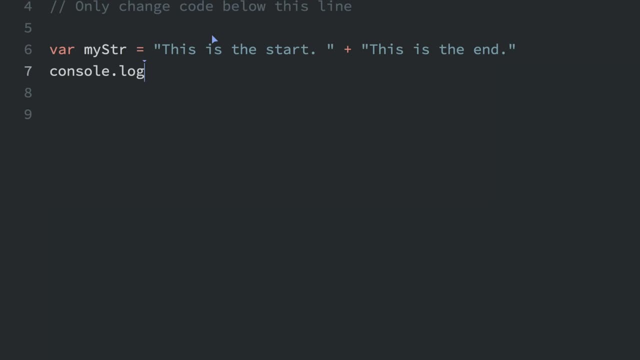 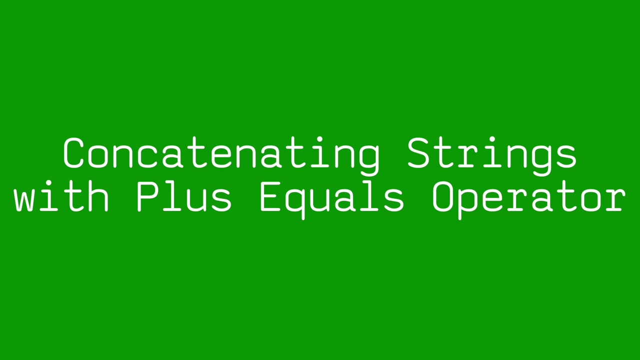 let's just see what that looks like. I'll do a console dot log and do a my string And let's see if I run this. we can see this is the start, this is the end. just one long string You can. 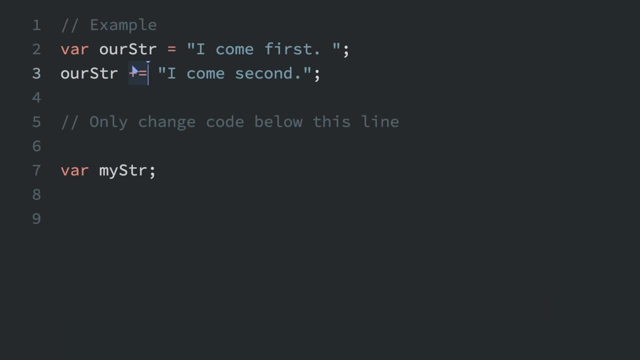 also concatenate strings using the plus equal operator. you can see here in this example, we have the r string- equals- I come first, And then we have the r string plus equals- I come second. So remember, just like in when you're using numbers, plus equals means that 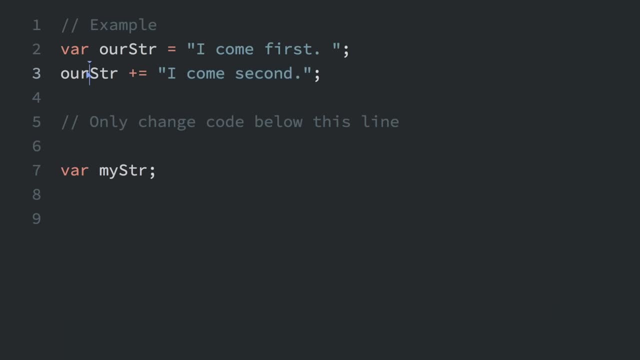 you take whatever is on the end here and add it to the variable. So we've just added I come second on to the end of I come first, And then we have the r string plus equals- I come second. So remember, just like in when you're using numbers, plus equals means that you take whatever is on the end of I come. 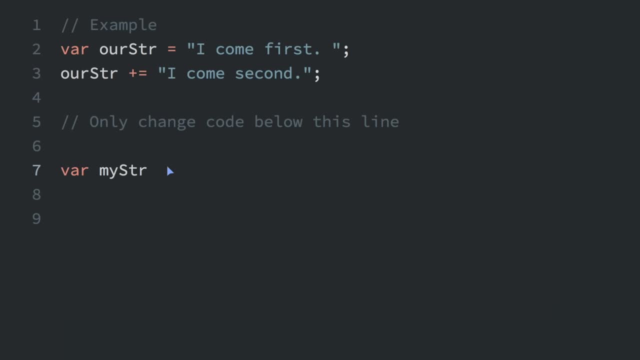 first Let's do another example down here: my string equals. this is the first sentence. And then I'll put a space at the end because we're going to do my string And I'll hear: I'll do the plus equals. This is the second sentence. Now, if I just do a console dot log here of my string, we 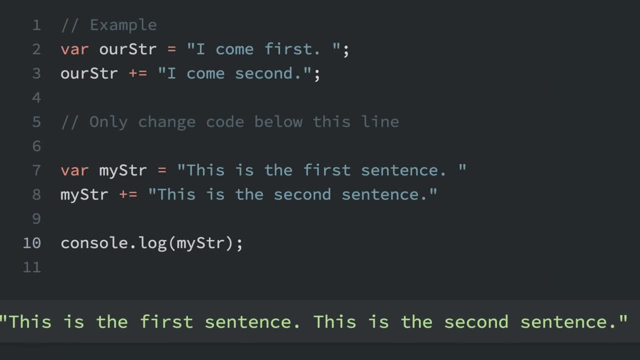 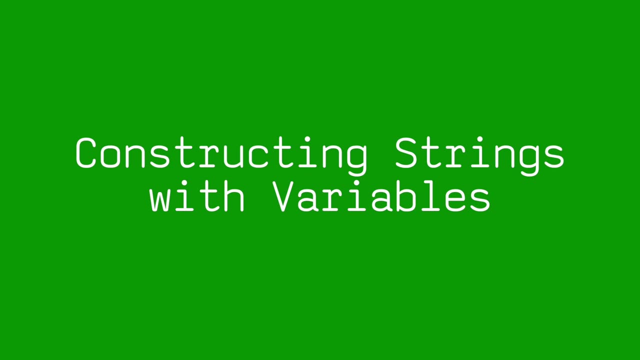 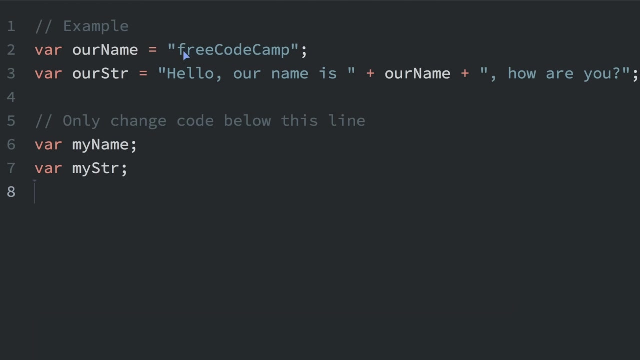 should see that those sentences have gone together. This is the first sentence. This is the second sentence. Good, You can concatenate strings together with variables. You can see here our name, free code camp. Hello, our name is, and then we add this variable to our name variable which is free. 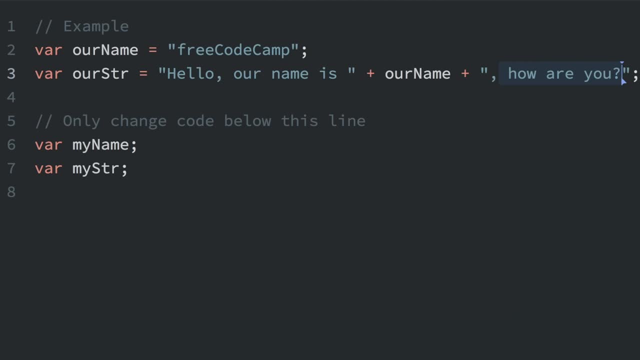 code camp: Hello, our name is free code camp. How are you? Well, we're going to do the same thing down here. So I'm going to do: my name equals bow, And then my string is going to equal my name is, and then I'm going to add the variable name, which is my name, And then 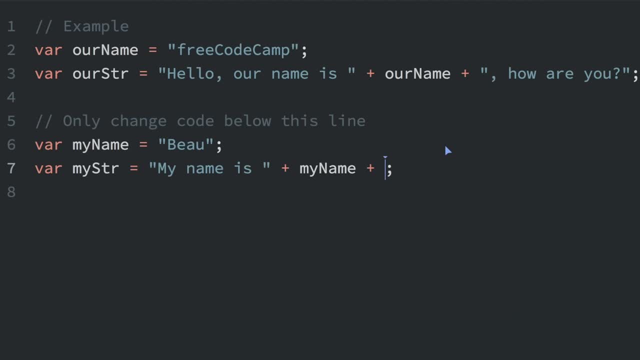 I'll continue the string here. Oops, that's supposed to be a plus here And I am well See that I put a space here and here because you have to make sure you put appropriate spaces in And let's see what that looks like. I'll do a console that log. 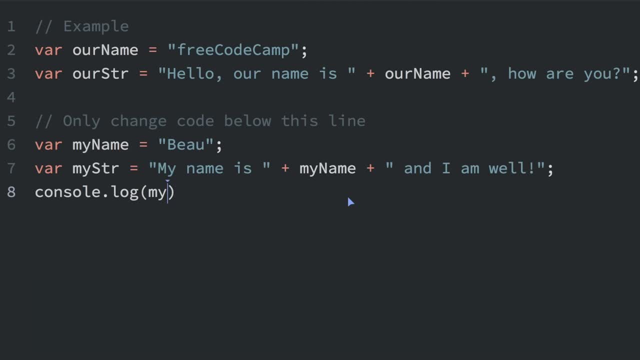 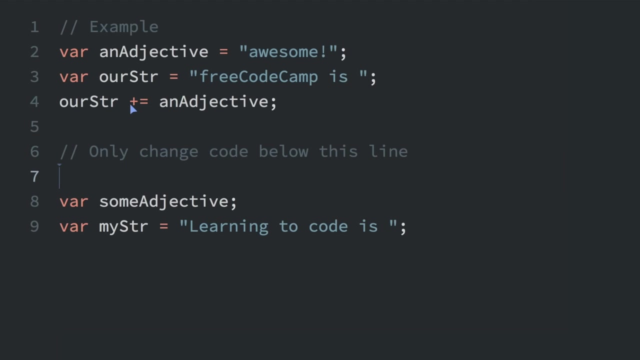 I'll just put my string here. If I show that my name is Bo and I am, well, looks good And you can append variables to strings with this plus equals operator. you can see with this variable and adjective which is set to the word awesome, And then we have another variable free. 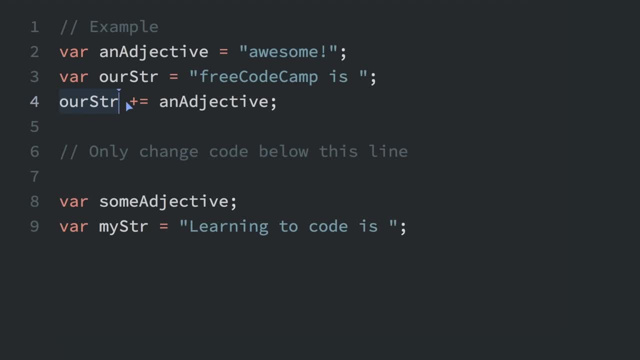 code camp is: and then we have the R string variable plus equal, an adjective. So now our string is going to equal free code camp is awesome. So let me show you another example. We're going to say some adjective equals worth while, And now I'm going to use the plus equals, so my str plus equals. 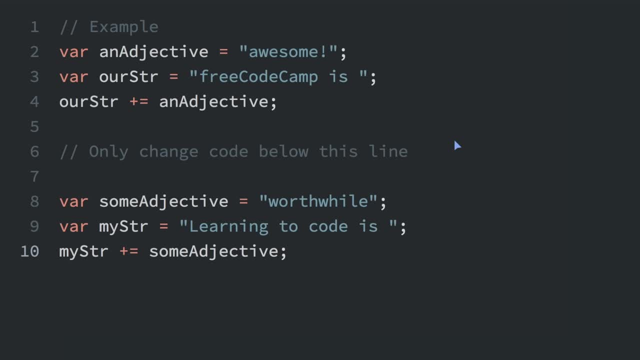 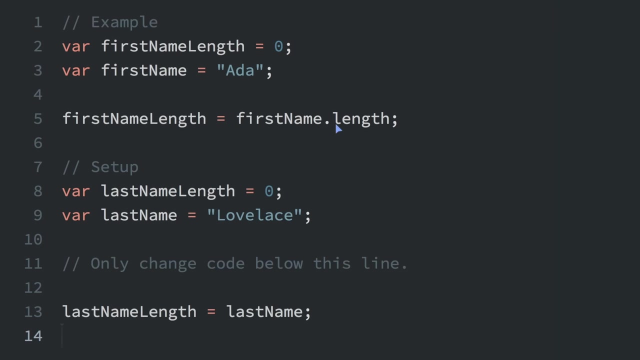 and then I can put some adjective. So now, after we do the, my string plus equals some adjective. my string is going to say: learning to code is worthwhile Sometimes. you want to find the length of a string. you want to find the length of a string. you want to find the length of a string. 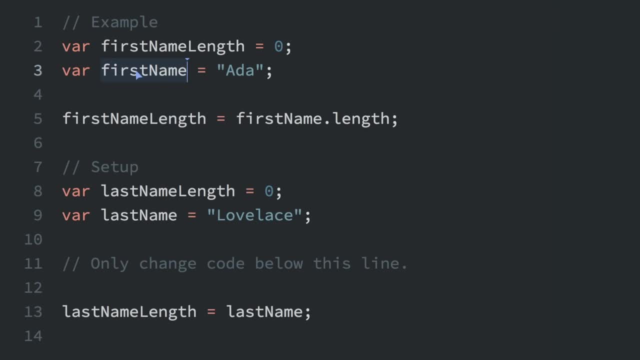 JavaScript makes this easy. So we have the first name is set to add a, but we just use the dot length property to find the length. So first name, dot length- remember. first name is added here and then dot length will return an integer, a number that has the number of characters in the 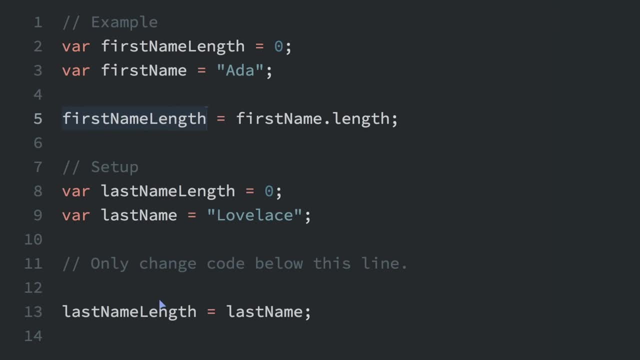 string. So that will be three. So let's try this again. Here's another example: last name length equals last name. we just have to type in dot length And just to show you, let me console dot log that And you'll be able to see if I put in last name length. 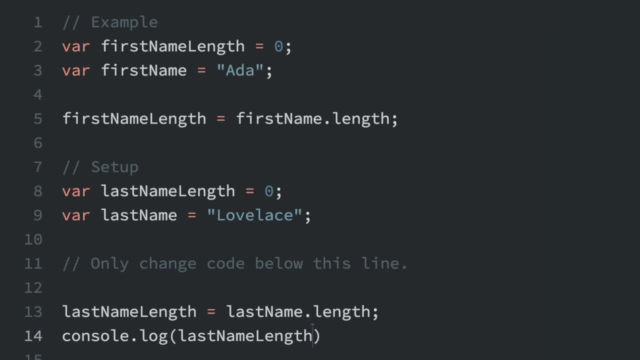 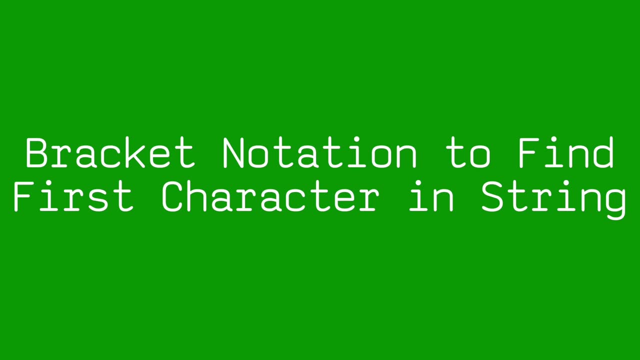 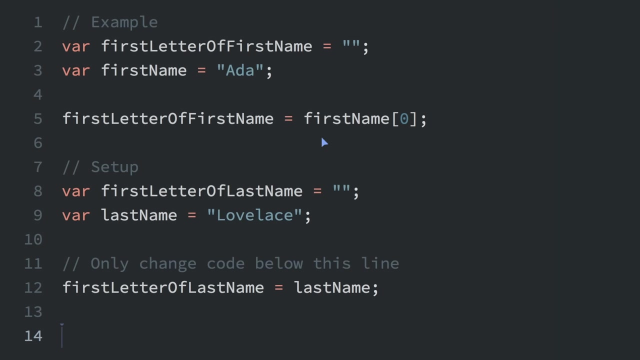 And if I run that you'll see eight, because there are eight characters in the word lovelace. bracket notation is a way to get a character at a specific index within a string. So you can see: right here we have the first name, add a and right here we have first name. And then here's. 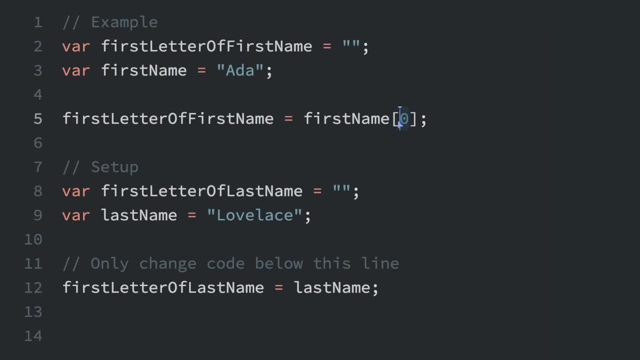 the bracket notation you can see there's brackets with a number inside. So most modern programming languages, like JavaScript, don't start counting at one, like humans do. They start at zero, which is called zero based indexing. So with the number zero that refers to the, in the first index of the 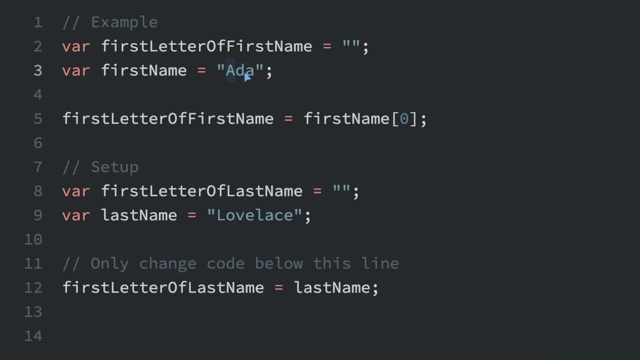 string which would be the A. So the A would be zero, D is one and then a is two. So this first letter of first name, if we do first name with the bracket notation with a zero, that's going to equal. 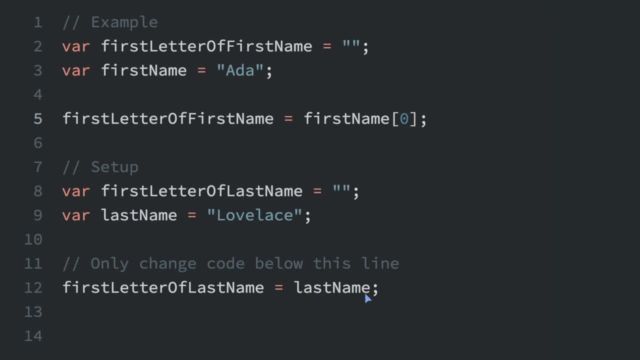 a. So let me show you another example. Let's say we want to get the first letter of the last name. Again, I'm just going to do the bracket notation and put a zero here. If I want the second one, we want the second letter of the last name. Definitely one will do that And I know I'm going. 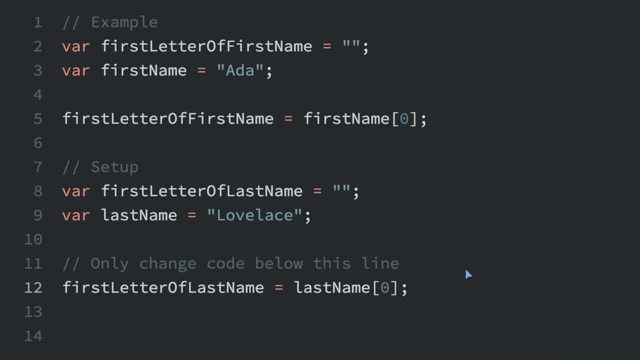 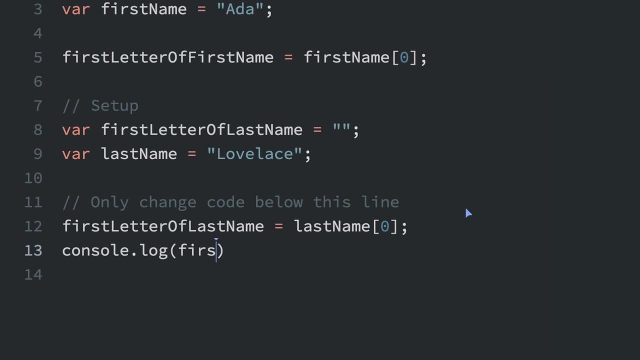 letter, the O, I will put a one here. So if I console dot log we can see what it came up with. So console dot log, first letter of last name. And if we look in the console L, because the 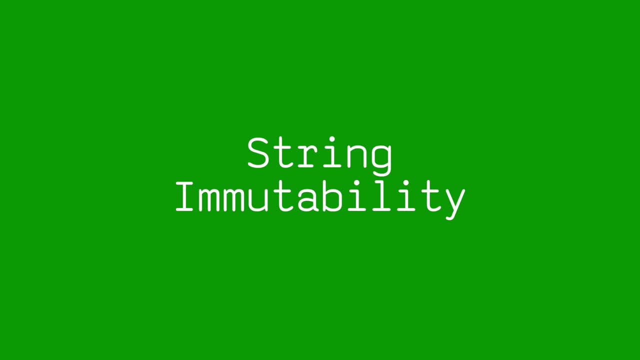 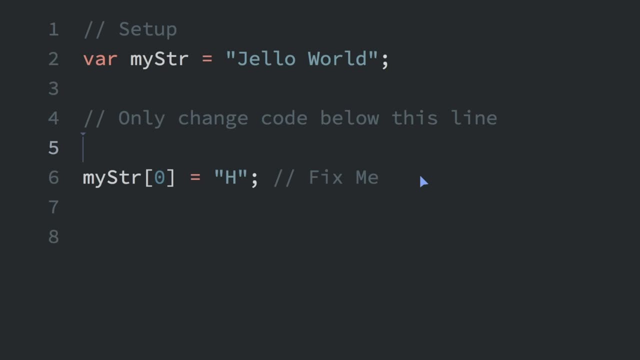 first letter of the last name is L. Strings are immutable, meaning they cannot be altered Once created. this does not mean that they cannot be changed, just that the individual characters of a string- literal- cannot be changed. So look at this example- my string- and then we're going. 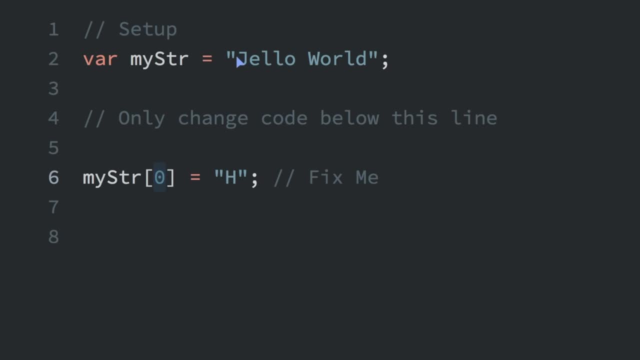 to use bracket notation to choose the first letter. So it currently says jello world. we want the first letter to change to an H to say hello world. But if I run that there's going to be an error because of the immutability of strings. Now we can still change this thing. 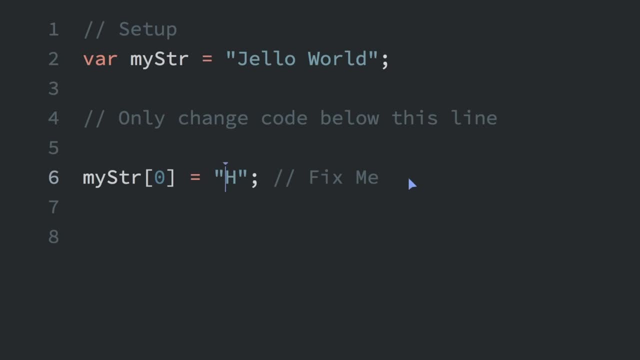 the Hello world. but we can't just change an individual letter like that. So we're going to have to do my string equals and I'm just gonna have to type in the whole thing which is Hello world, And now it we will change to the word Hello world. You can use bracket notation to get 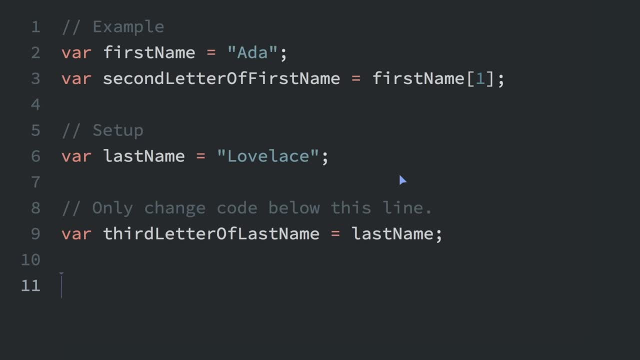 any character position in a string. So earlier we did the first position, But here's the first. how you get the second position: mirror: the zero index. So one is the second position, zero is the first position. we can also get the third letter of the last name using the brackets. we'll just. 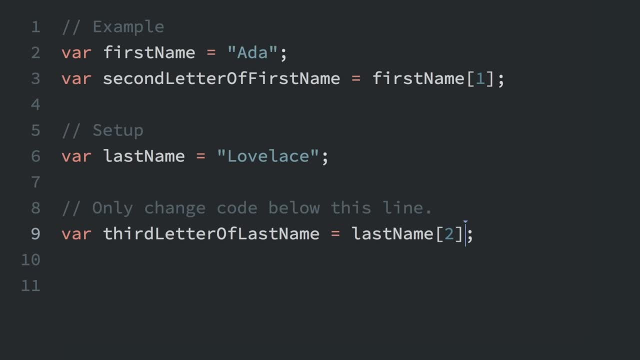 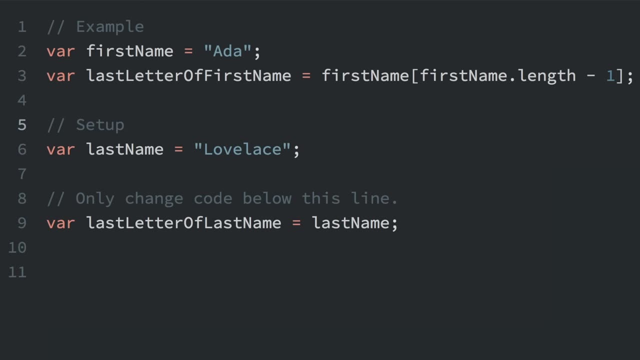 put two in the brackets to get the third letter of the last name. You can also use bracket notation to find the last letter in a string. Even if you don't know how many letters are in the string, you do it based on the length. 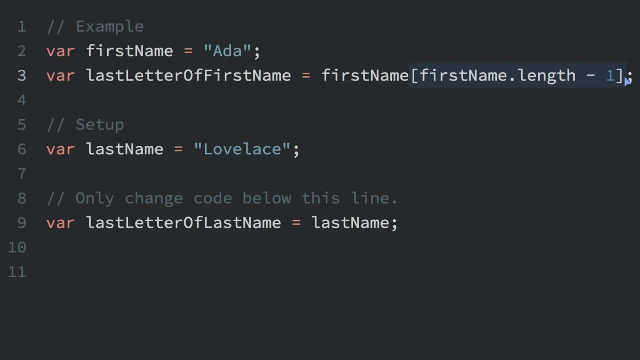 So if you look right, here in the brackets, we have a, an expression to be evaluated. first name: dot. length minus one. So the length is three. three minus one is two. The reason why we're doing a minus one is because, remember, we count starting at zero. So the link minus one is going to be the 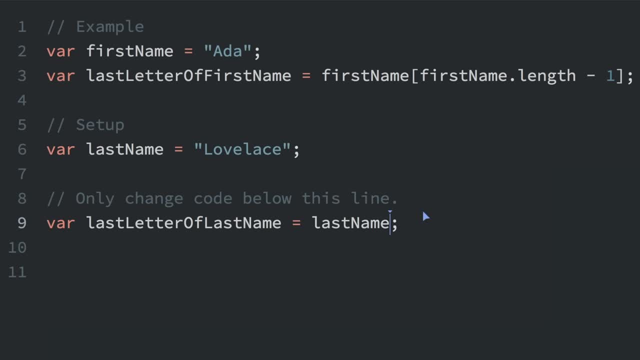 last index of the name. So we can do that same thing here To get the last letter of the last name. I can just do last name dot length minus one, And that's going to get the last letter of the last name, which is: 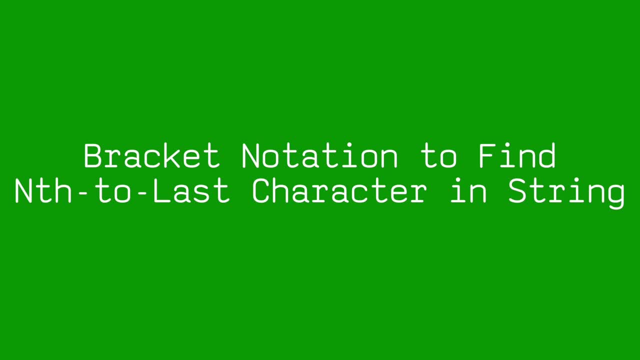 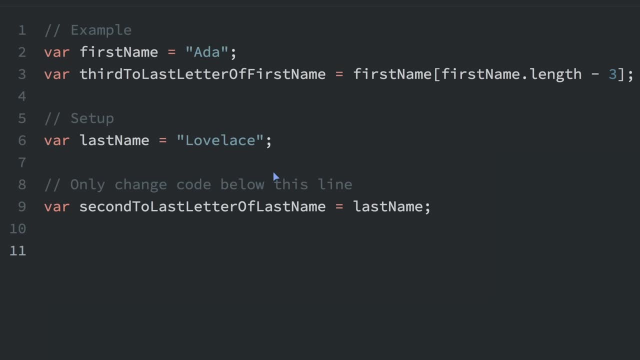 the E right. here We saw how to use bracket notation to get the last letter of a string. You can also do the third to last letter or fourth to last letter. So you just subtract however much you want from the for the length of the string. So we have the bracket notation. first name: dot length minus three. 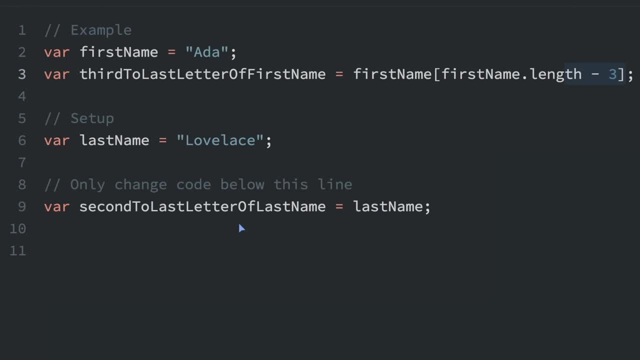 that's going to get the third to last letter. So we want the second to last letter into this variable. here we do something similar. we just do last name, dot length, And then we're going to subtract two to get the second to last character of the string. We are going to use our knowledge. 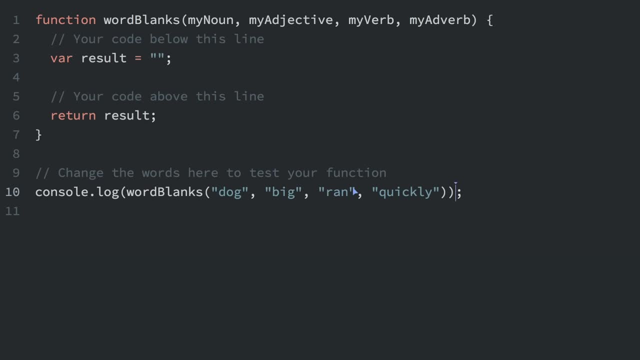 of strings to build a Mad Libs style word game. In a Mad Lib game, you are provided sentences with some missing words like nouns, verbs, adjectives and adverbs, And then you fill in the missing pieces with words of your choice to make a sentence that could be funny and hopefully makes. 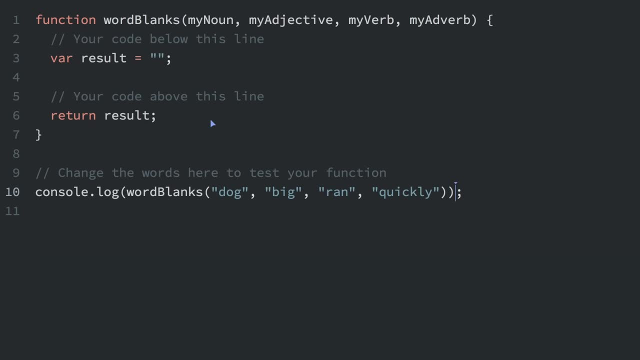 a little bit of sense, So let me show you how you do this. This also uses a function. Now, we haven't talked about functions yet. I'm going to explain how to use a function, So let's go ahead and let's play those more later. But for Matt, for now, just go with it, because that's not the point of 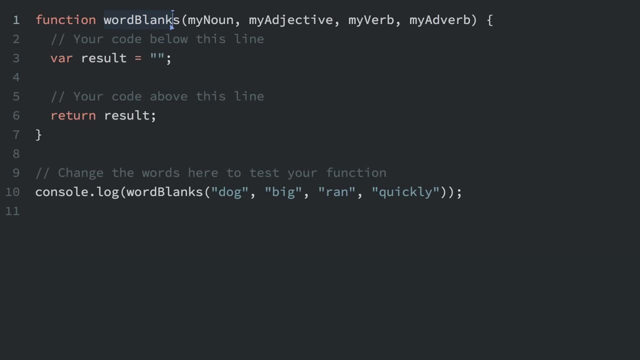 this lesson for now. But this function called word blanks, you can call the function and you have to pass in certain types of words. you pass in a noun, an adjective, a verb and an adverb. So down here you can see that we're calling the function called word blanks. that's the function name here. 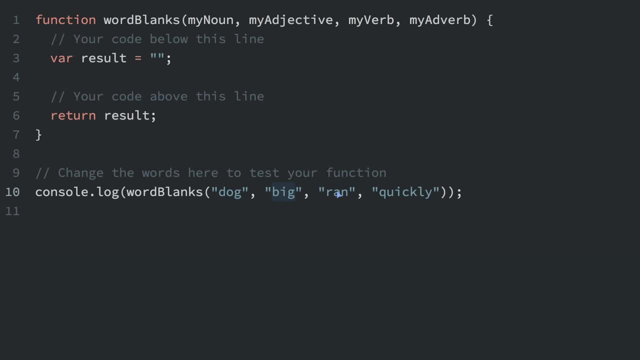 and we're passing in a noun, an adjective, a verb and an adverb. So the point is that we are going to use all these words that are passed in to make a sentence. So we know that var result equals an empty string at first. 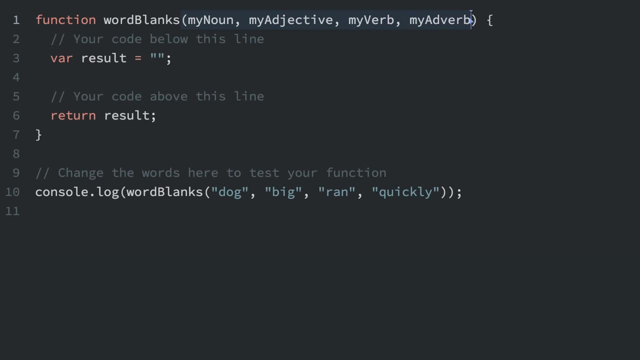 and then we have to use all these words and result, And then the result is going to be returned from this function And eventually will be logged out onto the screen with this console dot log. So what I'm going to do here is do result plus equals. we're gonna use the plus equals to add something. 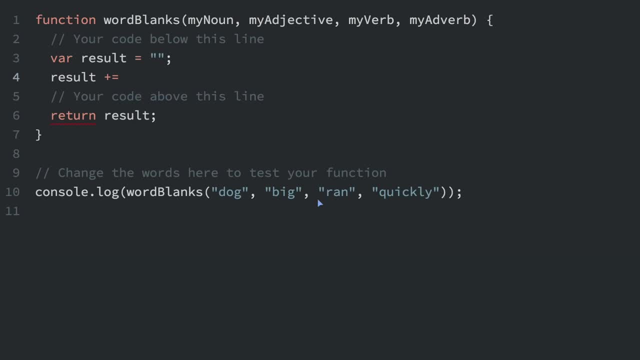 to this result using all the noun, the adjective, the verb and adverb. So let's see, it's gonna say the and we'll use the adjective, I adjective, This case will be the big, the big. and then let's put the noun, my noun, because adjectives are words that describe nouns. 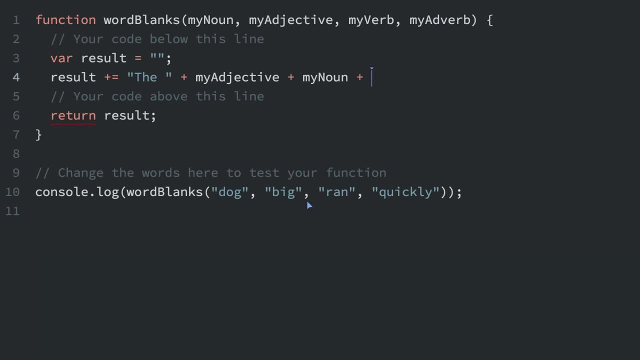 a big dog. And then we're going to say what this now is doing, the verb, my verb, the big dog ran. And then what? where does he run to? to the store. And then we're going to add: Oh, we need a space here, So there's a space between this to the store. And then we're going 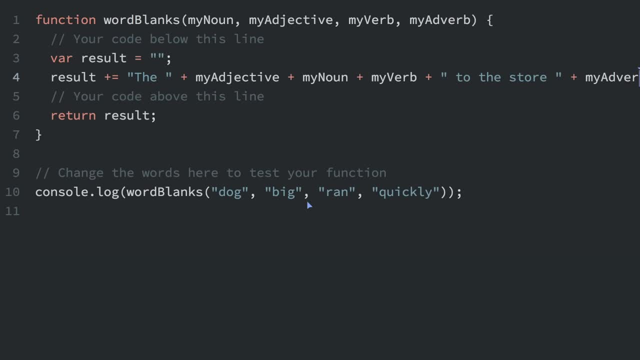 to add the final adverb. So now we have to add a period And there's one more thing we have to add or a few more things. So right now this my adjective, my noun, my verb, and there's no spaces in between those. So if I run that, you can see what that's going to look like in the console. 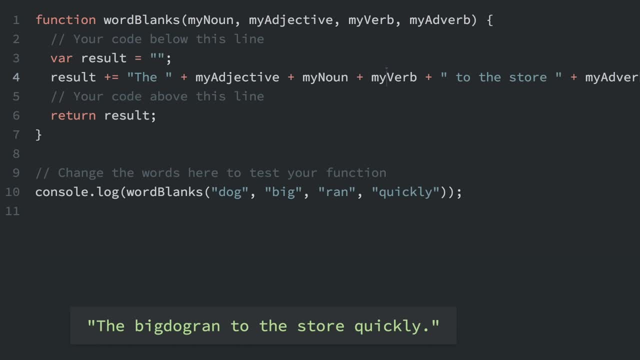 It just said: Big Don, big dog ran with no spaces, So we're going to have to add some spaces in here also. Let's do that Now. it's going to take in the noun, adjective, verb and adverb and then put it. 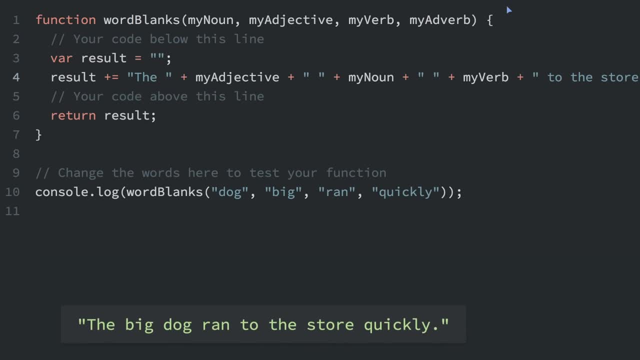 into that sentence. So one cool thing is we can actually pass in some different words, So like, for instance: if I copy this, I'm going to paste it. instead of dog I will put for the noun bike and an adjective I'll put slow, And then for the verb I'll put flu And the adverb 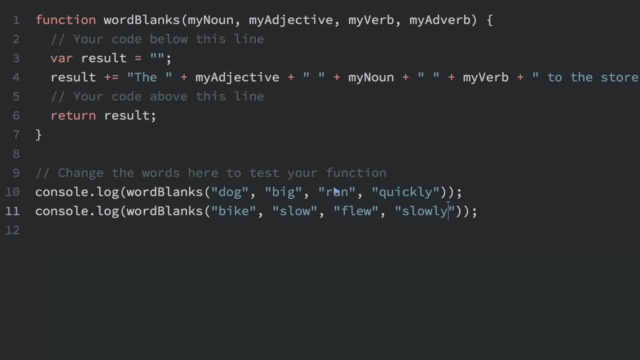 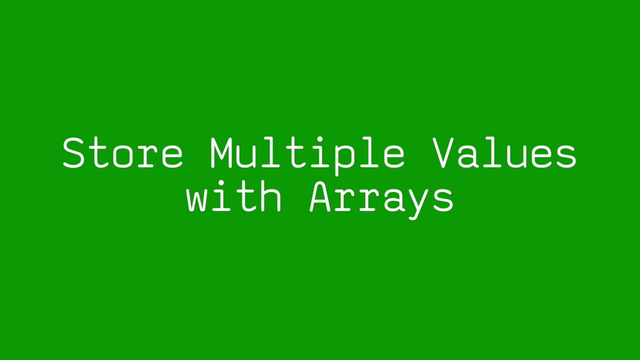 I'll put slowly. Okay, and now, if we look in the console, we have to work two sentences. the big dog ran to the store quickly. the slow bike flew to the store slowly. arrays allow you to store several pieces of data. 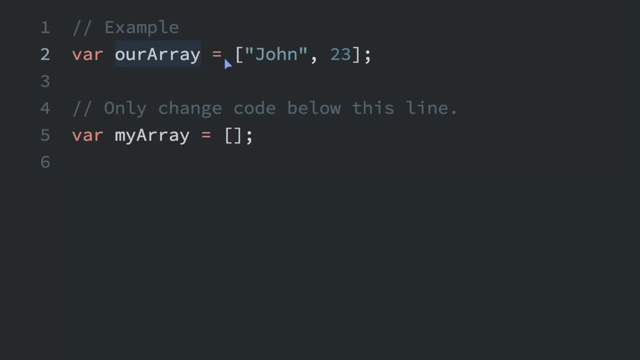 in one place. So look at this example, our array. Now, arrays always start with a bracket and then end with a bracket to show the beginning and ending of the array. And every element in the array is separated by a comma. So you can see here we: the first element is a string, the second 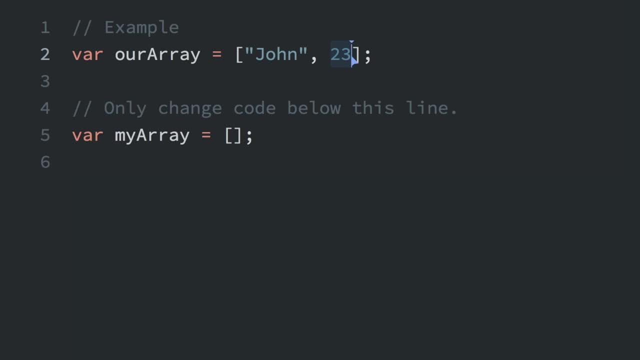 element is a number And you can have more and more elements. you just put comma and you can keep adding elements, And the elements can be any data type. you can see, here we have a string and a number, But you can always also use arrays or floating numbers or really any sort of other data. 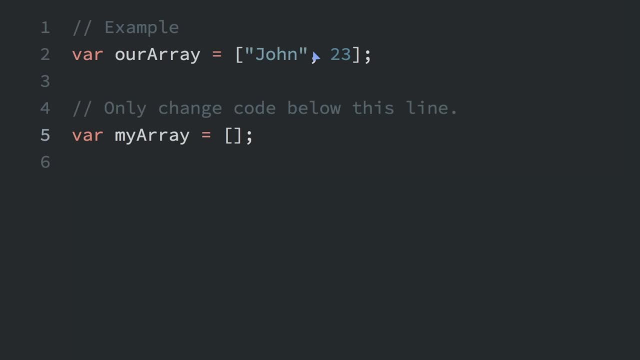 type in your array. So let's see another example. So let's do my array Quincy, And then for a number we'll do one, because Quincy is number one. When one of the elements in an array is another array, that's called a nested array. 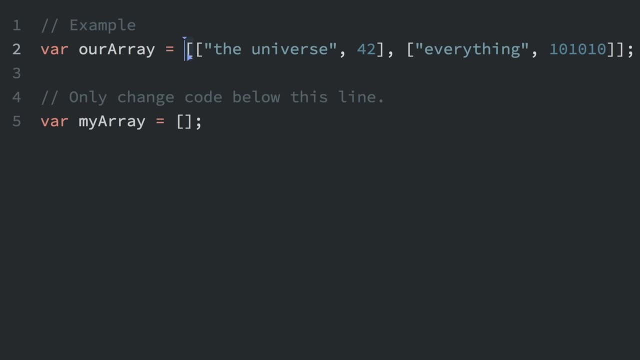 or a multi dimensional array. You can see here's the beginning of the array And here's into the array. But the first element in this array is another array with two elements of its own, Same with here. the second element is an array. So this is two arrays within another array. 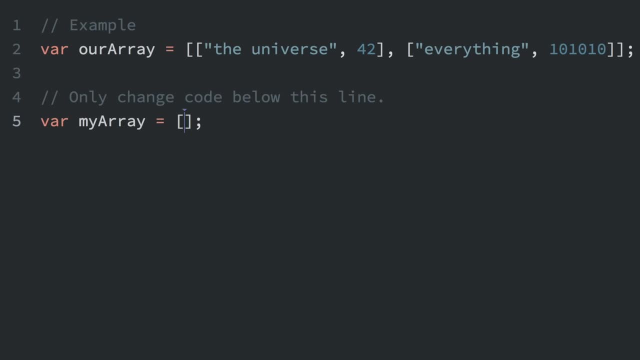 So we can do that here. Here's another example. So let's, our first element in the array will be an array with a string and a number, And then I'll put a comma to put the second element of the array, which will be another array with a string and a number. 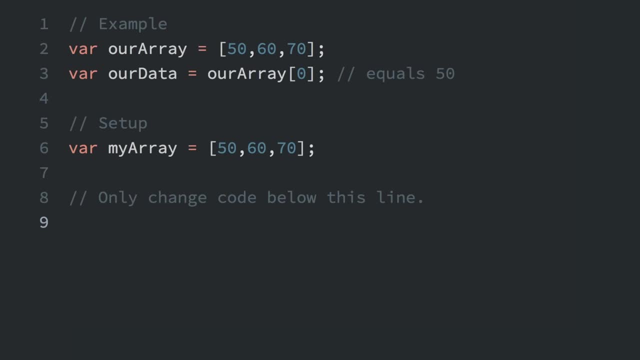 Earlier we learned how to use bracket notation to find a specific index in a string. you can do the same thing with arrays. So look at this array, our array. we have three elements: 5060, 70. And these have the indexes 012.. So with this, our array, with the bracket notation in the 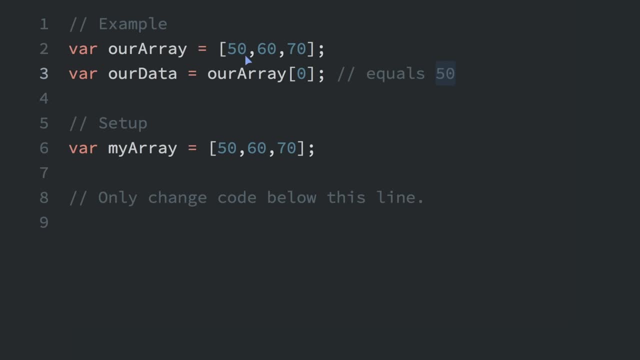 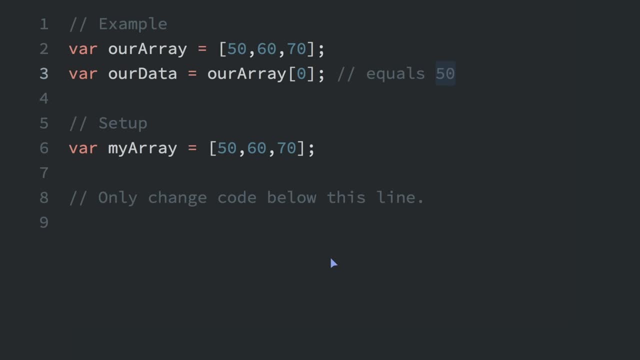 My array equals 5060, 70. So let's try to find the first element in that array. So var r, my data equals my array, And then I'm going to do index zero. I could do index one, index two, And then. 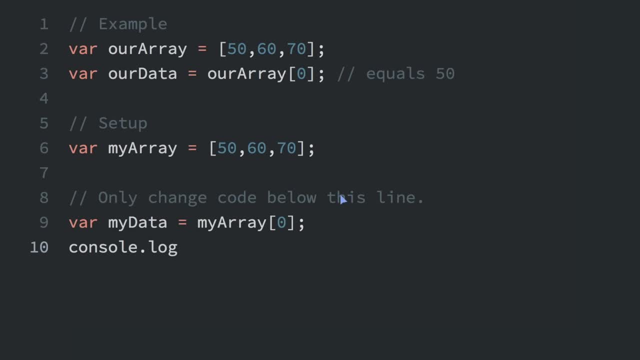 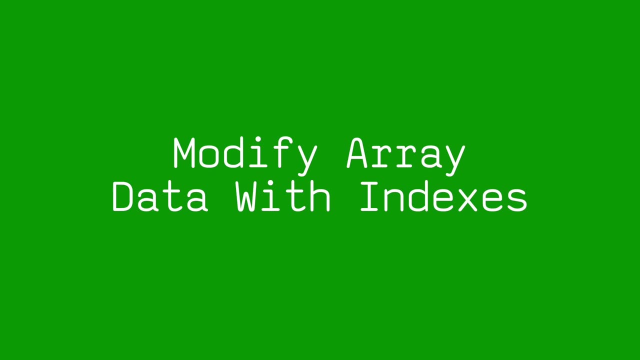 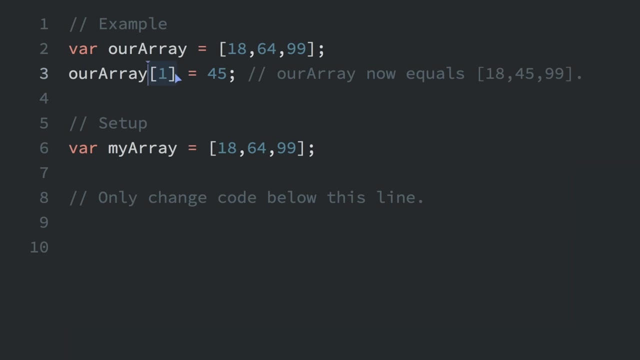 if we console dot log that we can see for sure what that is. So if I put my data and we can see in the console, it's 50.. You can use array indexes to modify arrays. Now we tried to do this earlier with strings using. 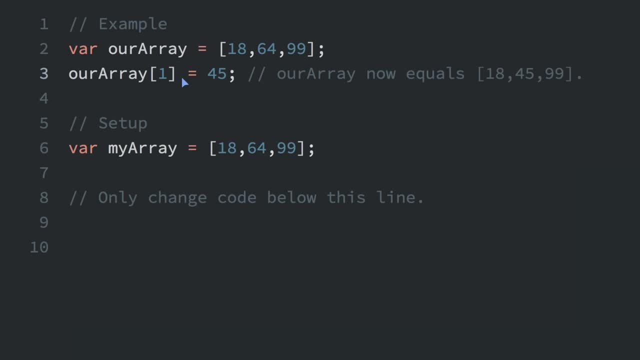 bracket notation And we were not able to modify a string using bracket notation, But with arrays you can. So the original array is 1864 99.. And then we're going to use the array index of one. Now, one is going to be the second number. 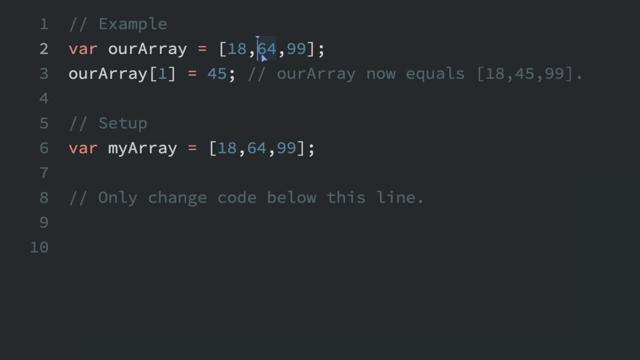 012.. And this number 64 is going to be set to 45. So the new array is going to be 1845 99.. Let's try it again with this 1864 99.. So let's do my array And then, instead of doing the first, the 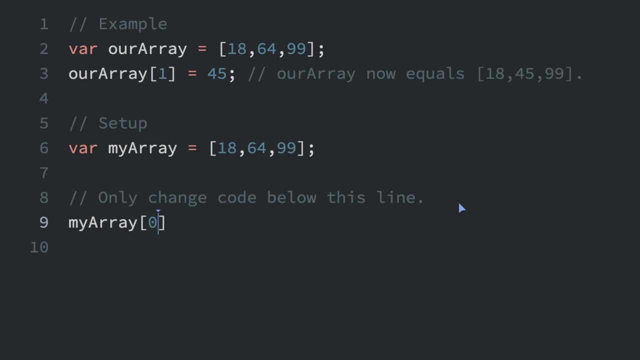 second digit. I'm going to do the first digit and the array, the first index, which would be index zero, And I will say equals 40. 45. So now this array has been updated. So if I do console dot log and then do my array, we'll see. 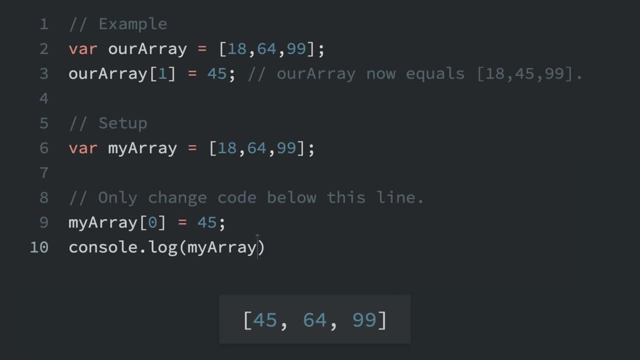 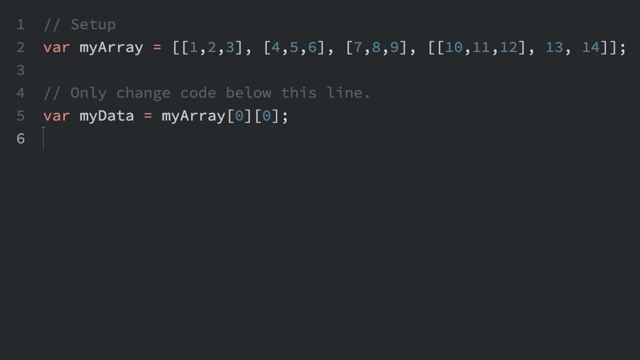 that the array is now 456 499.. You can also use bracket notation to select an element in a multi dimensional or array of arrays. So you can see this array. here we have our outer array, But inside that array are more arrays, the elements of the array or other arrays And the. 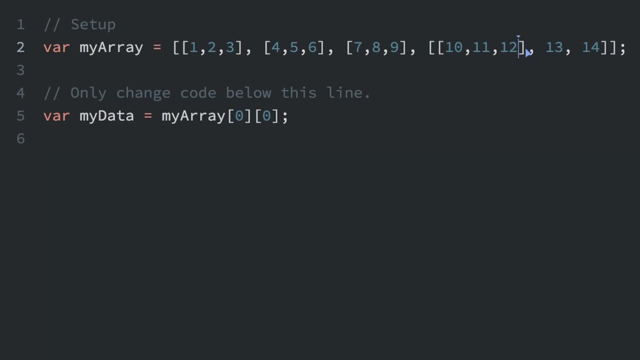 last element of the array actually has an array in this. So this is a three layer deep array right here. So to access an array of arrays or an element within an array, that's within an array, you use a double bracket notation. So if you see this example here, my array, the first bracket, is: 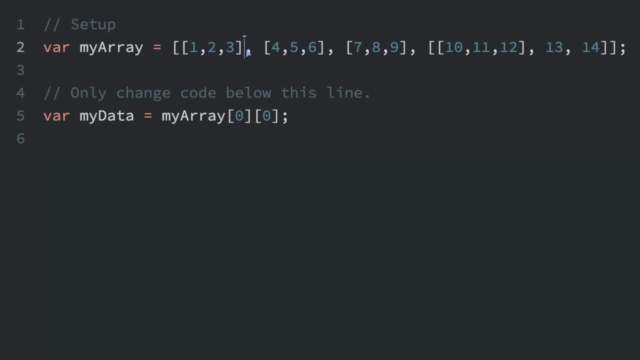 zero that's going to get the element in the array, which would be right here, And then that element is an array. So the second bracket would be the index of the array within the array. So this zero will point to here. So 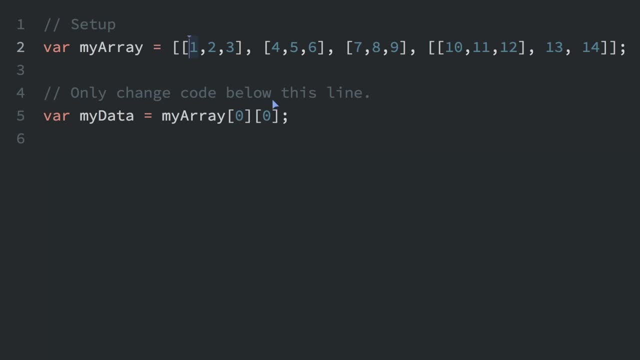 let's try to figure out how we can select a value equal to eight. Well, let's see, I see an eight right here. So let's figure out what this first number should be. Well, let's count 012.. So the 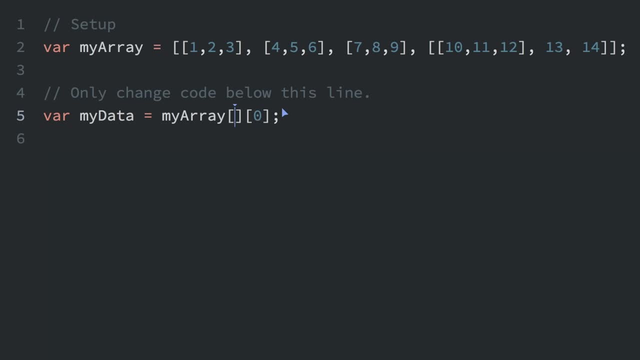 third array would be index two. Now we want to go 01.. Now we have to do index one to get the second number in the third array. So let's test to see if that equals eight. So I'll do a console dot log. 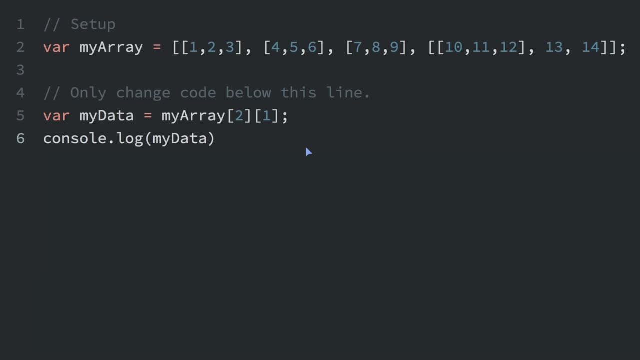 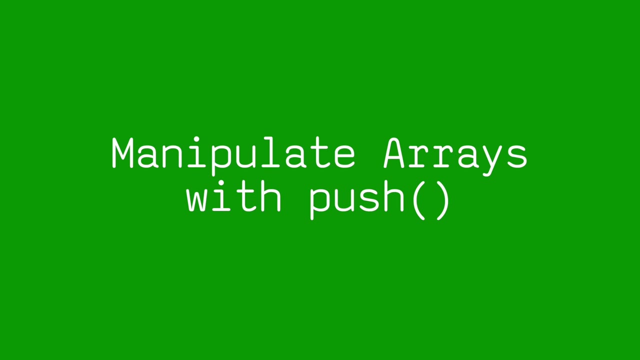 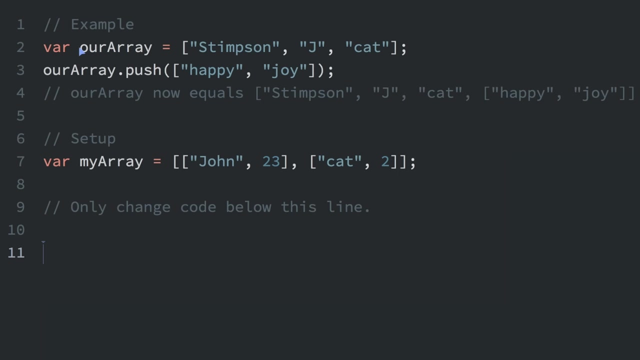 and then do my data here And we'll see if that equals eight. It does, we did it. you can append data to the end of an array with the push function. So C and array has been set up here, our array Stimson J, cat and then we. 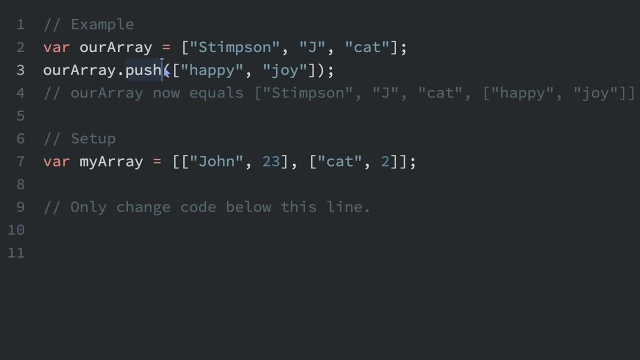 take our array right here and use the push function to push into the next element in the array- another array here. So now it's going to look like this: we can see at the end of the original array we've pushed this other. 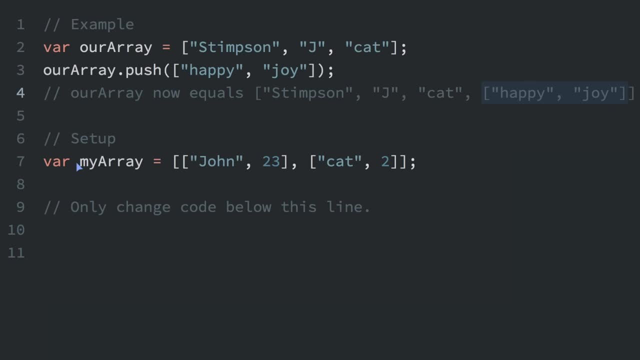 array at the end. So let's try it again. down here we have my array And you can see what we have. each element in the array is another array. So I am going to do my array dot push And then I can push something on the end here which will be like: above another array. So this is going to 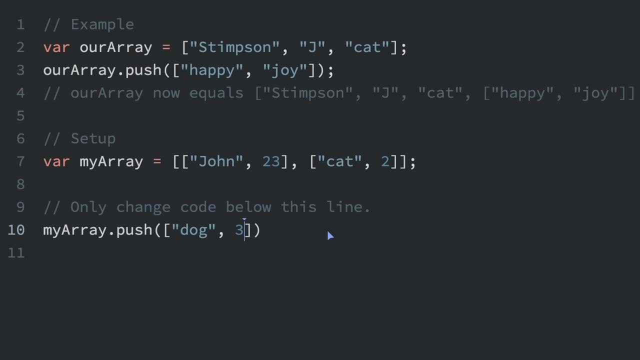 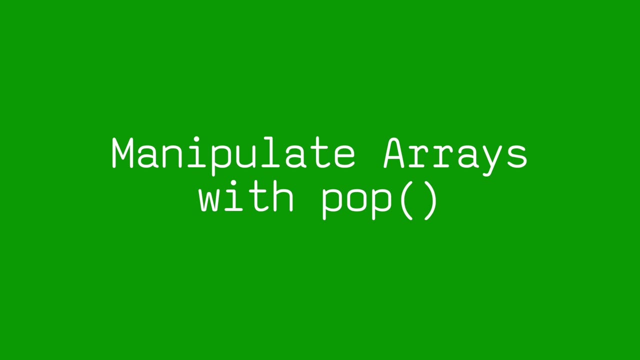 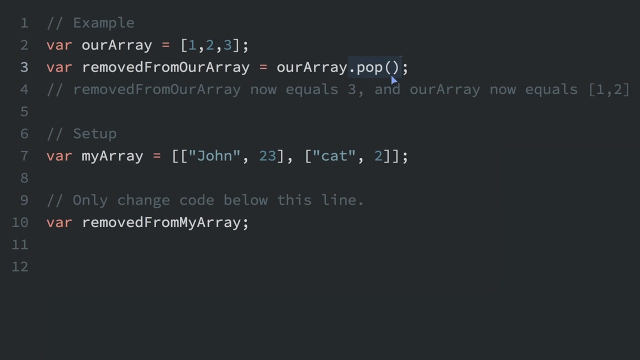 say, dog, I'm a three. And now we've pushed this on to the array. We can remove an item from an array with the pop function here. So see this pop here. And then we know it's a function because of the parentheses at the end of the word pop. So the array starts with 123.. So now we do this array dot. 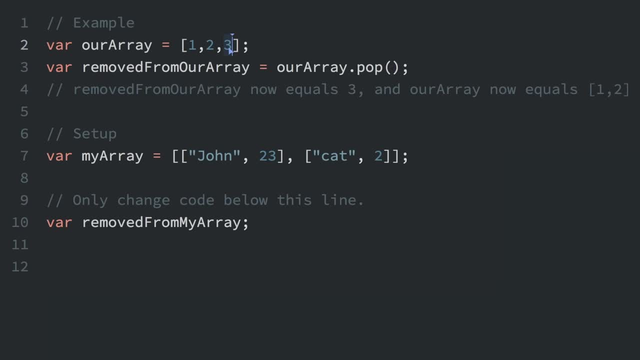 pop and it's going to return the, it's going to remove the last element, which is the three, and then it's going to put it right into this variable here. So now, as you can see down here, remove from our array now equals three, and then our array is. 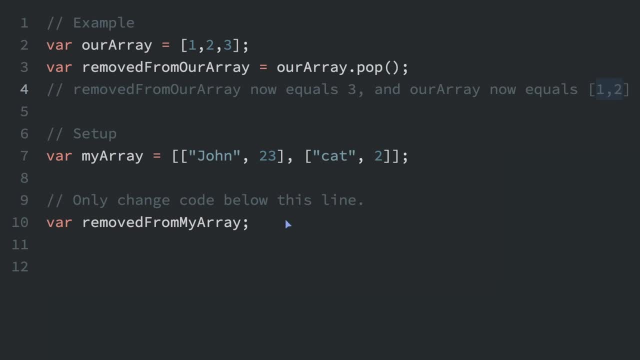 going to equal 12, because the three has been popped off. So we can do the same thing here. So remove from my array equals. I'm going to do my array dot pop And we can see what the array is going to equal now if I just do console dot. 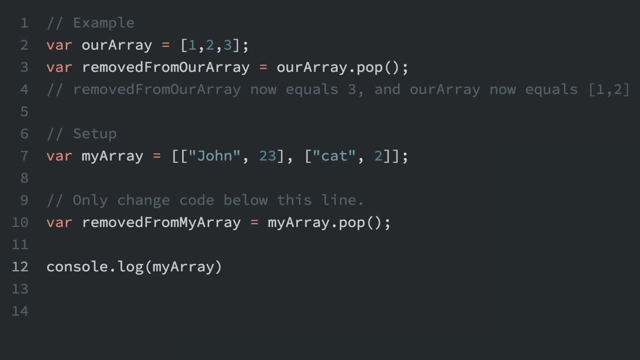 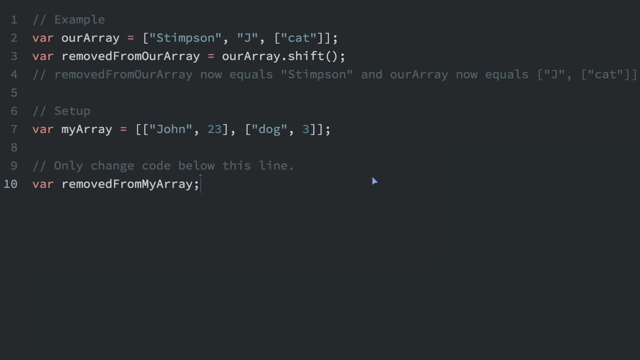 log my array And if you do this, we can see that the array only has the one item, the one array, instead of the two arrays. The shift function is very similar to the pop function, except it removes the first element of the array instead of the final element. So we see the shift function on. 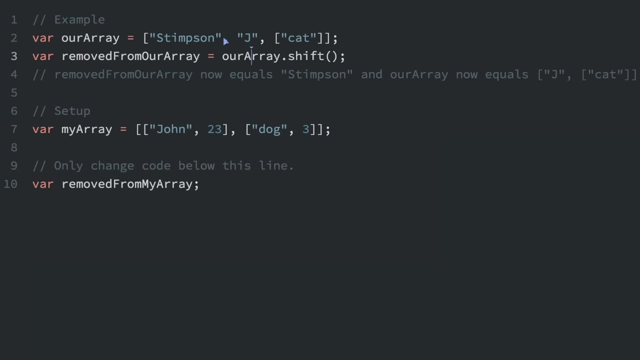 the end of the array here And the array is the same as before. But now the first element, Stimson, is being removed. After we shift off the first element, the array is going to equal J cat and the removed from our array is going to equal Stimson. So let's do another example. 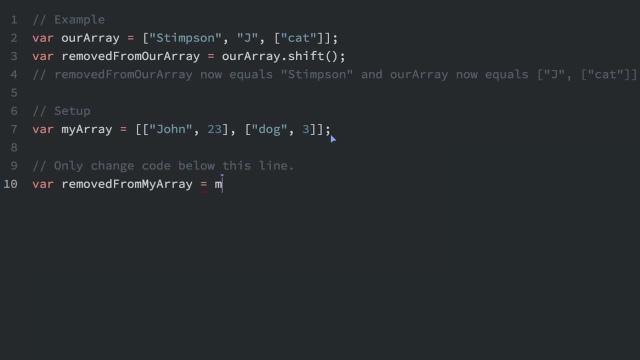 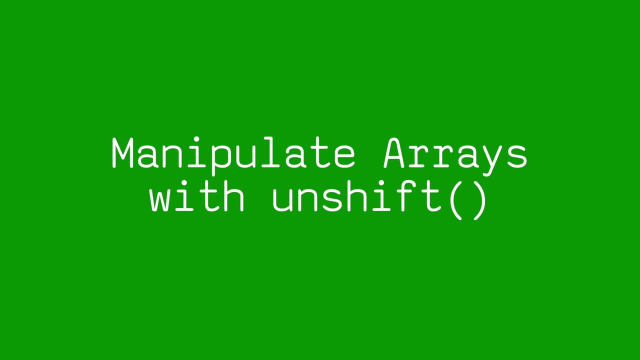 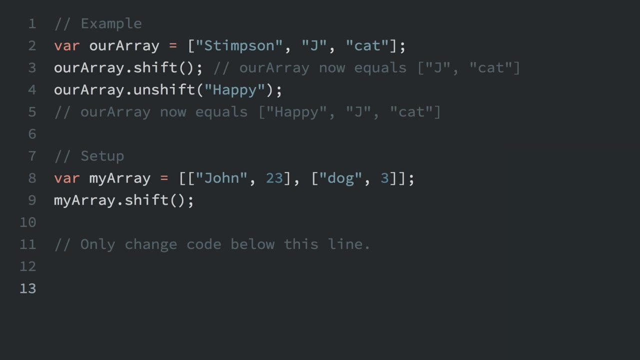 down here we're going to do a shift again, So I'm going to do equals my array dot shift. And now the my array is just going to equal dog three and the removed from my array is going to equal John 23.. The unshift function is similar to the push array function, While push adds an element to the 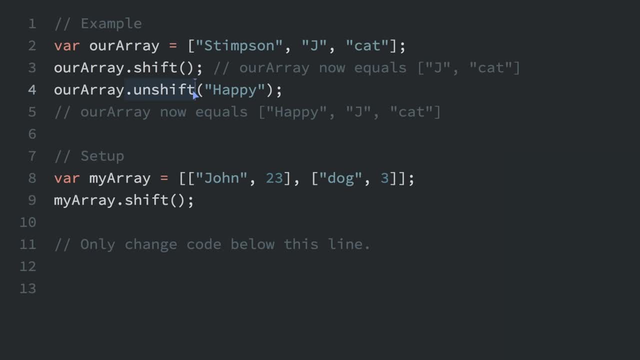 end of the array. unshift adds an element to the beginning of the array. So let's look through this example code. we have the array Stimson J cat. we're going to shift off the first element, remove the first element. So our array is J cat. Now we're going to unshift. 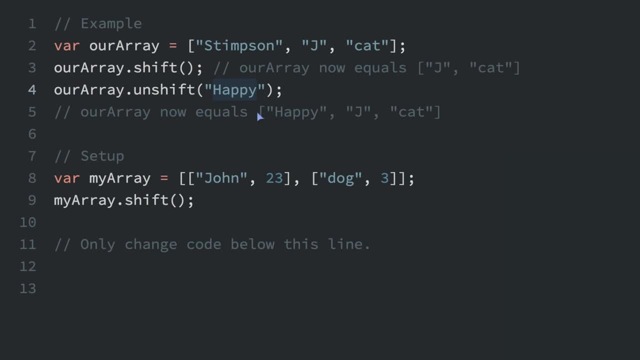 or add an element at the beginning, which is the string happy. So the array will now be happy, J cat. So let's try again. This time the array is john 23,. dog three: because of the shift, we've shifted off the john 23.. And now I'm going to unshift something, So I'll do my array dot unshift. 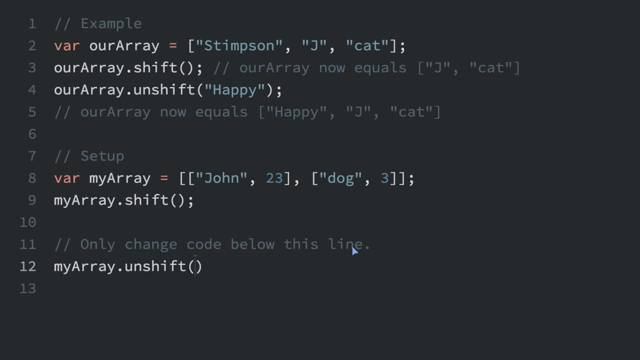 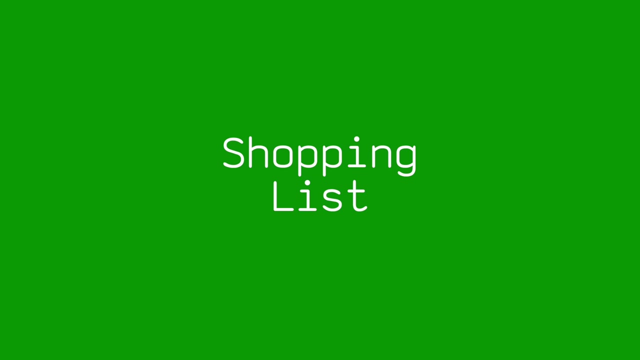 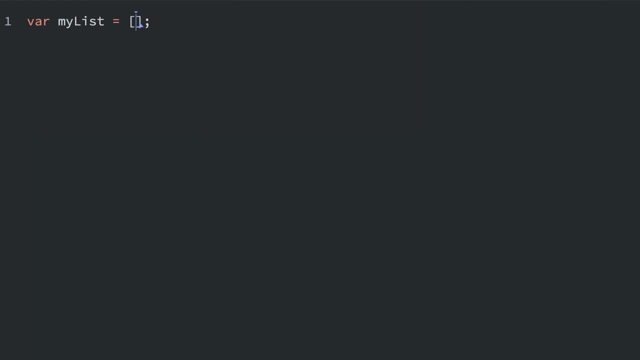 Now we're going to add something to the beginning of the array. We'll do Paul 35. So now the array is just going to be Paul 35.. Dog three: Let me give you another example of nested arrays. This will be a shopping. 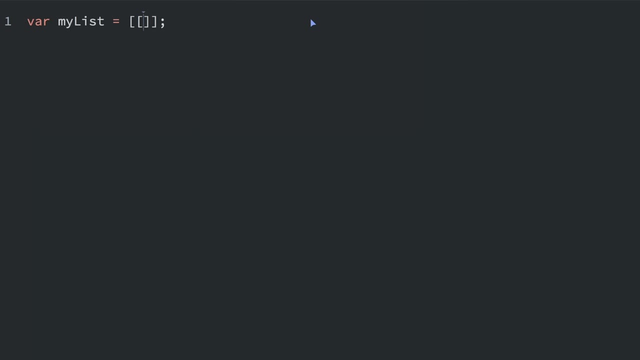 list. So inside this array, we're going to have another array And we're going to have items: cereal- how many boxes? three boxes. We also need some milk. Let's get two cartons of milk. Let's get some bananas: Three bunches of three bananas. We'll also get some juice. 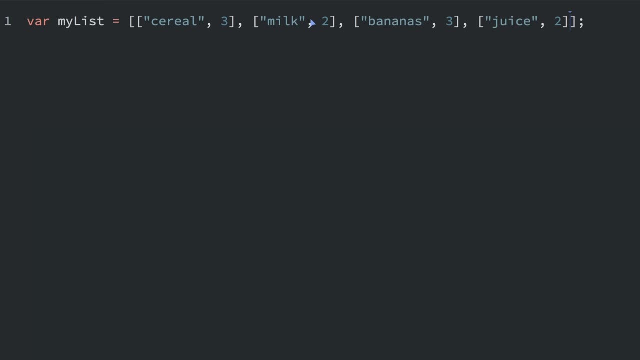 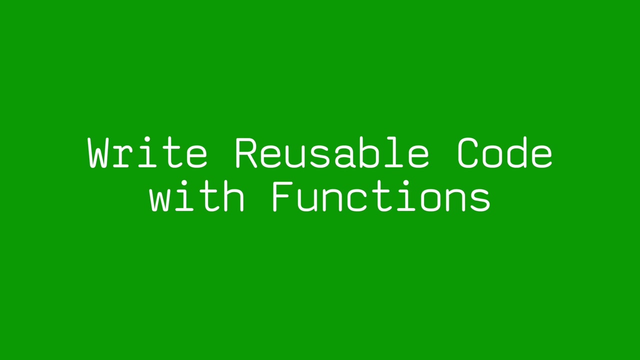 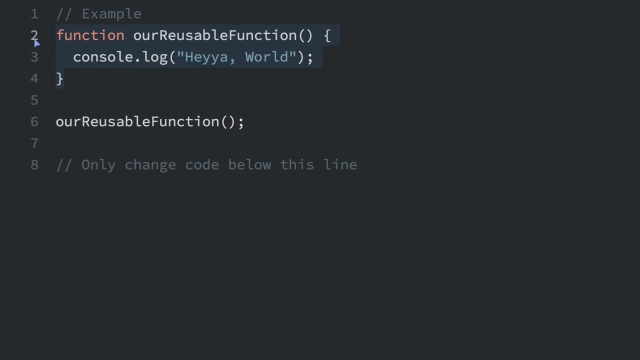 Two containers of juice And finally, we will get some eggs. We'll get 12 eggs And now we've created an array of arrays, which is our shopping list. Functions allow us to create reusable code. in JavaScript is how a function is set up. We have the word function, then we have the function name. There's 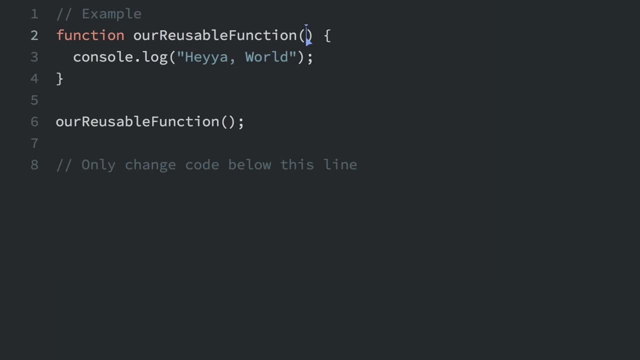 always parentheses here And you can pass information into the parentheses. We'll talk about that later. And then we have these curly brackets. So this is the opening curly bracket And then we have the closing curly bracket And everything inside the curly bracket is run anytime. 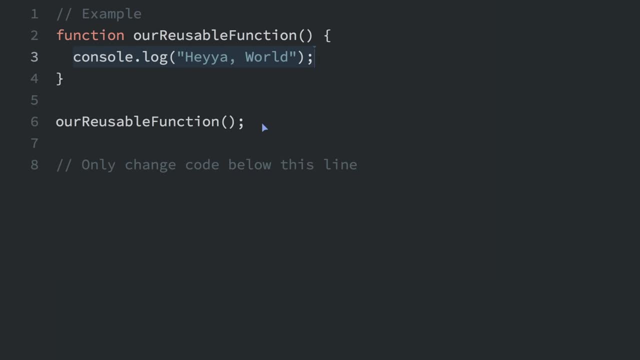 the function is called or invoked. So here the function is being called by just putting the function name with parentheses after the name. So every time this function is called, just like this, the console is going to say: Hey a world. So if we load the console right now, you can see it says: 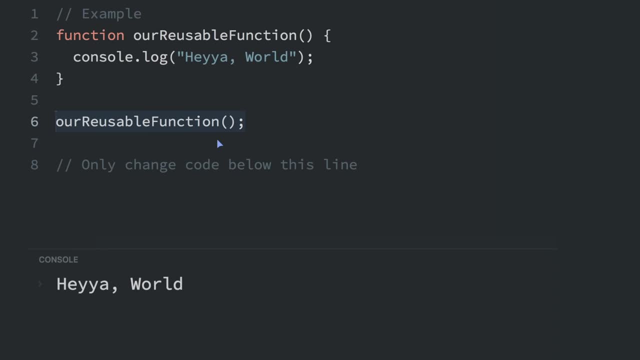 Hey a world. And if I just copy this and paste it a few times, we'll see that it's going to say Hey world, Hey world, Hey world. in the console, Since we have run the function three times, we see the words Hey a world three times. So now I'm going to create my own function. 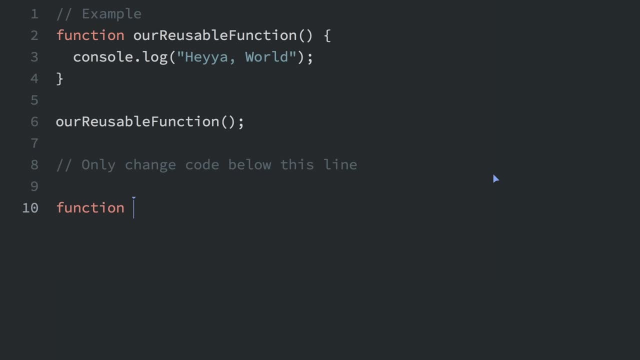 that's going to be very similar. So we'll do function the usable function, And this time it's going to say something slightly different. It's going to say Hi world, Hey a world, And now I can call the function down here, just like this reusable. 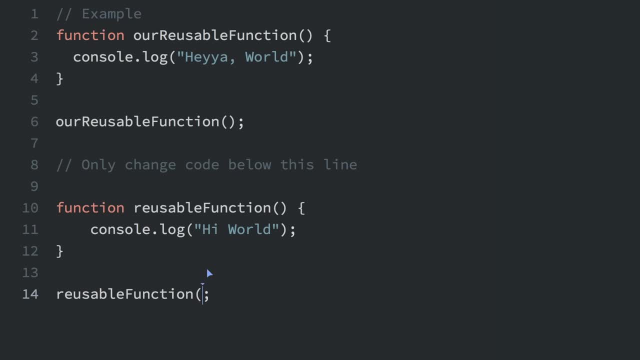 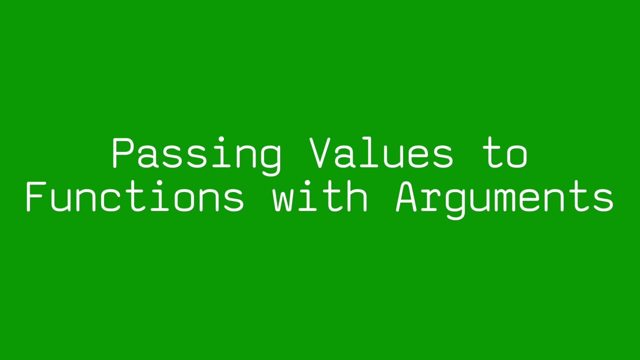 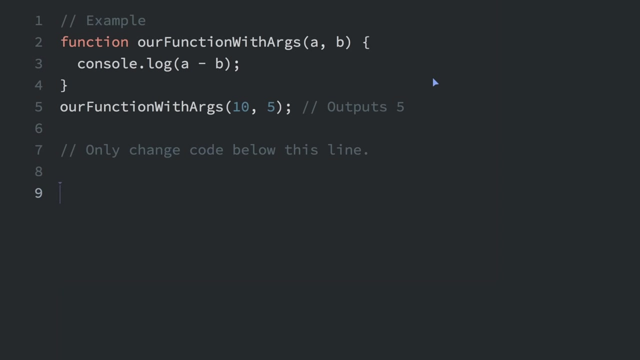 function. Oh, forgot to put the parentheses. That's important. Now you see Hey world and Hi world in the console. Parameters are variables that act as placeholders for the variables that act as placeholders for the variables that act as placeholders for the. 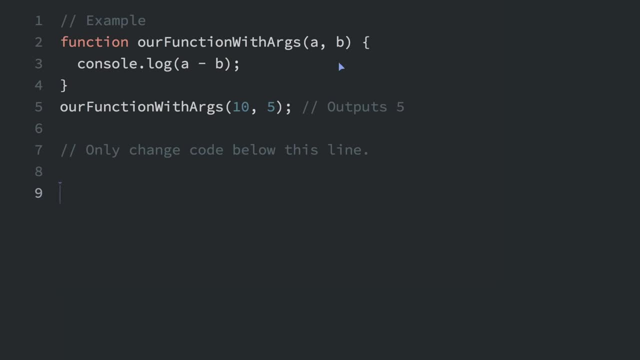 values that are to be input to a function when it is called. So we have defined a function right here, called our function with args, And inside the parentheses we see the letters A and B. Now these can be any name that we call these anything, not just A and B. they could really be any words. 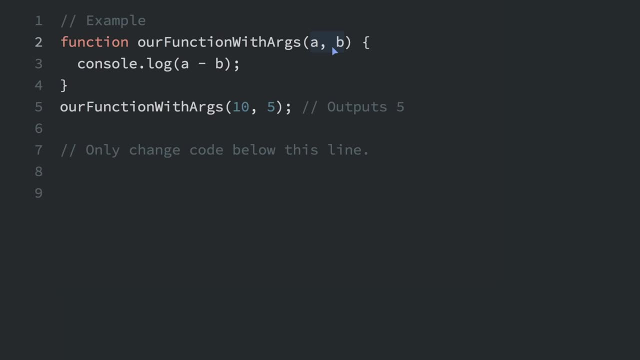 up here, And that means that when this function is called, we're going to pass data into the function. we're going to pass data into the function method or input data into the function. So you can see the example here where we're calling the function and instead of saying A and B in the parentheses- 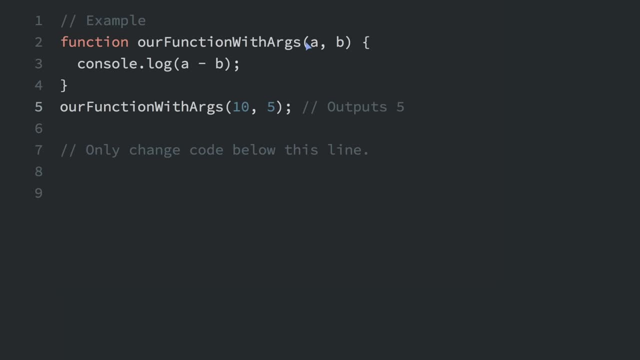 we're actually passing the values 10, and five, So when the function runs it can use the information that's passed into the function. So in this case it says console dot log a minus b. well, that's going to be 10 minus five because the numbers 10, and five have been passed into the function. So in 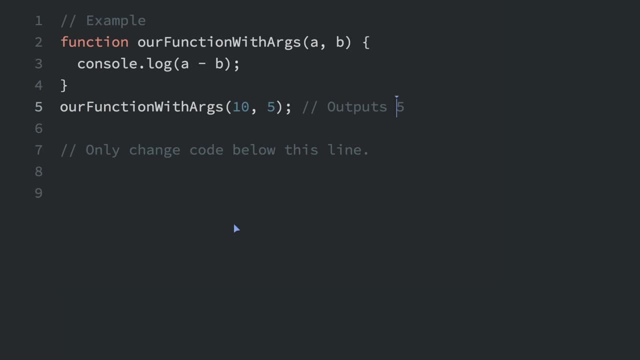 this case it says: console got log a minus B. Well, that's going to be 10 minus five because the to the function And that's going to output five. So I'm going to create a function that's very similar to that function. This one is going to be called function with args And it's also going to 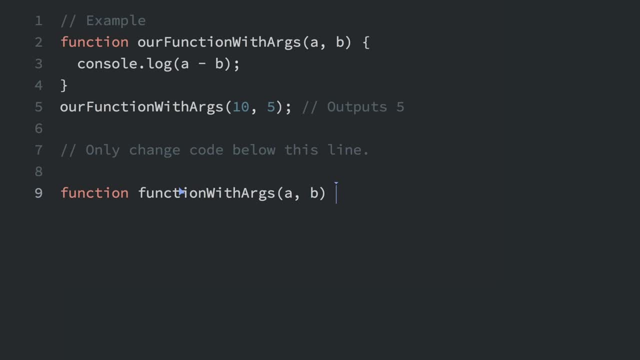 accept an A and B, But we could call that anything we want, And inside, instead of subtracting a minus B, we're going to do a plus B. Now I'm just going to call this function function with args and I'll pass in 10 and five, And let's see what that looks like in the console. So first, 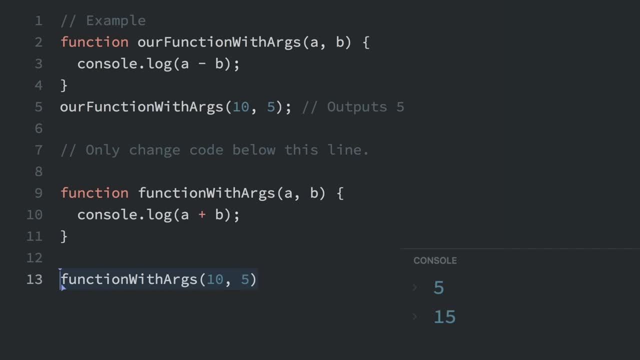 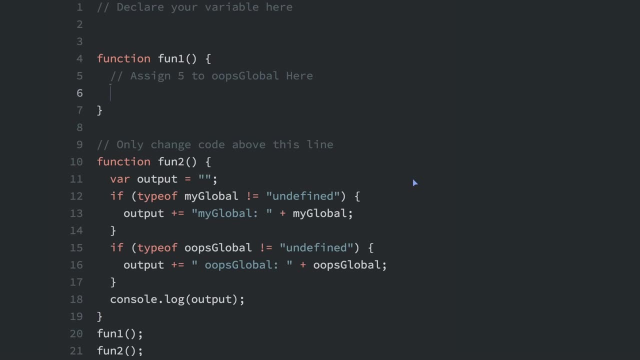 it output five for this one, then output a 10 for this one. And scope refers to the visibility of variables. variables which are defined outside of a function block have global scope. Global scope means they can be seen everywhere in your JavaScript code. For instance, I'm going to declare a variable right here called my global. 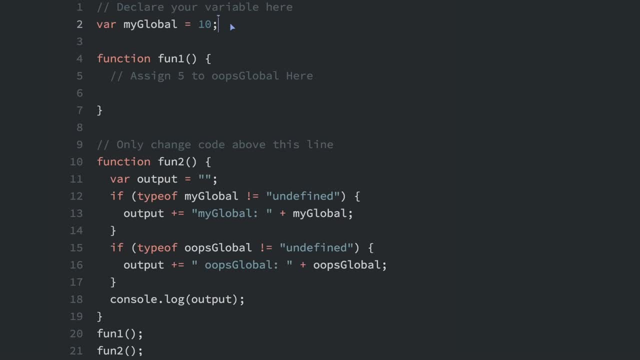 I'll set it to 10.. Now, since this is set outside of a function, we can see it anywhere in the whole code. And we can see it anywhere in the whole code Now, since this is set outside of a function. 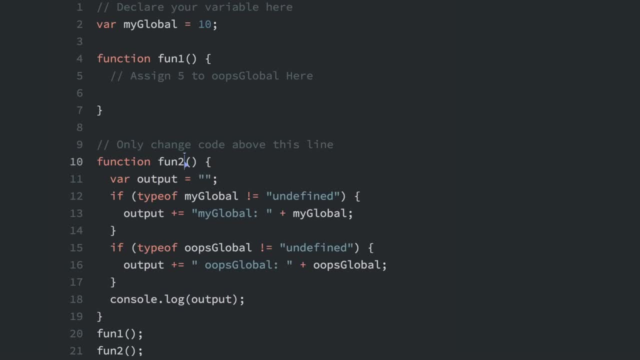 we can see it anywhere in the whole code. Now, since this is set outside of a function, we can see it anywhere in the whole code. Even in this function right here called fun, too. We can see that we reference it here and here And what we're going to be able to see it. Now, this is an if. 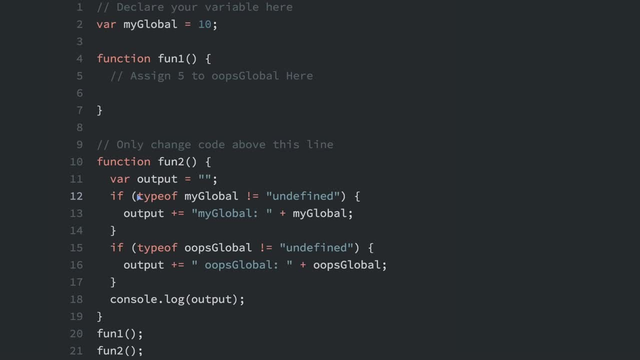 statement which we will talk more about later, But we're checking if the type of my global does not equal undefined, So it will not equal undefined If it has been defined and the program knows about the variable. since this is global scope, it does not equal undefined. 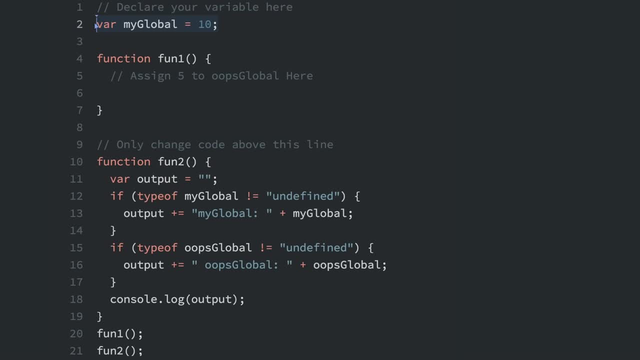 equals 10.. The program knows about the variable because this is in global scope. So since the this function can access the my global variable, we'll run what's in this if statement, where we just add to this output variable my global and then we put with the value of my global, which is 10.. And 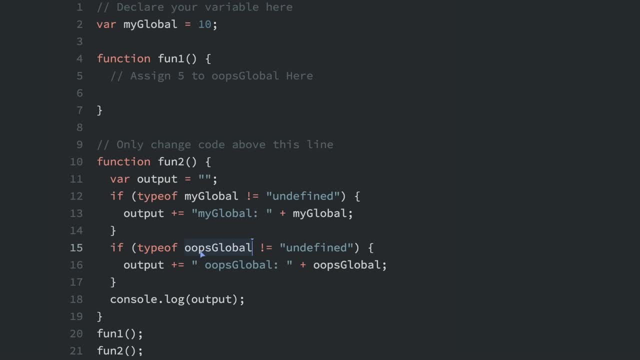 now here's another example where we're going to see if, if the type of oops global equals undefined, well, we're going to set that here, So it is possible to set a variable without using the var keyword. So I'm going to set this to oops global equals five, So you can see here that there. 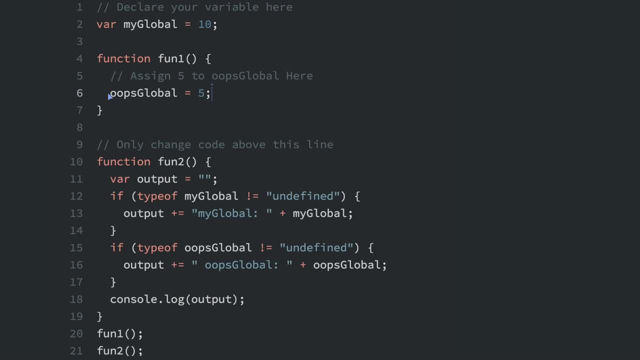 is no var keyword. So normally, if you do use a var keyword, since this is within a function, it will be scoped to that function. If we had the var keyword here, this would be scoped to this function, So you would not be. 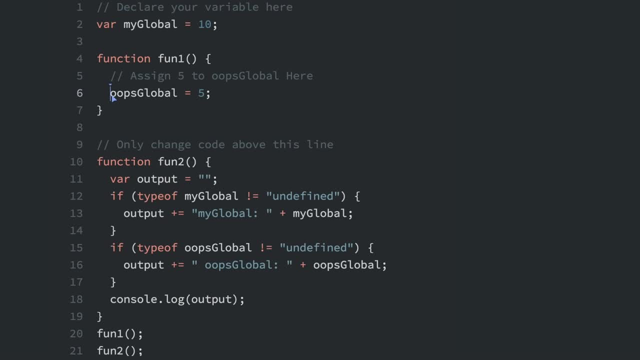 able to see it in this function. However, since we forgot to put the var keyword in this example- there's no var keyword- it becomes global automatically. that means you can access it anywhere else in the program, including here. So if 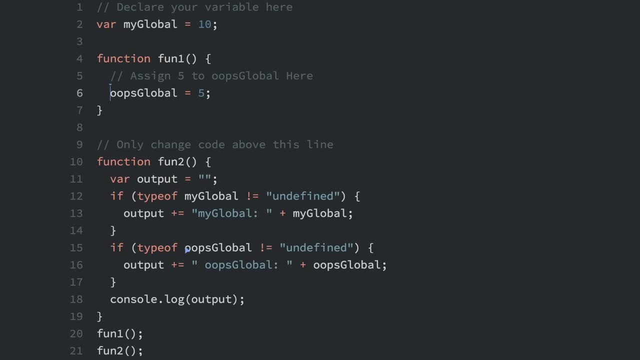 we put the var keyword, then oops global would equal undefined and then we would never have this line in the output. However, since we did not put the var keyword, oops global equals five and this will be added to the output. 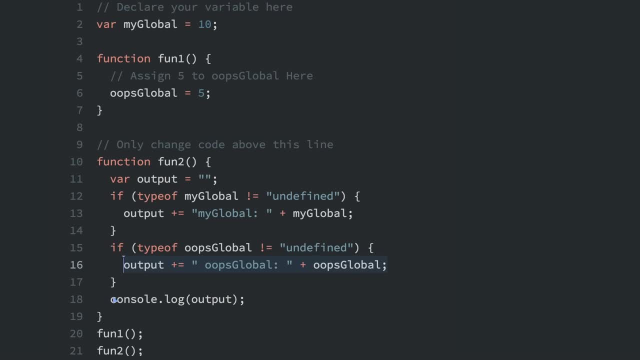 Oops, global. and then the colon five. So when we console dot log the output it's going to say: my global 10.. Oops, global five. Now, actually, it's not going to say that, because this is in scrimba, And in scrimba it's, it's. 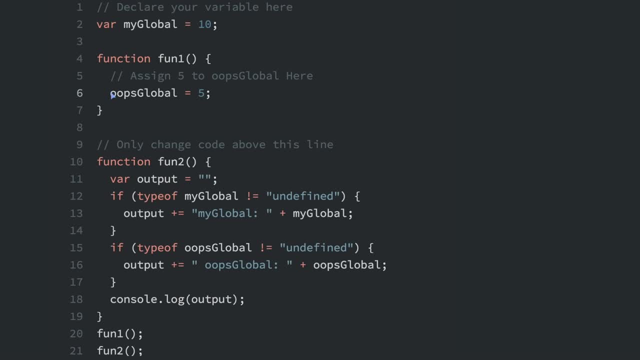 more careful and just enforces the fact that you have to use a var keyword. But if we were in our browser, it would not enforce the var keyword And then would actually show my global 10.. Oops, global five. If this was a little complicated, don't worry about that. 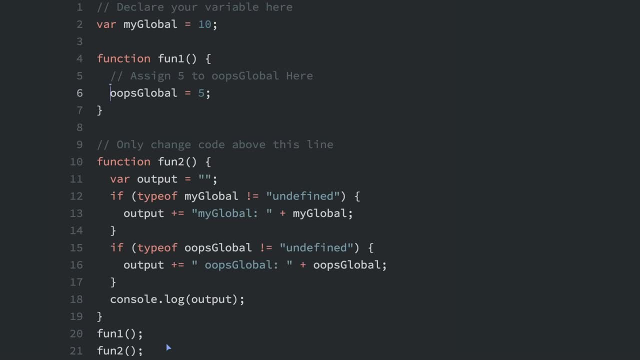 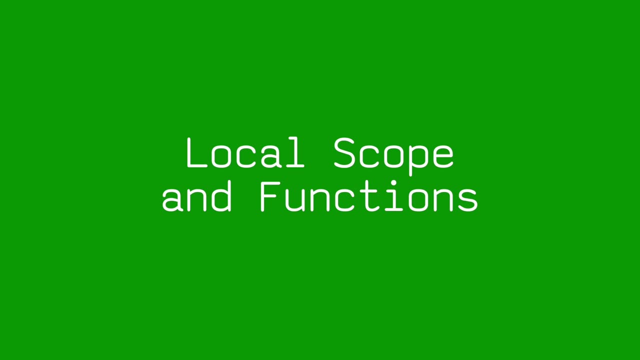 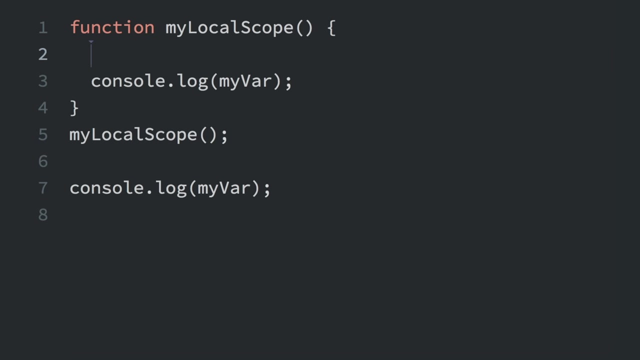 because a lot of these concepts will be going over again later with additional examples. variables which are declared within a function, as well as the function parameters, have local scope. That means they are only visible from within the function. Let me show you what I mean. If I declare a variable right here, my var equals five. So we've 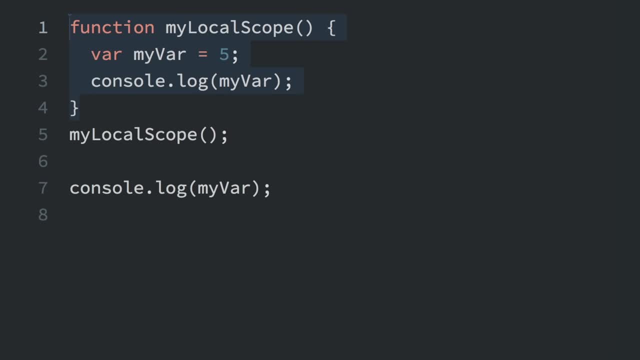 declared this variable inside a function. So this variable, my var, is only visible inside the function. So it says console dot log my var. it should console dot log the five. So we're going to call the function here and it's going to console dot log my var, But then the. 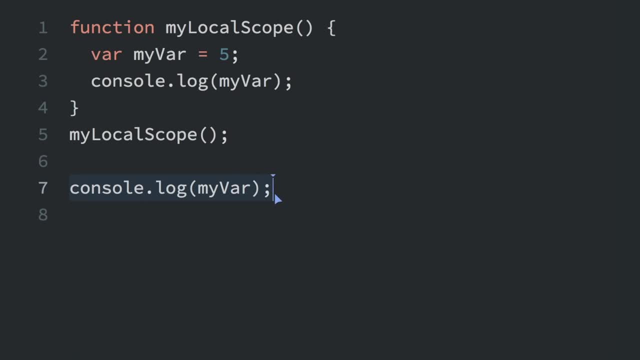 program is going to run this console dot log. that's outside of the function. it's still going to try to access my var And so let's see what happens. You can see in the console that first there's a five because it console dot log within the function. then 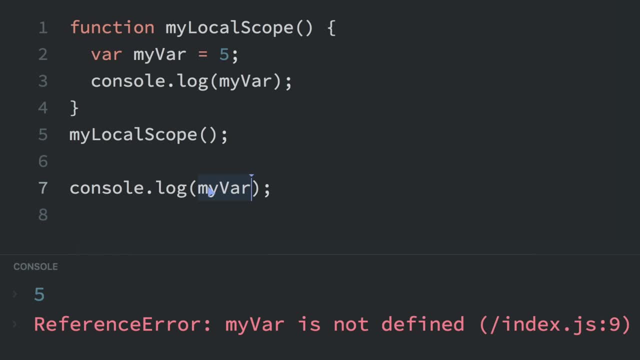 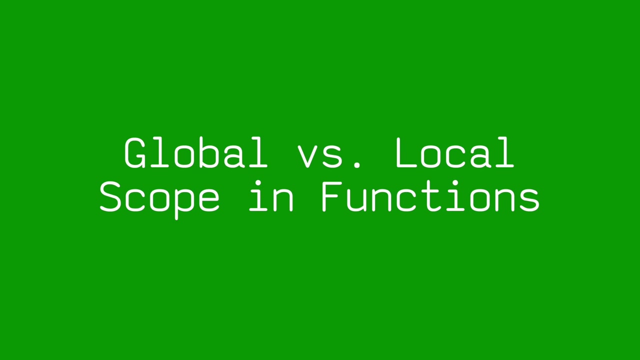 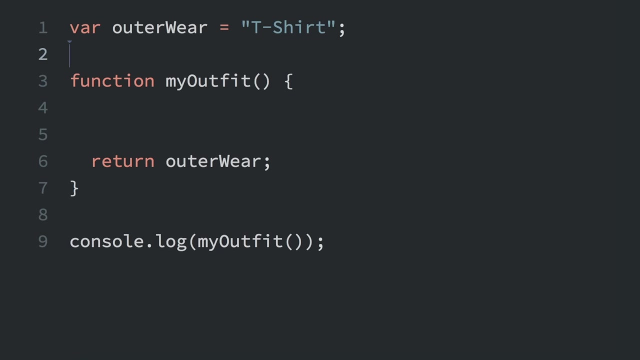 there's an error because it tried to access my var outside of the function. So really we just need to delete this, where we try to access the variable outside the function, And now there is no error. It is possible to have both local and global variables with the same name. When you do this, the local variable takes precedent over the. 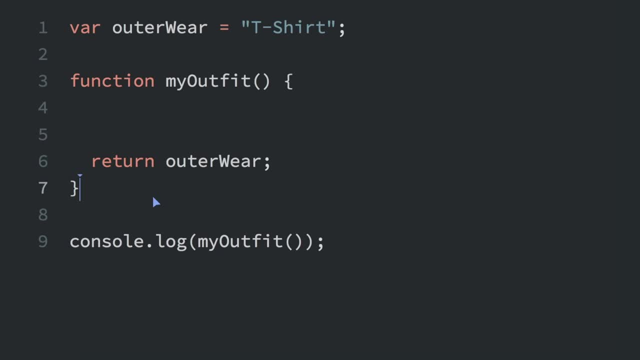 global variable. Let me show you an example Here we have a function called my outfit that's going to return outerwear. That's this variable up here. This is a global variable because it is declared outside of the function. So when we console, dot, log the output of the my outfit function or the 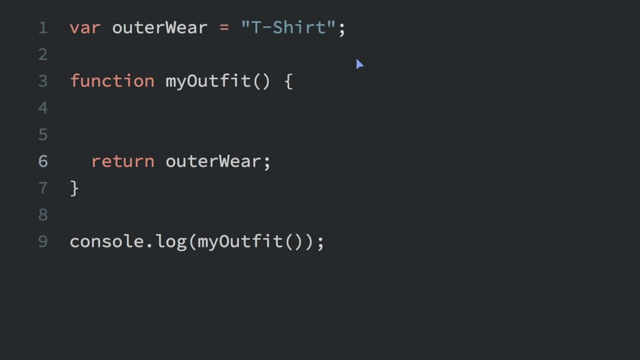 my outfit function is going to return outerwear, which is the word t shirt. So let's check the console And you can see: Yep, t shirt is there. However, let's change this up a bit So we have some space here, because I'm going to put var outer. 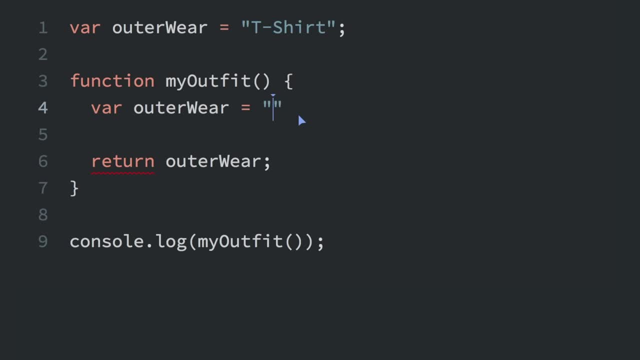 where equals sweater. So now if I run this program you can see in the console it's going to say sweater instead of t shirt. It's because this local variable, outerwear, took precedence over the global variable. Another interesting thing about this: if I do a console, 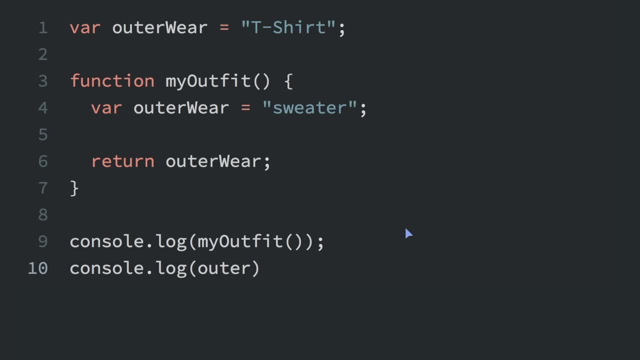 Outerwear, Outerwear log. and I console dot log that outer wear variable, we'll see that it's still t shirt. So first you see in the console says sweater and t shirt. So first we console dot log this function which is sweater, it returns sweater. And then we console dot log the global variable which is t. 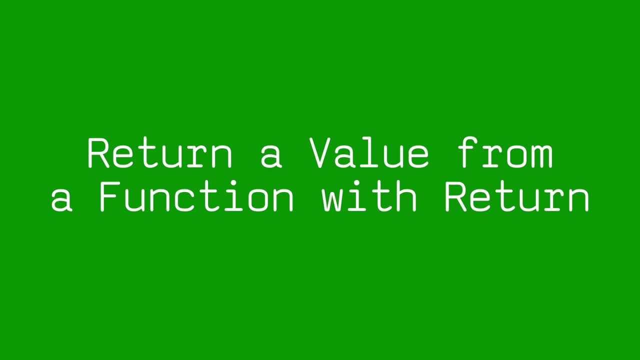 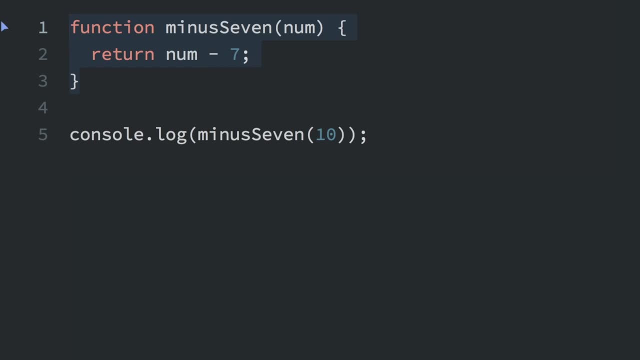 shirt, And you can return a value from a function with this return statement. So we have this function here and we are passing a number into it, the num, and then it's going to return whatever's after the return keyword, in this case num minus seven. So here we're going to console, dot, log the function. 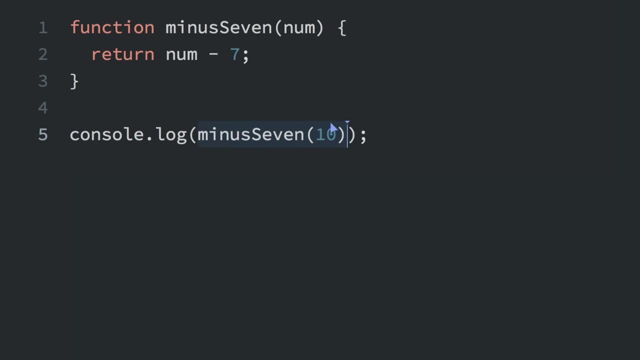 and the returns, the result of minus seven is this: 10 minus seven, which is three. So it's going to console dot log the number three. So if we look in the console, yep, it console dot log the number three because the function returns. 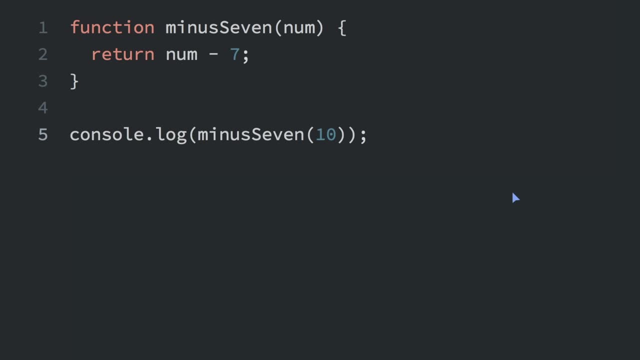 three. let's try creating another one. this function is going to be called times five. again, we'll pass in a number And it's just going to return something. it's going to return the num times five And then, just like before, we can test it. 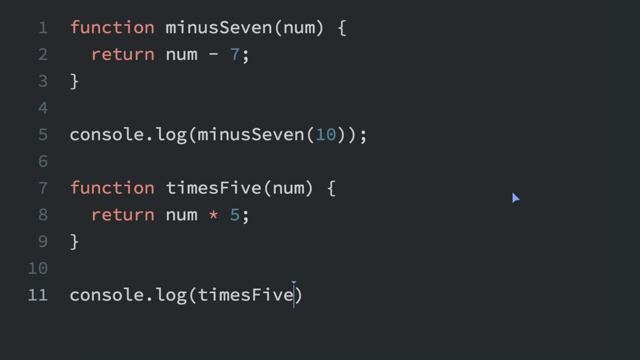 using a console dot log times five and we'll pass in the number five here And if I run this, we'll see that it returns number 25.. Functions can have return statements, but they don't have to In this case. this function adds three to the sum variable, which is a global variable, because 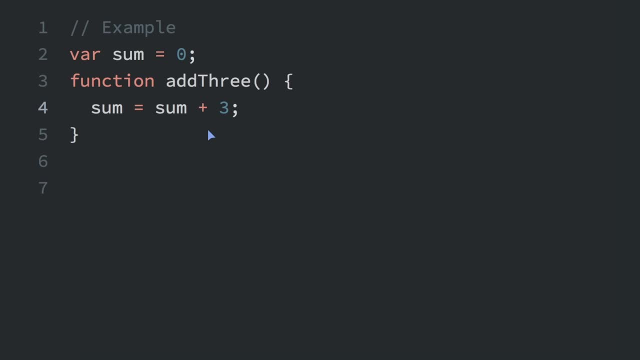 it's defined before the function, And then we're going to return the number five, And then we're going to return this one and we're going to coordinate for examplegs, and then we'll dumb this part of this function And then, as it gratitude maker doesn't do, it does not return anything. So if you 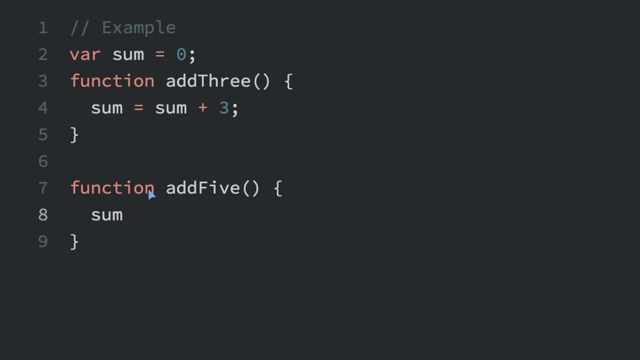 don't specify a return value. the return value is just undefined. Now I'm going to create another function that is similar. This one is going to be called add five, And this time we'll just do some equals sums. So now that's going to add five to some also, but it's not going to return anything. 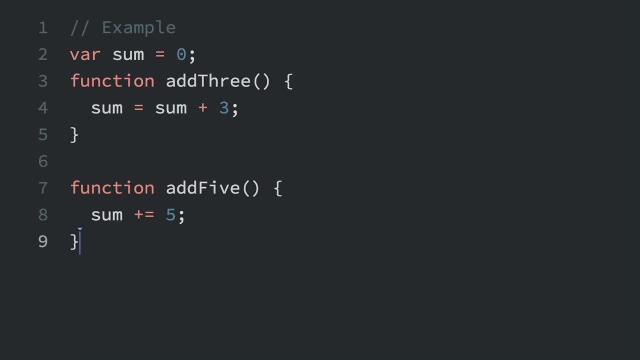 So if we log this out, it would be undefined. It's simple to assign a returned value to a variable. See right here we have the function change and you pass the number and it's going to return the result of this mathematical expression. 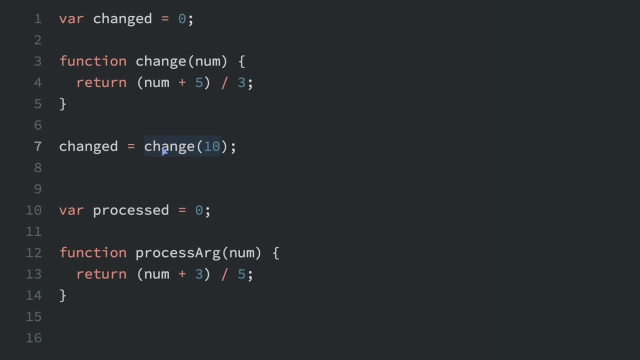 So when we call the function change and pass in the 10, the value that is returned from this function is going to be stored in this variable. here We can do the same thing down here. First we initialize the variable processed and process arg. it's going to return the. 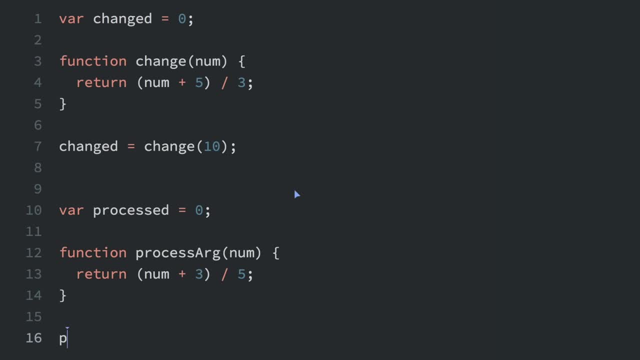 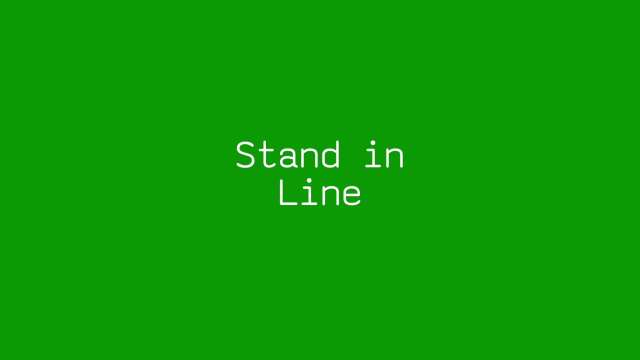 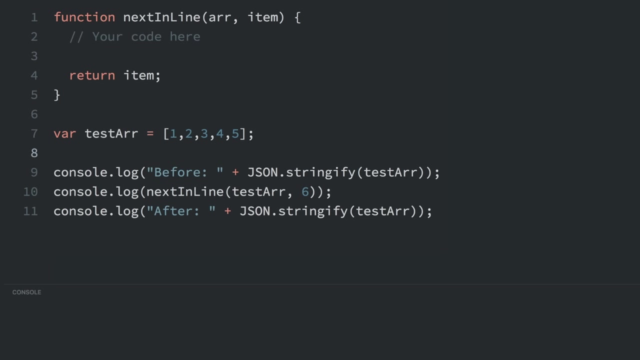 result of this mathematical expression. So I can set processed to equal what this function returns. So I can say processed arg, and I'll just pass in the number seven here And now, processed equals the result of this mathematical expression. In computer science, a queue is an abstract data structure where items are kept in order. 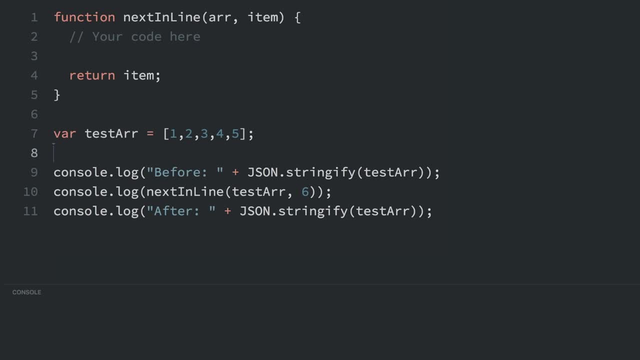 New items can be added to the back of the queue and old items are taken off from the front of the queue. We're going to simulate that right now. Now some of the functionality of a queue using this next in line function. So the purpose of this is to show that in this next in line function, you can add an. 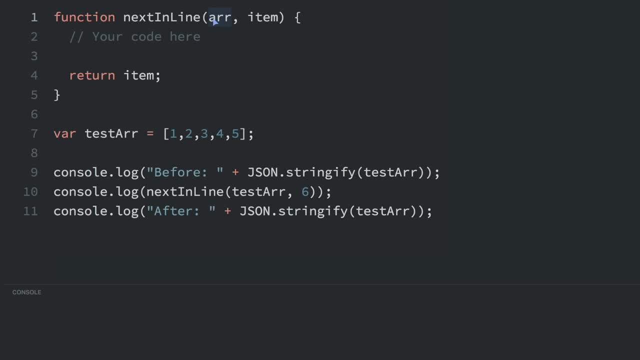 item to the array that's passed in and then it's going to return the first item on the list. For instance, if we have this array right here, if we add an item to this array, it should come after at the end. 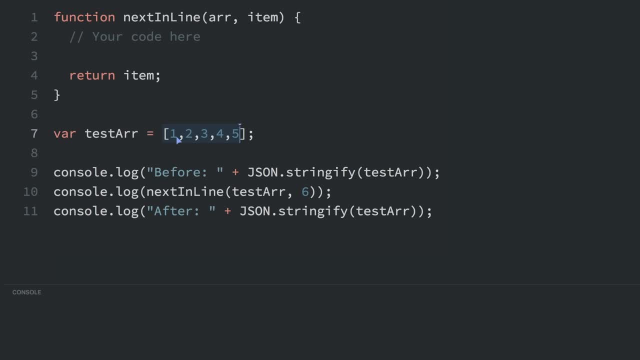 So it should come after five and then it should return the first item on the list. In this case it's one. So you see, we have some console, that log setup, So it should show what the list looks like, the array looks like, beforehand and then. 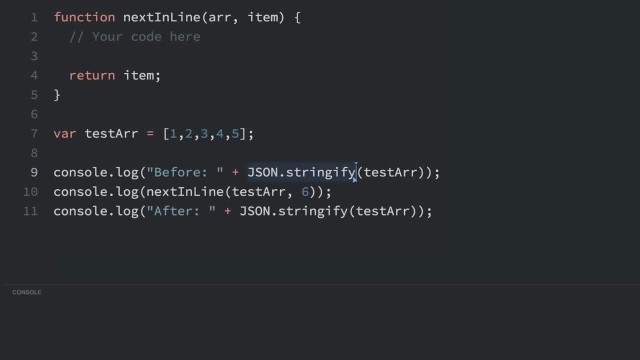 show it looks like afterwards. This JSON that stringify is just a way to change an array into a string that can easily be printed out to the screen. So to do this, we're just going to have to do two things that we've learned about already. 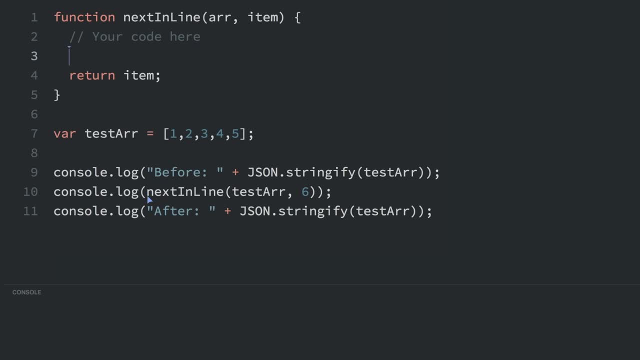 So the first thing is to add the item onto the list. So we see right here, next in line, passed in the test array, and six. So we're calling this function, next in line, we're passing in this test, in this test array here. 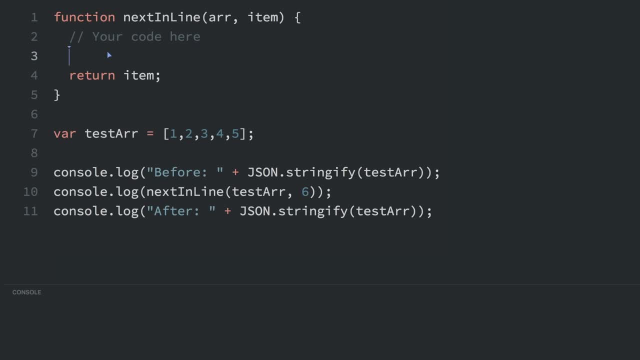 And the number six. we want the number six to be added to the end of the array, So we'll just do our push, Okay, And then I'll put in num, Just like that. Well, actually it's item. So what we did? we took this array that was passed in here, which is, in this case, test. 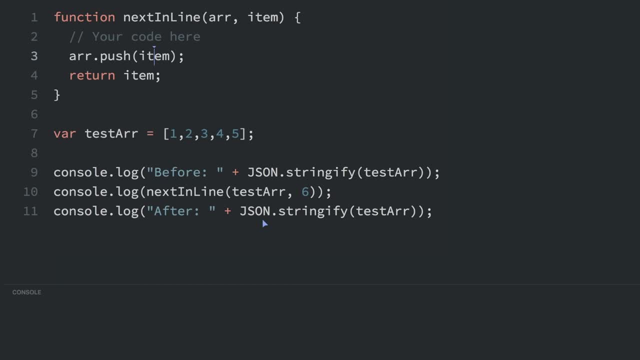 array and we push the item that was passed in, And in this case here is the item six. Now we want to return the first item on the list. we want to remove and return This item so that when we console that log here it should show the number one. 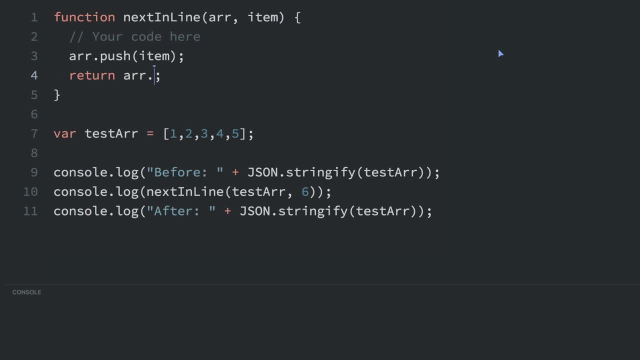 So instead of returning item, I'm going to return our dot shift. That's what shift does. shift removes the first item and returns that first item. So let's check this out. Okay, you can see before 12345.. Then we've popped off the one and after. 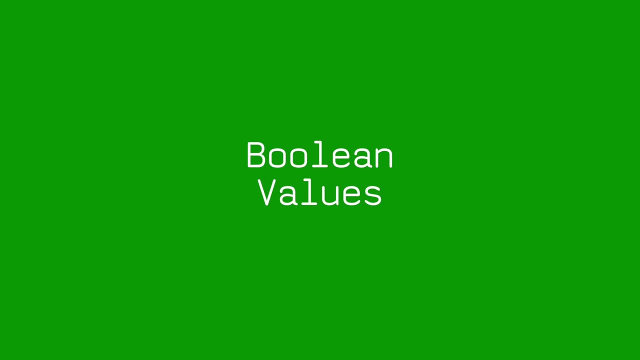 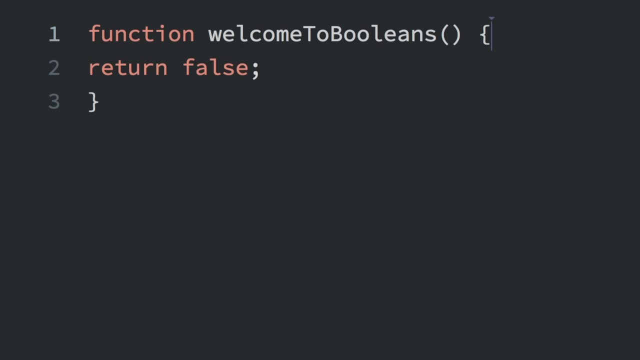 It's 23456.. We did it. Booleans are another data type in JavaScript. There are only two values: true or false. They're basically little on off switches where true is on and false is off. They don't use quotation marks around the Boolean. 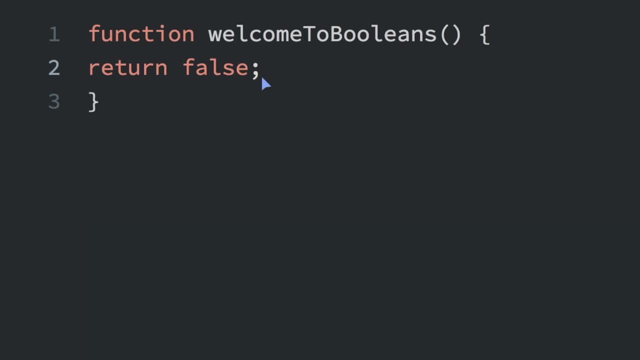 See, it just says return false. So this is a function here should be indented. There is just going to return false. when you call this function, It could also be true, So we could return true. You can use true and false in more places than just function returns. 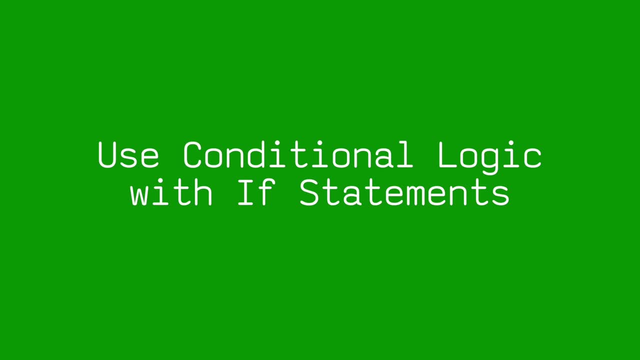 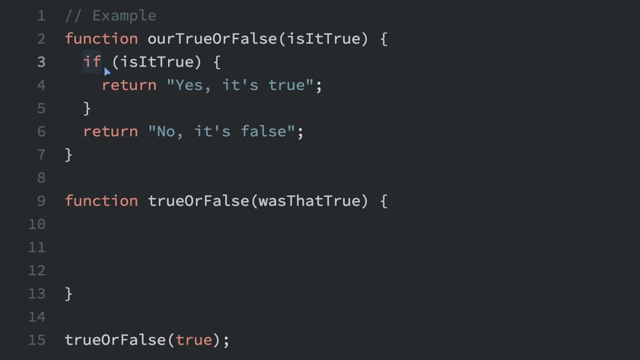 And we'll be talking more about that later- And if statement is used to make decisions in code, the keyword if tells JavaScript to execute the code in the curly braces And you can see here in the first line that these are the conditions defined in the parentheses. 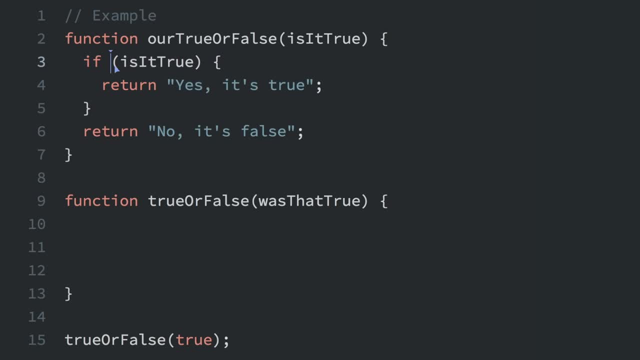 So here is a full if statement right here, And there's always parentheses after the keyword if, And here's the condition. So if the stuff inside this print, inside these parentheses, evaluates to true, then the code within these curly braces will be evaluated or run. 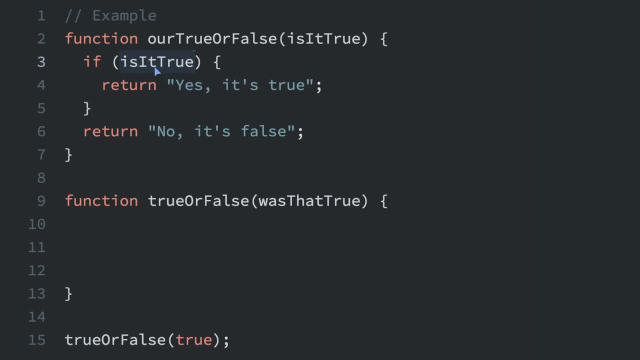 So in this case it's a variable. So if the is it true, variable is true, variable is true, it will return: Yes, it's true. Now, if it is not true, then we'll get to the second return statement: No, it's false. So this whole function here takes in a variable and we check. 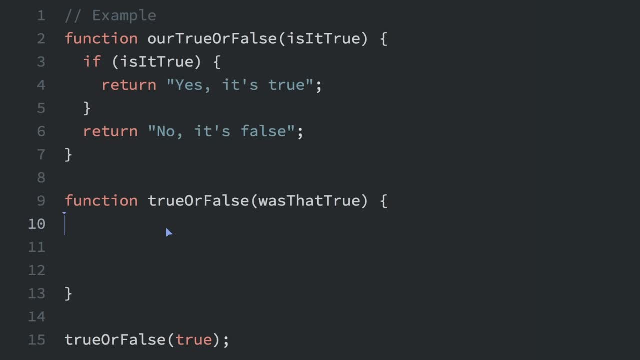 if that's true or not. So I'm going to make another example, just like this. we have another function that hasn't been filled out yet- true or false- And there's a variable that's passed in. was that true? So we'll say if, and then the parentheses: was that true? If that's true. 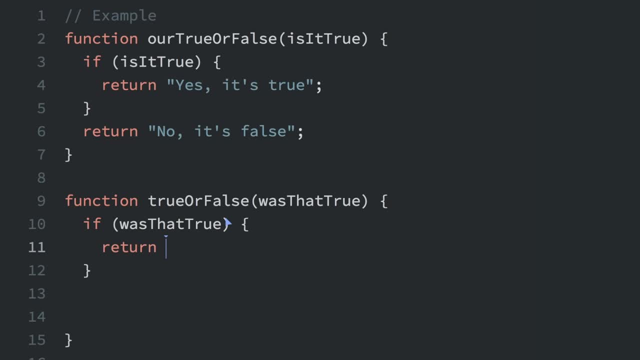 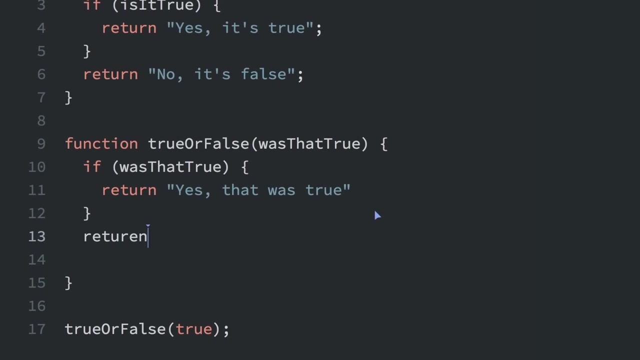 we're going to return something. it will be a string, just like before, And the string is: yes, that was true. If it's not true, then we'll get to the second return statement in the function And we'll return a different string. we'll return. 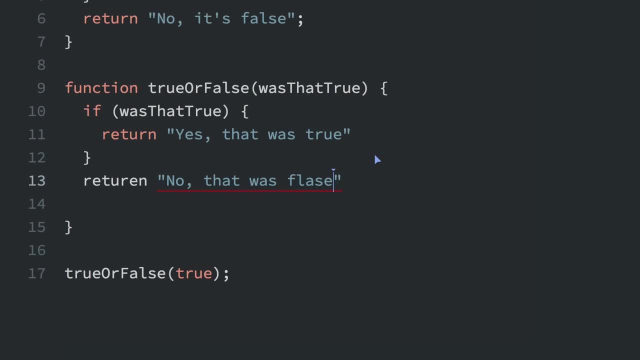 no, No, that was false False. Let me just add some semicolons And then I can run this And we'll see what happens. Oh, return needs to be spelled correctly, So let me spell return correctly. So, before I run this, I'm. 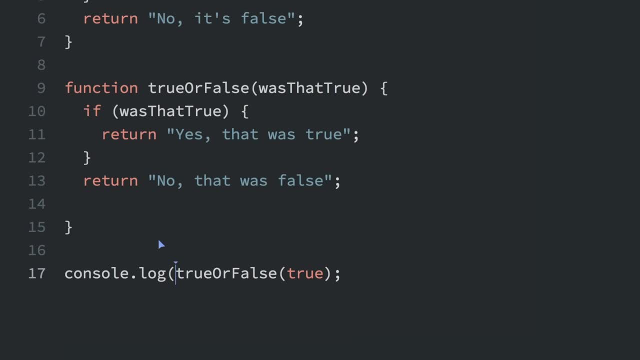 going to edit console dot log here So we can console dot log the the answer. So this is the the function call here, true or false. we're passing in true And then we're going to log what is returned here. Yes, that was true, Since we passed in true. This if statement evaluates to: 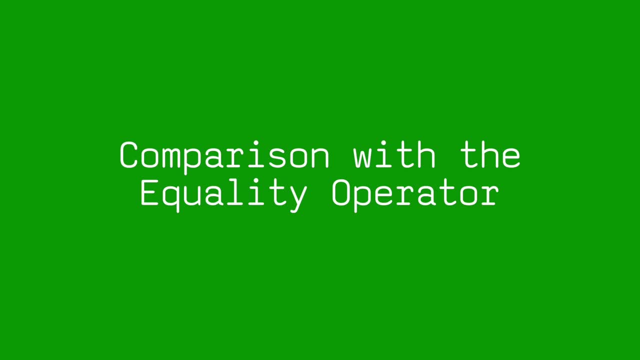 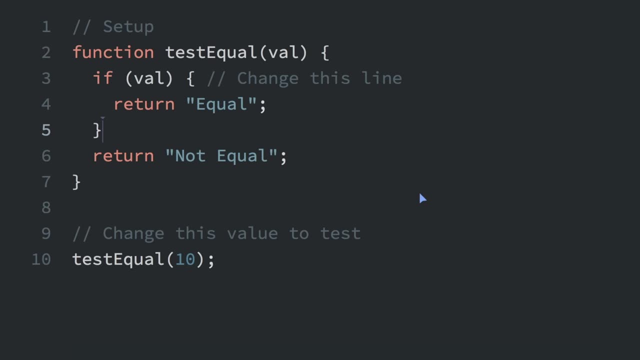 true and this code is run right here. There are many comparison operators in JavaScript that will return a Boolean of true or false. The most common is the equality operating in the job. But since we passed in true, this is true in true. 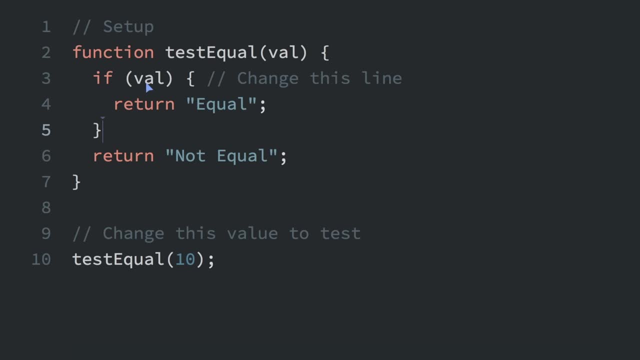 operator And it's often used in an if statement. So here it just says if Val. so we have this whole if statement right here. if Val, we're going to see if if Val equals 12.. Now to check if it. 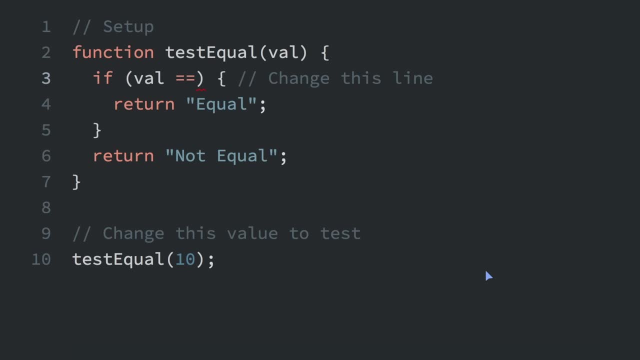 equals 12, we're going to have to use the double equal sign. that is the equality operator, And we'll say if Val equals 12.. The reason why we can't just use a single equal sign is that a single equal sign is the assignment operator. if we just had a single equal sign, that would mean 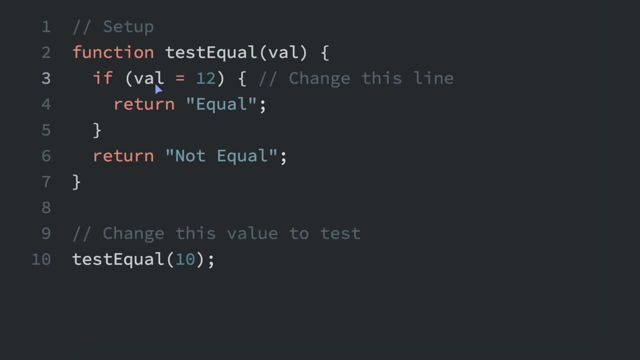 that we were setting the value, the value of the Val variable, to equal 12.. We're not trying to set this to equal 12.. We're trying to check if the value of this variable equals 12. So we have to use the double equal sign. So now this test equal function is going to test to see if the number we 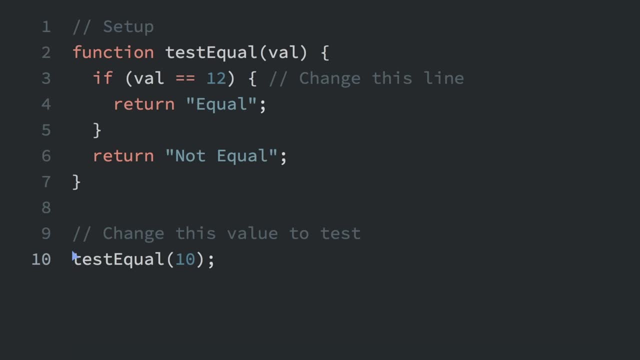 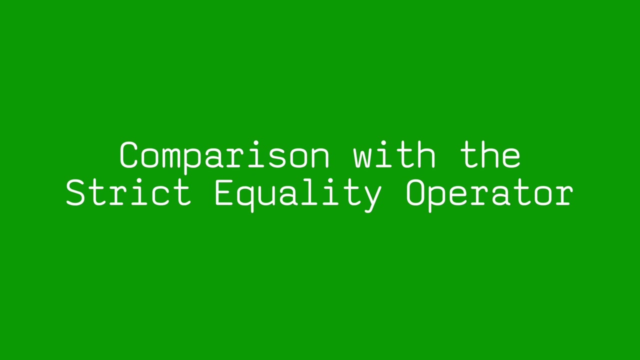 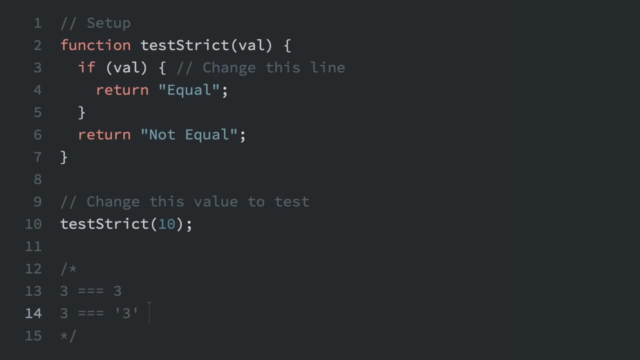 pass in is equal to 12.. I can do a console dot log here, console dot log, And then we can see what appears in the console here. not equal, because 10 does not equal 12.. We learned about the equality operator, which is the double equal sign. There's also the strict equality. 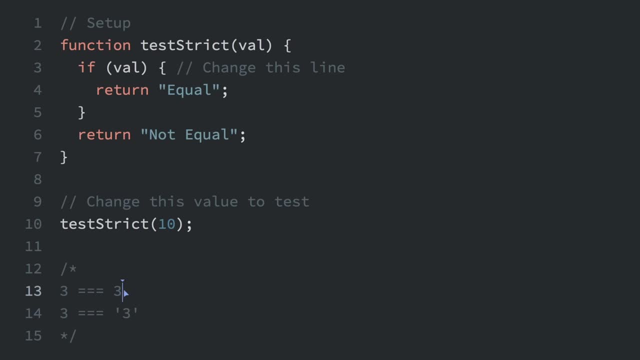 operator, the triple equal sign. So here we're checking if three equals three with the strict equality operator. So the difference is that the equality operator, the double equal sign, attempts to convert both values being compared to a common type, while the strict equality operator 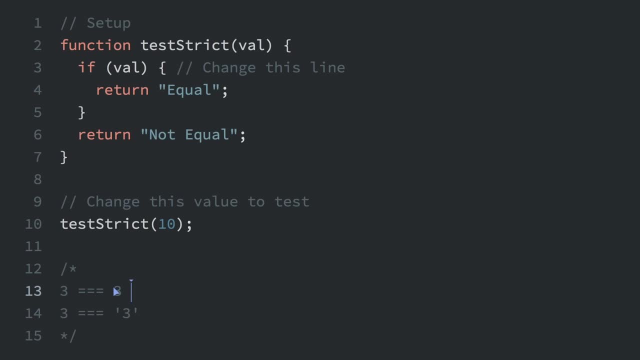 does not do the type conversion. So this is going to evaluate the truth of three equals equals equals three. But the three equals equals equals three with the double equal sign. So the string on this side is going to evaluate to false. Both of these would be true if we were. 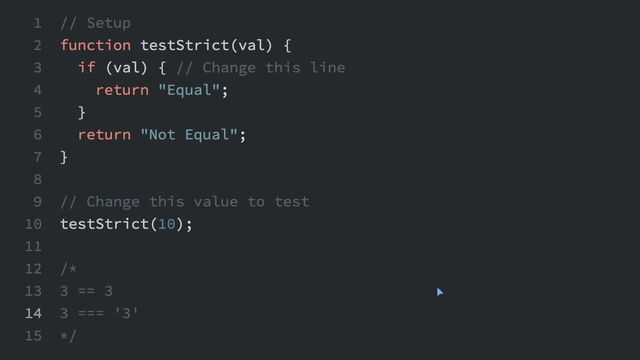 using the double equal sign, because the string would be converted to a number and they would be equal to true. But with the triple equal sign it does not get converted to a number, So it would be evaluated to false. the second one with the three equal signs. So here we're just going to. 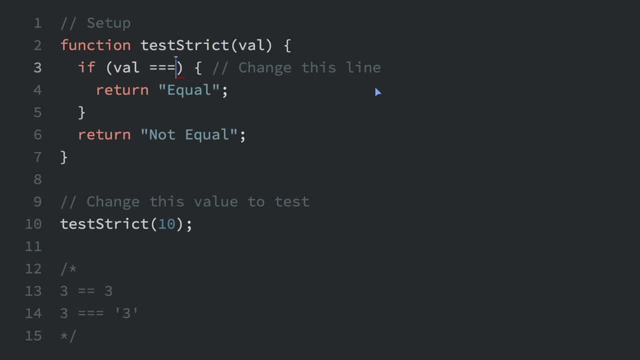 use it right in this. if statement and do equals equals, equals equals seven. So now we can pass in the number seven and it's gonna evaluate the true. but if we pass in a string seven, it will evaluate to false. We will do one more review with the. 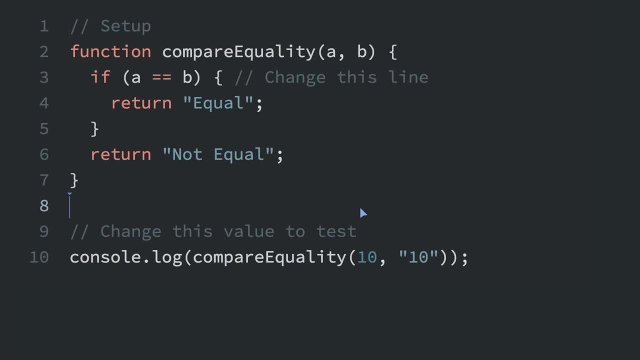 equality operator and the strict equality operator. So if I run this year we'll see in the console says equal, because is checking if the number 10 and the string 10 are equal. So if A equals B, the number 10 equals a. 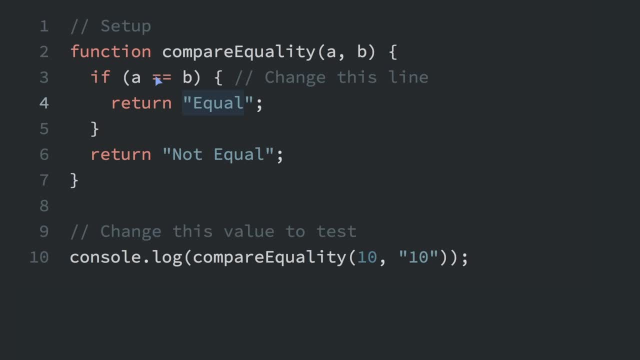 strict number 10 return equal. Since we're using the equality operator with with two equal signs, it performs a type conversion and it converts the string into a number. But if we use the strict equality operator with three equal signs, I'll run that again And you'll see: not equal in the 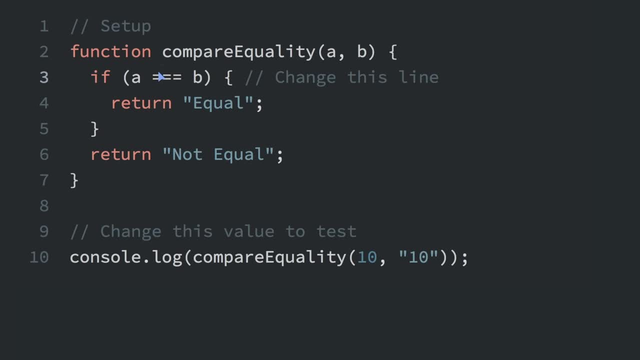 console, because now it's not converting the types And it's just checking if a number is equal to a string, which is not, so we get not equal. Now I will show you the inequality operator, which is basically the opposite of the equality operator. So I'm going to do the 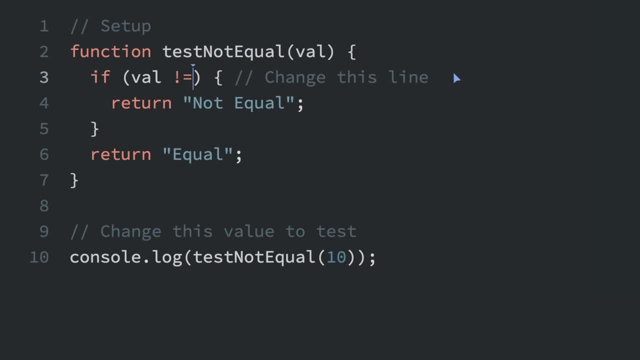 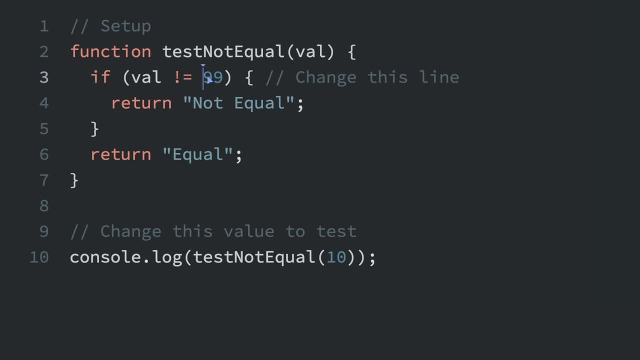 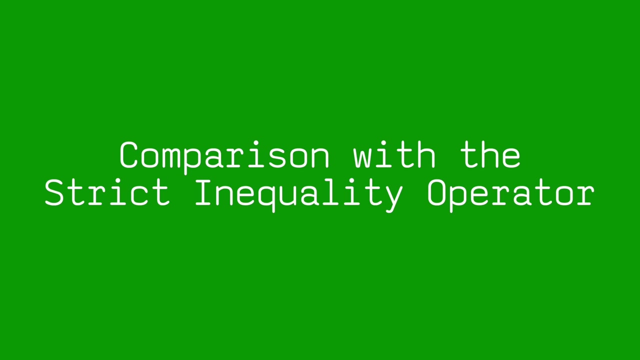 if the value is not equal to 99. And again, just like the equality operator, this does type conversion. So let's just run this program And we'll see it is not equal, because 10- we pass in 10 into the function here in 10, is not equal to 99. So we get not equal. The strict inequality. 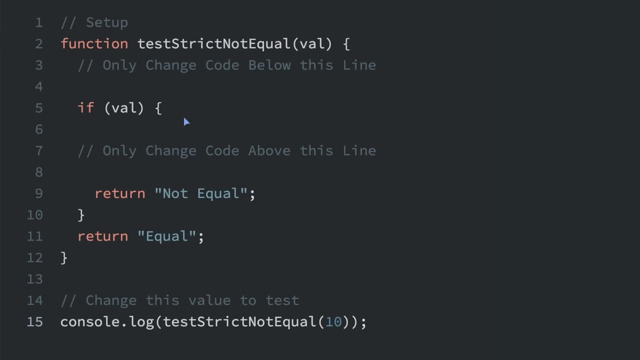 operator is basically the opposite of the equality operator. So we're going to run this program. and opposite of the strict equality operator And it works like this. So it says: if Val, I'm going to do if Val does not equal 17.. So this is the strict inequality operator instead of one equal sign. 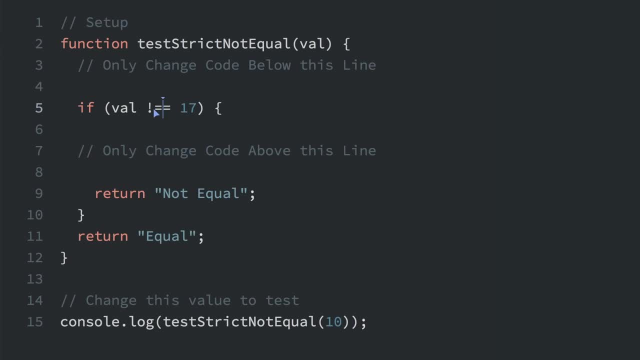 we have two equal signs And that means it's going to check if this is not true, but it's not going to convert types. So, for instance, if we are checking if the number three does not equal the string three, that would be true, And if we're checking if the number three does not equal the 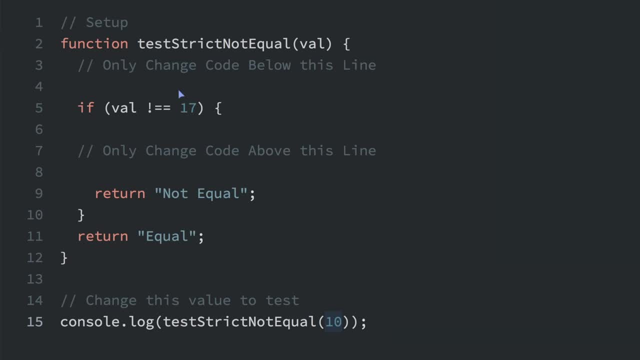 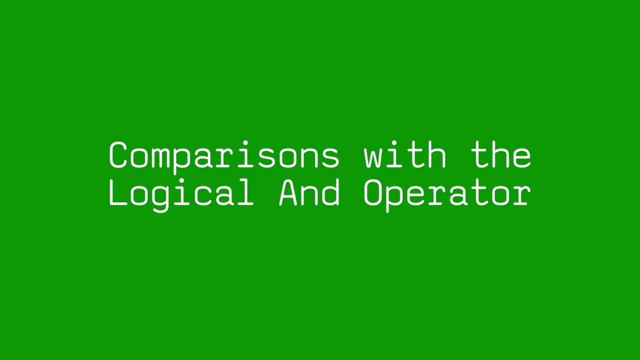 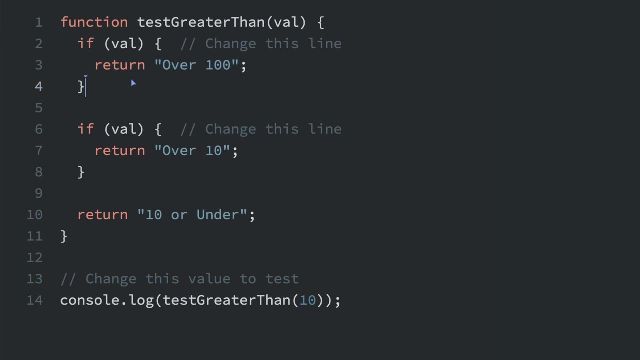 string three, that would be true. So in this example we're just checking if 10 does not equal 17.. If we run this we will see it's not equal. We can also use the greater than operator. So in this function we're checking if a value is over 100.. So I'm going to put greater than 100. And 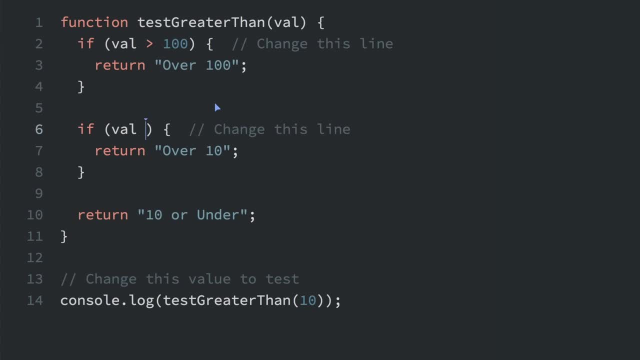 then here we're checking if a value is over 10.. So I'll put greater than 10.. So here we call the function: we pass in 10.. And if I run that function you'll see 10 or under, because we're not over 100, we're not over 10, or 10 or under because we passed in 10.. 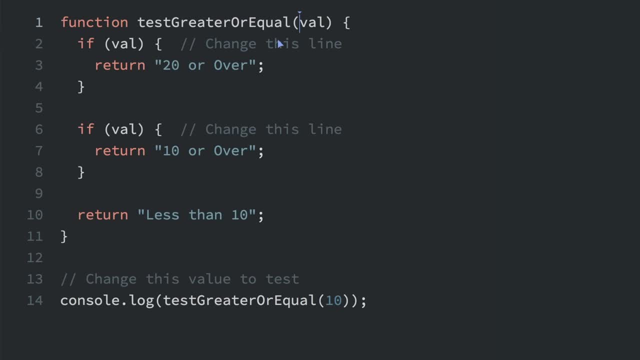 We can also use the greater than or equal to operator. So we'll finish this function by using greater than or equal to. that's just a greater than sign and an equal sign, And we'll put 20 down here, And then we'll put 10.. And then we'll put 10.. And then we'll put 10. And then we'll put. 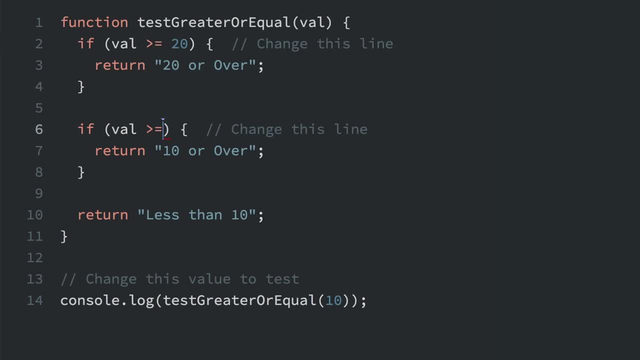 here just greater than or equal to 10.. If I run that we should see 10 or over, because we're passing in 10 and it's greater than or equal to 10.. Now I'll show you an example of the less than operator. 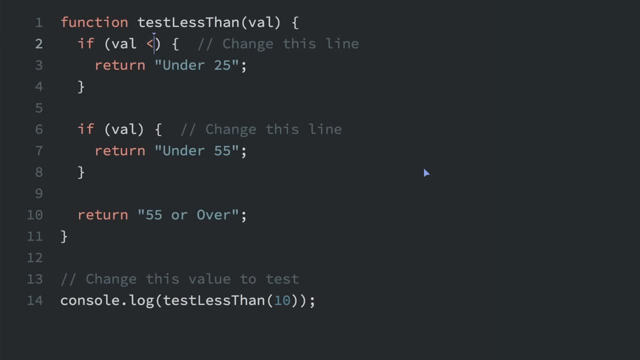 with this function we're going to check if the value is less than 25.. And then here we're checking if a value is less than 25.. less than 55.. So here's a trick I use to remember which symbol is less than when which symbol is. 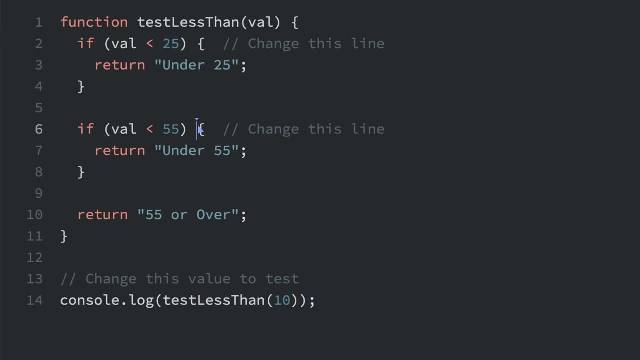 more than. if you see, the less than symbol looks kind of like the letter L, which is the first letter, and less than, and then the more than symbol is just the opposite. And we also have the less than or equal to operator we can use in JavaScript. So here we're going to check if it's less than or. 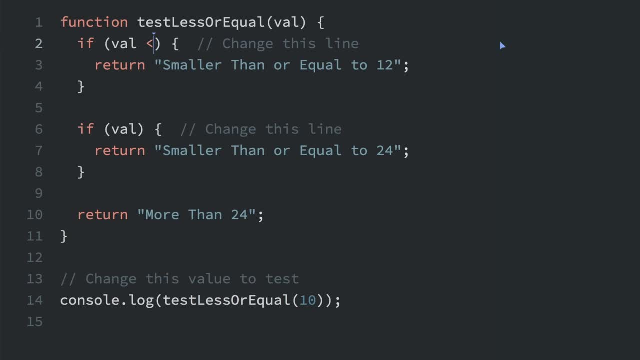 equal to 12.. So we just put the less than operator 12.. Oh, equal, less than or equal. That's an important part Here. it's the less than or equal to 24 to make this statement true. And if we run, 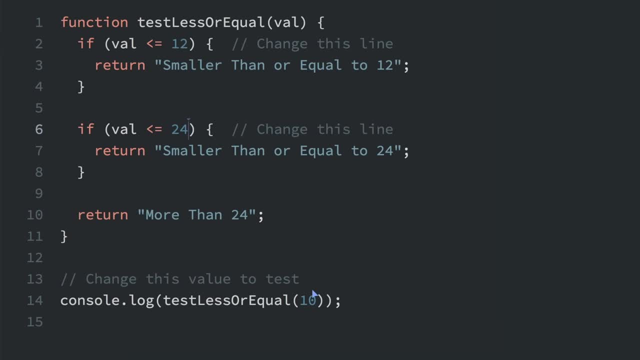 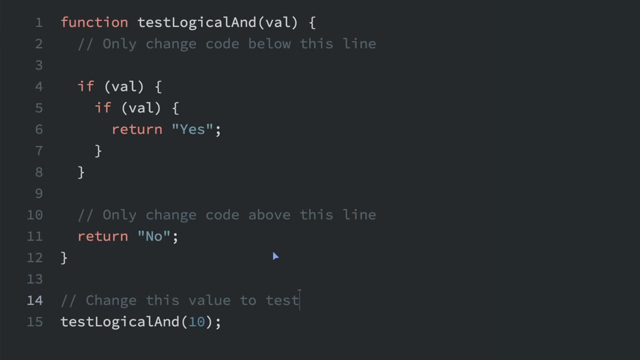 we see, smaller than or equal to 12.. Number 10, we passed in. Sometimes you want to check if two things are true at the same time. So, for instance, you may want to check if this value is less than or equal to 50. And you also 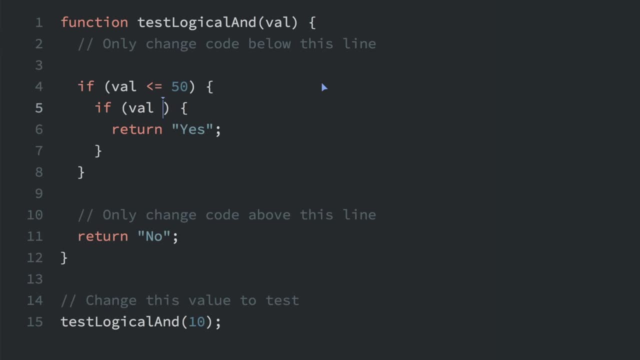 want to check if the value is more than or equal to 25.. So we have here, we have a nested if statement, So it's going to check if it's less than or equal to 50.. And if it's more than or equal to 25,. 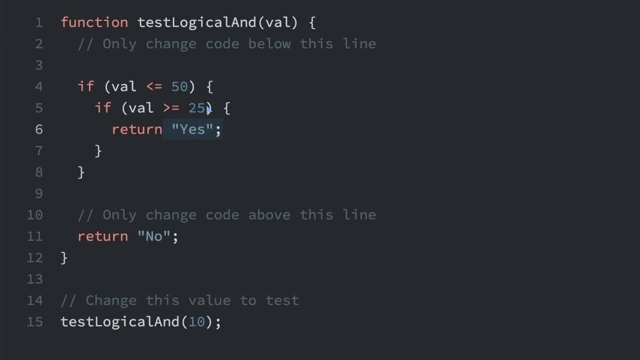 then it's going to return Yes, But there's an easier way to do this to do is copy this where it says value is more than or equal to 25.. I'm going to delete this nested if statement, So we don't need that if statement, and I'm going to use the and operator. 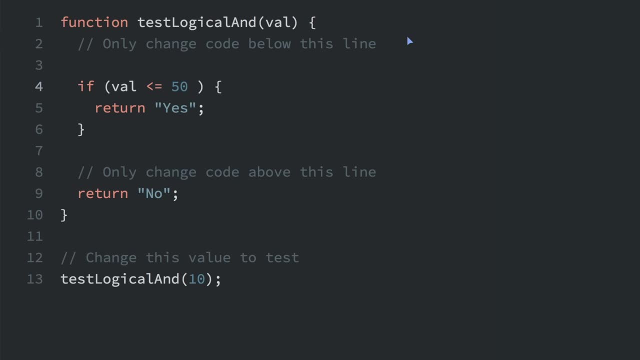 So we have less than or equal to 50. And if I put two ampersands like this, that means- and now I'm going to put: value is more than or equal to 25.. So this says: if value is less than or equal to 50,. 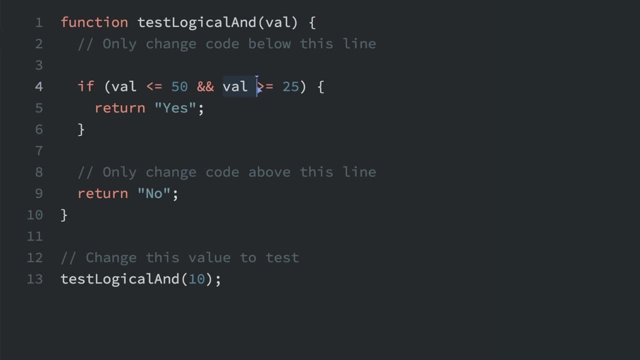 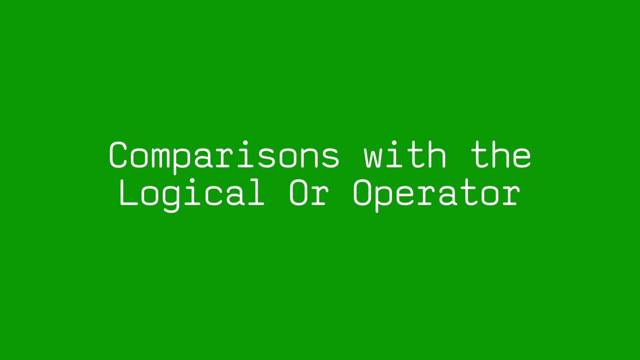 and the value is also more than or equal to 25,, then we're going to return Yes. So both this statement and this statement have to be true to get into inside this if statement. here In this code. here we're checking if the value is. 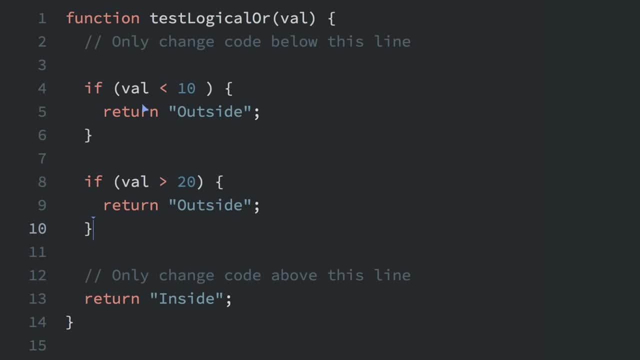 not less than or equal to 25.. And then we're going to put: value is more than or equal to 25.. So this is not between 10 and 20.. So if the value is less than 10, we return outside, And if the value is, 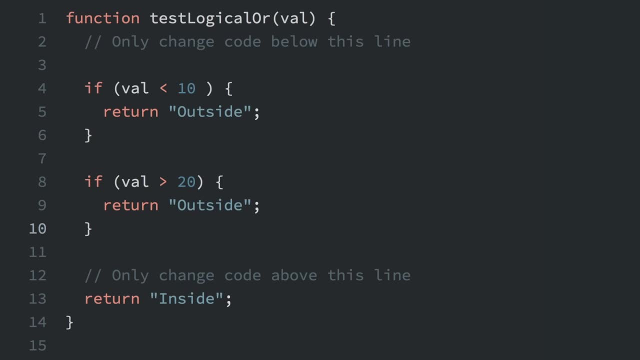 more than 20,, we return outside. there is an easier way to do this with the logical or operator, So I'm just going to delete this whole if statement here, And then I can add an or statement which is just two pipes. So I'm gonna put: Val is less than or equal to 25.. And then I'm going to put: the value is less than or equal to 25.. And then I'm going to put Val is less than or equal to 25.. And then I'm going to put Val is less than or equal to 25.. And then I'm going to put Val is more than 20.. 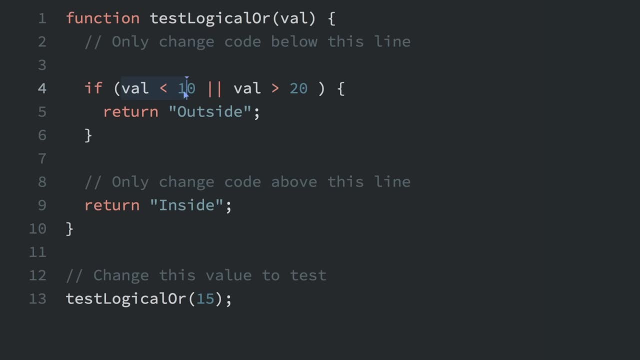 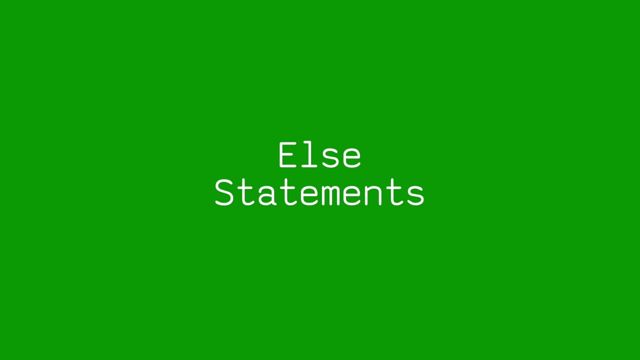 here. So now we're checking if the value is less than 10.. Or if the value is more than 20.. Either way, we're going to return outside, And if that's not true, we'll return inside When an if. 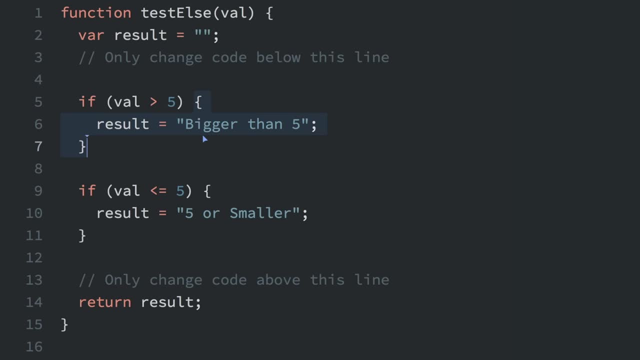 statement is true, normally the block of code right after the if statement will be evaluated And if, if it's not true, nothing happens. But with an L statement, an alternate block of code can be executed when it's not true. So this is a perfect use case. If value is more than five, the result 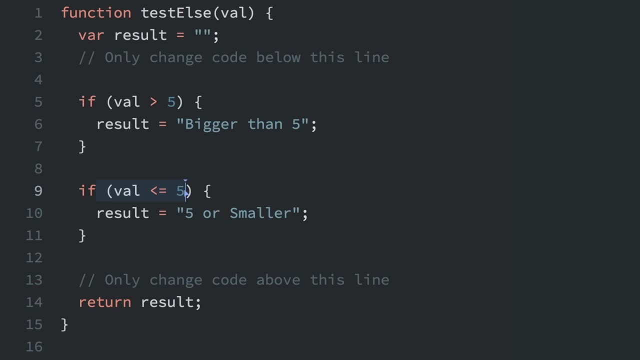 is bigger than five, If there is. if the value is less than or equal to five, the result is five or smaller. we can do this with an L statement. So I'm just going to type in else here And then we can just delete this whole if statement, just like that. And now we have: if the value is less. 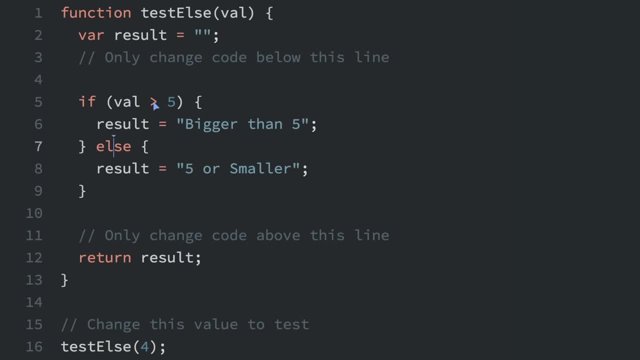 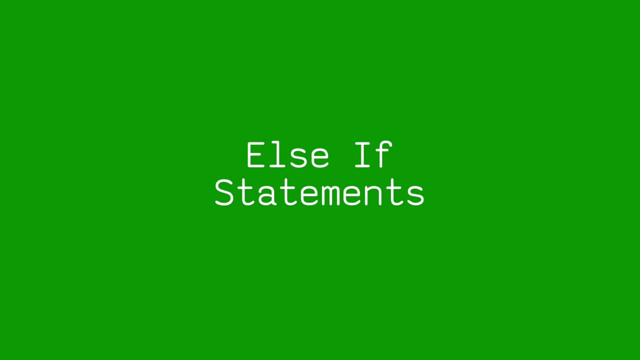 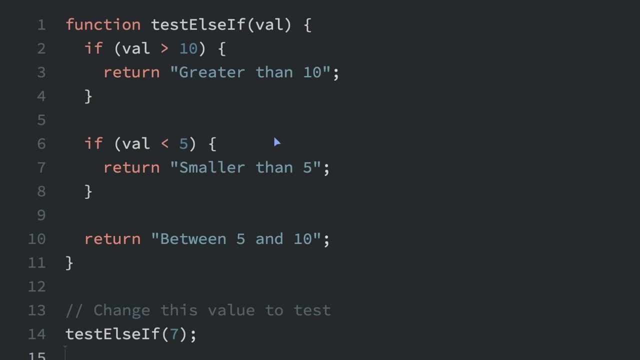 than five, the results will be bigger than five. else, if it's, which is, if it's not more than five will return five or smaller. If you have multiple conditions that need to be addressed, you can use else if statements. it's a way of chaining if statements together. In this example, we have 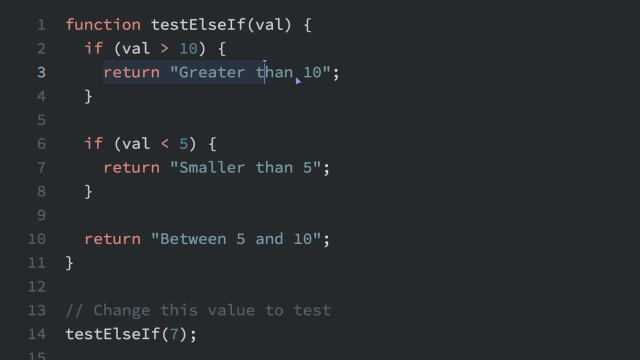 three conditions. If value is less than or equal to five, the result is less than or equal to five. If value is more than 10, we're going to return greater than 10.. If it's less than five, return smaller than five, or else we're going to return five and up. So this is a perfect use case for an. 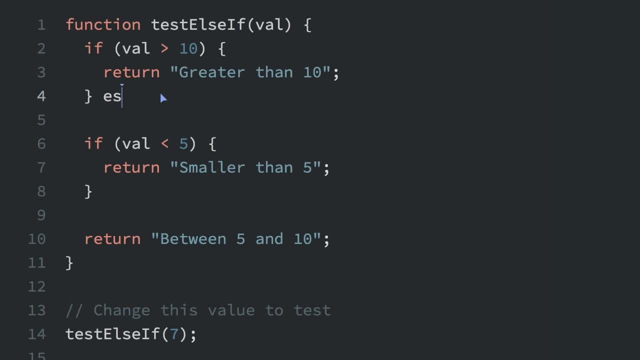 else if statement. So this is how we do it. We'll do else And then just we're going to add the if statement at the end of the else. I'm just going to delete all this stuff. So else if value is: 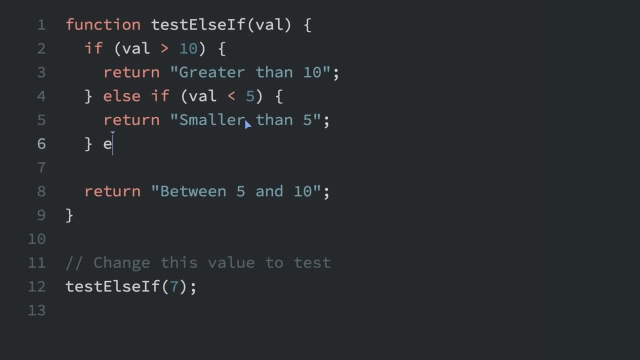 less than five. and then we're going to have one final else statement else, And then we're going to put this statement here, this final return, just going to cut that and then paste it right in there. So now we, instead of using multiple if statements, we have the if and with the else, if. 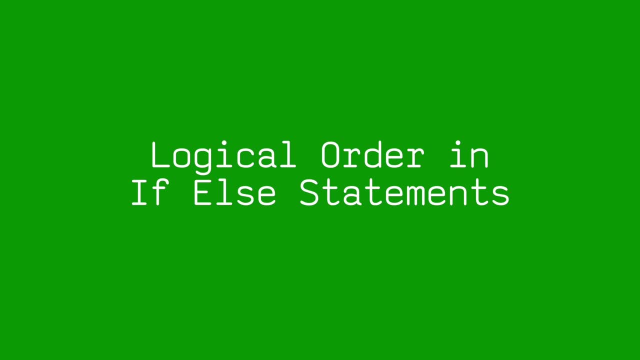 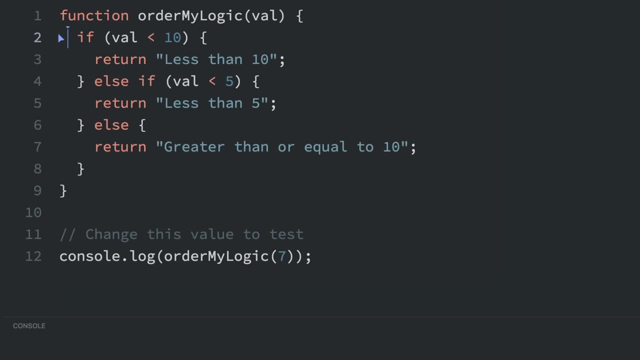 and then we have the else When you're using else if statements. order is very important. Let's look at this example here. In this function, First we check if the value is less than or equal to five and return less than 10.. Then else, if we check if the value is less than five and return less. 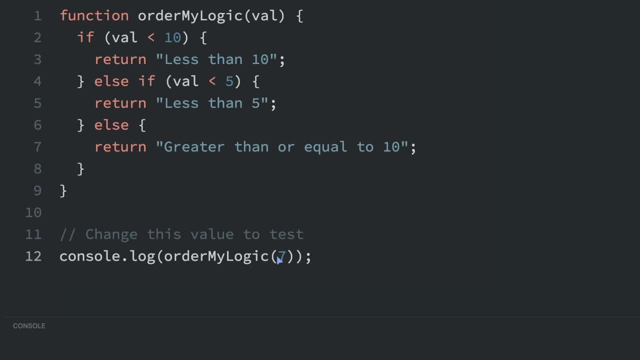 than five. Well, if we look at this example and we pass in the number seven- if I run this, you'll see it's going to say less than 10, which is what we want. However, if we put three, 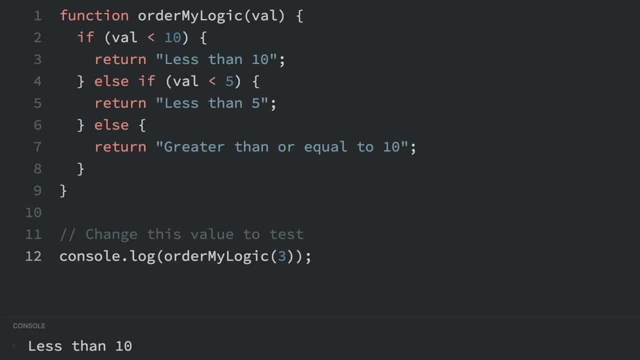 it's still just going to say less than 10.. Really, we want this to say less than five, because it is actually less than five. However, the this is in the wrong order, So what we need to do is change the order. So this should be five, this should be five and this should be. 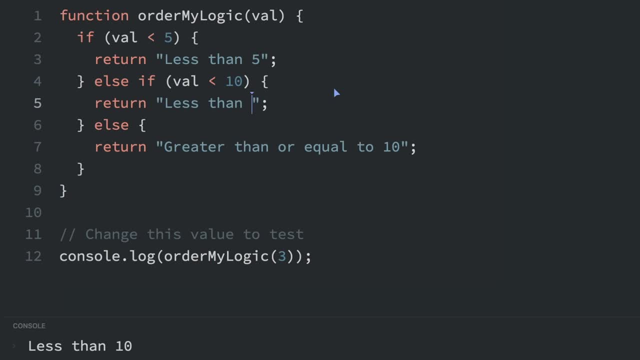 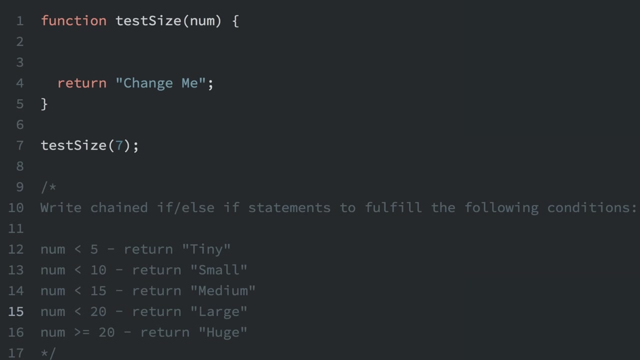 10. And this should be 10.. So once the first condition is met, it doesn't even check for the rest of the conditions. So that's why it's important to think about the order. So if we run this now, yep, less than five, that's what we want. You can also chain if and else if statements. So I'm going. 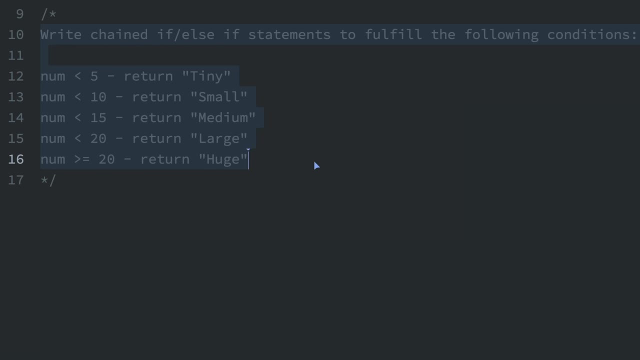 to complete the following challenge here: right chained if slash, else if statements to fulfill the following conditions. So we have these conditions where if the number is less than five, we're going to return tiny, if it's less than 10, return small, and so on. So what I'm going to do is actually just 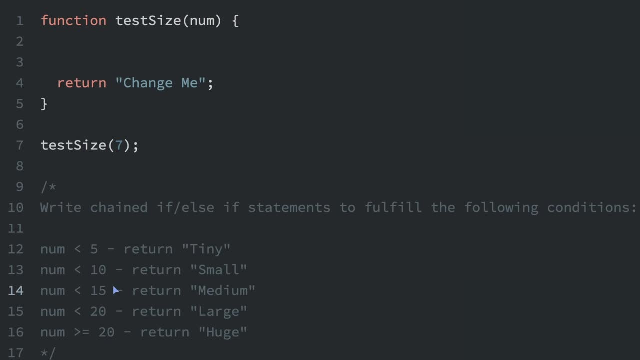 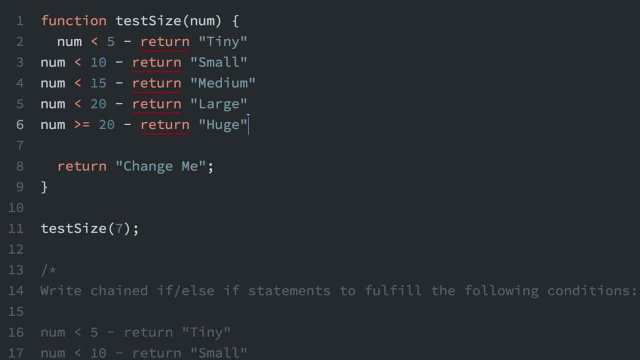 copy this right here. So I'm going to go ahead and copy this And then I'm going to go ahead and paste it right here, Because this is written as part of it's written exactly how we want to be written. I'll just paste it here And I'm going to just add the if and else statement. So it's. 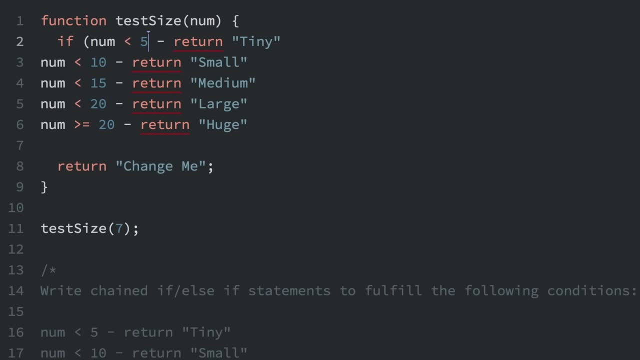 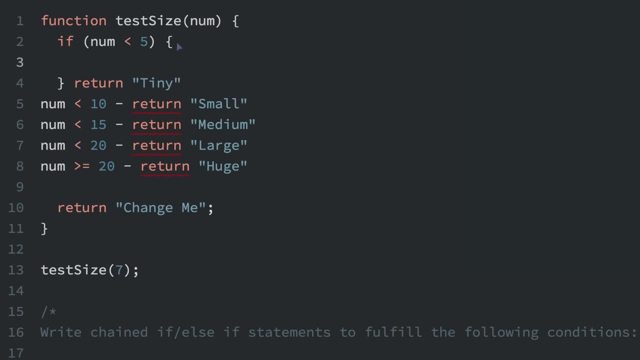 gonna be if, and then we put this in parentheses, because the condition is always in parentheses: if number is less than five, then we're going to use the curly braces And we're going to return tiny. So let's move that up here. I'll cut it and paste it. Now we're going to use an else. 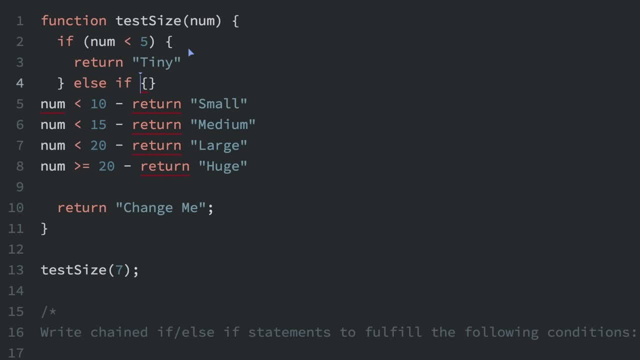 If statement- and I got the curly braces First of all. also, I need to put the condition in these parentheses. I'm just going to cut: this number is less than 10, put it right here, And we're going to return this small. So I'll put that in the curly braces here And then we have another else: if. 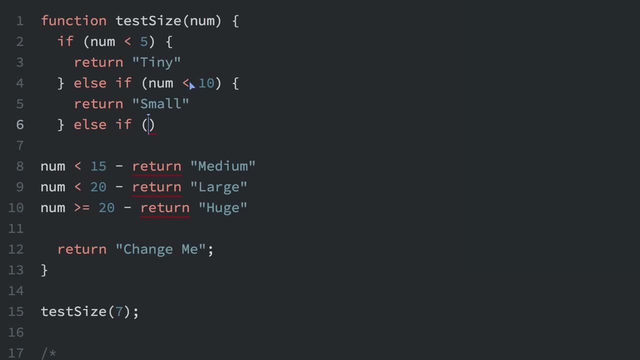 statement: Else if and the condition, just like before, number is less than 15.. Put that in the. there We get. we always need the curly braces to show what's going to happen in the if statement, So I'm just cutting and pasting the text text Again. we have an else If and then we have this: 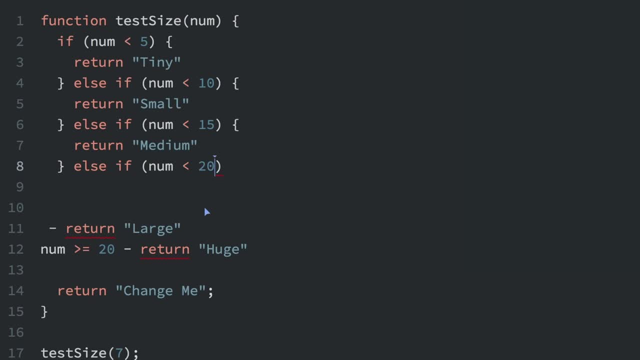 here And we have return large And now they're actually. the final thing is just going to be else. We don't even need an else. if at the statement at the end we're not, we don't even need to put the condition, because if it's more than or equal to 20, that's going to be everything else. So I'm just 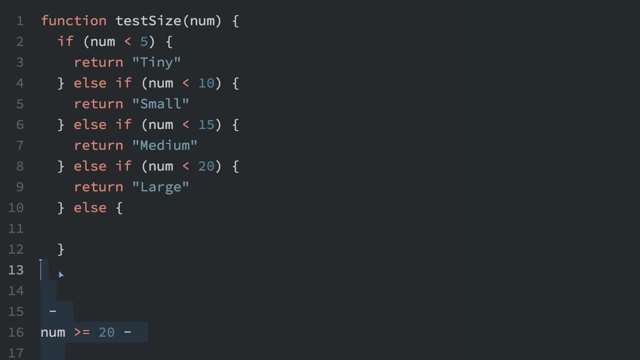 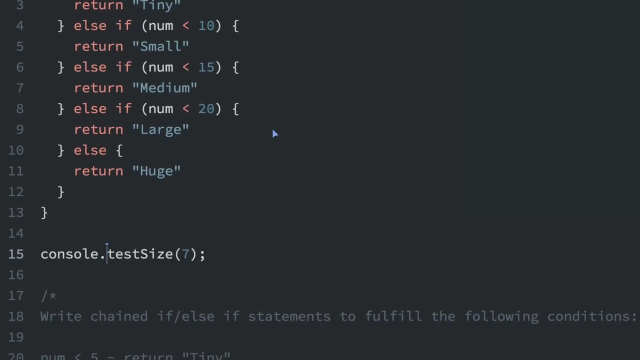 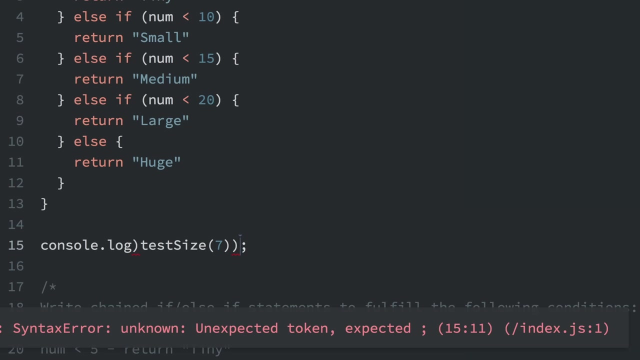 going to cut this. we don't need any of this stuff here And we're just going to return large. So with this one test here for test seven, we can actually console that log, that console dot log, And see what returns for seven. we can try a few different things. Oh, we have an error here. Oh, 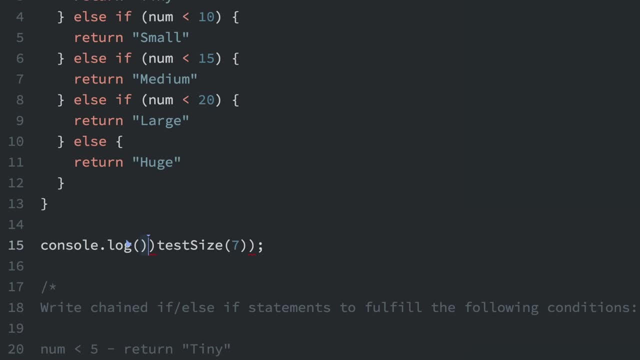 forgot to put this parentheses wrong way. Let's try that again. Small, but if this is 20,, it should be huge, And if it's 19,, which will be less than or equal to 20,, it should be less than or equal to. 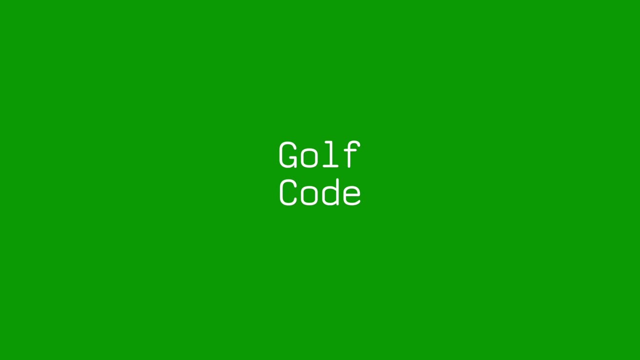 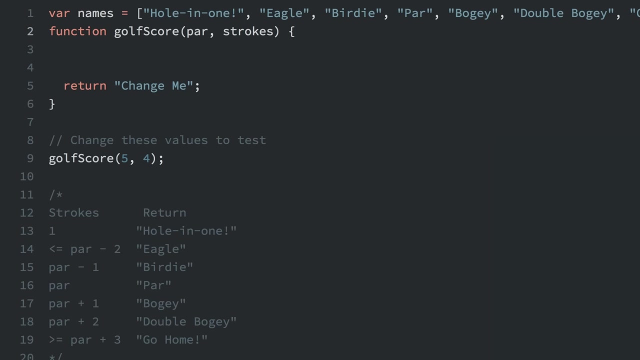 20. We should see a large Yep that work. In the game of golf, each hole has a par, which means the average number of strokes you're supposed to use to get the ball into the hole. So depending on how far above or below par your strokes are, there's a different nickname. So here are some of the. 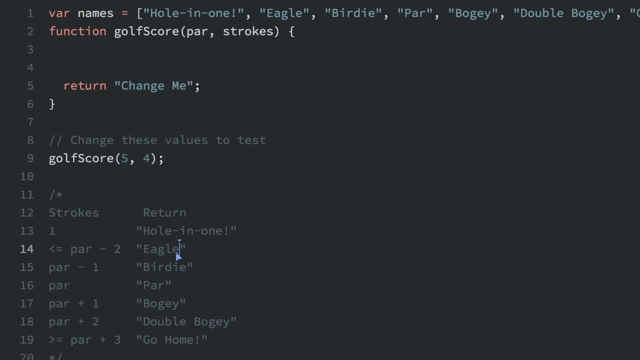 nicknames hole in one eagle birdie, par, And we're going to write a function where you pass in the par And you also pass on the strokes. you can see up here par and strokes, and it's going to return the nickname. So 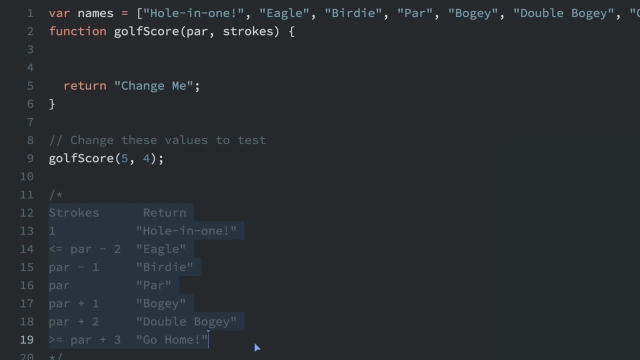 that's what we're going to write. you can see. this table here shows what we have to do. If the strokes are one, then you get a hole in one. if the stroke is less than or equal to par minus two, you get an eagle, and so on, And we also have this array. that's going to make it easier, because we 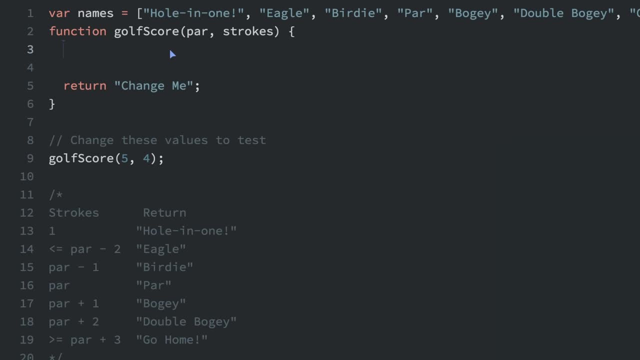 can just use things from this array instead of typing out the words. So we're going to start with this, Start with an if statement, if, and then we have to put the condition: if strokes equals equals, that's the equality operator. we don't want to use a single equal sign because that would be the 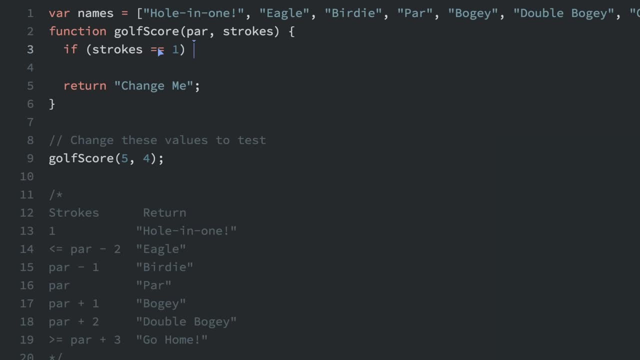 assignment operator. If it equals one, then we can return And we can see down here. we're going to return hole in one, but we can just use it from this names array. So it's going to be names And this is going to be. 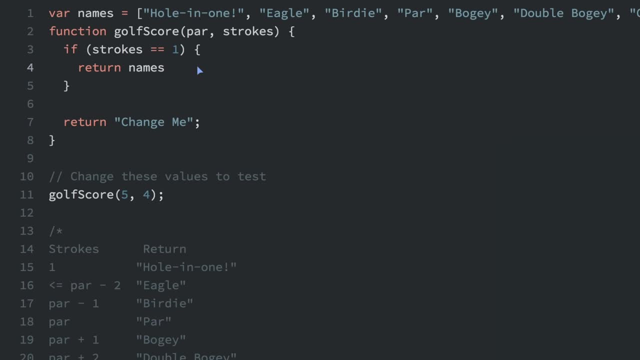 indexes zero of the array. So we'll do names and then zero, And then we can do an else, if else, if, and then we can put the condition strokes at the spell strokes, right Spokes, and then we can just actually copy this right from here: less than or equal to par minus two, And 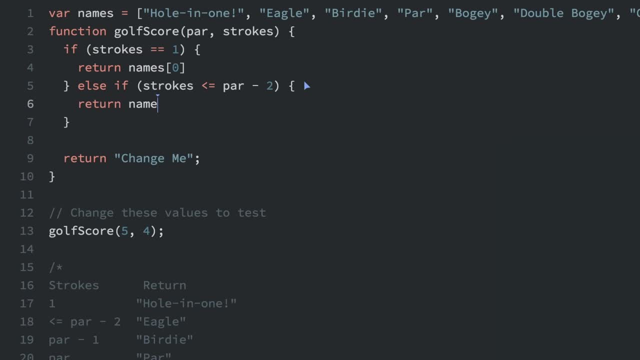 then we're going to return name And this will be the index one which is an eagle. At this point I can do some copying and pasting. I'm going to copy this whole thing because a lot of this rest of this will be else, if so else. 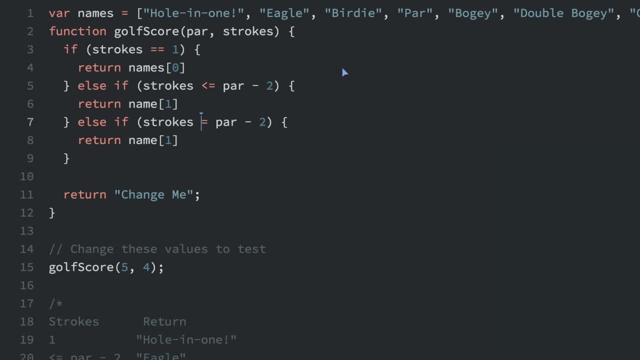 if strokes is, this time is going to be equal to par minus one, And we're going to return this me birdie, which is an array index too, And I'm going to continue just like this. So this time it's if strokes equal par, we're. 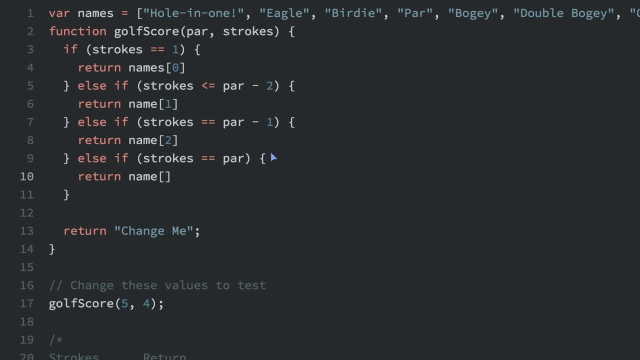 going to return name index three. c0123 is gonna be the word PAR up here, though just keep just like this. Now it's going to be par plus one. we'll change this to 4. now it's going to be par plus 2, and we'll change this to 5, which is going: 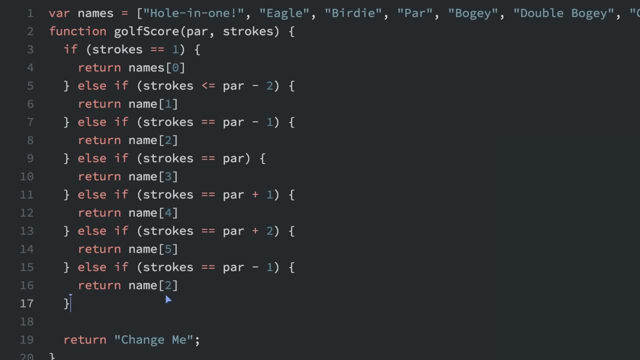 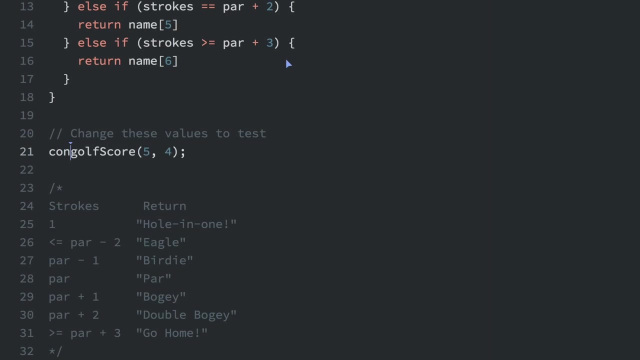 to be the double bogey. and finally, if strokes is change this to more than or equal to par plus 3, that means you did very poorly, so you should just go home. so it's going to be name index 6 and we don't need this anymore. so now we're going to do some tests here. I'm going to do a console console. 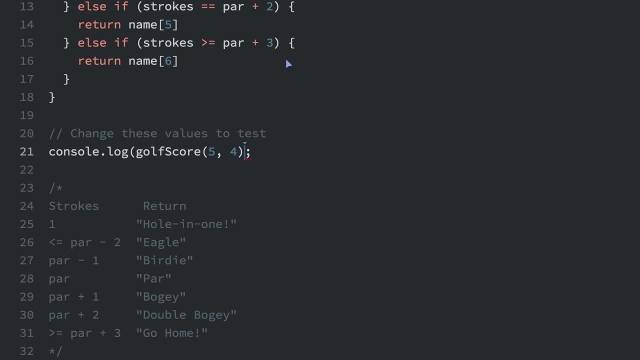 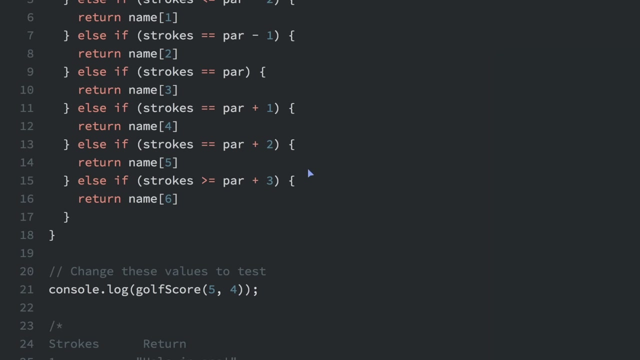 dot log and we're going to pass in the function that we're calling. so in this case the par is 5 and the strokes are 4, so that should result in a double bogey. so that should result in a double turn birdie. let's see what happens. no, okay, that's not what I expected. it's because this should be. 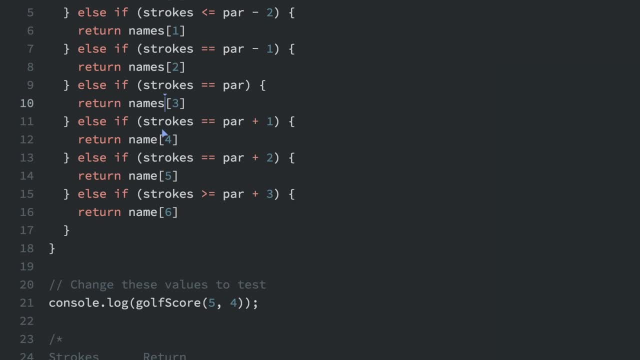 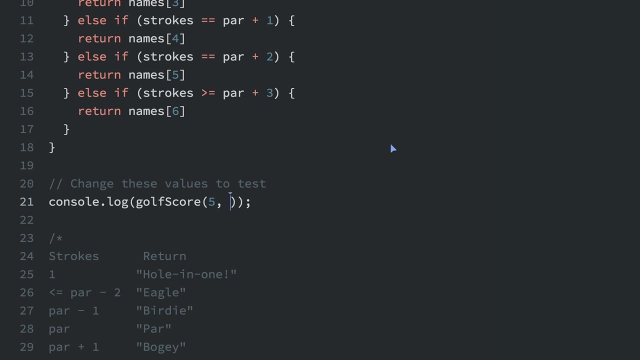 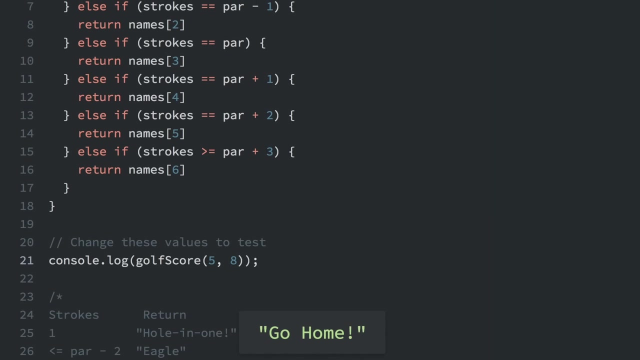 names spell this wrong. okay, that's why sometimes better to check before you go through the whole thing. you can test things as you go, but let's do that again. yep, birdie. and if I type in to here Eagle, if I type in eight, it's probably gonna tell us to go home. go home. yep, we just completed this. 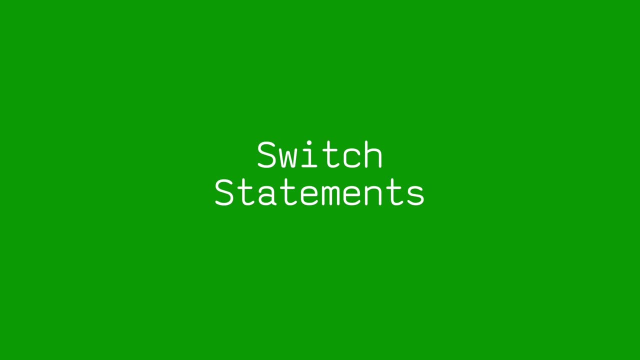 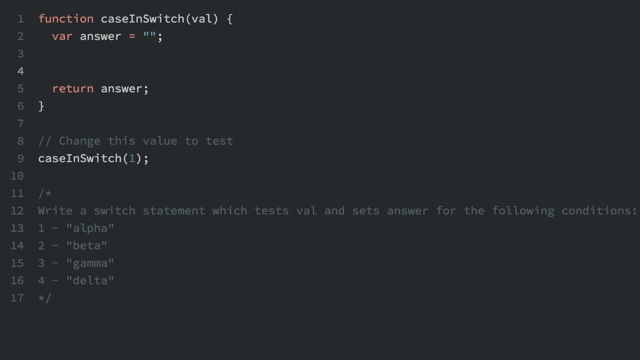 challenge. instead of using chained else if statements, you can use a switch statement, a switch statement test of value and can have many case statements which define various possible values. so let me show you how that works. here we're going to write a switch statement which tests Val and sets the answer to the following question. 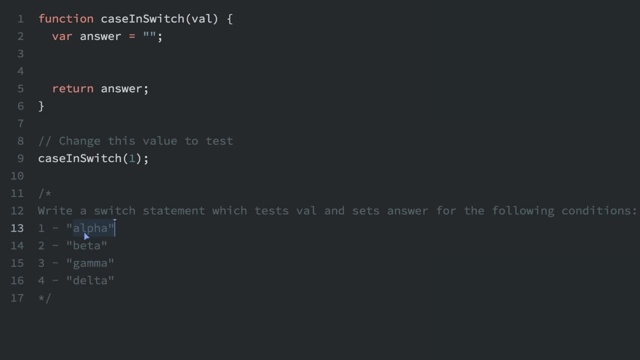 conditions. if we pass on one, the answer should be alpha. if we pass on to, the answer should be beta, and so on. so let me show you how that works. we'll just type in the word switch- that's a keyword here- and we're testing the vowel that's passed into this function. so it starts off kind of like. 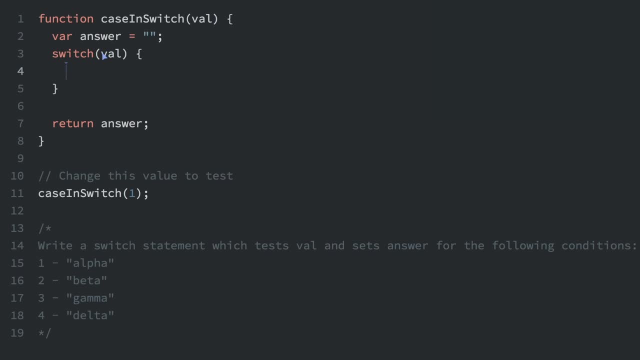 an if statement and right now. so we're gonna compare the vowel to the different cases that we have. so we'll have case and the first number is going to be one. so here we're saying, if the case of Val is one, if Val equals one and it's using the strict equality operator, so it's like the equals, equals, equals, it's going. 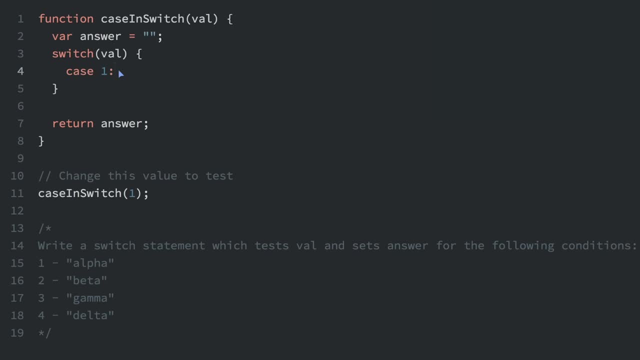 to make sure that the type of the variable are the same. so a string one and a number one will not be equal. but if the case is one, then we're going to set answer to equal alpha. we'll just use the like this alpha and then we are going to break. break means that we're at the 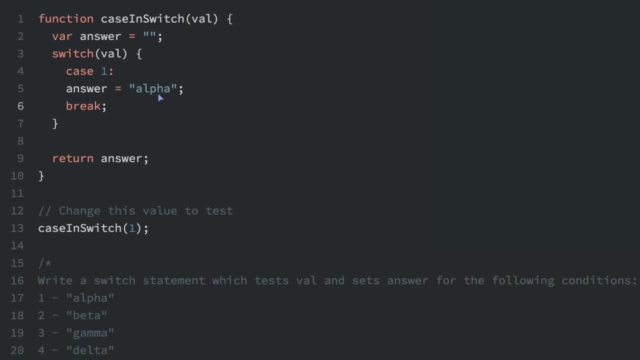 end of that case statement and once you break it it just goes to the end of the switch statement. it doesn't evaluate anything else in the switch statement. so we're also going to have case two. and one thing I forgot that we're going to just going to indent that. so it's. 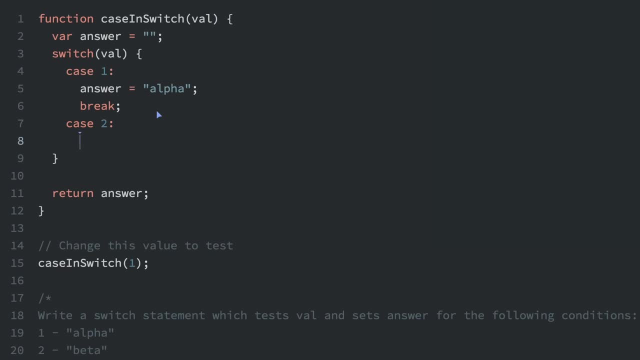 easier to see the different cases. and case two: the answer is going to set equal to beta, and then we always need the break statement. if you don't have a break statement, it will just run through to the next case statement automatically. so if the case was one and you did not have a break here, 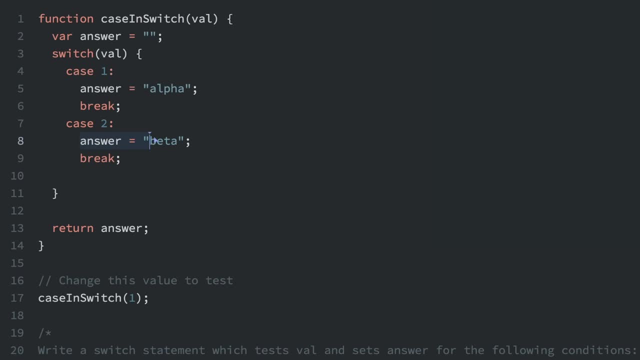 first it would set the answer to alpha and then it would set the answer to beta. it would just skip over right to the next case statement. but since the break is here, it's going to go out of the switch statement, so it will go start running the code after this last curly bracket. so now we're. 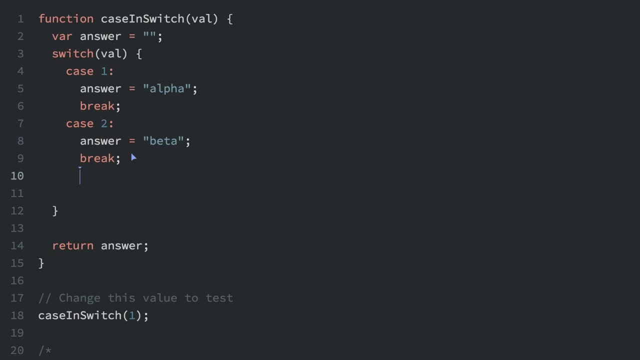 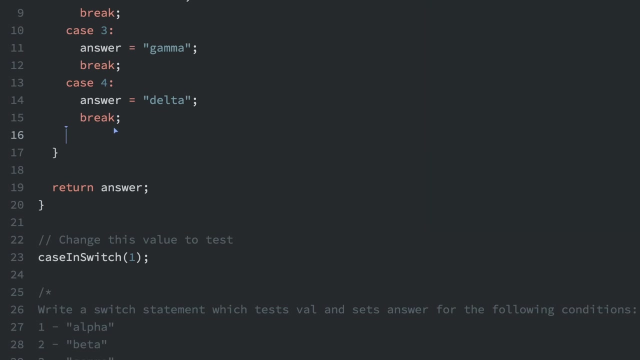 going to case three. we'll just do some copying and pasting here, and we're gonna have four cases, so I'll just do the rest of the cop the pasting here. so we'll have three and four alpha beta and then we have gamma and Delta and we know that the switch statement is over because we have this: 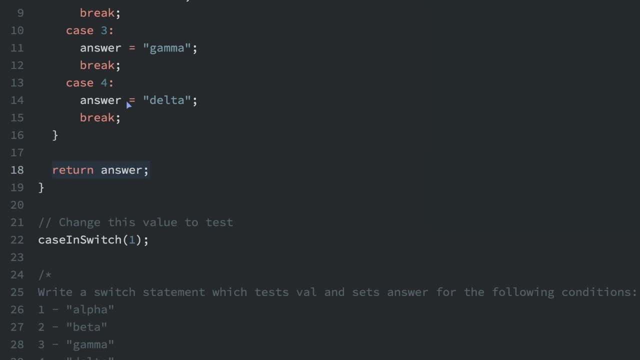 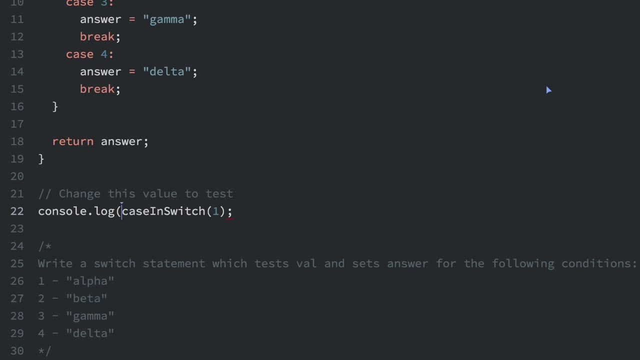 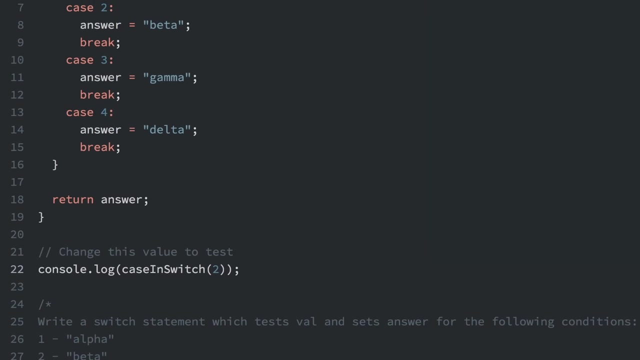 file, curly bracket and then we're just going to return answer. so let's do some tests. to really test this, we're going to have to add a console dot log here to log what it's going to be, and I'll run this: alpha good now. 2 should be beta, 3 should be gamma good, and we'll just assume 4 is. 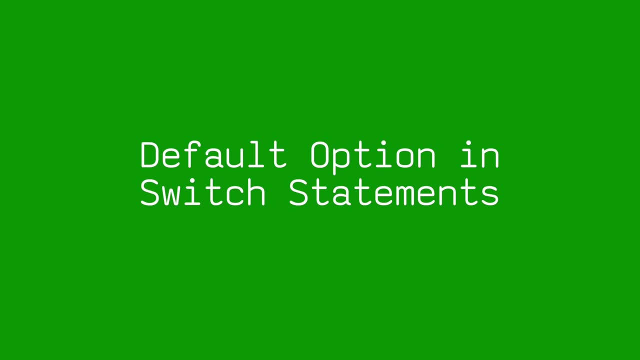 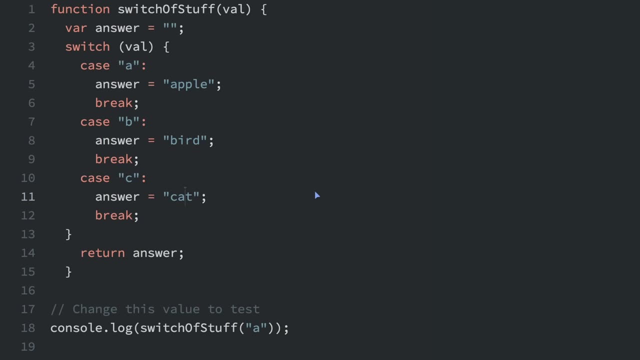 correct, so we're done. now I'll talk to you about the default option in a switch statement. the default option is kind of like else in an if-else statement. so here's a switch statement that's very similar to the one we already saw and it's inside this function where we pass in a value into the function and we're going to check. 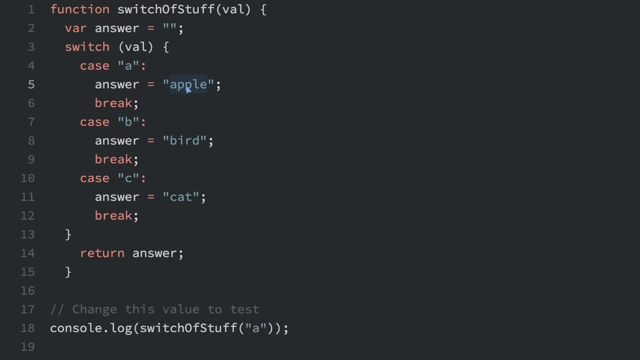 if the value equals a. if it equals a, the answer is going to be set to Apple B enter. set the bird, see cat. so in this example we can see that we passed in here, we pass in the a and it returned Apple because that was one of the options. but what if we pass in something else? if I pass in the? 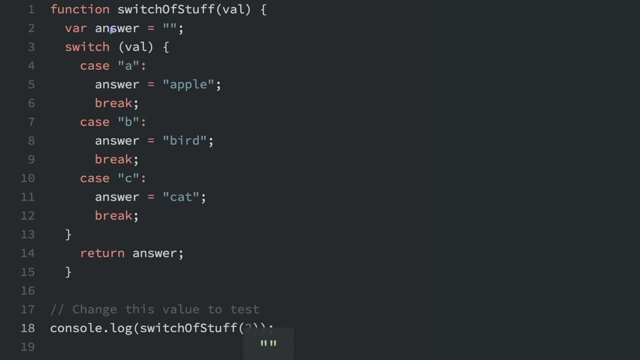 number two: here it's going to return an empty string. that's because the answer is set to an empty string and we never override the answer here, so it just returns that empty string. what if we want to return something any time? a, B or C is not passed through. so for anything else that's passed into the function, we're going to do default. 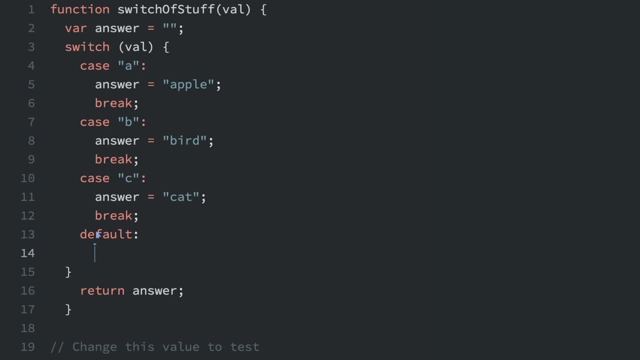 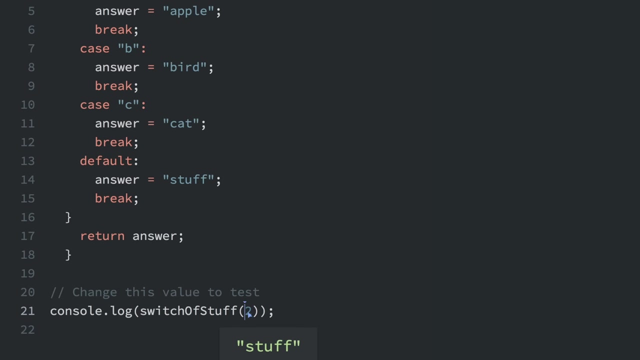 this is like the else statement. so the default: we're going to answer equals stuff again. we're going to have the bird set to a if-else and we're going to pass in the number two and we're going to break. so now, whenever we pass in something that's not a, B or C, it's going to return stuff, so we can. 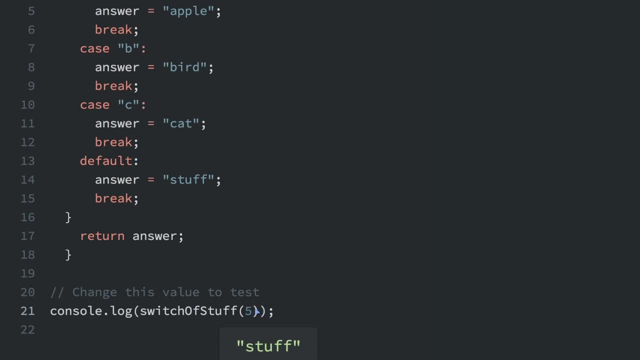 pass in five. it's gonna rare and turn stuff. but if I go back to passing and see one of the things we have a case for, it will return cat and that's the switch statement. sometimes you want to switch statement where multiple inputs give the same output. 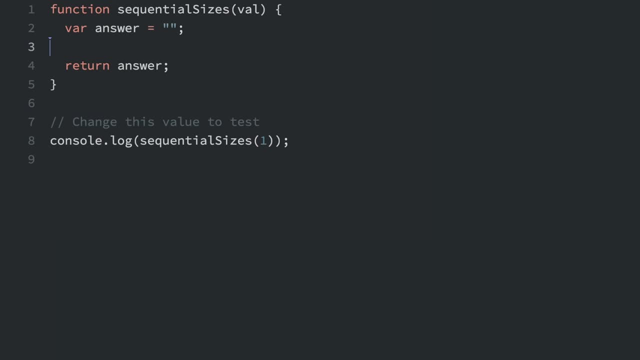 well, that's easy enough by omitting the break statement. let me show you how that works. so let's get a switch statement here and we're gonna have Val. that's what's passed into the function and in this case we want the case of one, two and three all to return the answer of low. so I can do it. 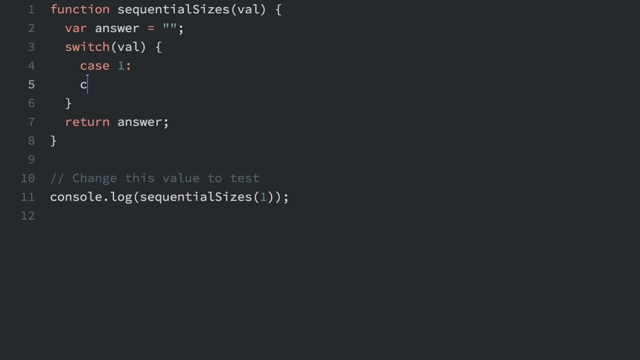 like this case one, and I can go straight into case two, and then I can go straight into case three, and since I don't have any break statement between each cases, it will just keep going to the next one automatically. and now I'm gonna say that the answer is gonna be set to equal low, and here 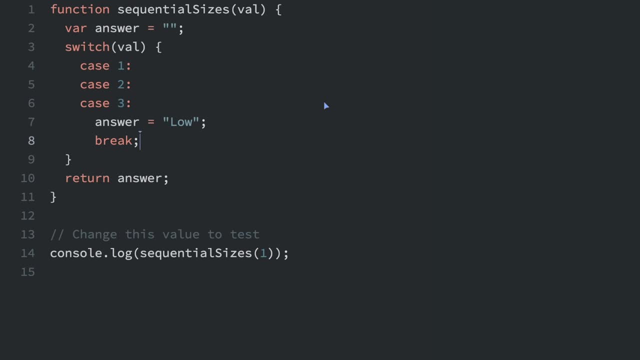 is where I put the break statement. okay, now we're gonna do the same thing with cases four through six, and actually I'm just gonna do some copying and pasting. I'm gonna copy all this and now we're gonna paste and paste. that's four, five, six. we're gonna do the same thing with seven, eight, nine. so I'm gonna do copy and. 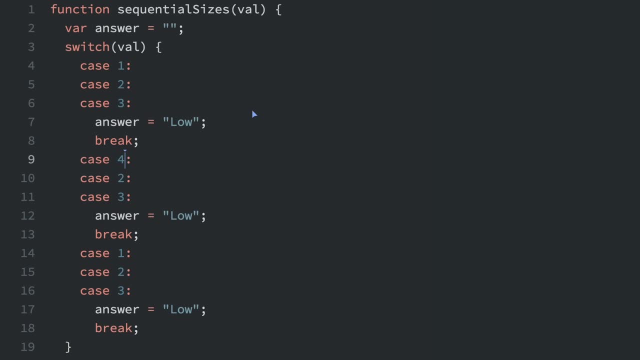 paste again and I'm just gonna update the code. so this is gonna be four, five, six, we'll have seven, eight, nine and we're gonna have mid and high. so if the case is one, two or three, like for instance, if it's one, it's gonna pass through two and three to get low and then it's gonna break out. if it's. 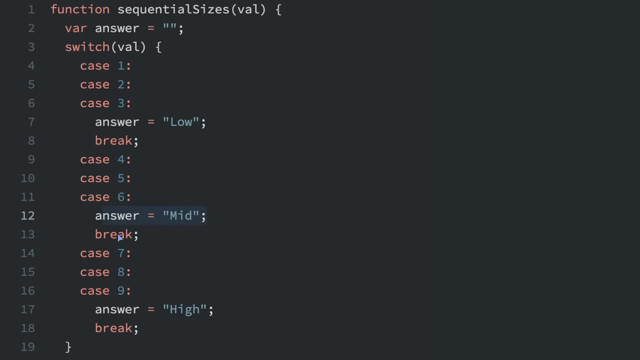 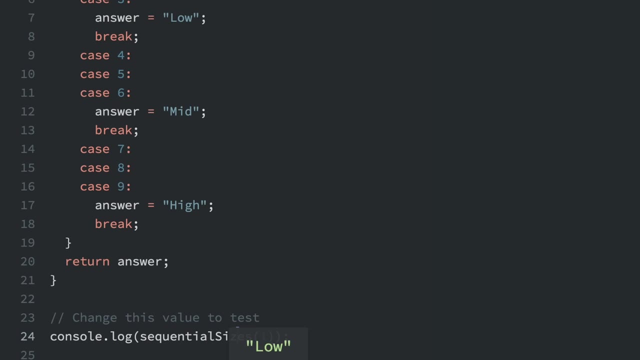 four, five or six, it's gonna pass through to get to mid and it's gonna break out. seven, eight, nine, it's gonna pass through to high and break out. so let's test this out and see. since we're passing in the number one here, it's gonna be low, but if we pass in five, 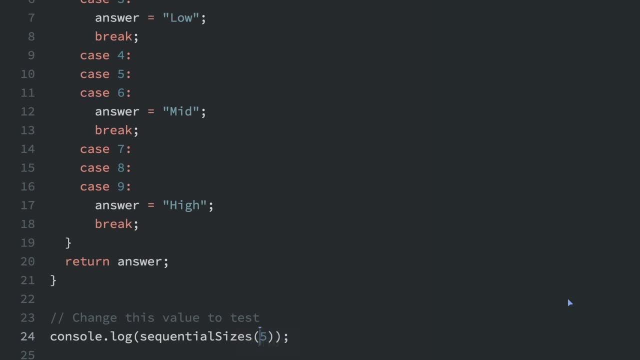 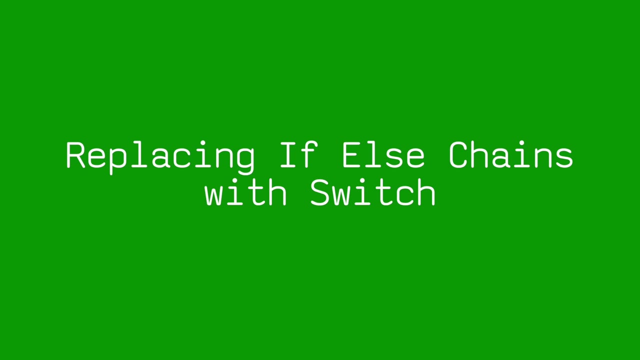 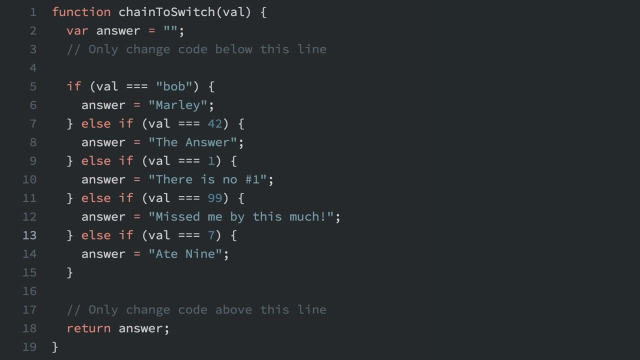 we should get mid, and if it's seven, eight or nine we should get high. sometimes a switch statement can be easier to write and easier to understand than a chain of if-else statements. so I'm just gonna- so we're going- to change this chain of else if statements to become a switch statement. so let's. 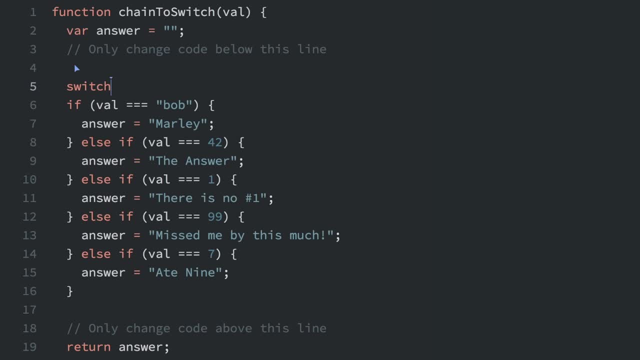 do that right now. so we're gonna start with the switch keyword and we're going to be evaluating the value with open curly bracket and we'll have to make sure to have an in curly bracket. and so, for a case, Bob, we're going to set the answer to Marley and 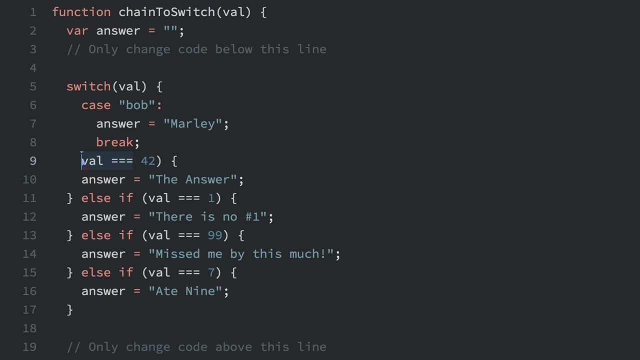 then we need to have a break in here. for case 42, we're gonna set the answer to the answer. or case one, we'll set the answer to. there is no number one, oh, we need a break up here. or case 99: the answer is missed by this much. and then we need a break. now we have for case seven. 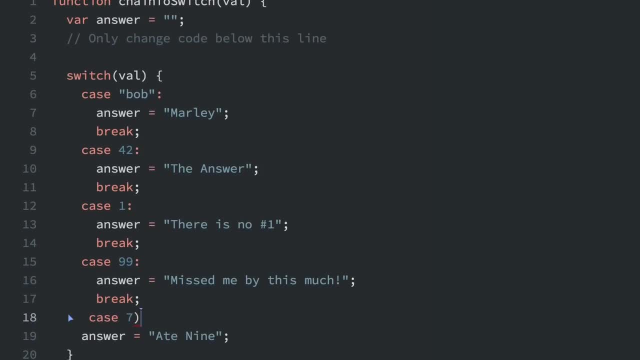 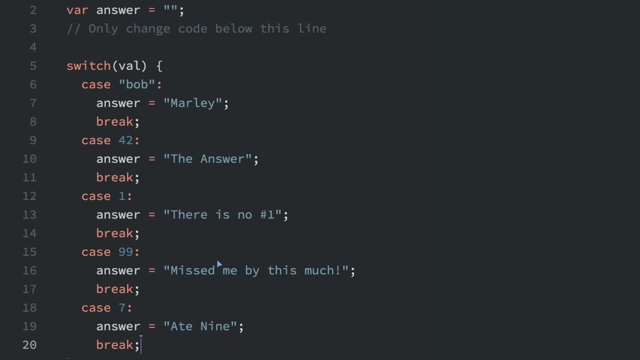 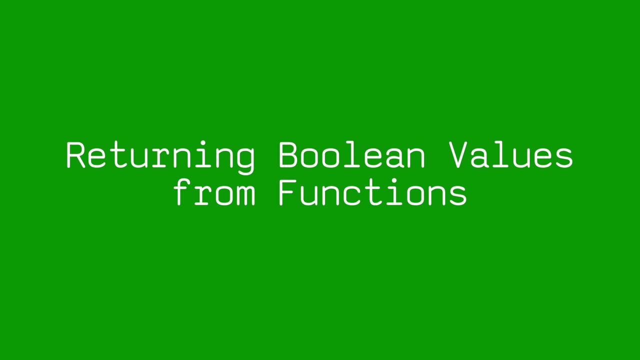 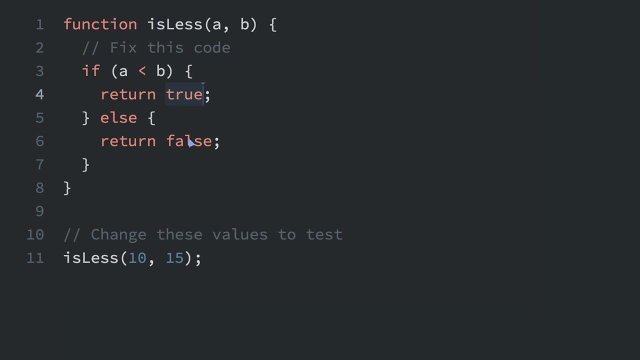 well, seven, eight, nine and break, and now we just changed that chain of else if statements into a switch statement. here's a little trick: when you want a function to return a boolean, a true or false value, you can see in this function we're checking if a is less than B and if so we return true, else. 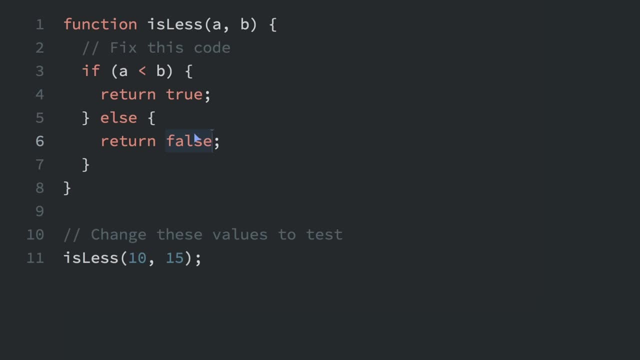 we return false. you may remember from before that all comparison operators return a boolean true or false value. so instead of using this if statement here, we can just do that we can actually delete all of this and just return the result of this return. we're just returning the result of a is less than B, so this is going to be true or false. 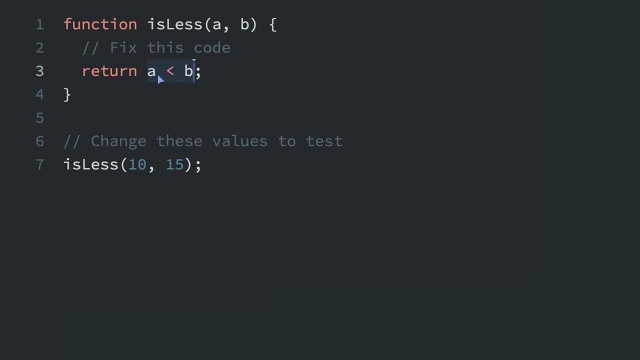 and we can just skip that whole if statement logic and just return this so, and then you can jump up and down for out into the function and you'll have to change the value itself to it, because we've already changed the value of it right, so we need to get it into our function. and by means of need it to change the sure or false. I'd prefer thatworking. it's going to change the value of the version up and down. hold true or false now, if it's痛 that warnings otherwise is already the full value, or if it's out and we can just apply change in the Draper's. 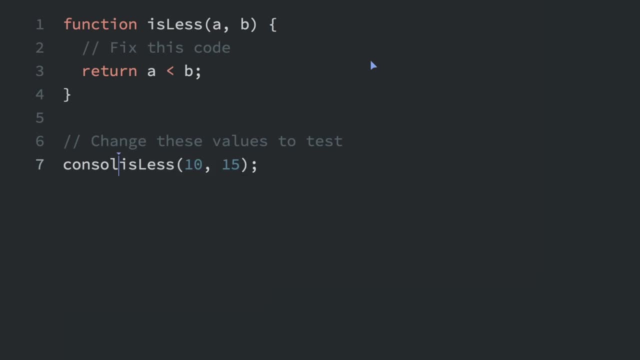 we console dot log this out. console dot log. we should be able to see if 10 is less than 15.. And is less than 15. It's true, But if we put a 20 here, then it's false. We've already seen a few. 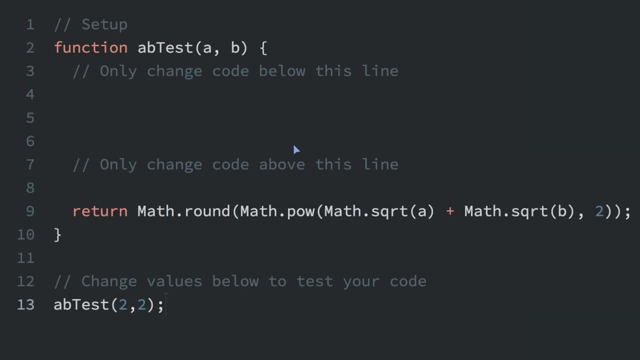 examples of this. but you can return early from a function with the return statement. So, if you see this, this function right here. we return at the very end of the function And so it leaves the function and returns this value from the function. But you can leave the function anytime with a. 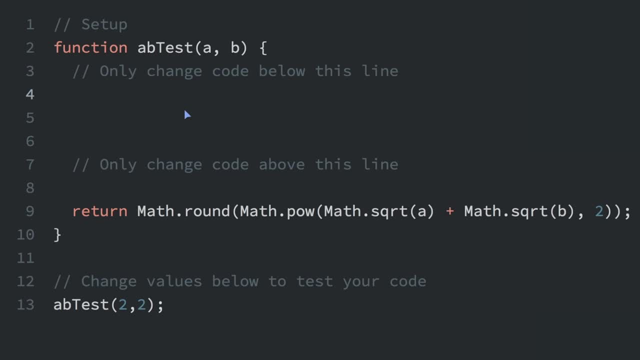 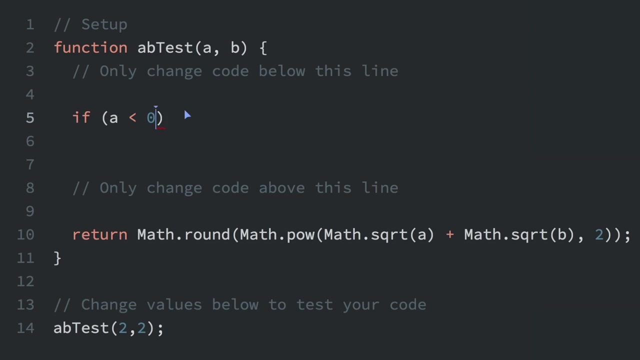 return statement. So we're going to modify this function so that if A or B are less than zero, the function will immediately exit with a value of undefined. So let's do that. we're going to set an if statement if a is less than zero. 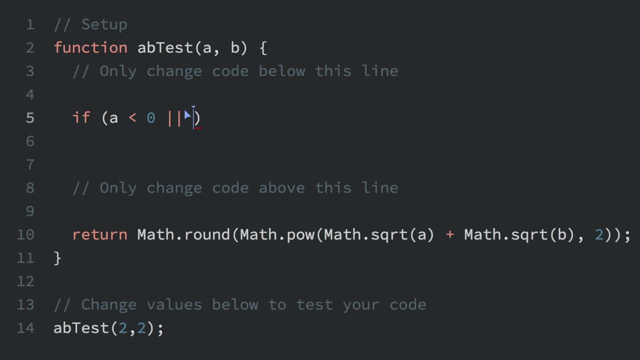 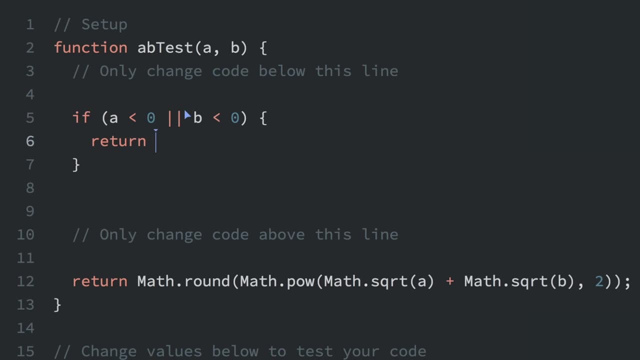 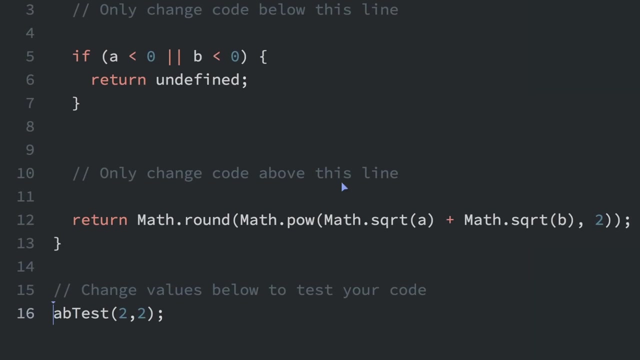 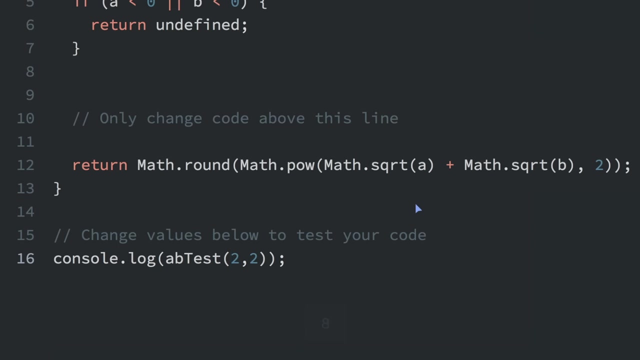 or it's two pipes. B is less than zero, then we're going to return on undefined. So we can do a test here: console dot log eight. but what if this is a negative number? it's going to return undefined. And if we do a test here, console dot log eight. but what if this is a negative number? it's going to return undefined. And 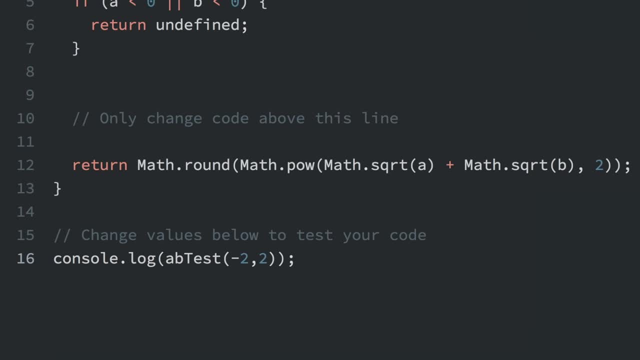 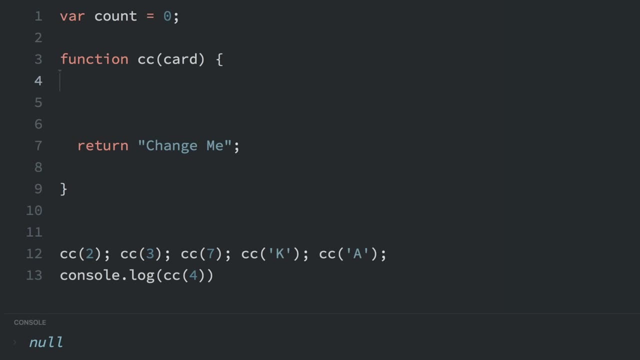 Escrimba has a little quirk here, where it just shows no, but in a browser it will show undefined. We are going to create a blackjack card counting function. So how card counting works, or at least how this function is going to work, is that when you see a low card, the count goes. 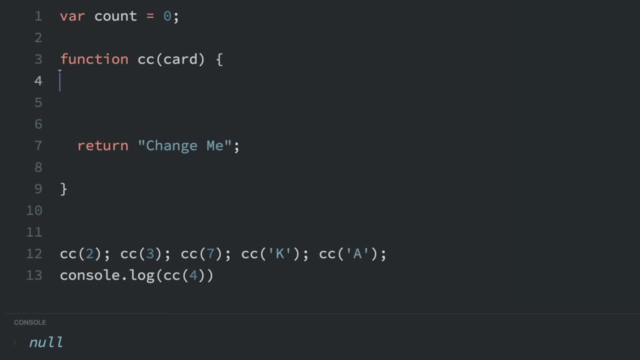 up, And when you see a high card, the count goes down, And if it's a middle value card, the count goes top. So when you see a low card, the count goes below down If it's a middle value card. the count goes down. And when you see a low card, the count goes goes down. And if it's a middle value card, Okay, in this integration represent one of the other functions. And then when you see a button level, vienen las abandon de la capitario. 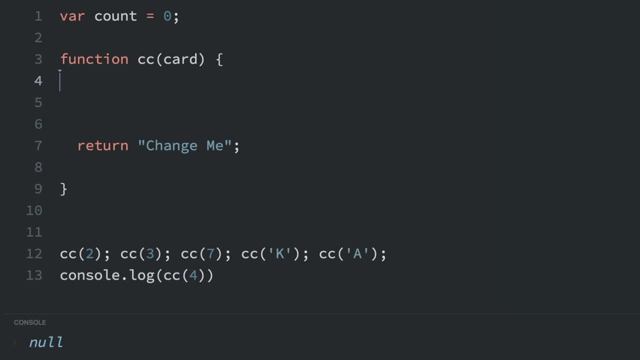 count stays the same And then when the count is positive, the player should bet high And when the count is zero or negative, the player should bet low. So we are going to use a switch statement to figure out what card has been passed in and what to do about it. You can see that the function looks. 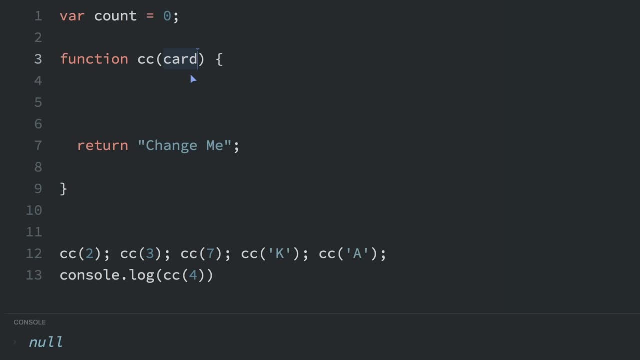 like this CC, and we pass in a card And, depending on what the card is, it's going to increase this global count variable or it's going to decrease it, or it's going to stay the same, And then we are going to return two things. we're not going to return change me- we are going to return the. 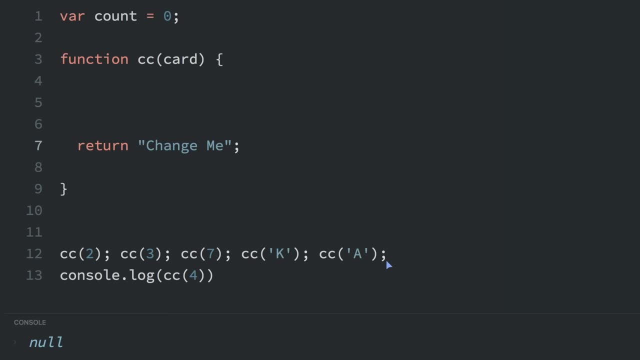 current count value and whether the player should hold or bet. So every time you call the CC function, it's going to change this count value and return the total count. So let's see how this is going to work. We are going to use the switch statement, like I said, and we're going to check the card value. that 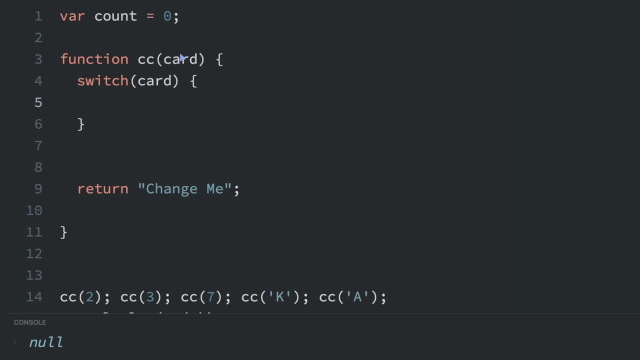 was passed in. So if the case is 23456, we are going to increment the count variable. So we're going to do like this case to. I'm going to do some copying and pasting If the case is 23456,. 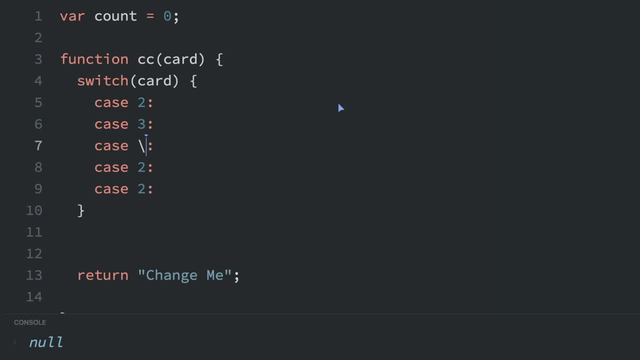 we'll just have to actually change these values. Now, there are many ways to write any program. this could be done with if statements and else statements. it could be even done with other other ways that we haven't even talked about yet. as long as the program works In this case, that's all that matters. So if you find a different way, 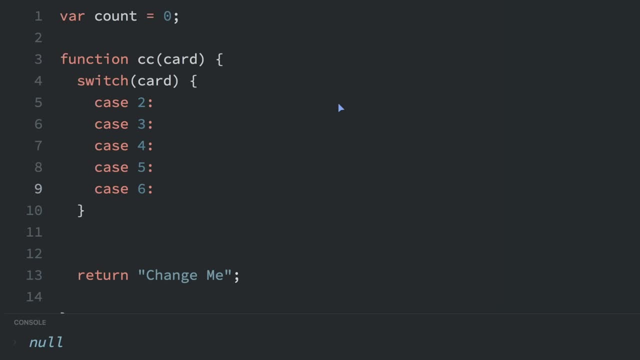 to write this program. that's great. So if the case is 2345, or six, we are going to. we are going to take the count value And if we just do plus, plus, that increments it by one and then we're going. 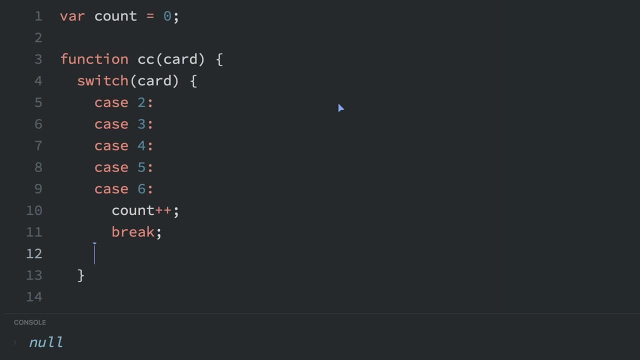 to break Now. if the case is 789, so let's paste in three of these Luke 789.. Actually, we're going to do nothing. that count is not going to change at all, So we don't even need case 7 or 89.. So instead, 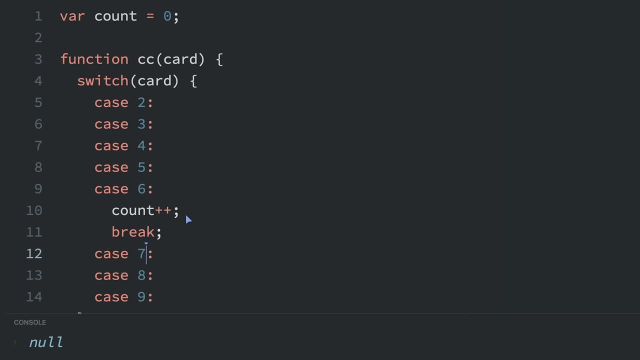 of doing 789, we just need to check in the case that something's actually going to happen. So we are going to decrement the count variable if we have 10 jack, queen, king or ace. So that's what we're going to. 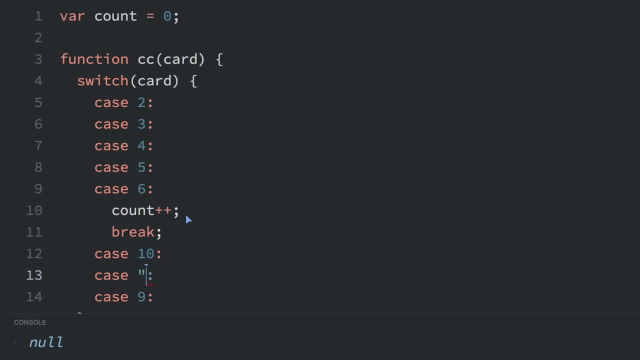 change this to 10.. Back queen king or ace. In this case we're going to decrement the count, So you can do count minus minus. So that's the same as count equals. count minus one, And then we will. 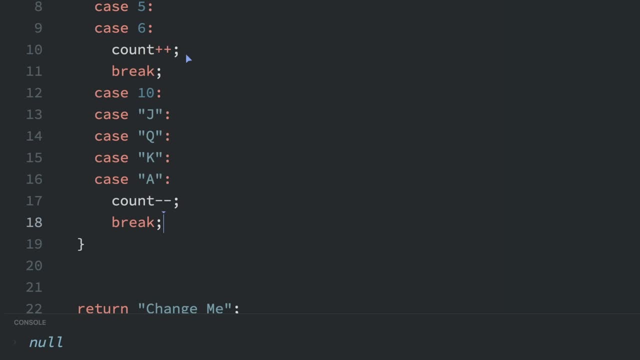 break. Now we we've taken care of the count and updating the count. Now we have to take care of what we're going to return. we are going to return the count And we're also going to return whether we are going to hold. 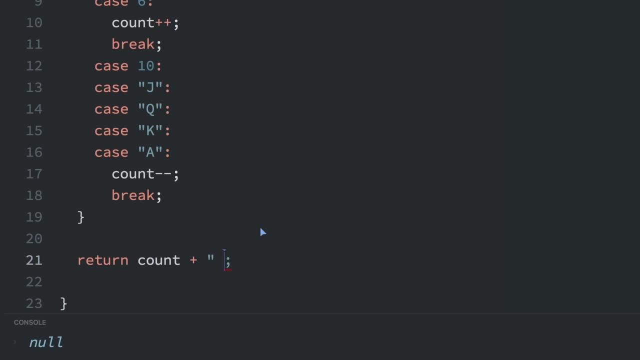 or bet. So we're going to actually return a variable, But first there's gonna be a space, there's a space between the number, And then we're going to return the hold, that variable. Now, this is a variable we haven't. 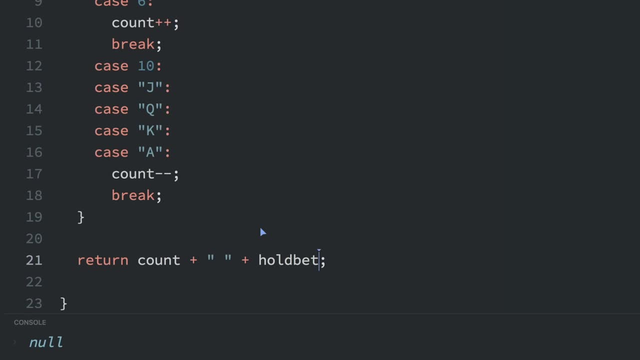 created yet. Normally, this would be the perfect time to use the ternary operator, But we haven't learned that yet And we're not going to learn that for a few more lessons, So I won't use that now. we are going to set what that hold that value is First. we'll create the hold that variable. 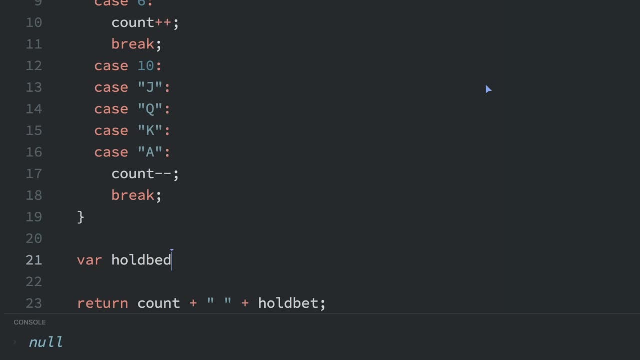 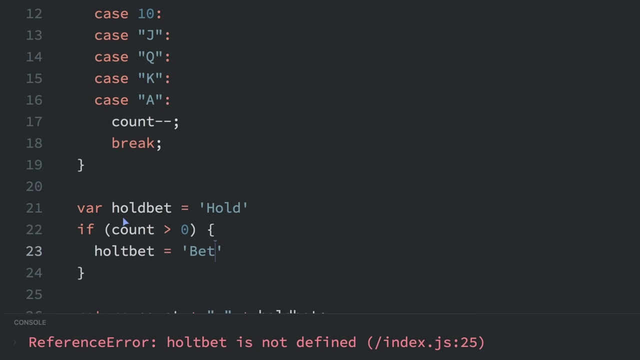 variable hold back And we'll set it to hold. However, if count is more than zero, then we can set hold back to equal. So now this should work. Let's test it out and see if we've made any mistakes. yet Hold that is not defined. Well, we have it right here. 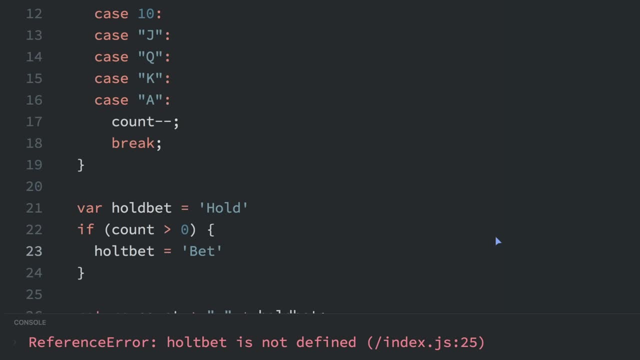 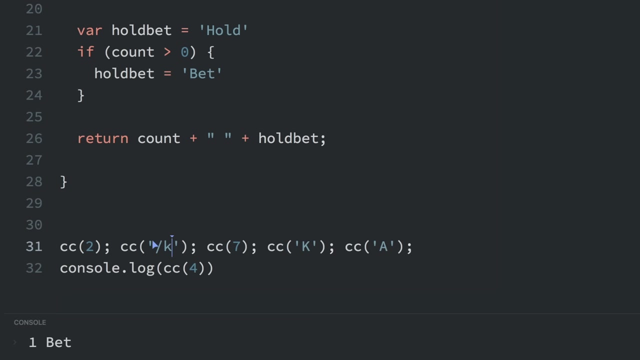 Hold. Oh, we spelled that wrong. So instead of Holt bet, that should be hold back. Okay, in this case we're going to bet, because we had a bunch of positive numbers and negative numbers, But if we change this to k, 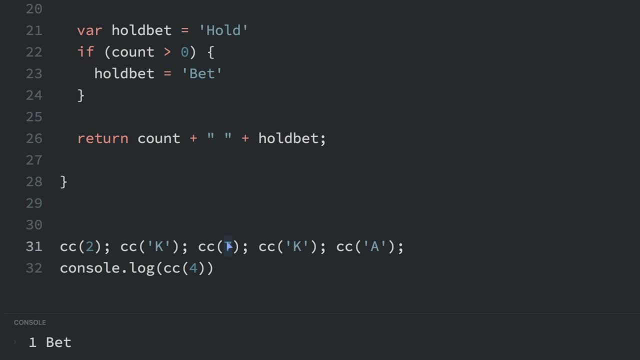 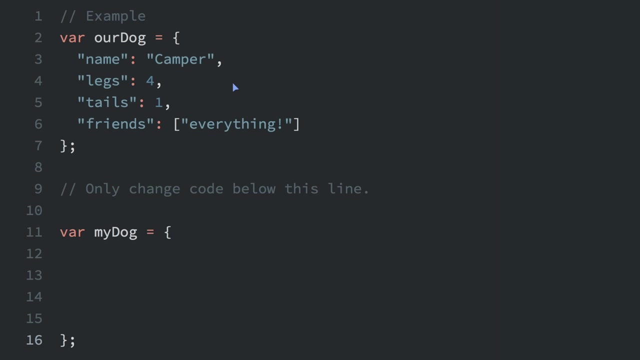 we change this to 10.. Let's see what happens Now. we're gonna hold: Okay, it worked, And I'm gonna tell a format: reduced value inside the same略. So this Let's go again to the subtibogeb. It is a let's make it treated as something we'll be talking about in a second. 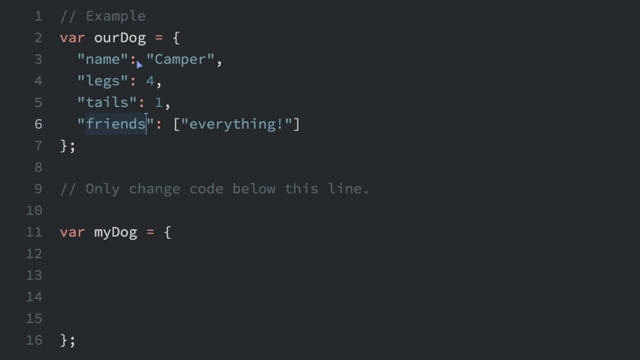 From the neighborhood. I'm going to just erase objects. objects are similar to arrays. the values are the things after the colons here. So the name is camper, the legs for tails. there's only one tail on this dog and friends are everything. Now you can see that with the 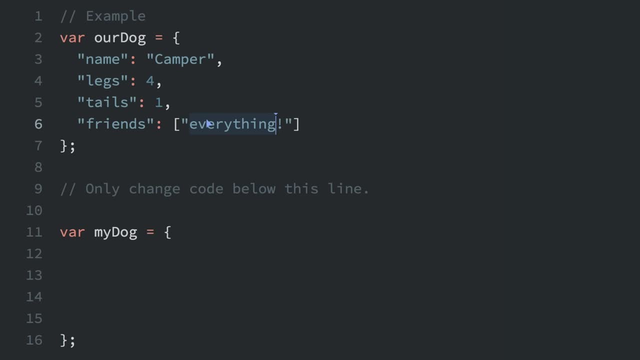 properties can be strings, they can be numbers, they can be arrays, they can be any data type in JavaScript. So now we are going to create our own dog, So this is going to have a name. Personally, I like the name Quincy, So we'll use that for our dog's name. Also, we're going to have 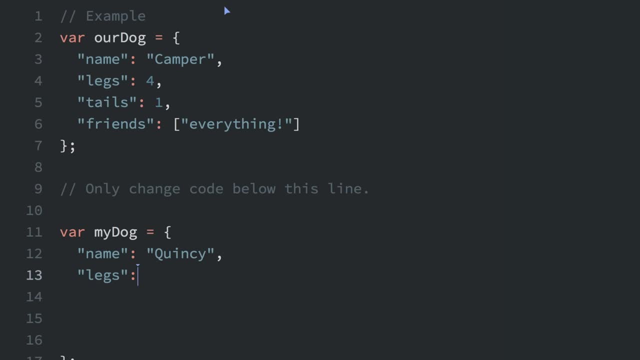 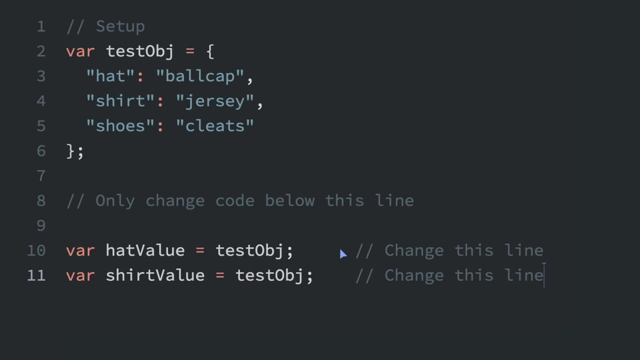 legs. Unfortunately, our dog has had an accident. he only has three legs. But to make up for the only having three legs, he does have two tails. And for friends- Another unfortunate thing- it's an empty array. He has no friends. Okay, we've now created our own object. There are two main ways to access a. 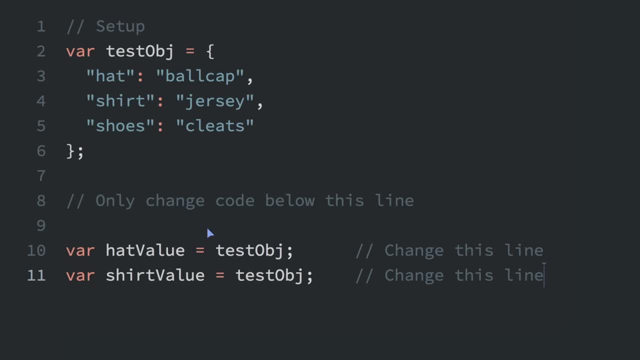 property on an object. The first I will talk about is dot notation. So we have this test object and we have hat, shirt and shoes And we want to find out the value of these properties. So right here, the hat value, we're going to set the test object. Now here's where we use the. 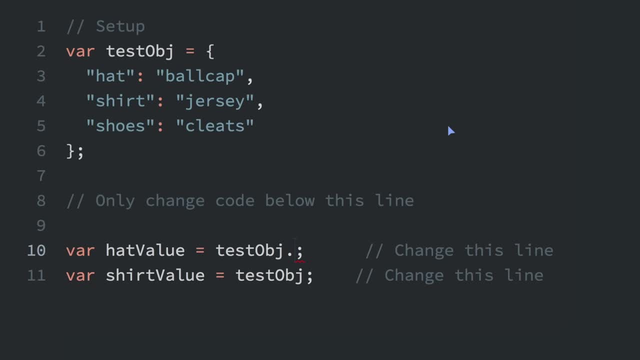 dot notation. we just put a dot or a period, And then I put the name of the property, dot hat, And then for the shirt value I will do dot shirt. So see this word right. here is just the word here. So the value of hat value test object: hat is now going to be ball cap- And the value of the 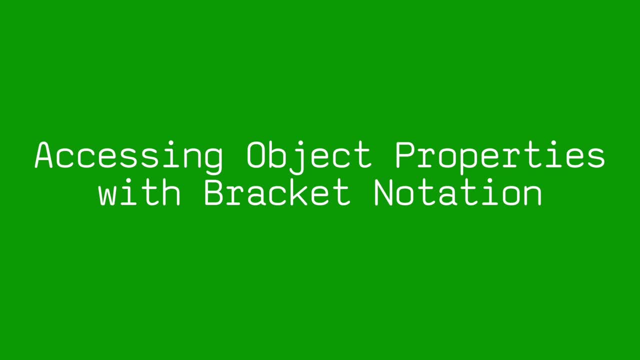 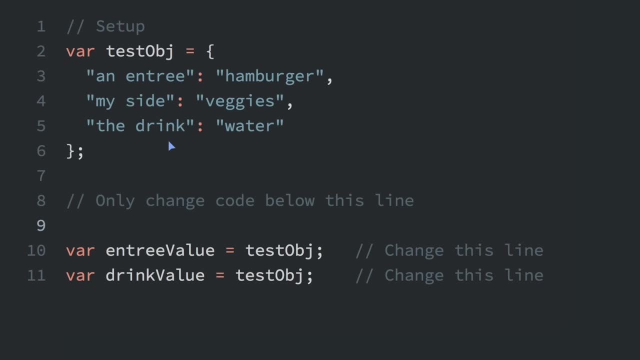 shirt, value is going to be Jersey. Besides using dot notation, you can also use dot shirt or shirt or shirt, And you can use bracket notation to access a property in an object. You can use bracket notation anytime, but it is required If the name has a space in it. 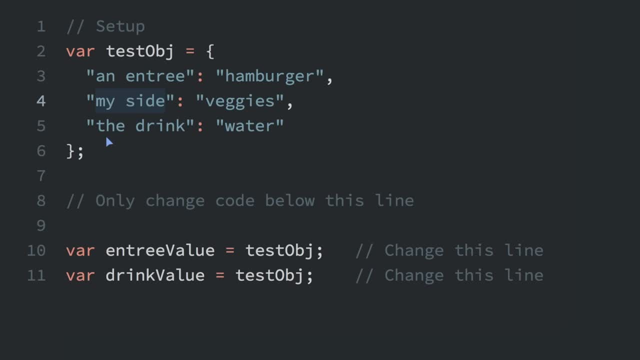 you can see, in this object we have three properties and each of them have a space. So to get the value of these properties we're going to have to use bracket notation. So the entree value we're going to test object, that's the name of the object, And then we're going to put brackets. 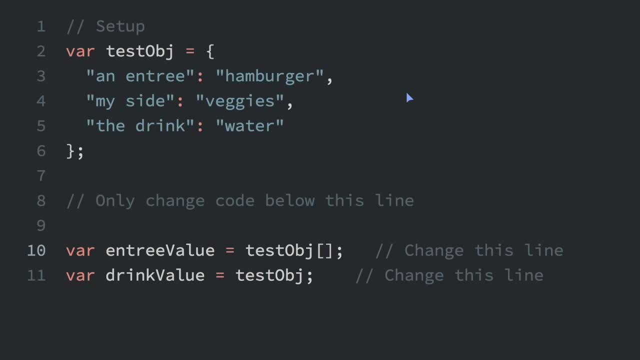 like an array index. So you need the opening and closing brackets And inside we will put the name of the property. So I'll do an entree And then we can do it again down here for the drink value, And I'll use a single quote this time instead of double quote to show that each of those will work. 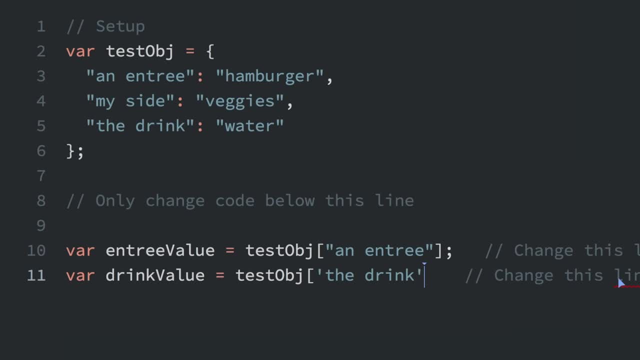 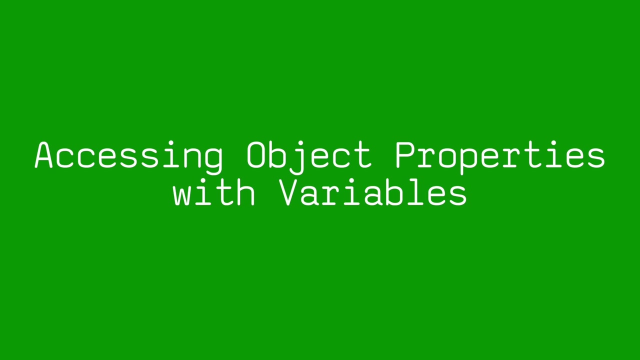 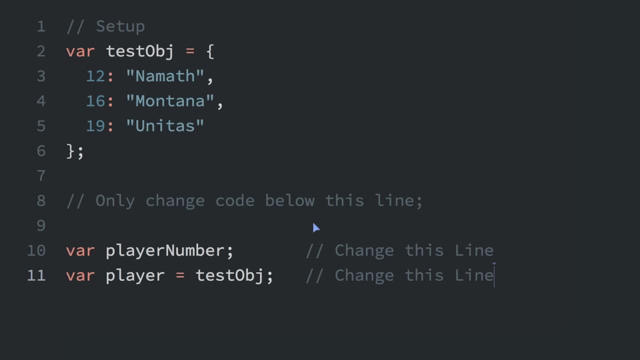 notation can also be used to look up object properties using variables. So here we have this test object, we have these different numbers associated with these names here, And we are going to set this variable to be one of the numbers. So I'll set this to be 16.. And then I'm going to 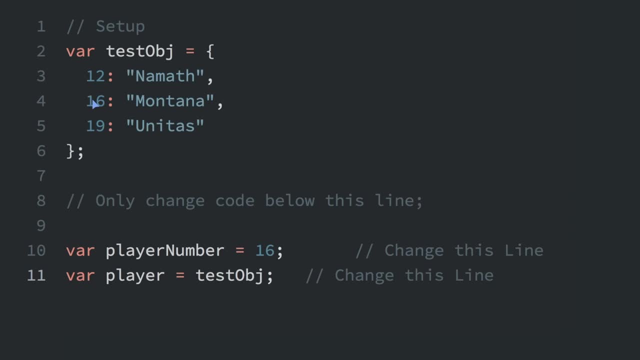 say that them, And then in the test object you can use the variable name instead of the number. So instead of putting 16, I'm going to put player number in. here And now, player is set to the word, the string Montana, And we use this variable to look up the object property. We can use dot notation. 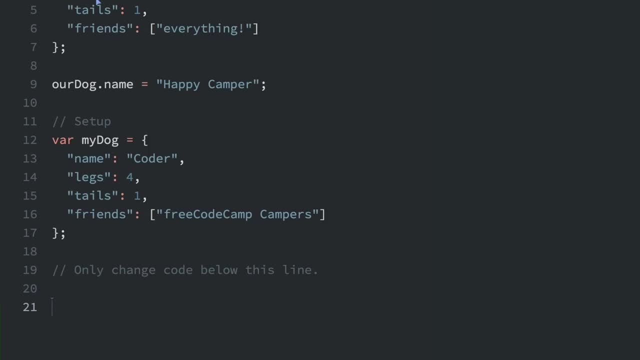 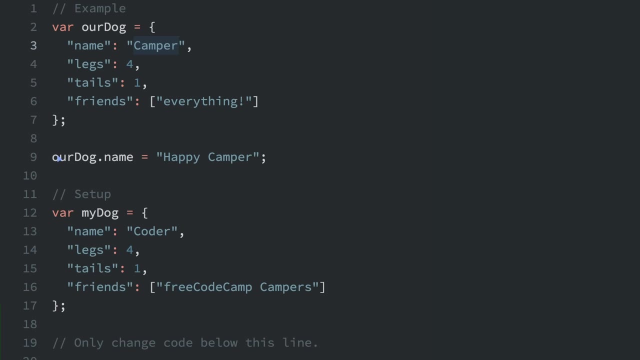 to update object properties. Here you can see an object called our dog. it has a name, legs, tails, friends and the name is camper. However, here we use dot notation, our dog dot name, and use the assignment operator, the equal sign, to set the name to happy camper. So if we did console 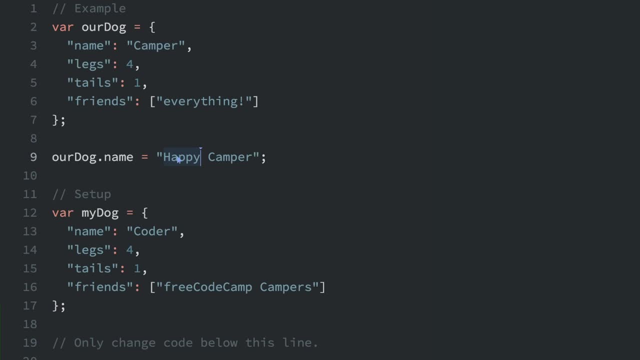 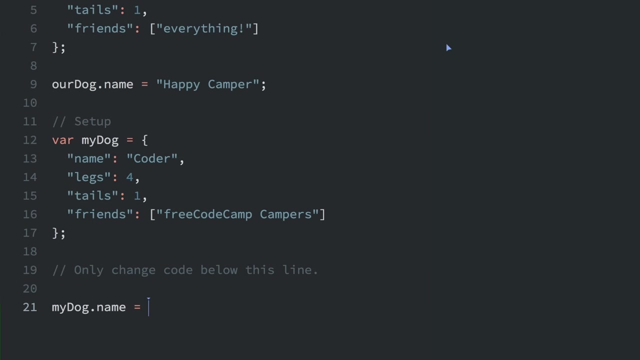 dot. log on our dog dot name. it would no longer be camper, it will be happy camper. Well, we have another dog here with a name of coder, but we want to change the name to happy coder, So that's what I'll do right here. So my dog dot name equals happy coder. So, just like above, we use dot. 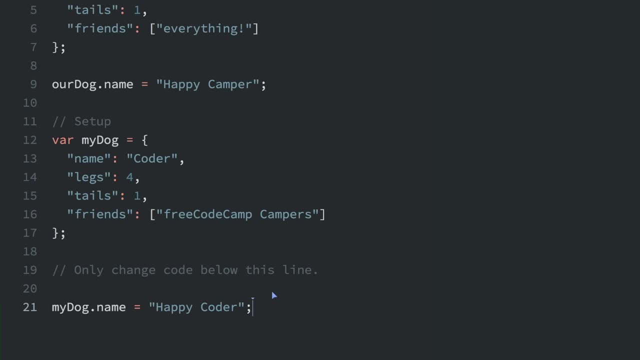 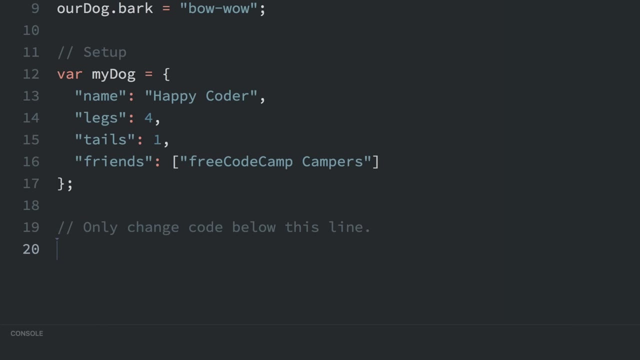 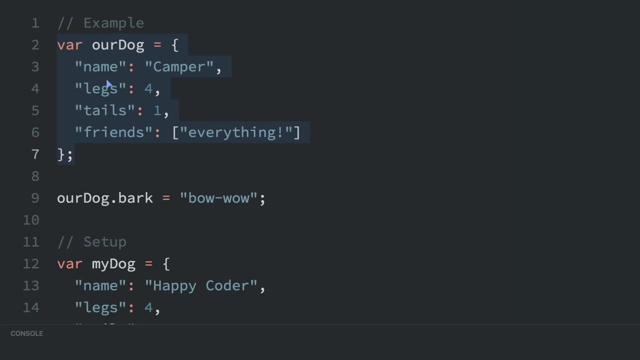 notation to set the object property to a new value. You can add new properties to an object using dot notation. So you can add properties to an object using dot notation. And also you can add properties or bracket notation. so here's an example: right here we have this object, our dog, and there's four. 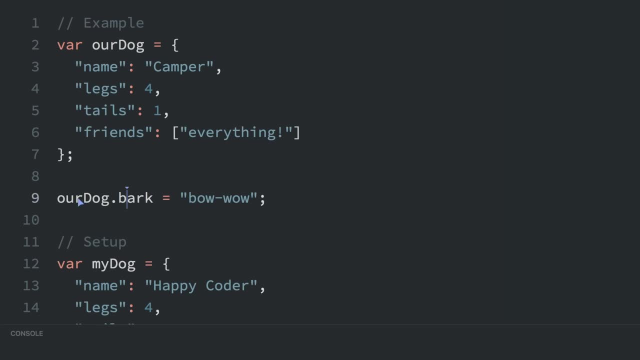 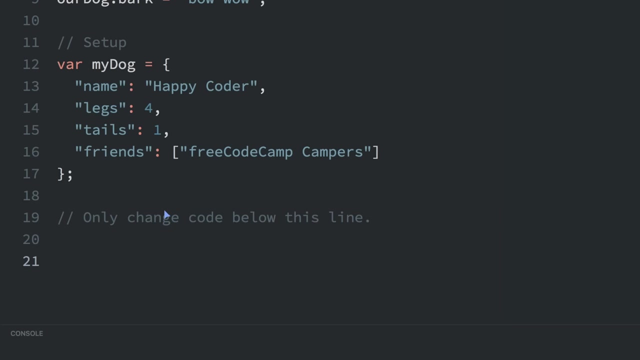 properties here, but down here we're adding a new property. our dog bark equals bow, wow. so it had four properties, but now it has five properties as the property bark as well. now down here we'll add a property to the my dog object, so we can do my dog. and then here I'm going to use bracket notation. 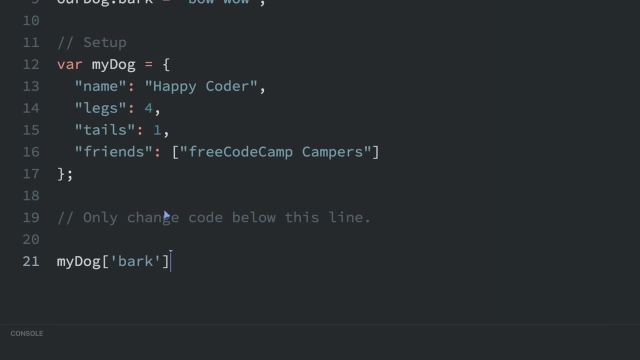 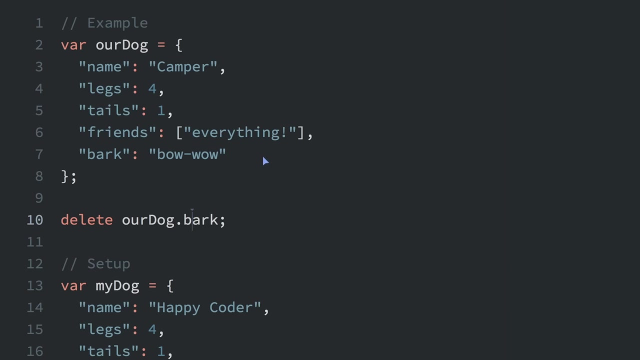 instead of dot notation bark. I'm going to set that to equal woof. and because he's yelling, it will have an exclamation point. and that's how you add properties to objects. it's simple to delete a property from an object. our, our dog object has all these properties and with the 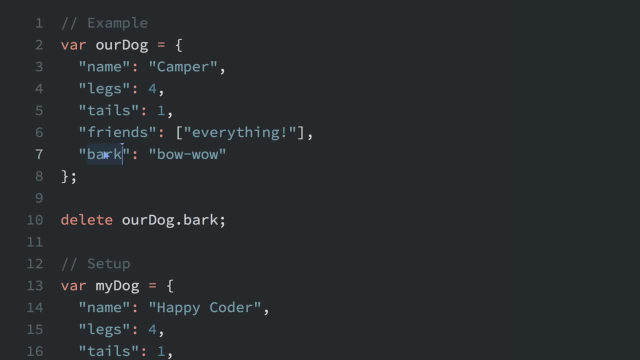 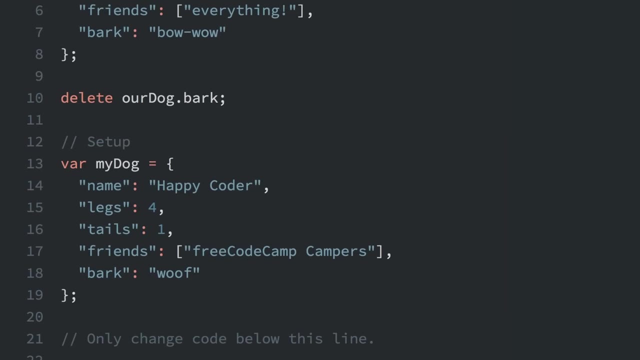 delete. keyword: delete our dog bark. so now this property here, the bark- has been deleted and it's going to be a property that we're going to add to our object. so we're going to add a property that is no longer in the object after we've deleted it, so we can do the same thing down. 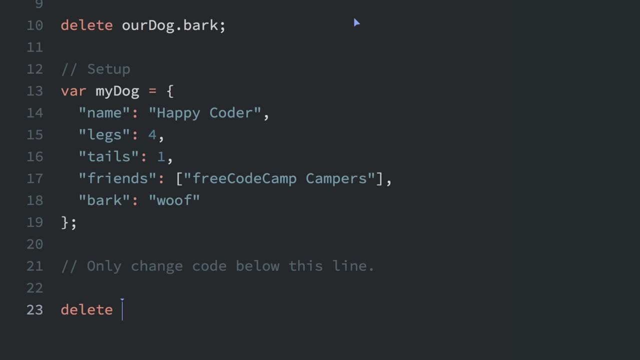 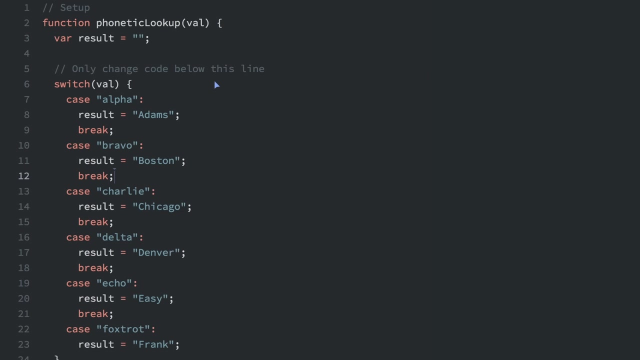 here, and this time we will delete the tails property my dog tails. so now the my dog object no longer has a tails property. objects can be thought of as a key value storage like a dictionary: you can use an object to look up values. so in this case we have a switch. 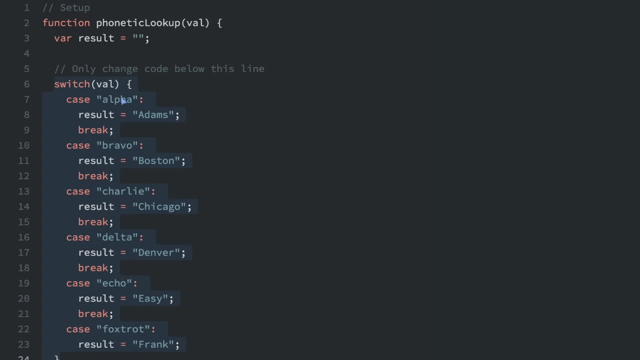 statement that returns certain values. so when you pass an alpha to the function, it returns Adams. if you were to pass in Bravo, it returns Boston. we can replace this switch statement with an object and use the object for lookups instead of the switch statement. let me show you how that's done. 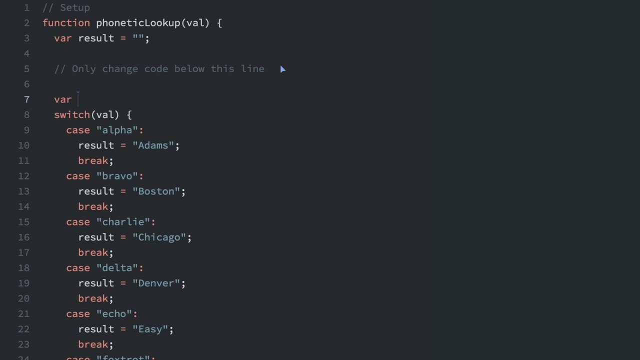 I'm going to create our look up. this is going to be an object here and the object is going to have a bunch of key value pairs. so if I two these objects and one of these objects and one of these objects, I'm going to add a formula here and when I add a new variable to this variable, 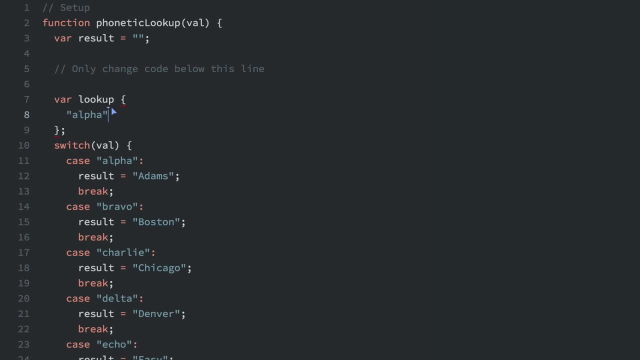 So we have alpha and that's going to be Adams. And then we have Bravo And the value for Bravo is going to be Boston, And that's it. So we can now delete this whole switch statement And now we can say: result equals. look up in bracket notation we put the value that was passed in. 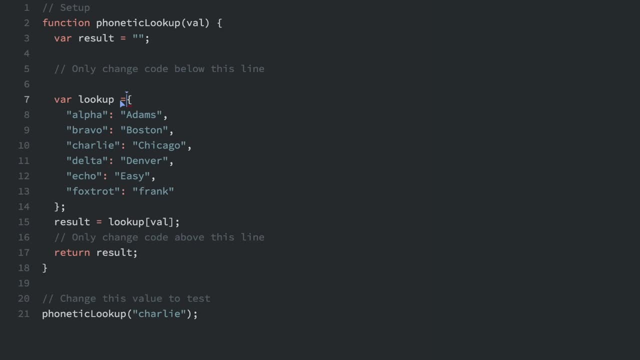 then I forgot one thing, which was the equal sign here, because look up equals this object And let's do a test. So let me put console dot log So we can actually see what happens here. So if we do, Charlie, we're going to get Chicago And 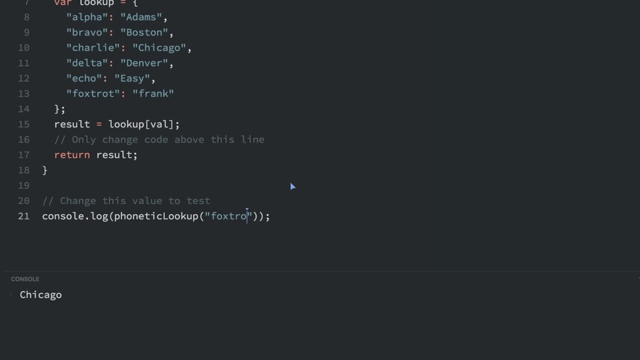 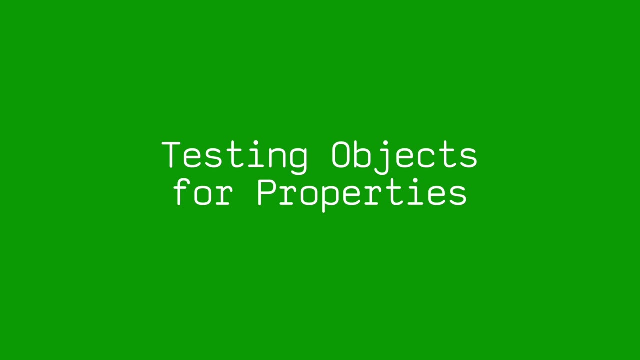 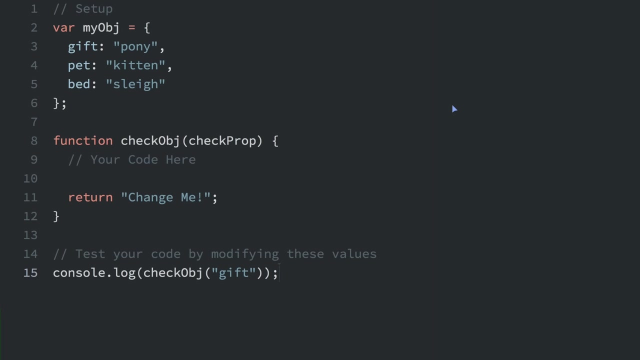 if we do foxtrot, the result will be Frank, So it works. You can check if an object has a property with the has own property method. Let me show you how to use this method and finish making this function, where we check if an object has a specific property. If it doesn't have, the property will. 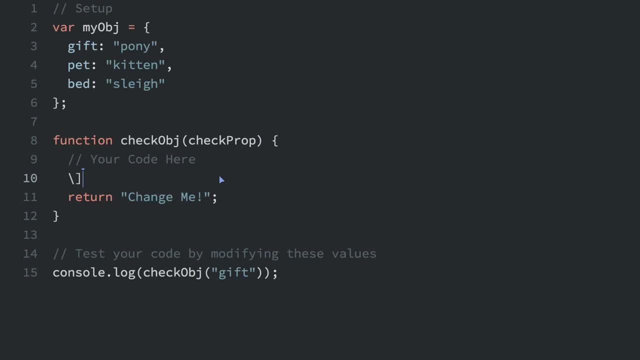 return not found. So let me show you how that's going to work. We'll do my obj, that's, the object up above dot has own property, And then we pass in the property we're going to check which is check prop. this is either: 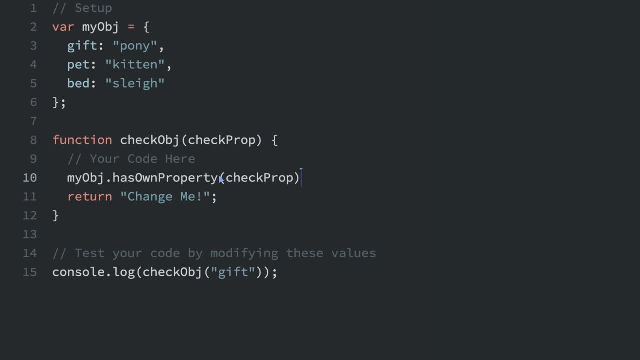 going to come back as true or false if it has the property. So let's make this into an if statement. if my, my object has own property check prop. But if that's true we're going to return my obj And then use bracket notation check prop. So we're going to return the value of that. 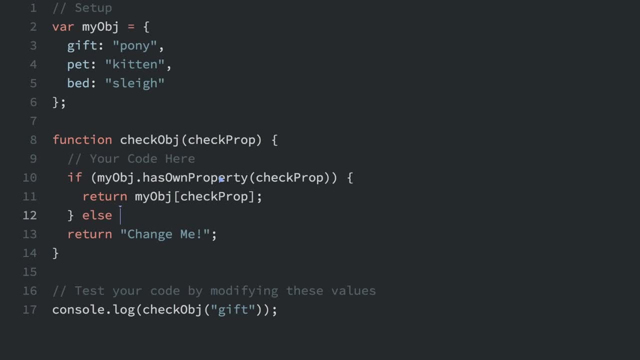 property Else, we're going to return not found. So let's take off this other return statement And I'll do a test. So when we pass in gift here, we returned Pony, but let's say we passed in hello, Hello, that not. 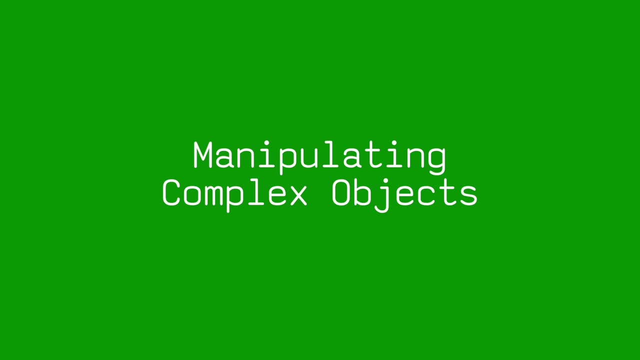 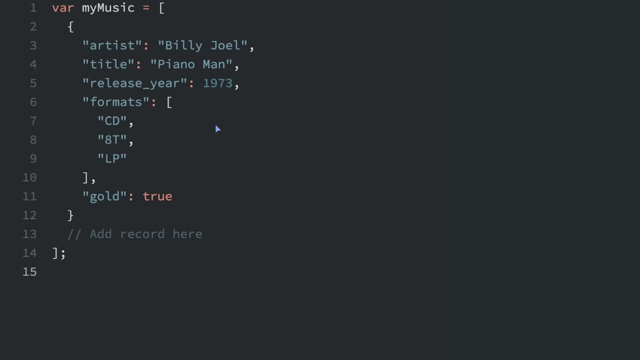 found. Okay, it works. A JavaScript object is a way to store flexible data So you can store strings, numbers and arrays and even other objects. So in this example we have a string and a number And then we type in xj, And then we press enter And now we action the. 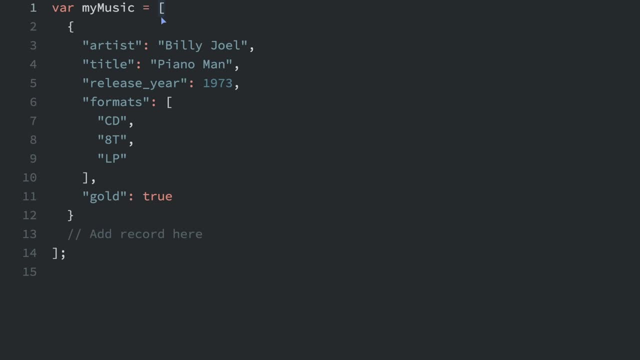 have an array called my music. we can see it's an array because we have the open bracket and close bracket, But inside the array are objects. So this is one of the objects, And inside the objects are all these key value pairs with the strings and the numbers and so on. So I'm going. 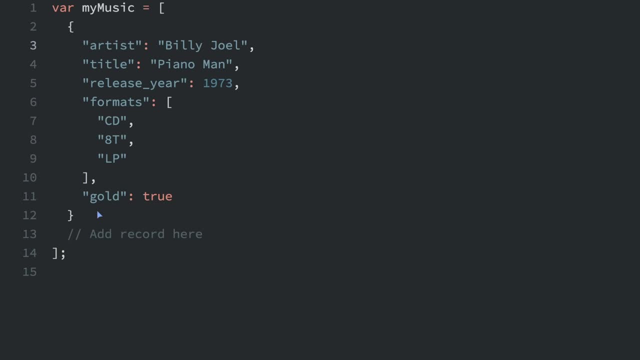 to add another object. So, since this is array, after each element in an array you have to have a comma. So I'm going to add a comma here And then I'm going to add my next record right below this comment here And we are going to have, just like well above, we're going to have an artist. 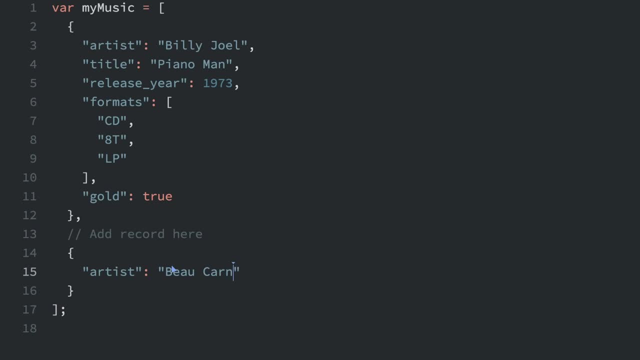 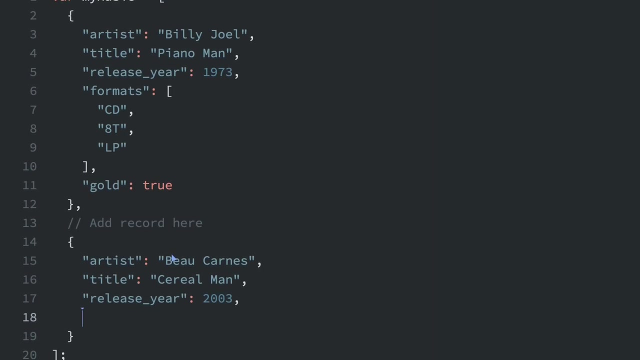 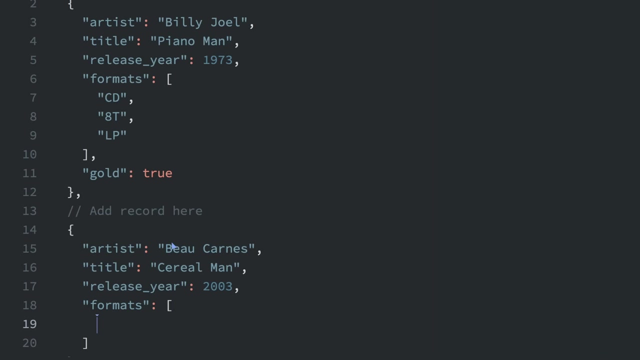 the artist is going to be Bo Carnes, And then we have a title. The title will be serial man, The release year will be 2003.. And for a formats, this is going to be an array, just like above, so we can have any format I'm gonna put. 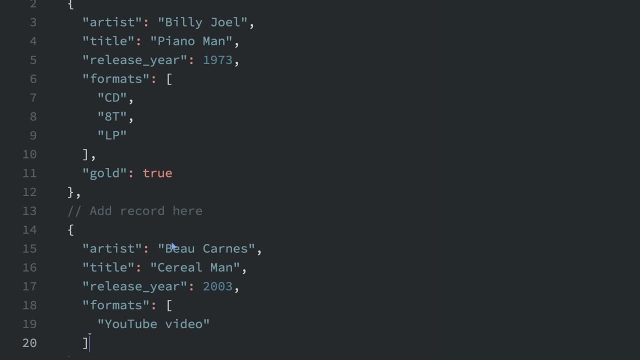 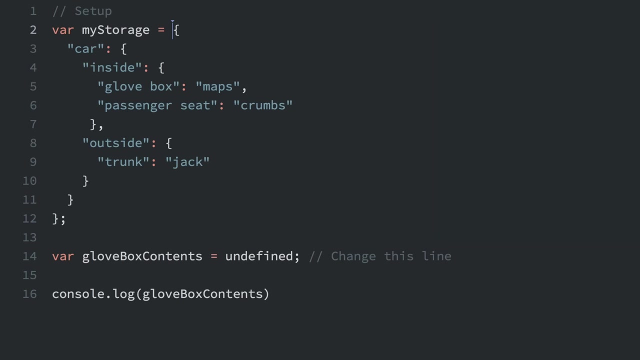 YouTube video. And now we've created a second object in our, in our my music array, And each objects hold data in a property, which is the key value format. This is very similar to JSON, which we will talk more about later. Here we have an object with other objects nested inside that. 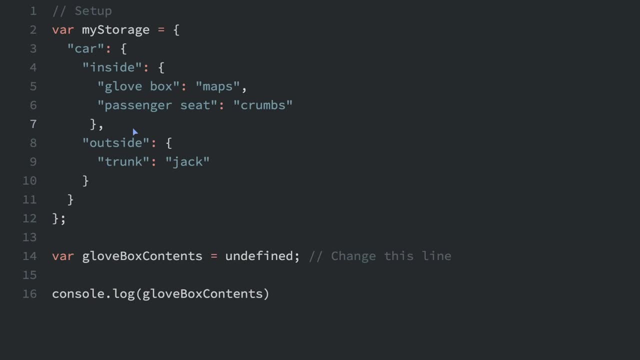 So in order to access sub properties of an object, you can chain together the dot or bracket notation. So I'm trying to get the glove box contents. So I'm going to take away this undefined here And I'll do my storage dot, car dot inside, And then I'm going to add a new object And I'm 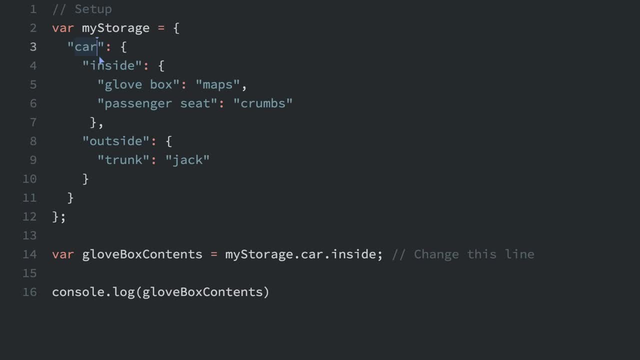 going to add a new object And then now the next thing it's a car inside, the last thing is glove box. Because there's a space here, we have to use bracket notation. So I'm going to use bracket notation on the end here and say glove box. And now if we run this, see, we are going to console. 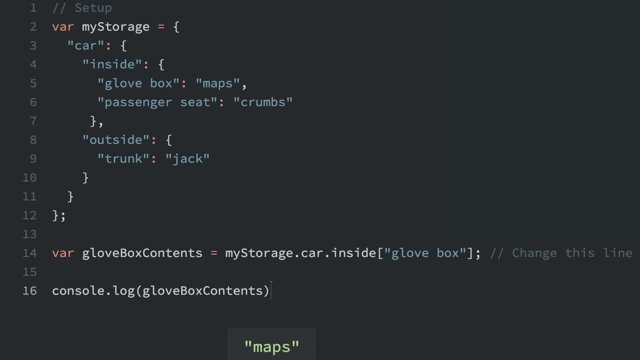 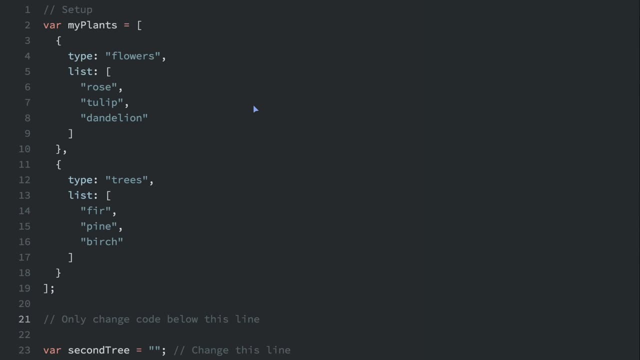 dot log. So let's see if we get the contents here. Yep maps: it worked. Array box Bracket notation can be changed to access nested arrays. you can see we have this array here And inside this array are two objects. The first element in the array is this object, the second 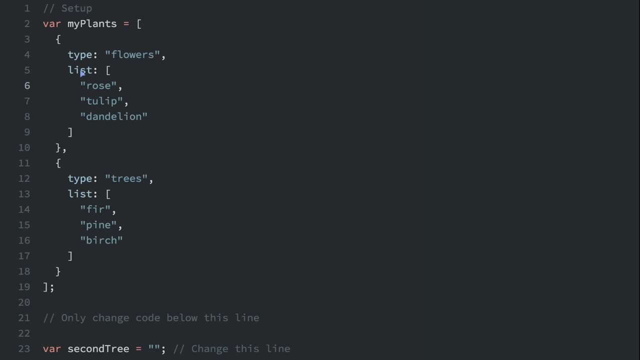 element in the array is this object And then inside the object we have a key value pair. the key is less than the value is another array here. So we can combine that notation and Brett bracket notation to access the second tree. That's what we're trying to do here. So 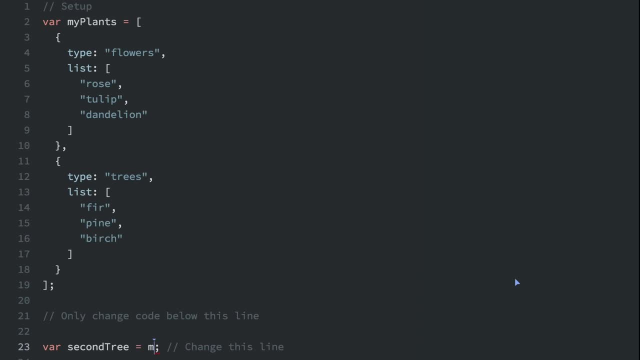 let's do that. First we need to do my plants, And the trees are the second element in the my plants array, which is index one. now we need to get the list, So the list of trees here. so I'm going to do 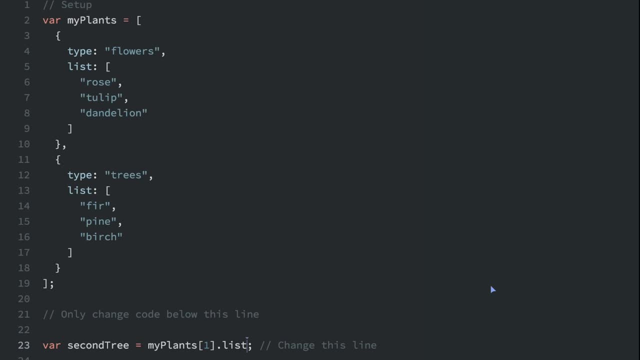 dot list And since that list is an array, I can use the bracket notation to get the second list element, which again is array index one. So if we run this it's going to console that log and we see pine. that's the second tree here. 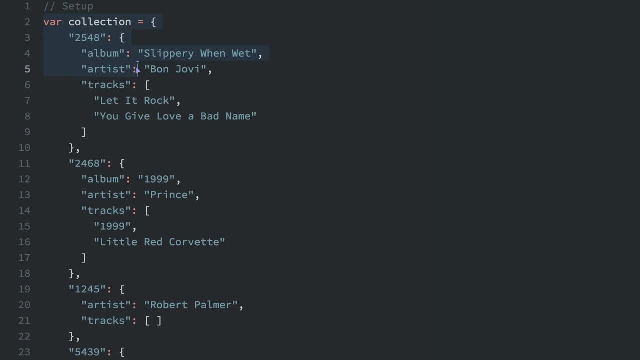 This is a coding challenge we're going to do. We're giving, given this object here, which is a record collection. Each record has an ID And then it also has different pieces of information about the record. They don't all have the same information, But see, we have our album. 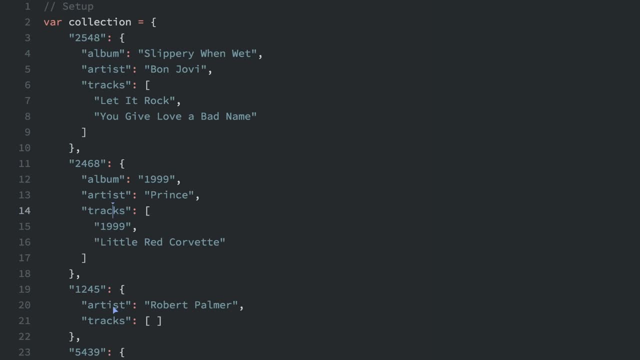 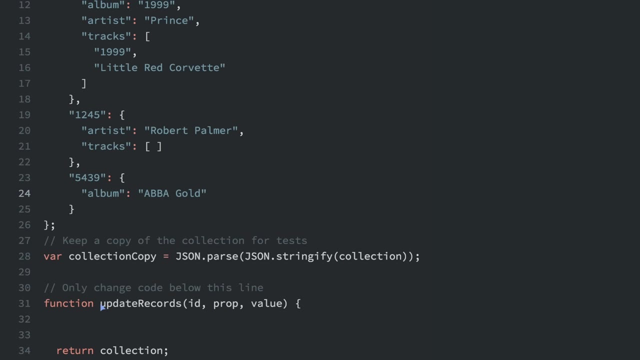 artist tracks: album artist tracks. this just says artist tracks and this just has album here. And we are supposed to create this update records function where we can pass in the ID, the property and the value, And it's going to update our record collection with the property and the value, So for 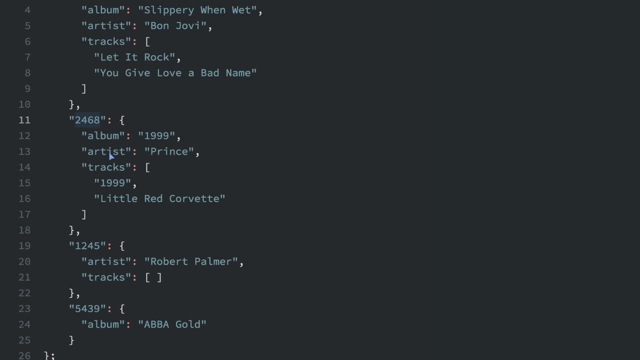 instance, if we pass in the ID 2468, and we put the property artists and if we set a different value, like Quincy or something like that, then we should update this whole object, So now it says Quincy instead of Prince. 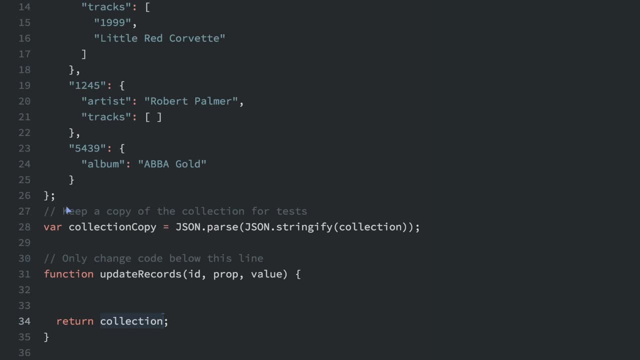 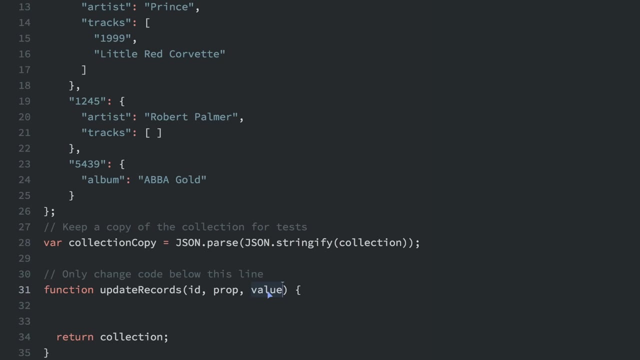 and we should return the full collection. So it's going to update the collection and then return the collection. If we have an empty string for the value, it should just completely delete that property. Also, if we have the property of tracks and then we have a value, instead of updating the whole tracks, 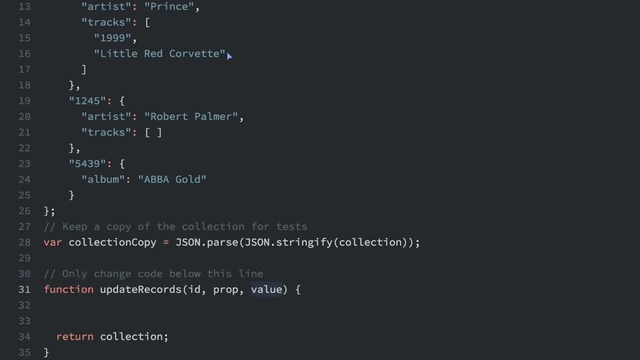 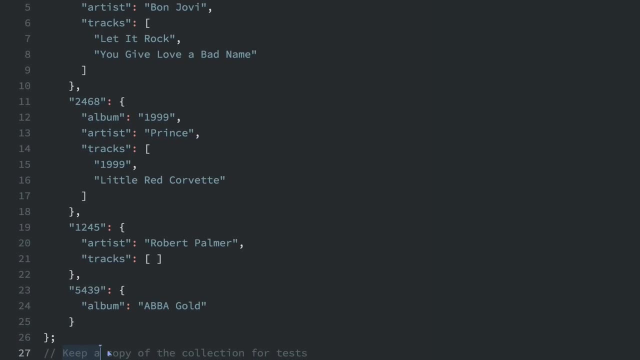 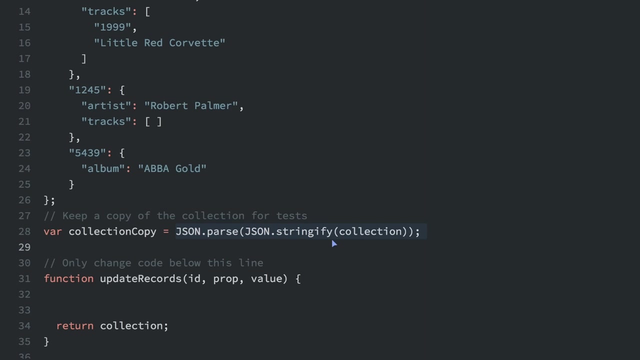 here with what we put in. it's just going to add the track to the end of this array. So if you look right here it says: the comment says: keep a copy of the collection for tests. this: JSON dot parse and JSON dot stringify And then collection. This is just a fancy way in job. 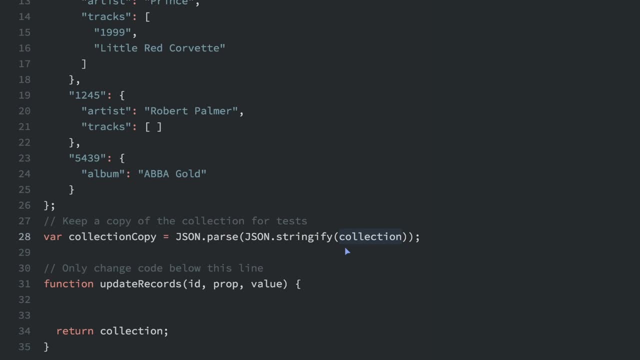 JavaScript to make a copy of the object. Remember, in our function we are going to be changing the collection object, but we want to have a copy of the original object before anything was changed. So that's what that's for. So let's go ahead and do that. So we were just updating this function here. 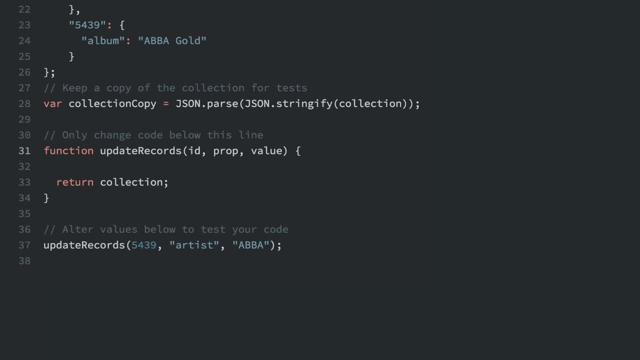 this update records function. Okay, so let's get to this. So we'll do. if value equals equals equals blank. because the first condition we are going to test for is if we need to delete the property. remember, if the value is set to blank, we delete that property. So if the 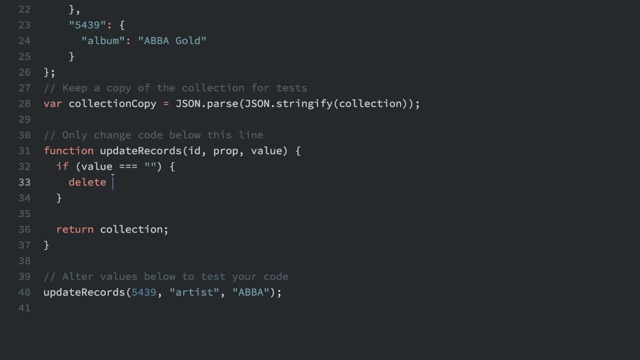 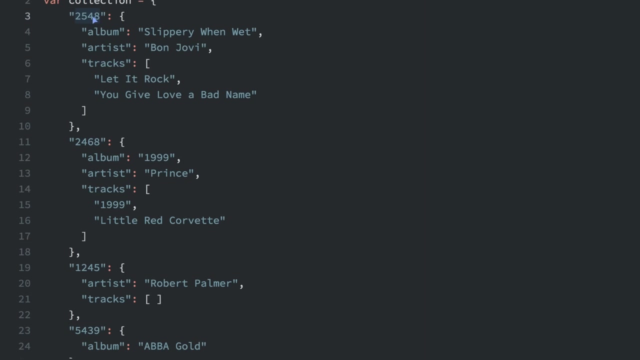 value is blank, we are going to delete collection And then we have to use bracket notation ID and then prop the collection ID. prop That's the collection here if we pass an ID 1248.. And then we go to there- the property. if we pass an album for the property, we'll go to here And then we'll. 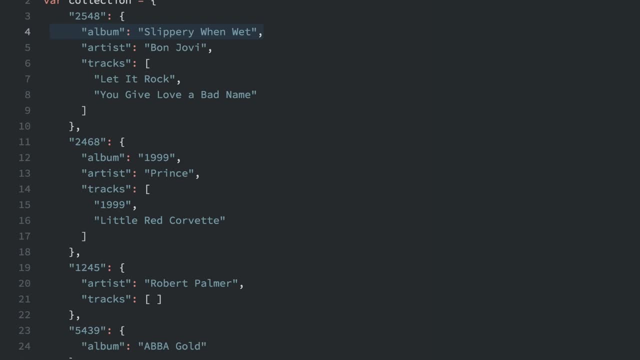 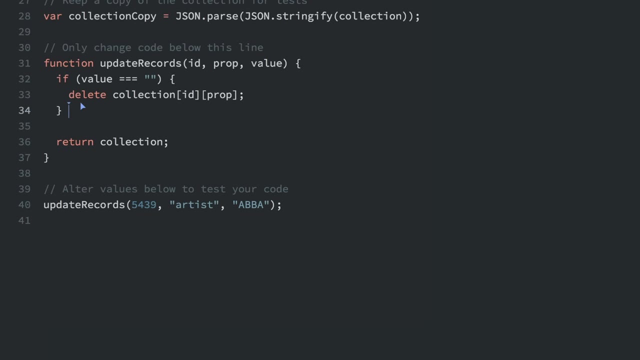 just delete that whole thing. If our values in the empty string Okay. the next condition we have to look for is if the property is tracks, because for most properties we're just going to override that property with the value passed into the function. But if the property is tracks we are going to 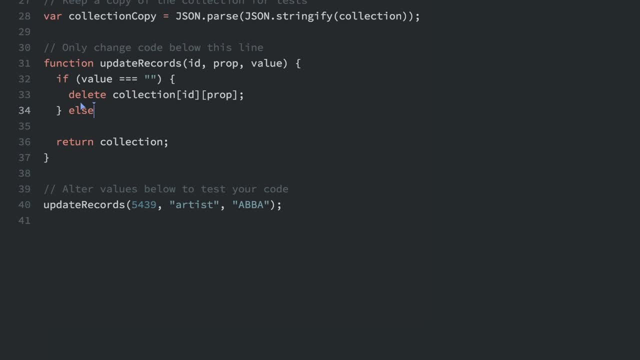 push on to the end of the array. So let's do an else. if else, if prop equals equals equals tracks, then we just have to push on to the end of the array. So there's also another condition here, which is if the tracks property is empty. if the tracks property is empty, 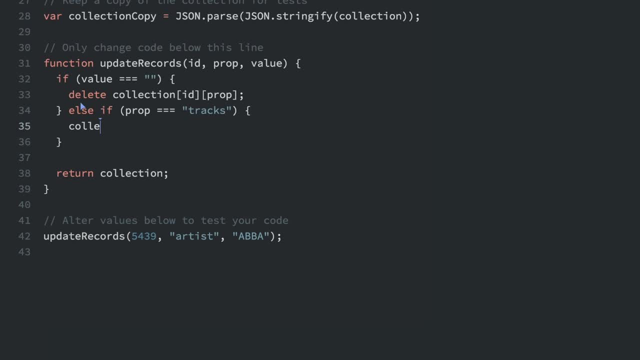 we need to create it. Here's a fancy way to do that: collection ID props. So if prop equals tracks, we are going to set the tracks, because mirror prop is going to equal tracks. we're going to set the tracks to equal. it's going to either equal itself. 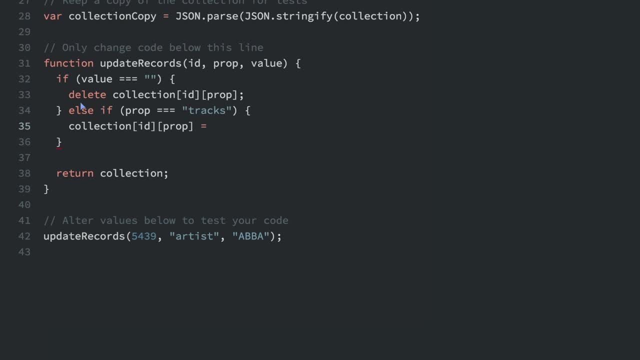 if it exists or if it doesn't exist, we're going to create it. I'll show you how: collection ID prop: it's going to equal itself, Or that's the or operator: it's going to equal an empty array. So if this already exists, we're going to set to equal. 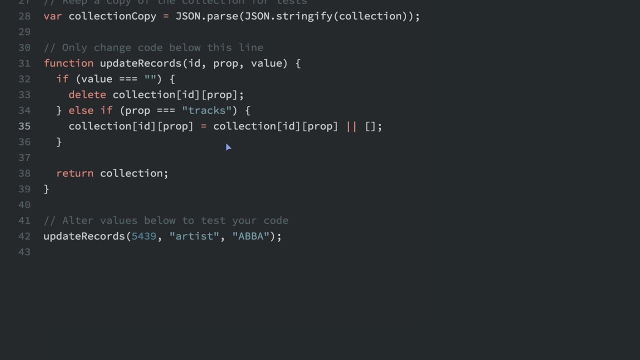 itself. But if itself doesn't exist, we'll just set it to equal an empty array. So that's just a way to create that property if it doesn't already exist. So now that we know it exists, we can just push the value to the end of the array. collection ID. 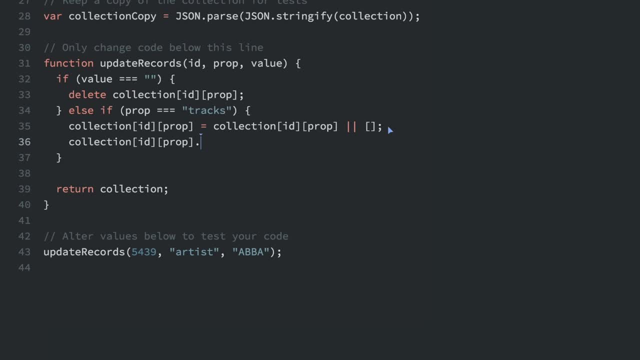 prop And we'll just do the dot push And then put in the parentheses the value, So we're able to push the value that was passed into this function on to the end of the array. Okay, there's only one last condition, which is the just the kind of the default condition, else So 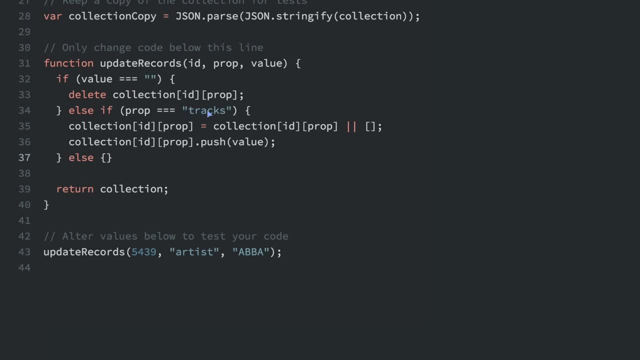 if the value isn't blank and the property isn't tracks, then we just push the value on to the property. then we just set the property to equal the value, just like this: collection ID prop equals value. Okay, let's test this out. So we already have. 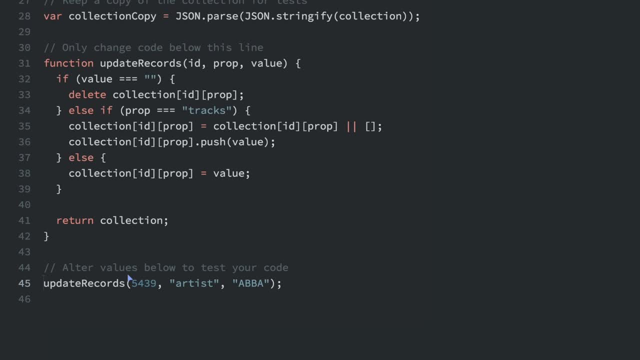 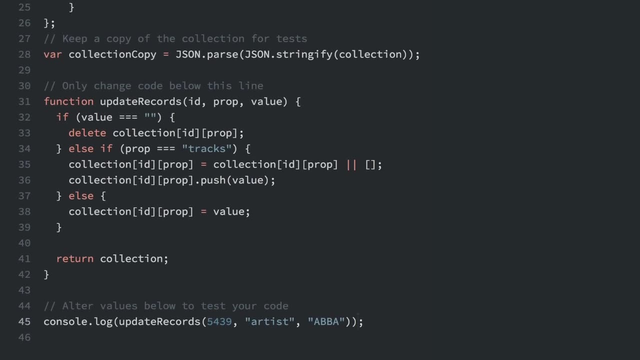 this example down here, But to see if it actually worked, we're going to do a console dot log So we can see the output there. And if I run that, I'll let me open up the console so you can really see it. So let's. 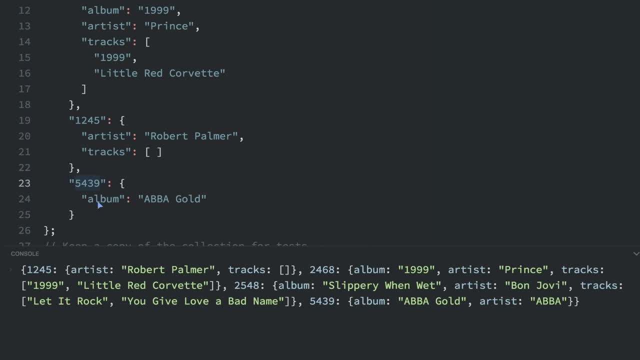 see what we change: go to 5439. And we set the artist, which didn't previously exist, to ABBA. So let's look down here in the console 5439. And the artist is ABBA. Let's see what happens when we add. 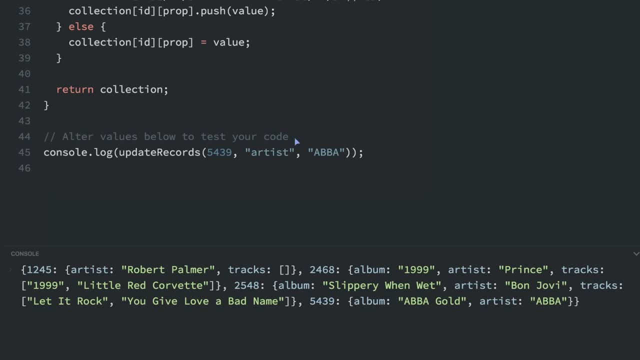 a track. So we'll do one more example here. I'll just put it right above here: Eight records and I'm going to pass in something I'll pass in. let's see the ID 2468.. And we'll pass. 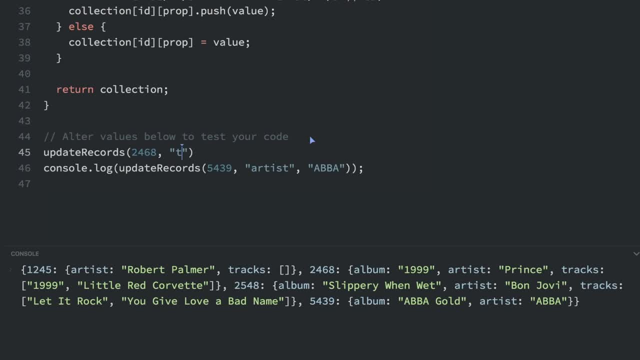 in the key, which is going to be tracks, And then for the value we'll put test. So let's see what happens here. If we want to add a track, we're going to do a test. So let's see what happens here. If we 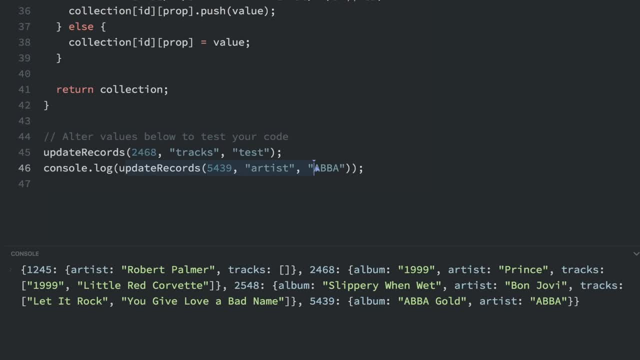 run that it's going to update the record here And that's gonna update the record again. But we don't care about that one. we mainly care that's going to console dot log what the final value is. So if we look at 2468, here 2468, let's see the tracks. we at 1999, little red Corvette and test. 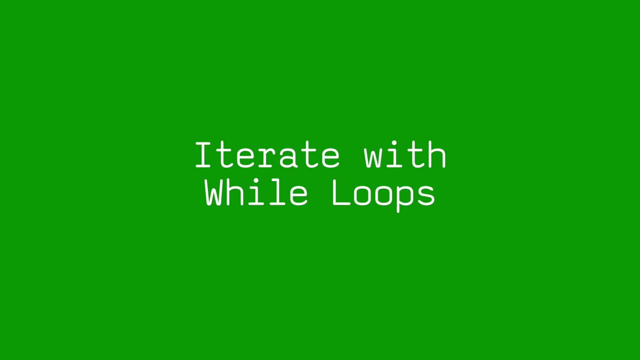 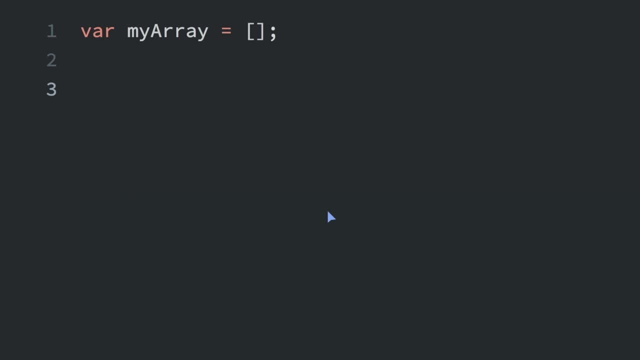 So it's working great. Loops allow you to run the same code multiple times. I'm going to talk to you about a while loop that runs while a specified condition is true and stops once it's no longer true. So we are going to push the digits zero through four onto this array. 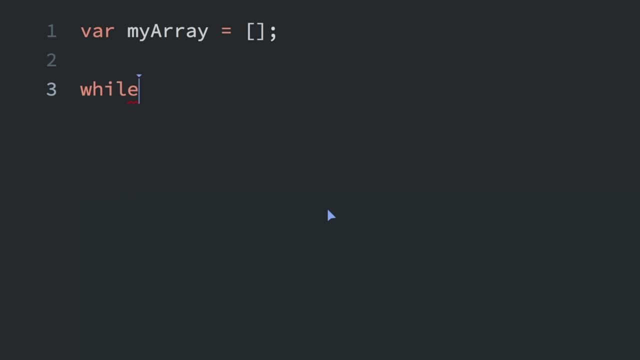 Here's how it's gonna work. While is the while loop, while I is less than five, And we're going to do something. while that's true. First we have to set what I starts off at. So var I equals. 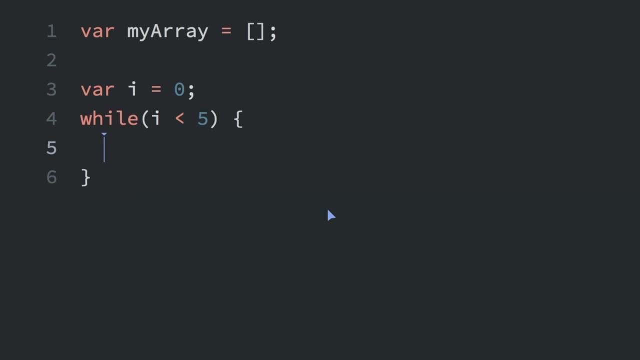 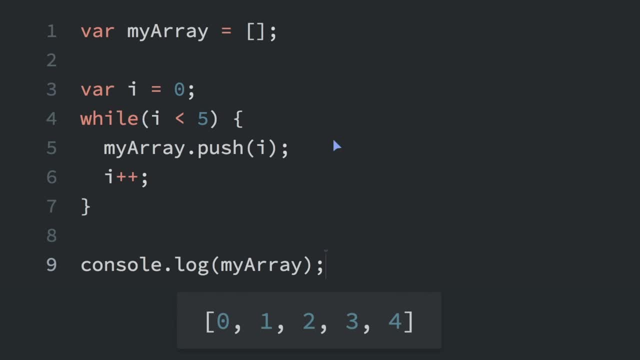 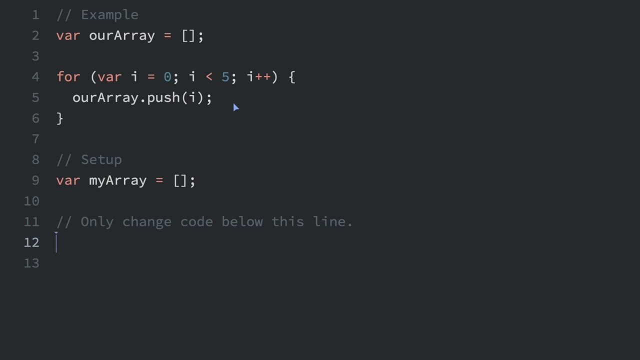 to console 01234.. The while loop worked it every time, went through this five different times and push 01234 onto the loop. A for loop is the most common type of loop in JavaScript, So here is an example of a for loop. you start with the keyword for and then we have these parentheses with three. 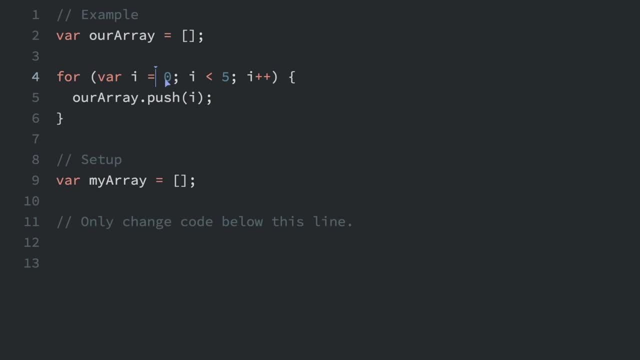 different items in there, separated by semicolon. The first thing is the initialization. then we have the condition, then we have the final expression. So the initialization happens before any of the code inside the loop runs. So we will start by initializing. i equals zero, So this is what most for loops start with, is you have a? 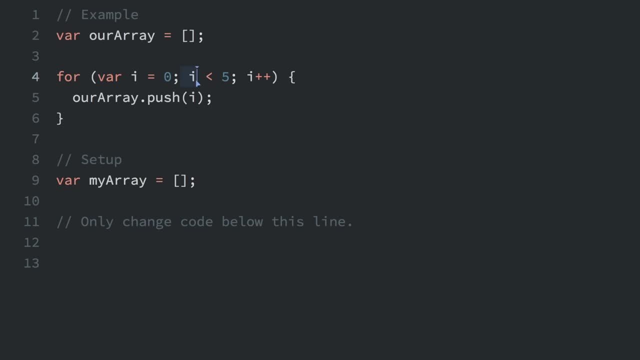 variable that you're going to initialize for the for loop. then the next thing is the condition. So once this evaluates to false, we break out of the loop. So while i is less than five will continue to run through the loop over and over. until this is false, then we break out of the. 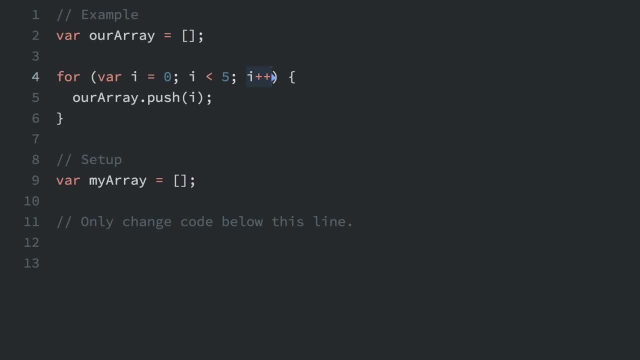 loop. The final thing is what we do at the end of each iteration. At the end of each iteration, we will increment i by one and this example we are filling our array with the numbers zero through four. I'm going to do another example where we fill an array with the number i equals zero. 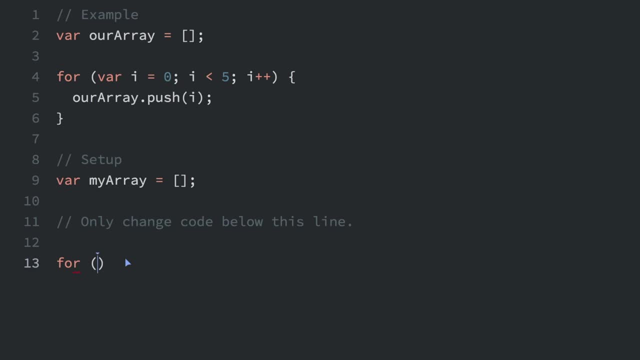 one through five. So we'll start with four. Now. we're going to initialize i to equal one. we're starting with one instead of zero this time And we're going to do: i is less than six. So, while i is less than six, or until i is more than six, we are going to run all the code in this loop And 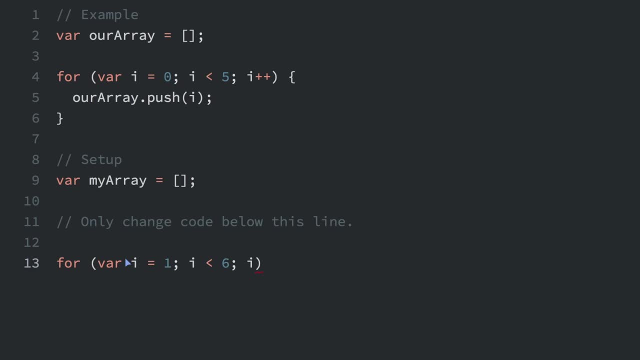 at the end of each iteration we are going to increment i. Now I can just do what we have before my array dot push i. So the final thing we will do is test this. I will do console dot log and put my array inside here And I'll just load this and see what we see in the console 12345.. It. 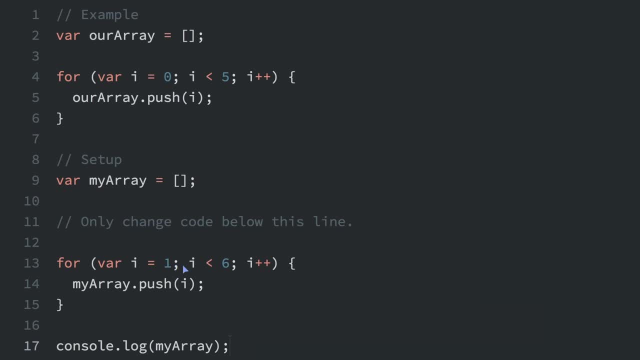 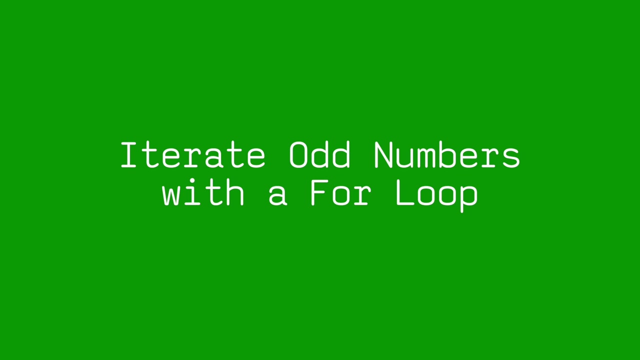 worked. we iterated five different times, And each time we pushed a new digit onto the array, And at the end of each iteration we incremented I, so it pushed a larger number onto the array. Loops don't just have to increment one at a time. 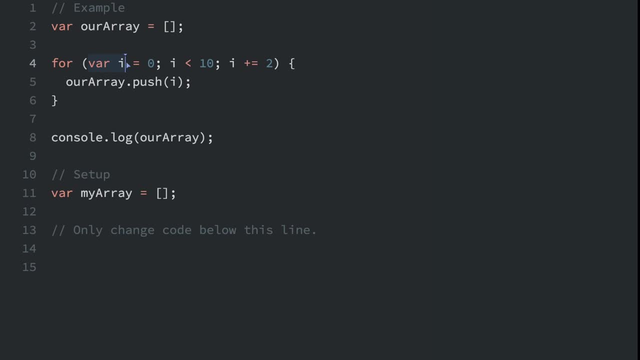 Look at this for loop. here we have our initialization, where we initialize i to zero, and then we are going to run the loop until i is less than 10.. And finally, their increment: instead of incrementing i by one, we're incrementing i by two. So now this: 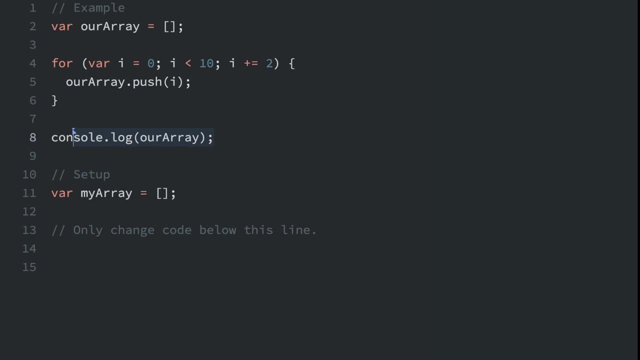 is going to push all the even numbers onto the array. We have consolelog, So let's log it out and see what it looks like: Zero, two, four, six, eight. I'm going to write another loop right now that creates an array of odd numbers, So let's do that. for var i equals one, we'll start at one. 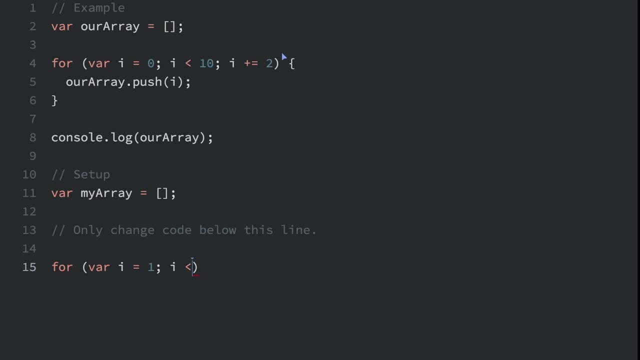 While I is less than 10, I can use 10.. Again, I'm going to do i plus equal two. So we're still going to skip count by twos, But since we're starting at one instead of zero, this should give us the odd. 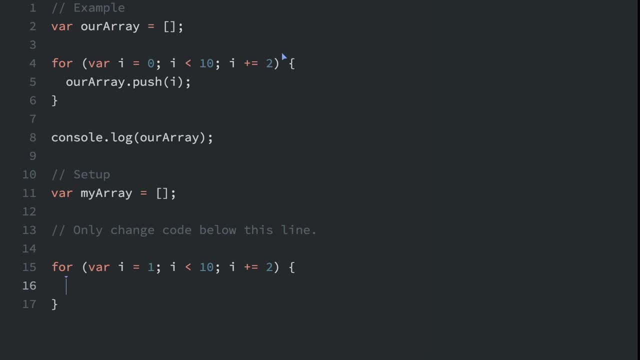 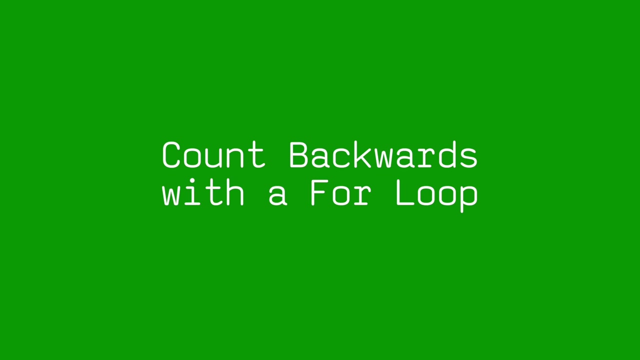 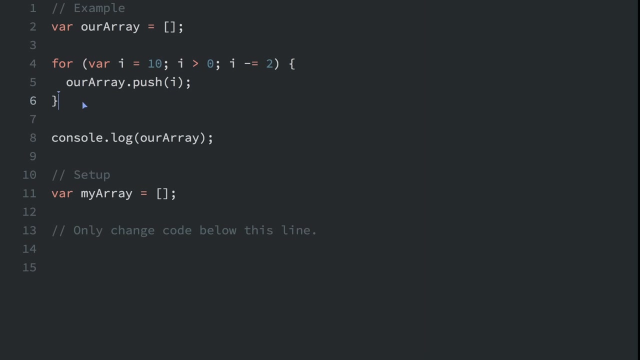 numbers. So let's see what's going to be inside our loop. my array, dot push And I'll just put either. So let's log this out and see if we did it right. console dot log my array And I'll run that. 13579.. It worked. A for loop can also be used to count backwards. So if we see this for loop, 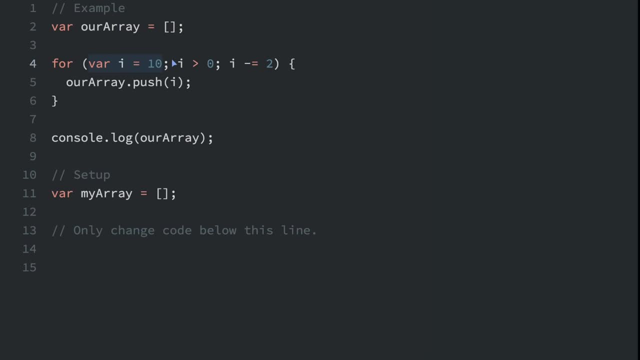 here we're initializing I to 10,, we're starting at 10. And we're going back to zero, And we're So we're going to iterate through this loop. while I is more than zero, we're going to keep iterating And at the end of each iteration, we're going to decrement I instead of increment it. 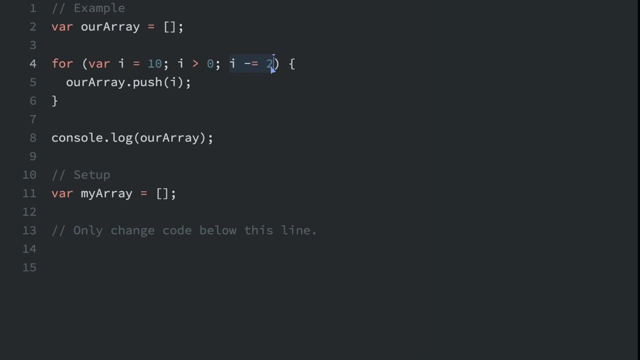 we're going to go down by two. I minus equals two means I equals I minus two. So we're going to continue pushing the lower and lower numbers on to the array until I is less than zero. So let's log this out and see what our array becomes. can see 108642.. Well, I'm going to write another one. 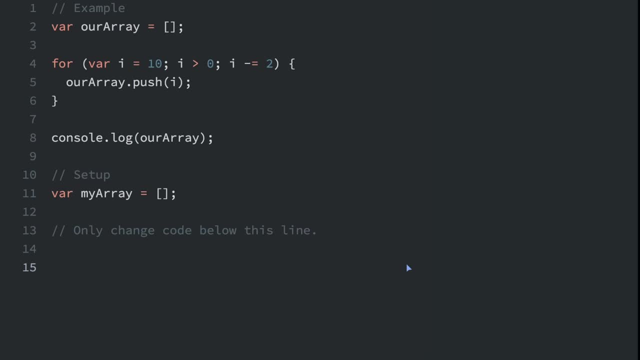 where we're going to push the odd numbers from nine through one to my, to the my array. So another for loop, and I'm going to do var i equals nine because we want to start at nine Now, we'll still do- is more than zero. So while I is more than zero, we're going to keep going through this array And 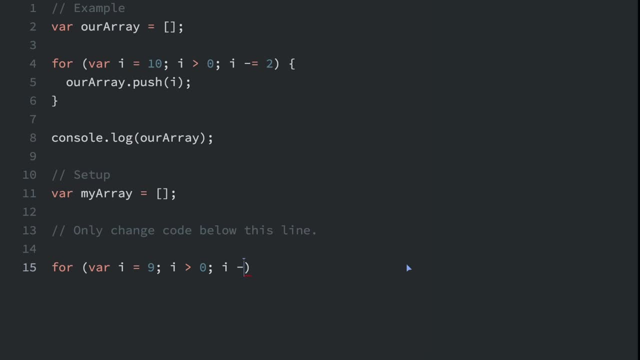 we'll do I and we, just. everything else is really the same. minus equals two And this is going to get all the odd numbers on to the array. So we just have to do my array, that push and then push on the I there. I'll just console that log So we can see what it ended up as my array And I'll run the. 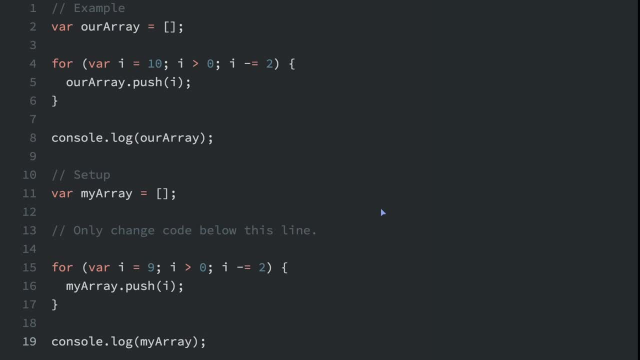 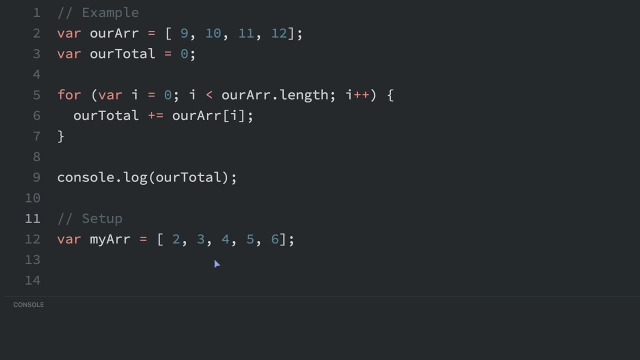 code 97531.. We did it. It is common in JavaScript to iterate through the contents of an array. So look at this example. we have this array here. before we were always adding items to the array, But this time the array already exists right here: our array 910 1112.. So we are going to start at zero. But now. 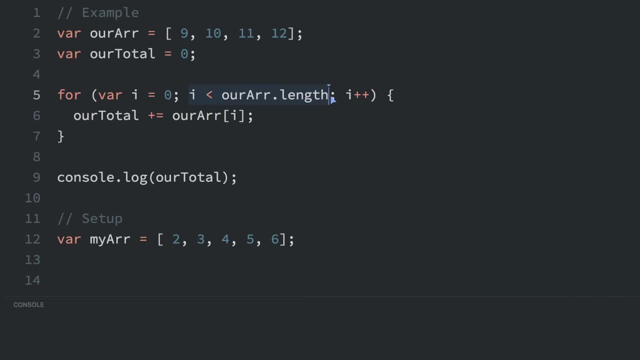 instead of going to a specific number of iterations, we're going to the, our array dot length. So the length is four here. But if we added elements to this array, that means this loop would just go even longer until we went through every element. 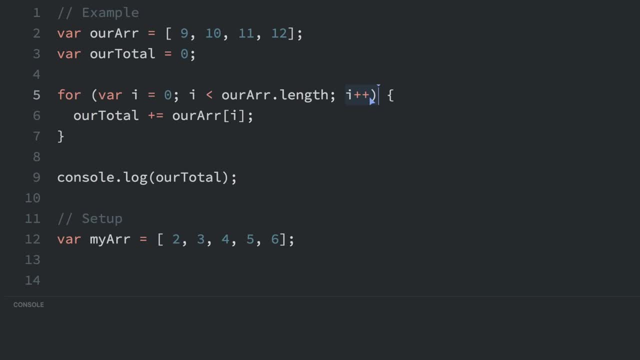 of that array And then at the end we're going to increment i by one at the end of each iteration. So look what we're doing inside the array. we're doing our total. that starts off at zero up here, and we're doing plus equals. that means we're going to do our total. 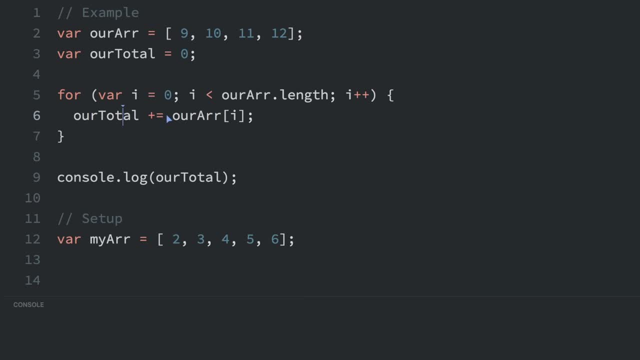 equals our total plus something else. So we're going to keep adding to the total whatever is in the array at that index. So our array I. so it starts at zero and then it goes 123 until it gets to four, which is the length of the array, And it doesn't even run the iteration. 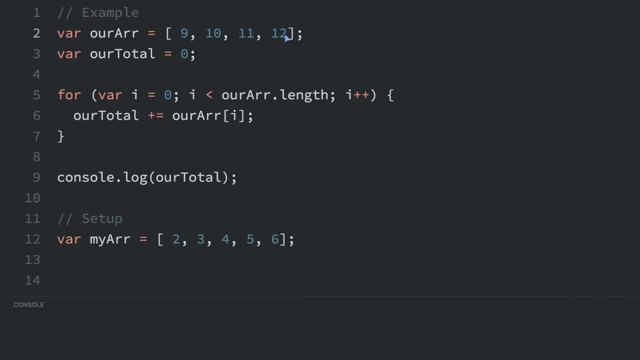 at four And there is no index four on the array. Remember it's 0123.. So this is just going to add up all those numbers. If we run this, we can see it adds up to 42.. I'm gonna write. 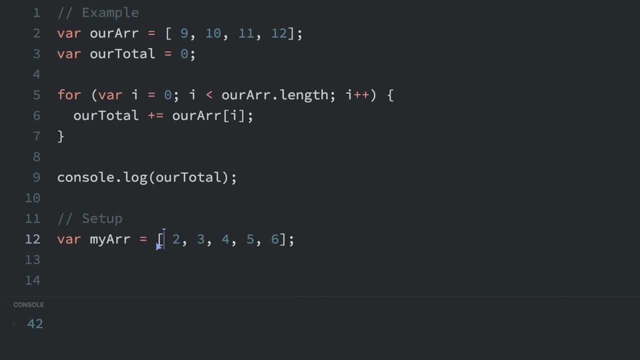 another for loop down here that's going to add up all the numbers in this array here. So we'll do four bar i equals zero, And then we'll do: i is less than i array dot length And i plus plus. So just like beforesell looks good, And we're going to multiply this by 4, flat i equals zero, and then 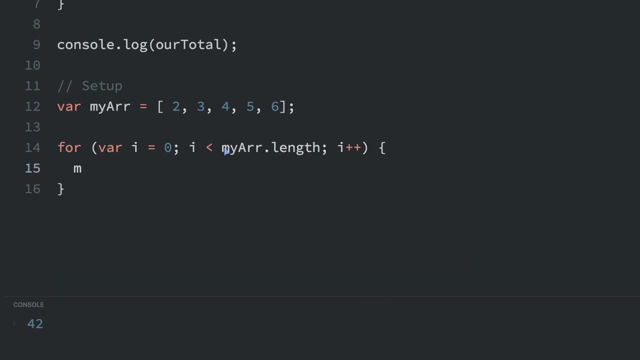 for each element in my array. we're going to do a, my, we're going to do a. total plus equals my array index, i. So we have to initialize the total variable right up here. So we'll do var total equals zero. And then at the end we can just, we'll just console dot log that out to see what. 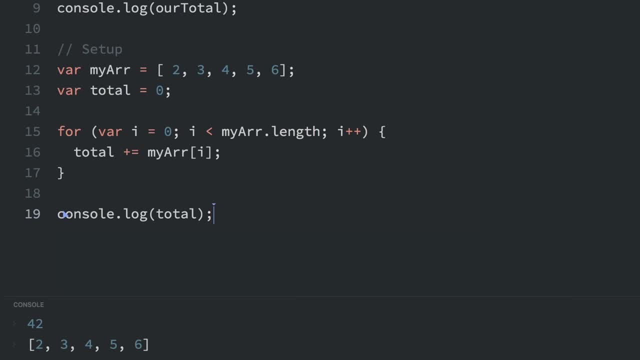 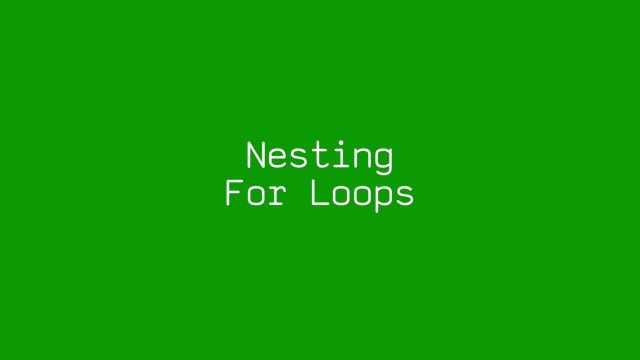 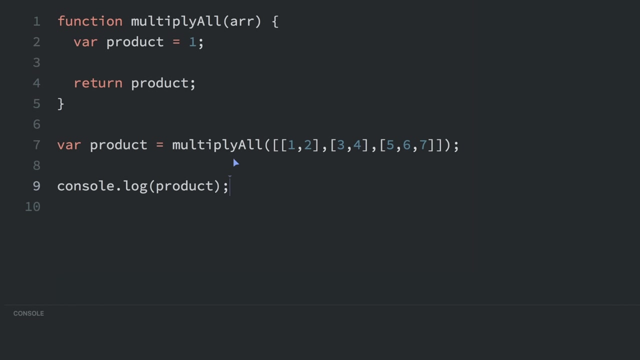 the total is. So by just run this we can see that the total this time is 20.. If you have a multi dimensional or nested array, you can use nested for loops to access all the array elements. So, for instance, we have this multiply all function. it's defined up here but we're calling. 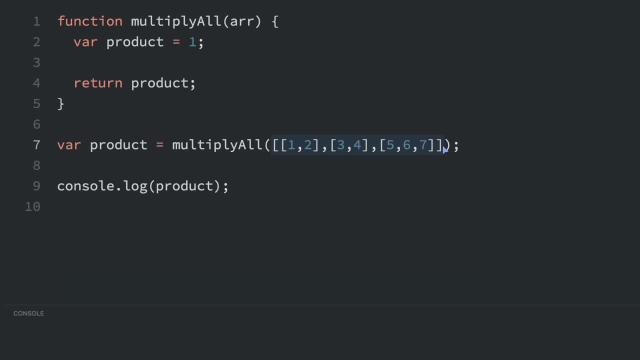 it here And we're passing in this multi dimensional array, which is basically an array, with arrays inside the array. So inside the first array there are three elements: one, two, three, and you can see each of those elements are an array with their own set of elements. So 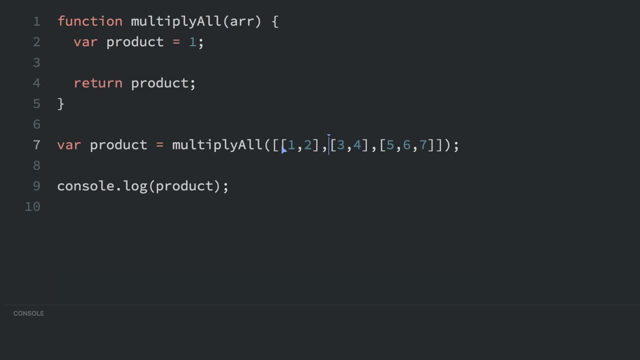 we are going to use nested for loops within this multiply all function to multiply every number in these nested arrays here. So let's get started. we're going to start with a for loop And it's going to look just like the other for loops we started. i equals zero. we're going to say: 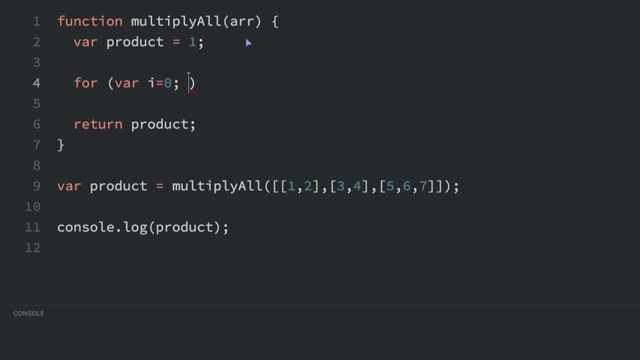 we're going to initialize i to zero And then we're going to say, while i is less than r dot length, And then we're just going to increment i at the end of each iteration. Now our dot link, that's going to start off as three, because we're passing in this array And the first level of the. 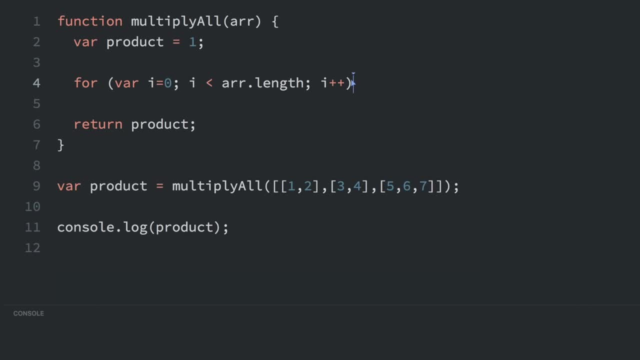 array there's just 123 elements, So that's going to be three. But now we're going to go inside the for loop and create another for loop, So we're going to do: var j equals zero. Normally it's standard practice to call the variable that we're incrementing i, but we already have an i within. 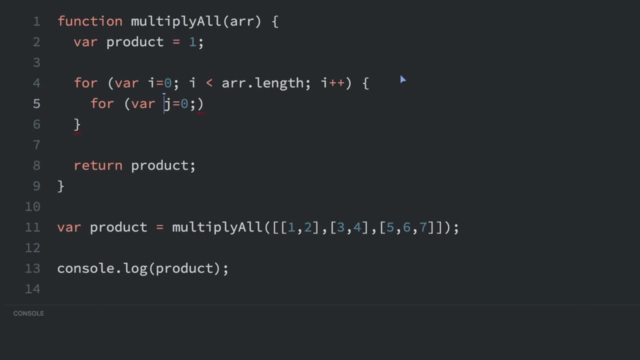 this scope. So we need to create another name, And it's pretty standard to call the next variable j, because j is after i, So now we're going to do j while j is less than now. this is where it gets a. 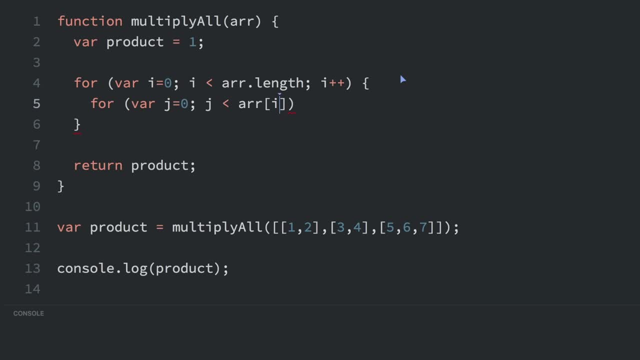 little tricky We're going to do. while a is less than our index, i dot length. Also, we're going to increment j here. So this is going to change. So first the first iteration of this outer for loop. we're looking at the length of. 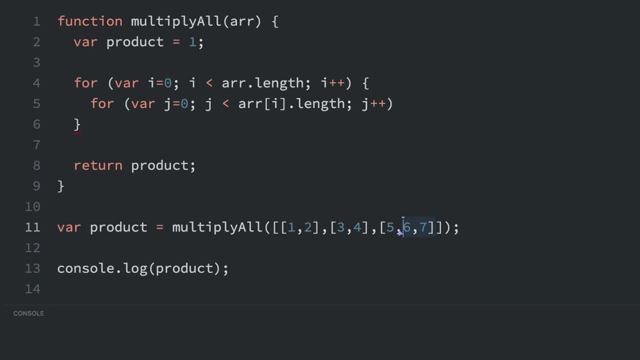 this array, then we're linking, looking at the length of this array, then we're looking at the length of this array. the index is going to be different every time, So we're going to be going to each different array inside the nested array. So at this point, 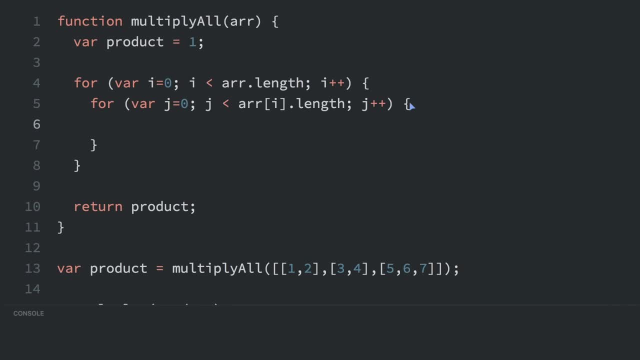 we just have to multiply all the numbers together So we already have the product that we've defined above. So we're going to do product times equals, which is just going to multiply everything together, And we're going to do our i- j. So the i references the outer array and the j references 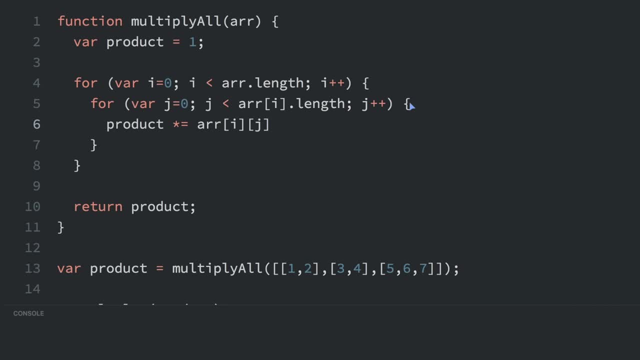 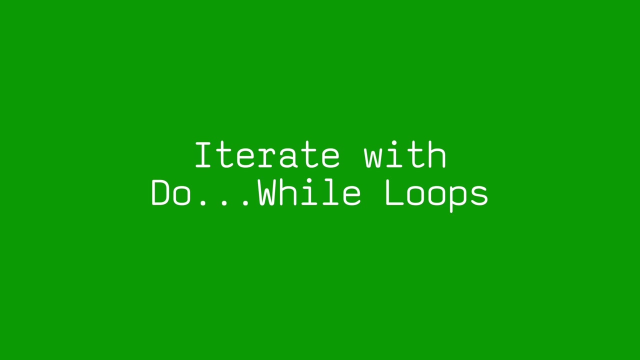 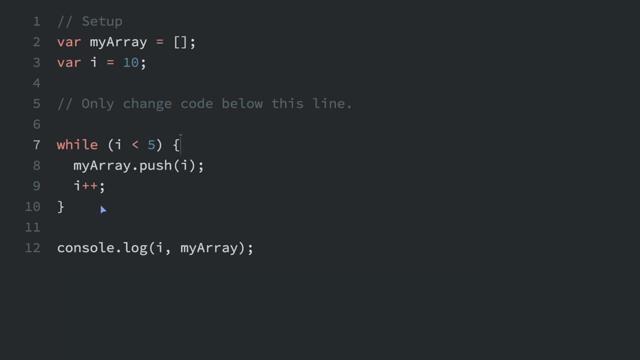 the inner array within the what we're passing in. And now we're done, So let's work. we have the console dot log here, So let's run this and see what happens. And 5040.. Next I'm going to talk about do while loops. Now we already talked about while loops. 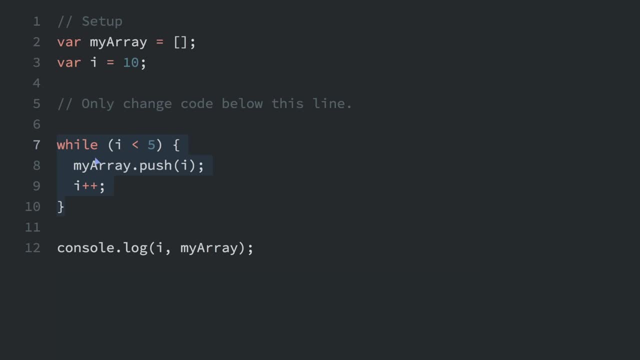 And I'm going to review this while loop And then I will tell you how a do while loop is different than a while loop. So this while loop first checks the condition of the loop And then we're going to run the condition before it runs any code within the loop. A do while loop will always run, at least 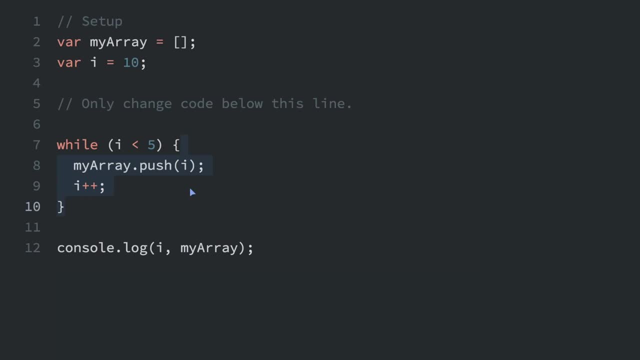 one time and then it will check the condition. So here we have this empty array. we have i equals 10.. So while I is less than five, well, I is not less than five, So it's not going to do anything. 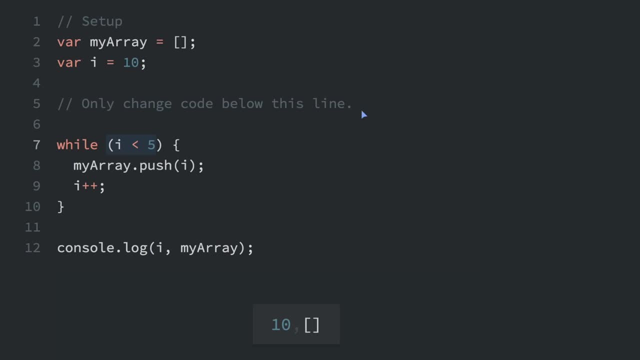 Let's see what happens. So we see it logged out 10. And then an empty array, because I started as 10. And my array started as this empty race. you were logging the I and my array with a do while loop. 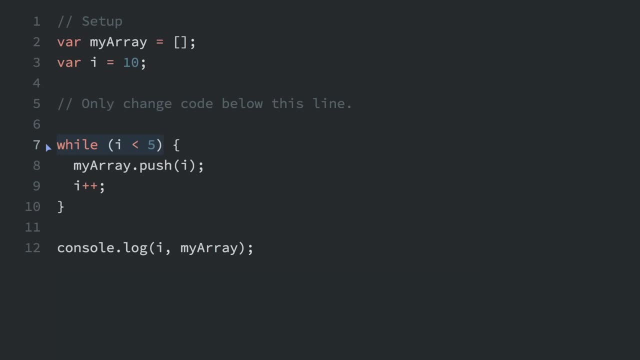 it's different. So what I'm going to do is cut this line up here and put it at the end, And then at the beginning, I'm going to put the keyword do in a do while loop. this is always run at least once before it checks the condition. So first it's going to do these things And then it's going. 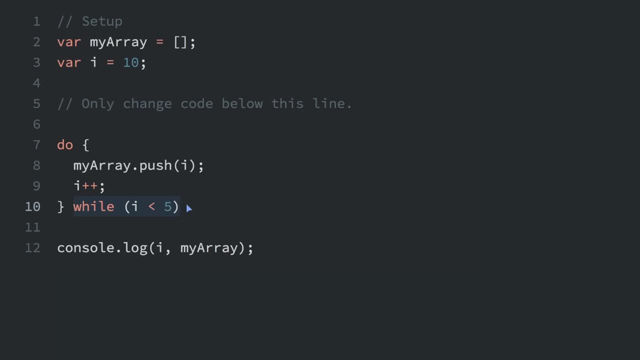 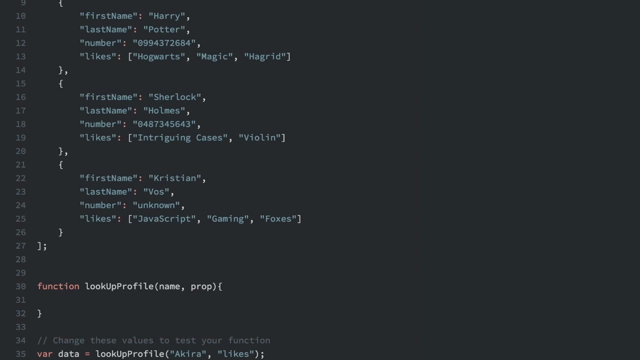 to check the condition. In this case it's going to find out. the condition is false And it's going to break out of the loop. Let's see what happens. So we're going to run the do while loop And then here see, now I is 11. And the array has the 10 added to it. This is a coding challenge we have. 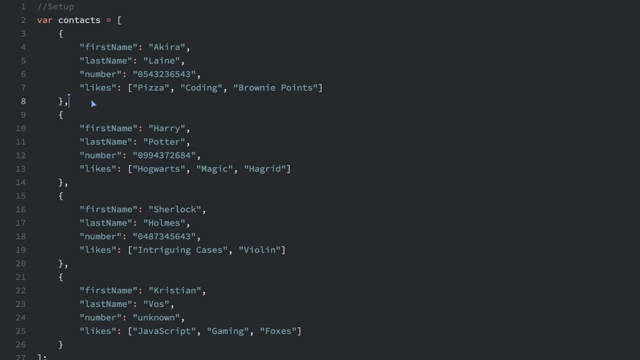 this array of objects in our contacts list And you'll see, each object is one of our contacts with a first name, a last name, a number and likes. So these are key value pairs here. So what we want to do is create this lookup list, And then we're going to create this lookup list, And then we're going. 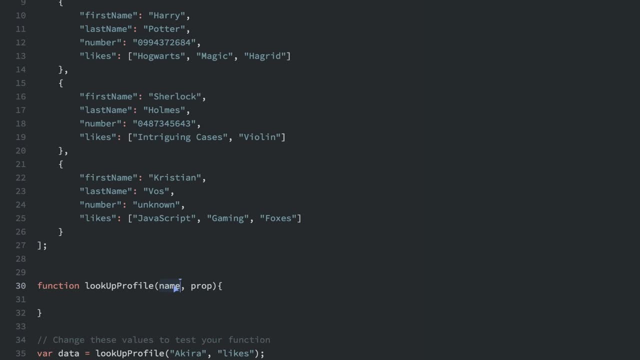 to create this lookup profile function. where we pass in a name, this is the first name and the property And it's going to return the value of that property. For instance, if we pass in the name Kristen here and we pass in the property of number, it should return unknown If we pass in. 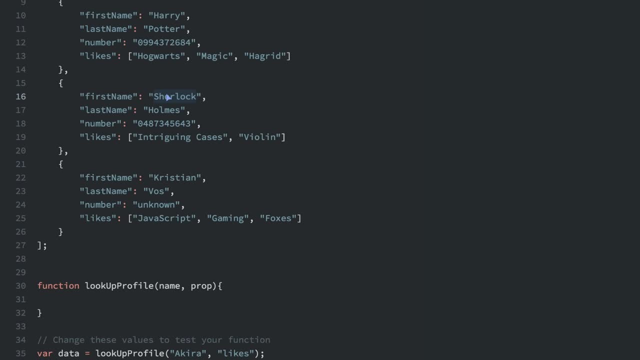 the first name of Sherlock up here and we return the property And we pass in the property of likes. it should return the array, intriguing case and violin. If the name that's passed in does not correspond to any contacts, then our function. 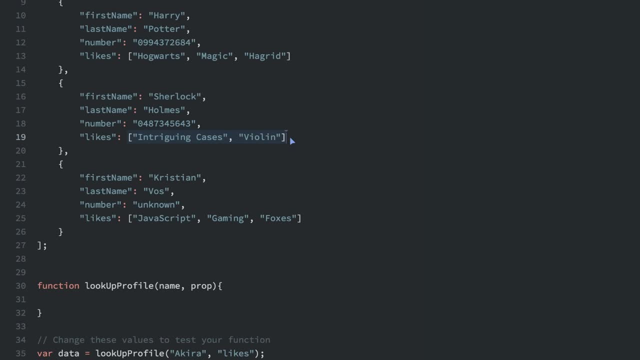 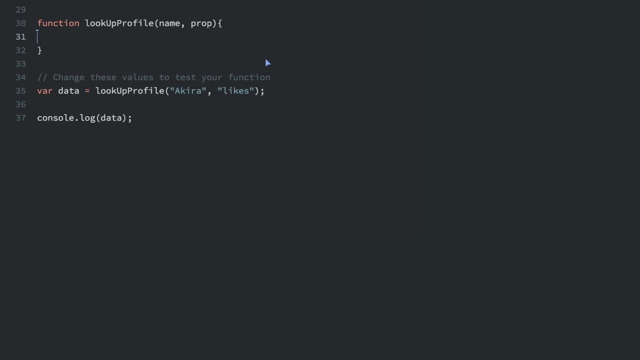 should return no such contact. And if there's no property, it should return no such property. So let's go to this function here and start creating it. So the first thing we're going to have to do is iterate through each element in the contacts list. So let's make a for loop. So for bar bar. 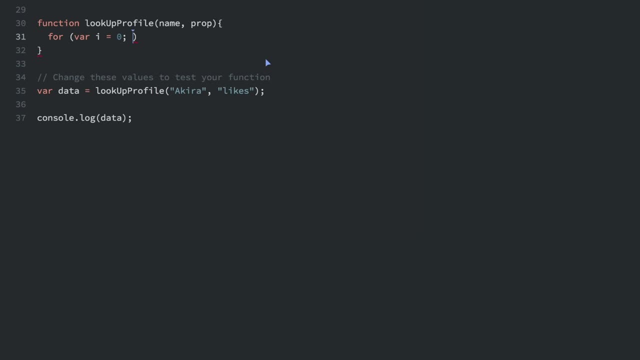 I equals zero, while I is less than contacts length, And at the end of each iteration we'll do I plus plus to increment that. So for each of these contacts, the first thing we're going to check is if the name is. 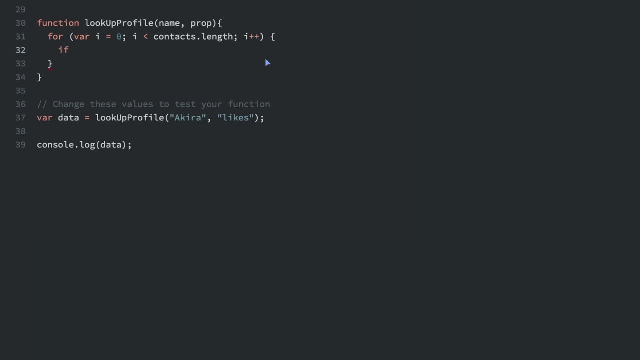 a name in this list. So if contacts I first name equals equals equals the name that was passed in. So we're checking each item to see if it was a name that was passed in And if so we're going to do something Now. if now we're. 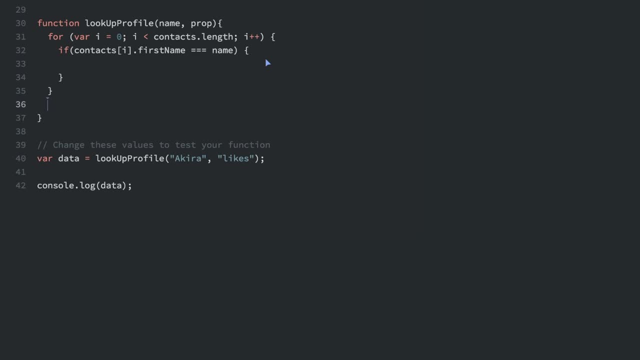 gonna do something else, So let's do that Now. Remember, if the name that was passed in is not in the array, we're going to return no such contact. However, if it is in the array, we're gonna do something else If the name is in the contacts. 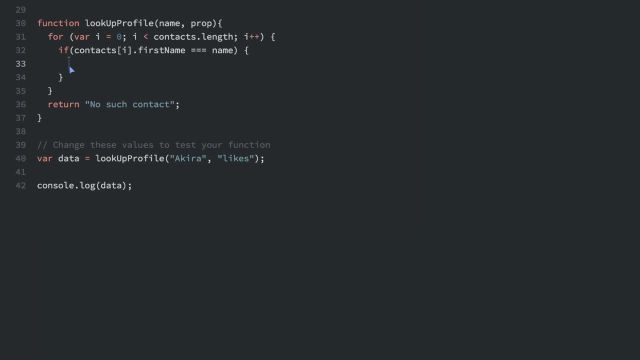 list. we're going to return the value of the property that was passed in. So return contacts, I crop. So this will return the value of that property that was passed in. However, there is another case, which is if the property does not exist, we return no such property. So 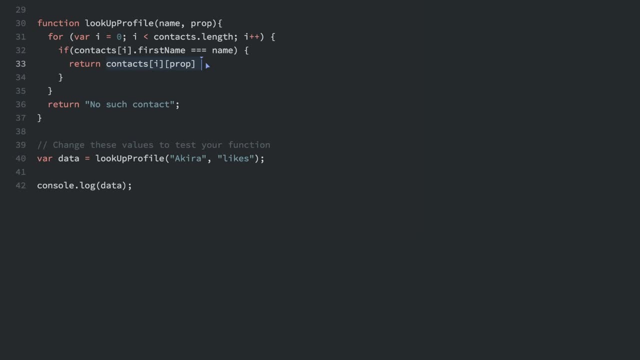 a fancy way in JavaScript of saying: use this value if it exists, but otherwise use a different value is to use the or operator. So we'll say return contact I prop or if it doesn't exist, we're going to return no such property. Just so you know there would be a. 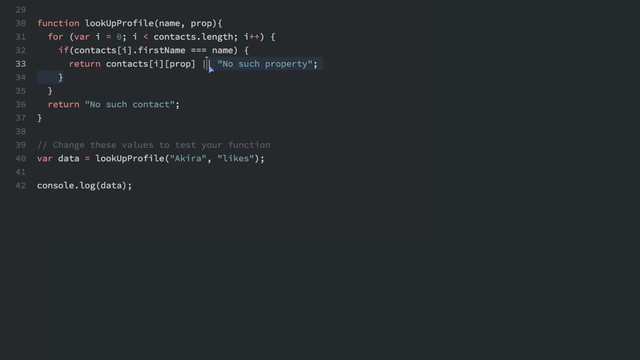 way to do this without using this or operator. as long as the your code passes the requirements, That's all that's important. There's many ways of doing this, But let's check it. So right now we have our lookup profile or profile, we're going to have our lookup profile and we're going to 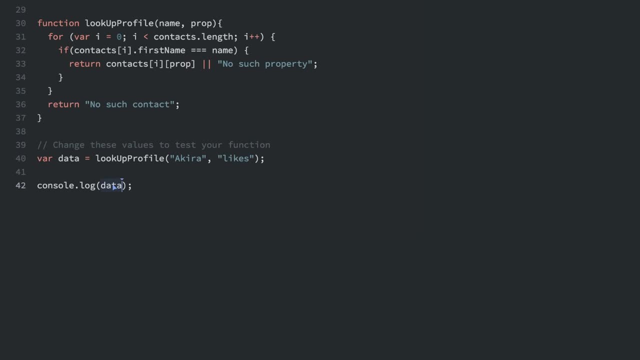 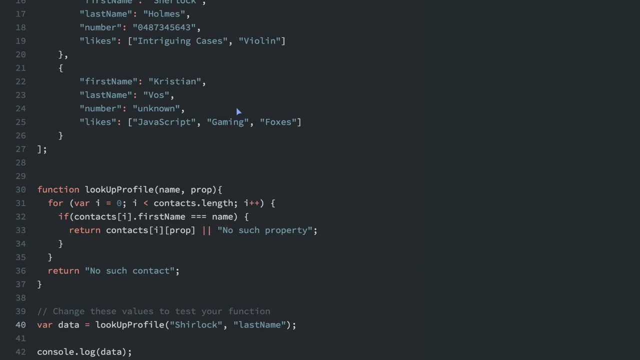 pass in a key run. we're trying to find the likes and we're console dot logging the data and pizza coding brownie points. So what if we passed in something else? if we passed in Sherlock, we pass in last name. Oh, such contact. Well, that's working, because I spelled Sherlock wrong. 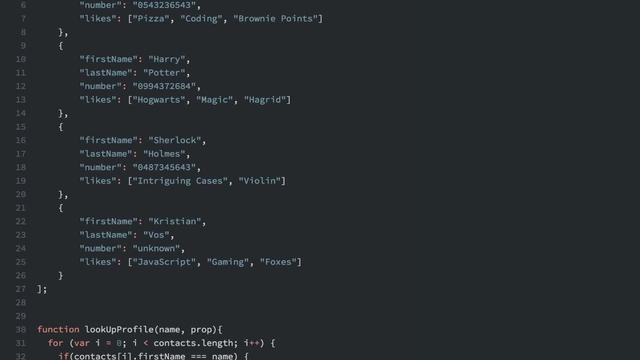 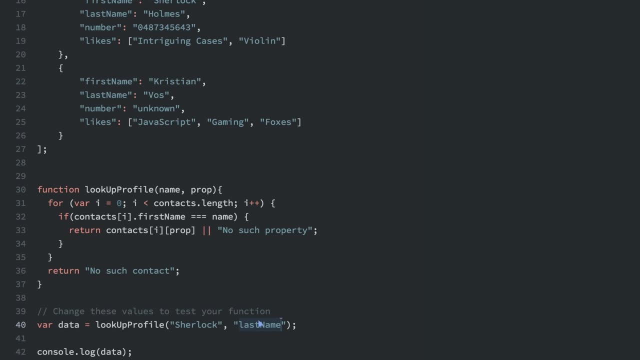 This is E, So it's good way, a good way to test that homes, And the last thing we'll check is if we pass in a property that does not exist, I'll just say hello and no such property. So our function works. 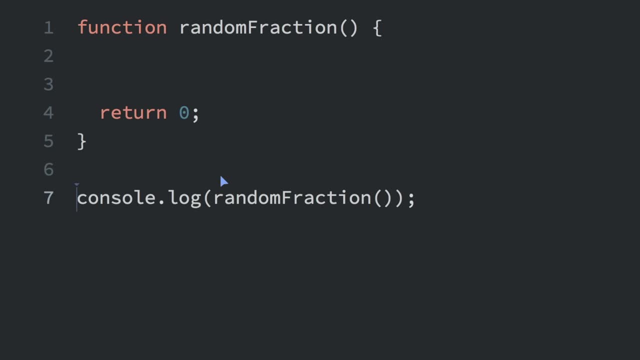 There is a simple way to create a random decimal number in JavaScript. It's with the math dot random function. So we have this function here which is says random function and it's returning zero currently. but we're going to use the math dot random function And you will see that when I 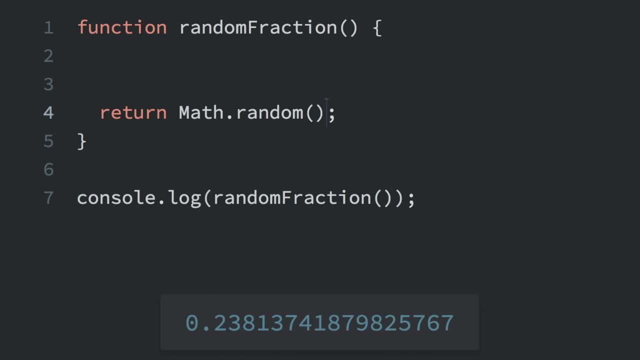 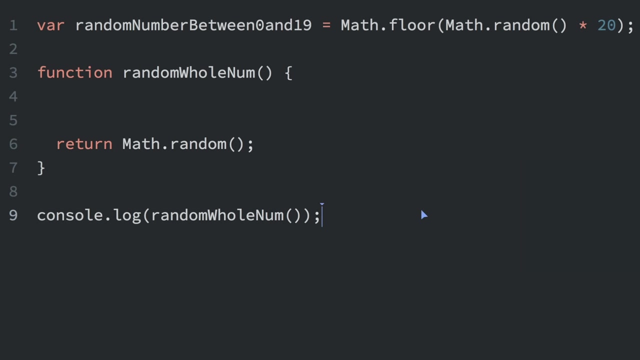 run this, we have 0.23813741 and so on. So it's always going to be a number between zero and it could be zero between zero and one, but it could not be one. Often you want a random whole number instead of a random decimal number. That can be accomplished with math dot random function. So if 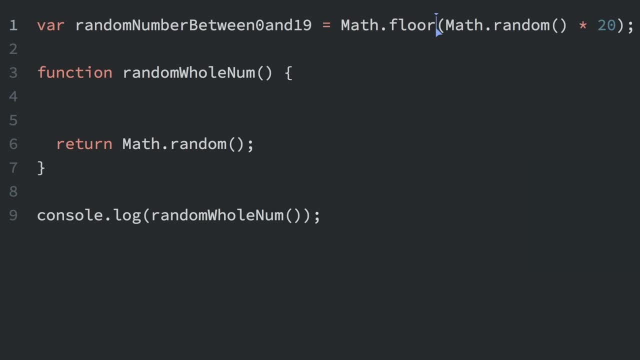 we run this. We have math dot floor, we have math dot floor here. this rounds down to the nearest whole number. So we pass in math dot random times 20.. And then we round down to the nearest whole number. this is going to create a random whole number between zero and 19.. Remember math dot. 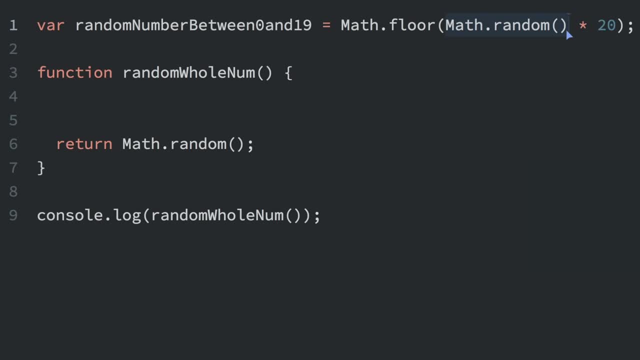 random, can never be one. it can be zero, but it can never be quite one. So when we multiply it by 20, going to get a number between zero and 20, but not including 20, then we round down which will end. 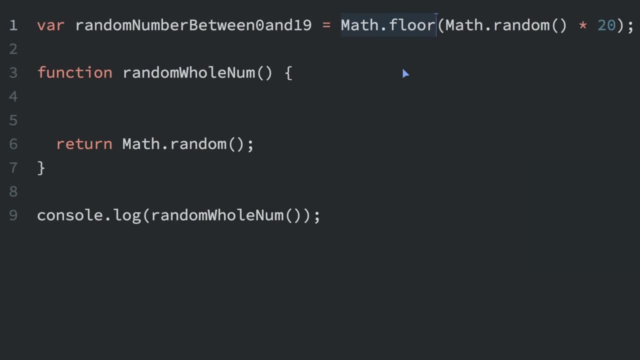 up being zero to 19.. So let me show you another example where we're going to get a random whole number between zero and nine. it's going to look just like this. So we're going to modify this function. So this math dot random, we're going to pass that into math floor. So I have to put 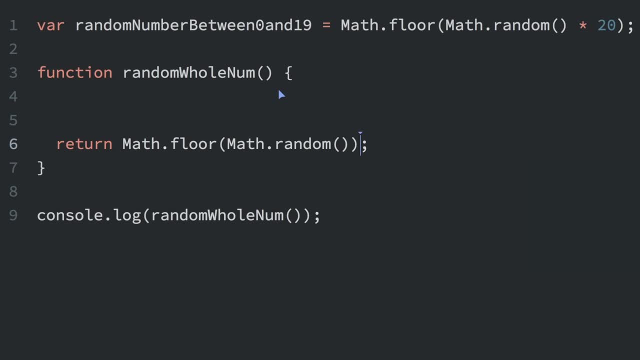 the parentheses because we're passing an end to that function And it's math dot, random times 10.. And that's going to give us a random number between zero and nine. So if I reload this, you can see 9541.. Every time I load it it's a different. 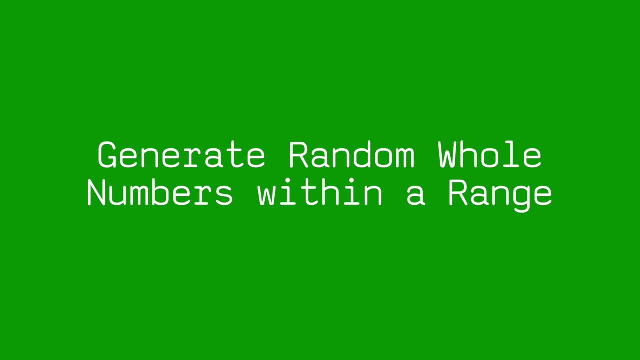 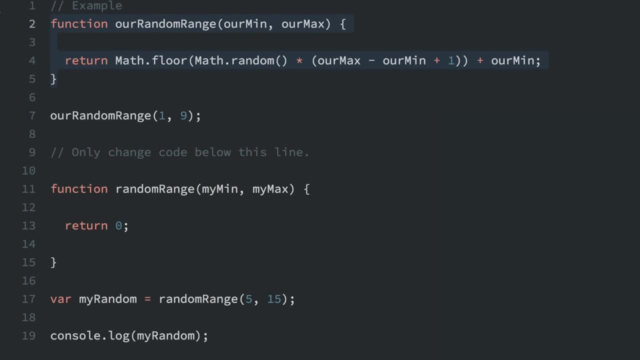 random number. You can also generate random whole numbers within a range. So look at this function here, our random range. it takes a minimum number and a maximum number And then it just runs through this calculation here. So we have the math dot random and we 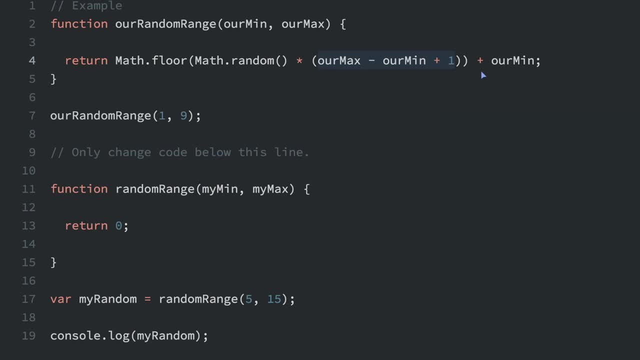 multiply it by the max number minus min number plus one, And then we get the floor which is rounding down and we add all that to our minimum number. So this is just a calculation to get a random number between the min and max. So as practice I'm going to rewrite it down here. 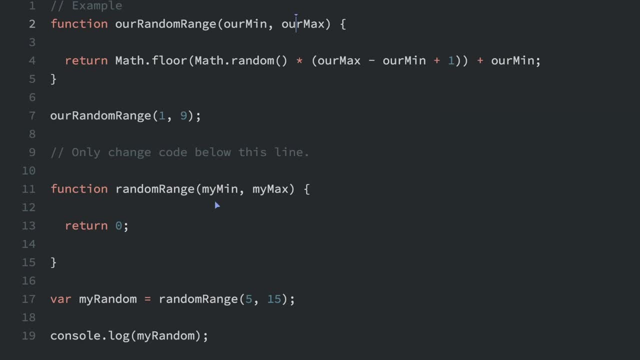 So we have the random range instead of our min and our max. we have my min and my max. However, the equation is going to be the same, So we have math dot floor. you can take a chance to actually just look over the equation and see if you can understand how. 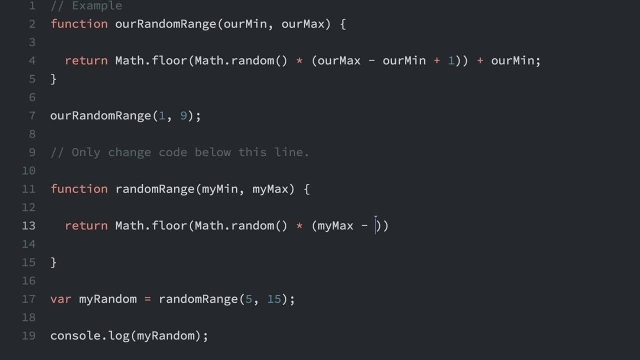 it works: My max, minus my min, And then we just have to do plus one, And then this whole thing is going to be plus my min. So we already have this example. So we're going to run the test setup down here, random range between five and 15.. And we're going 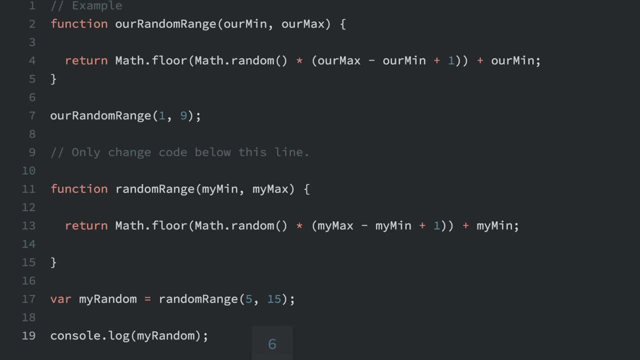 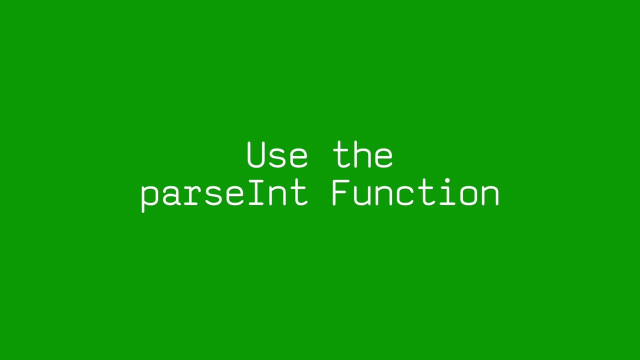 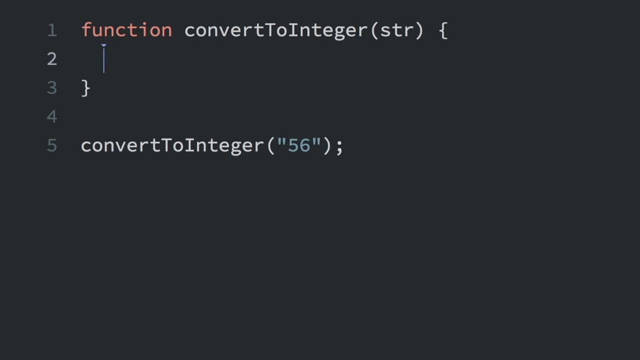 to log it out here. So let's try that. 1167.. See, every number is between five and 15. Whenever I run it. Another useful function is the parse int function. it takes a string and returns an integer. a lot of times you want to make sure you're dealing with integers and not strings. 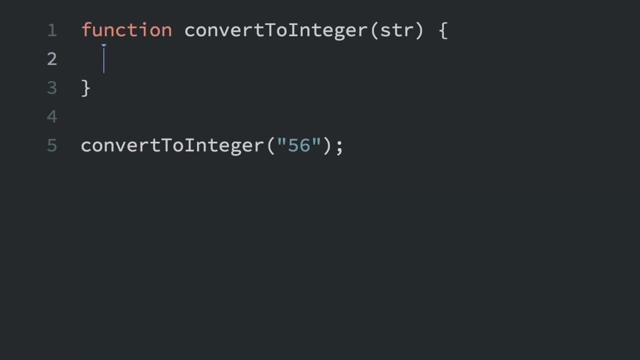 for different calculations and things like that. If the string cannot be converted into an integer, it returns in a n for, not a number. So let me show you how it works. From this convert to integer function, we are going to return And we're going to return the string. 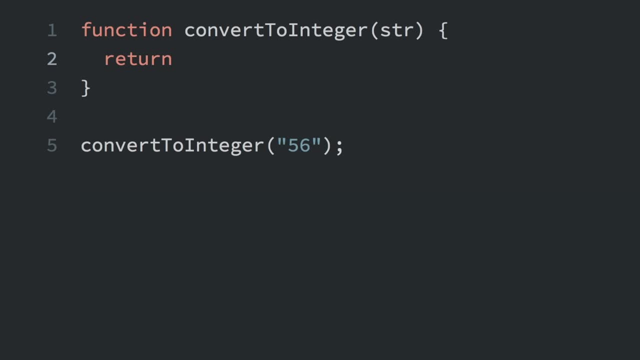 except we're going to convert it into an integer first, So we'll do parse int And then I'll pass in the string. Now it was a string, because you can see here we're passing in the string of the 56. But it's going to return it as a number. 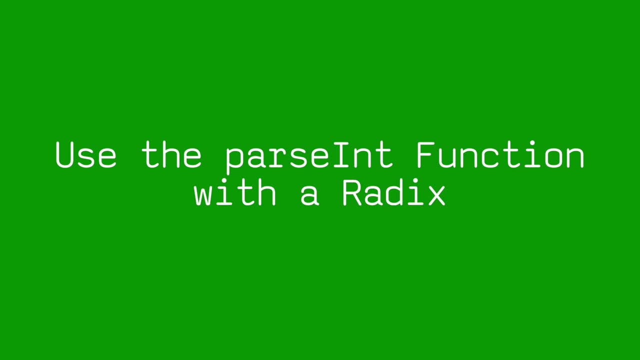 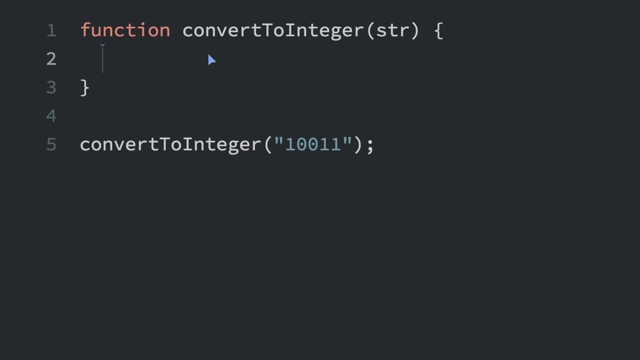 An integer. The parse int function can also be used with a radix. The radix specifies the base of the number in the string, such as base two or base seven or base eight. a base two would be binary, So that's one of the most common ones to use. Now. the default is base 10.. That's what. 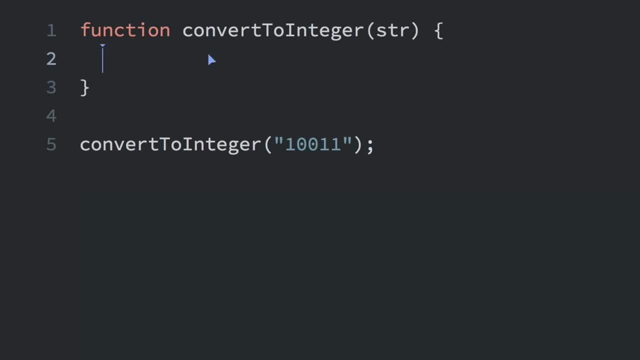 we use normally every day. But let me show you how that would work. We're going to convert this number, which is an integer, And then we're going to return it as a number And we're going to pass in a binary number to an integer. So we'll do return And I will do the parse And I'll pass. 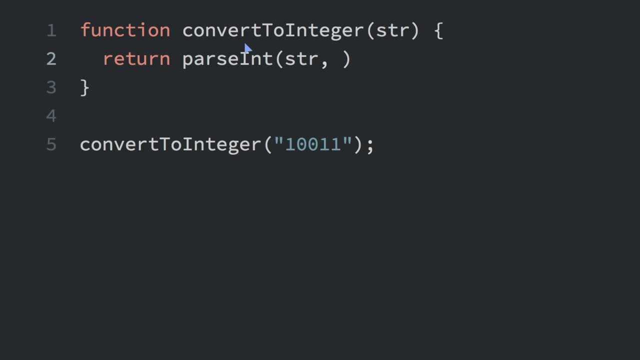 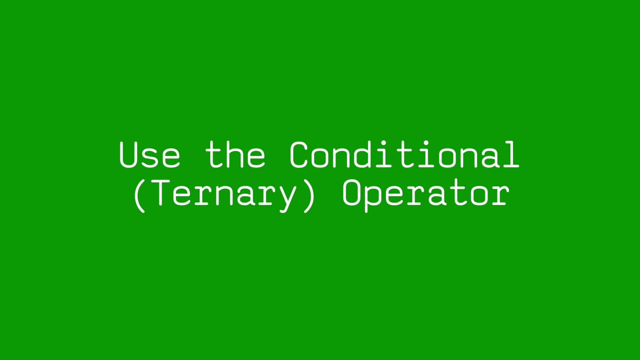 in the string as before, But now we'll have a second argument after the comma, which is going to be the number two. So instead of the default of base 10, we'll be passing it as base two. So the computer knows that this is a binary number. I love the ternary operation. 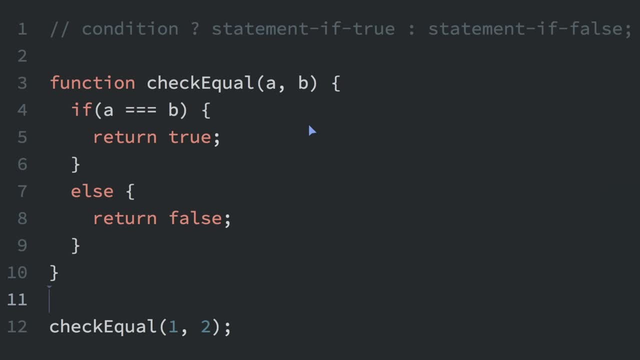 I love the expression. the ternary operation is actually a one line if else expression. Now, this is what it looks like. you have your condition, just like an if statement, and then you would have a question mark. After the question mark, you have what's going to happen. 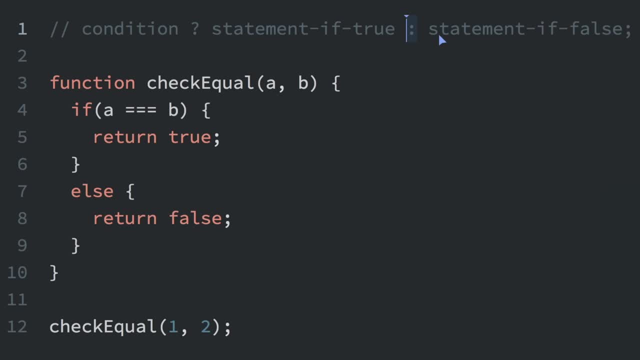 if the condition is true, then you have a colon, then you have what's going to happen if the condition is false? So we can replace an if else statement like this into something using the term area operator. So here we have this: if this condition is true, we're going to return true. 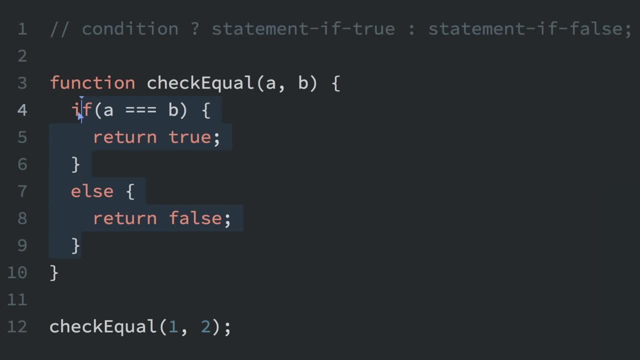 else we're going to return false. let's change this. So now we're going to use the ternary operator, So now it's just going to say: return a equals equals B. that's the condition. then we use the question mark. So if it's true, we're going to return true, And then we have a colon And after: 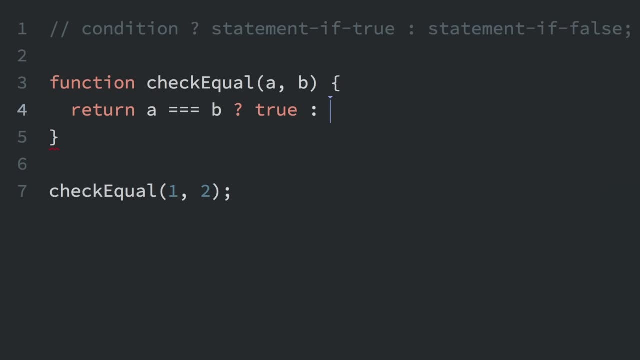 the colon we have what's going to happen if it's false, which is we're going to return false. Now I'll be honest: you would never write a line like this in real life, because you could just write: return a, equals equals, equals B, And this lines actually going to do the same thing as this line. 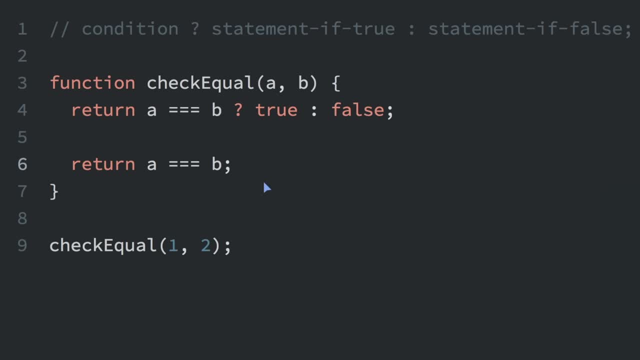 However, I just wanted to give you a simple example of using the ternary operator, And one of the great things about conditional or ternary operators is that you can nest them within each other, which gives them even more power. So we're going to read: write a function. 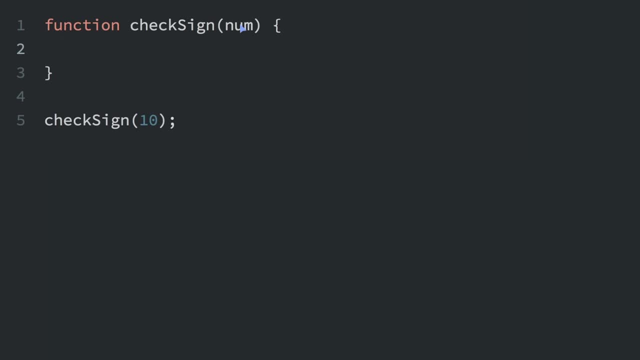 here the function check sign and it's going to return the string: positive if this number is positive, negative if if the number is negative or zero, and we're going to use a nested conditional operator. So here it is return, And first we're going to check if num is more than. 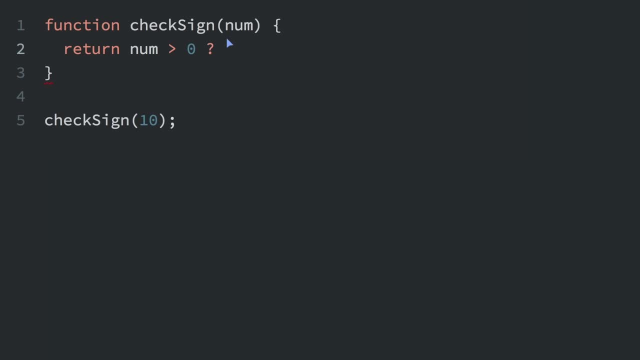 zero, And then we'll use the ternary operator. If so, the first thing after the question mark is: if it's true. if it's true, we're going to return positive. If it's false, if the number is not more than zero, we'll do something else. But here's where we're going to have another. 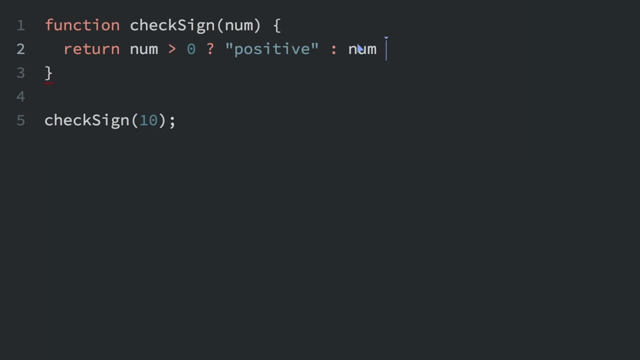 ternary operator. we're going to check if num is less than zero. So, if the number is less than zero, well, if that's true, we have to have the question mark mark for the ternary operator. If that's true, we're going to return negative, And if it's false, 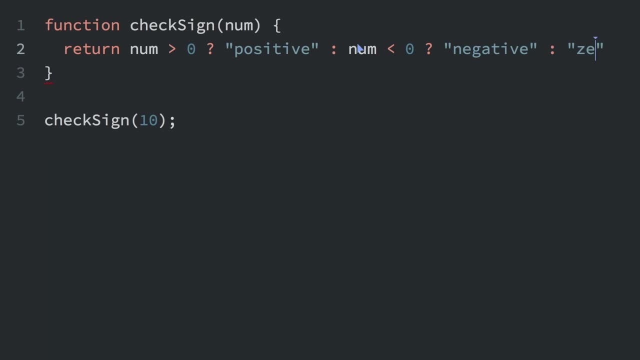 that's where the colon comes in. we're going to return zero. So let's do this check sign. I'm going to do a console dot log So we can see what this returns here. And we can see this is going to return positive. if we have a negative number here, it's going to return. 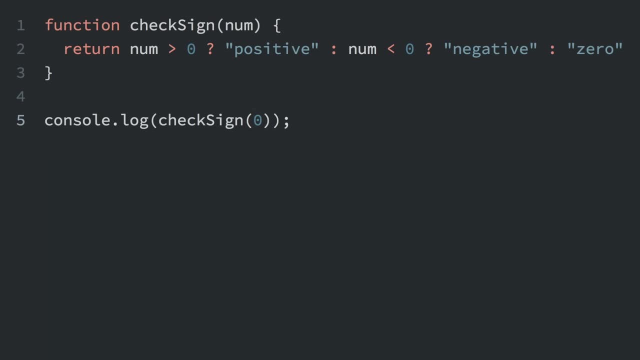 negative, or if we have a zero, it's going to return zero. Now you'll see that after this colon we have an entire ternary operator. So if this is true, we just return positive. if it's false, then we do everything here, which is another ternary operator where it checks if 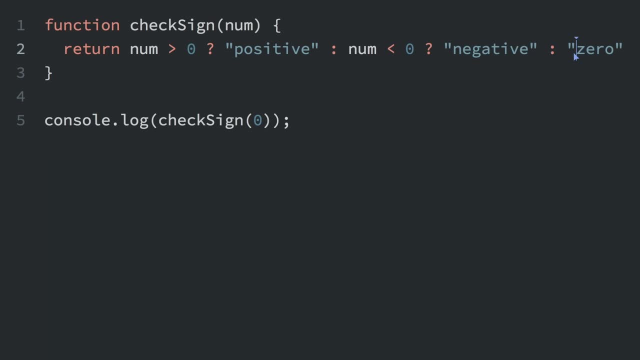 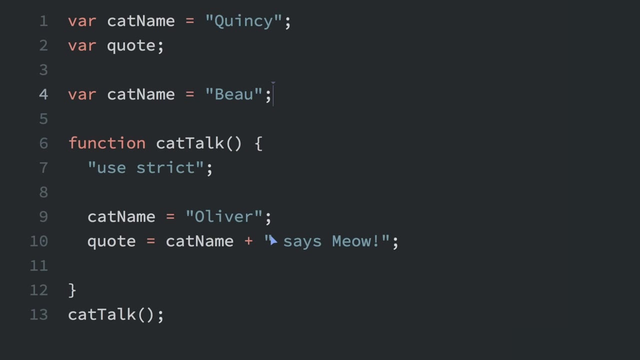 this is true, And if that's true, we return negative And if it's false, which return zero. For a long time in JavaScript, if you were going to declare a variable, you had to use the var keyword, But starting with ES six in 2015,, we can now declare variables with a let and const. 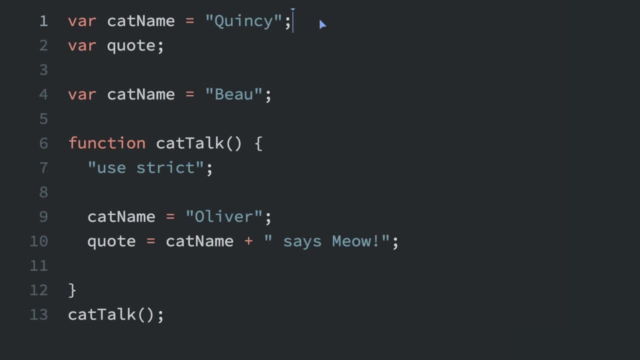 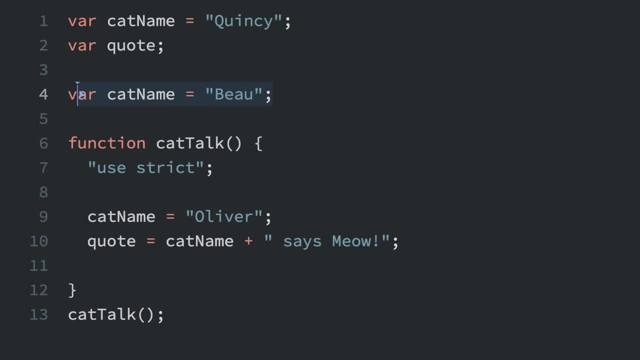 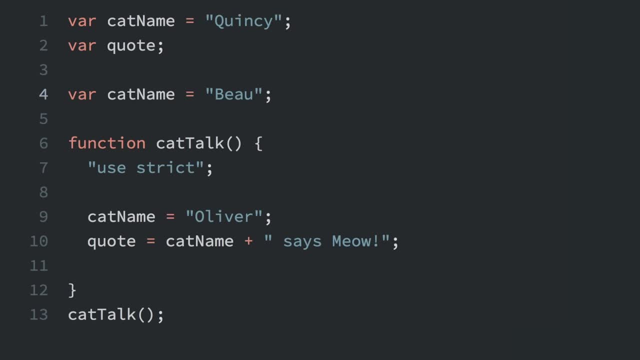 if I just run this code, you'll see that nothing is happening. It's just allowing us to set the cat name twice and declare it twice with the var keyword. However, if we change this to let, we're going to change all of our collect and you'll see that when we load it again. 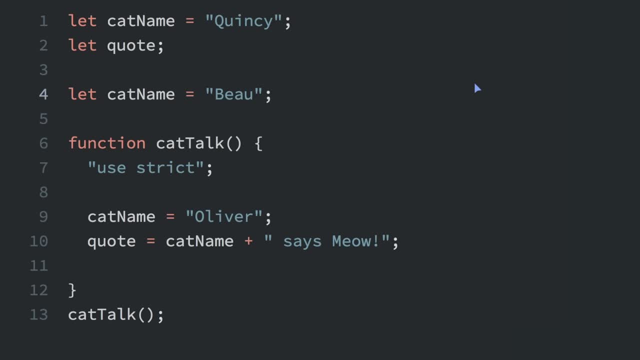 you'll see an error. duplicate declaration- cat name. So this is good that it's creating this error, because you usually don't want to declare a variable two times in the same scope, So this allows your program to give you an error to tell you that you've done something wrong. Now 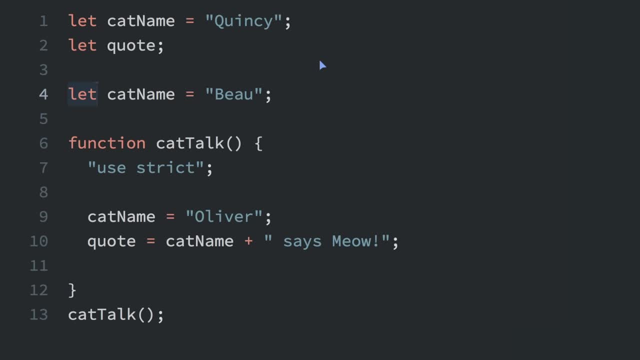 you can still reset it. So if we didn't use the word let here, we could just set the cat name variable. And now we're not going to get an error In this case. we're declaring the variable here to be Quincy And we're setting the same variable to a new name here. This is one of a few reasons that. 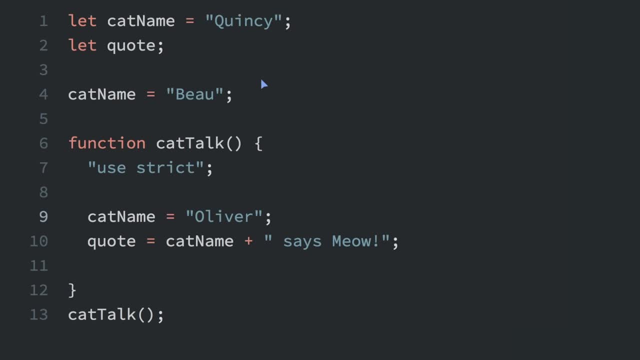 many people only use let and const and never use var to declare variables. Another thing in this code you can see is use strict. Now this enables strict mode, which catches common coding mistakes and unsafe actions. So a lot of people will use use strict at the top of a full JavaScript file. 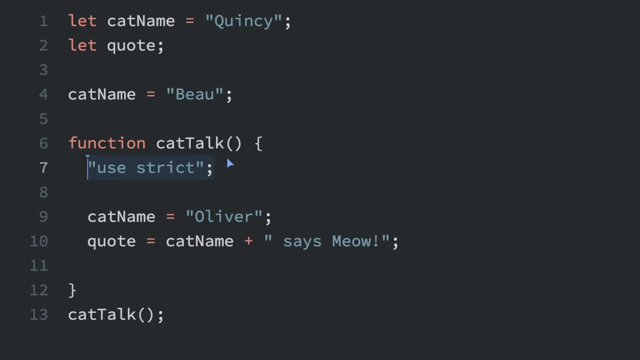 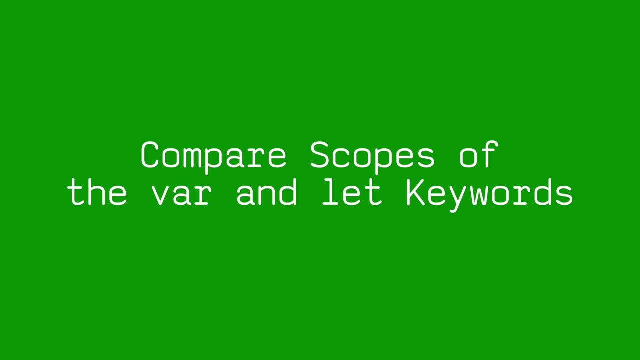 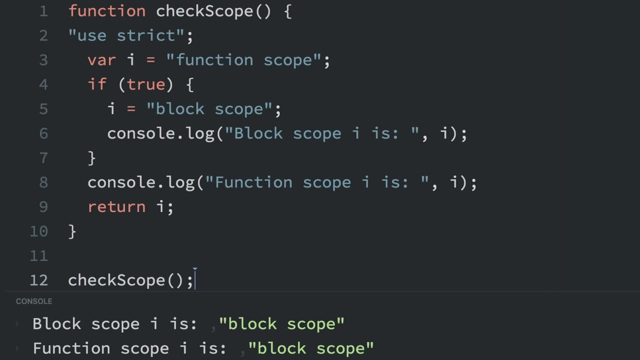 or maybe just in a file Function to catch coding mistakes, such as if you create a variable and don't declare it with var letter const. Another major difference between the var and let keywords is that when you declare a variable with var, it is declared globally or locally if declared inside a function. However, 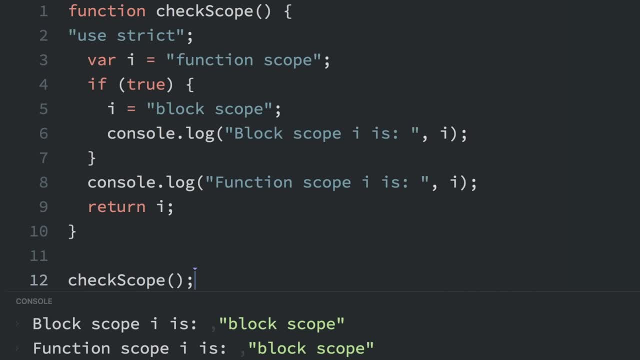 let- the scope of let is limited to the block statement or expression. let- The scope of let is limited to the block statement or expression that it was declared in. So let's look at this example here. If you see this code, we have this. 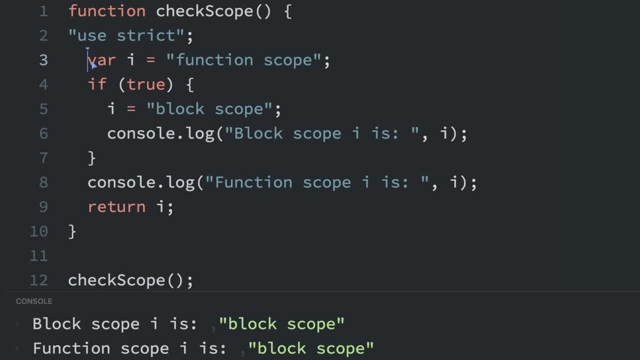 check scope function and we're calling it down here And it's setting I with a var here of our keyword to function scope. then we're setting it to block scope in here And you can see it's console that logging block scope I is. it says block scope And we will get down here function scope. 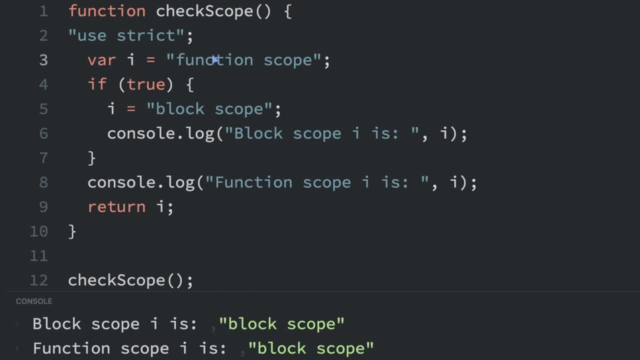 it's still block scope. If we want this to be a function scope, then we're going to have to do a function scope. If we want this to be function scope down here, we're going to have to use let. so we would use let here and then we would use let here, And if we run the code now, you can see. 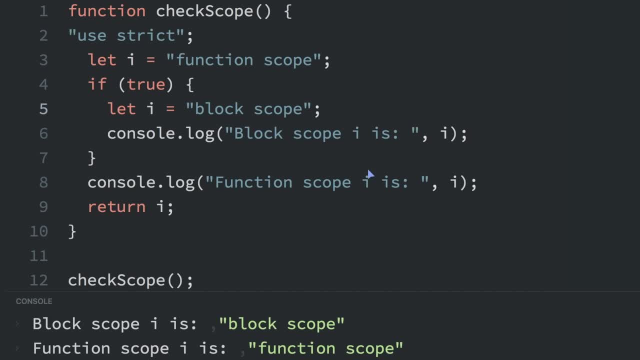 in the console: block scope: I is block scope. function scope: I is function scope. So even though we set I to block scope here inside this block- now a block is just anything inside these squiggly braces here. So we said I inside this block to block scope. But then when we get out, 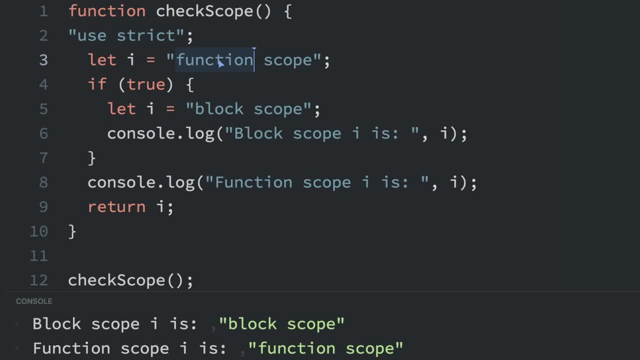 here. it's now back to function. scope because of this up here. Here's another thing I want to show you. If this is, if we comment this line out and we change this to var, what do you think is going to happen? Well, let's run and find out. Look, we set the var inside this block here and we're going. 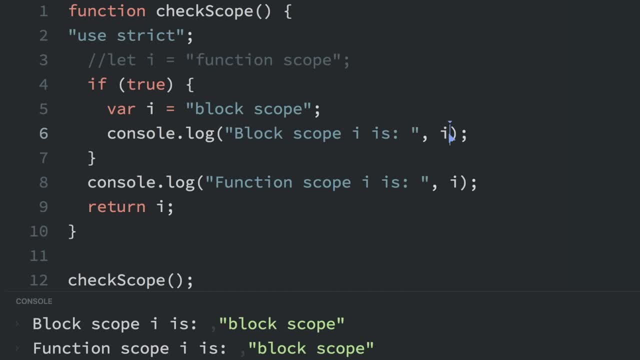 to use let here to block scope And it says block scope is block scope But then when we're outside of the block, when we're outside of these squiggly braces here, we can still access. I here- and it's set to block scope. But if this was a let and we're declaring inside this block, if we run that, 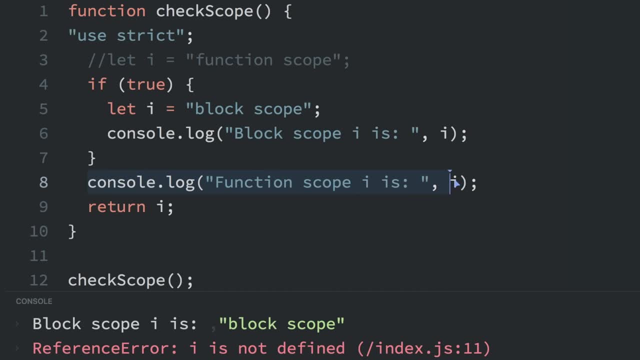 now, when we get outside the block, we get an error because it's not defined. So that's another reason why people use let instead of var, So that they can make sure the variable is only defined in the area they want it to be defined in. 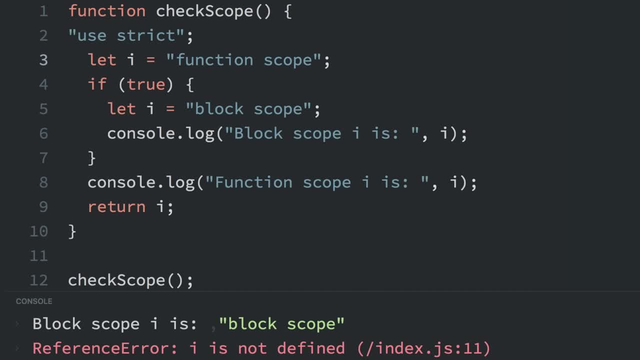 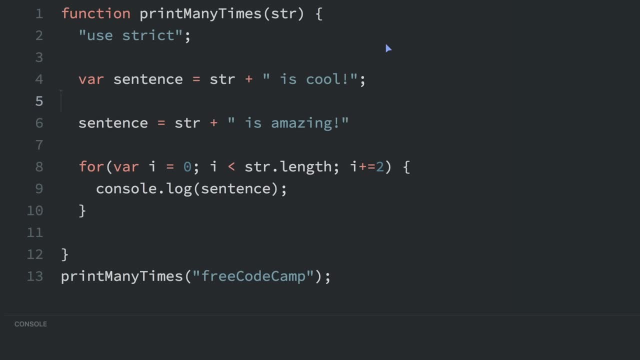 But for now I'll uncomment this out. Const is another way to declare a variable. It has all the features of let, but it's also read. only you cannot reassign a const. So let's look at this program here. We're running this print many times And it's going to log out this syntax. 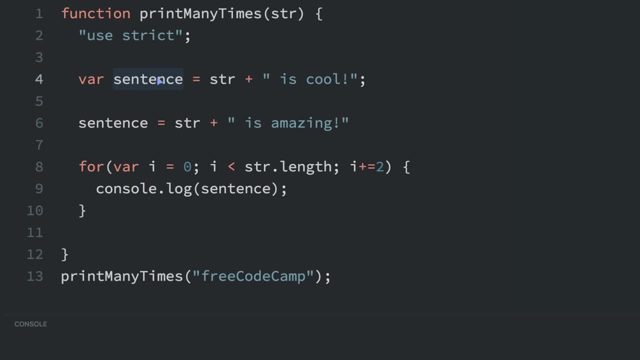 and then we're going to run it, And then we're going to run it, And then we're going to run it, And the sentence is up here, var sentence is declared, And then we reassign it here. So first we declare. 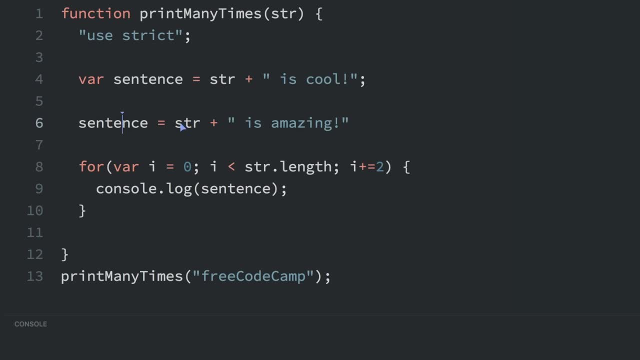 the sentence to be the string is cool. then it's reassigned to be the string. It's amazing. So if we run that, it should work. It prints free. code camp is amazing many times, But if we change this to const, let's see what happens. Now I'll run this and we get an error. Sentence is read only. 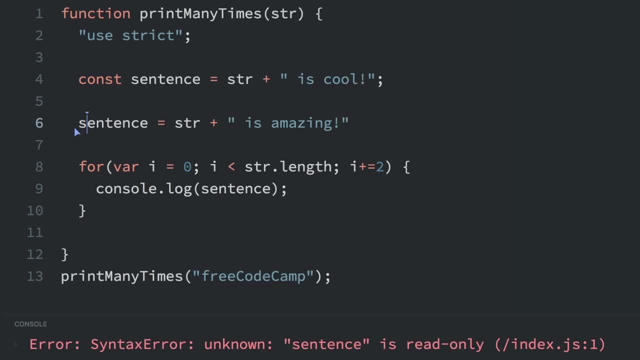 If you declare a variable with the const keyword, you cannot reassign it afterwards. This can be very helpful to prevent you from accidentally making mistakes later. If you know for sure that you never want to reassign a variable, always use const So you don't accidentally reassign it when. 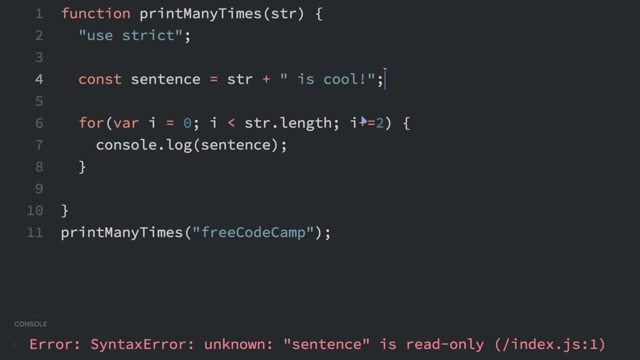 you don't mean to. Another thing is, when you're using const, it's very common to use all capital letters. So like this sentence, like that, And that's another way to remember that it's a constant. So if I rename this here, I'm also going to have to repeat it here. And while we're 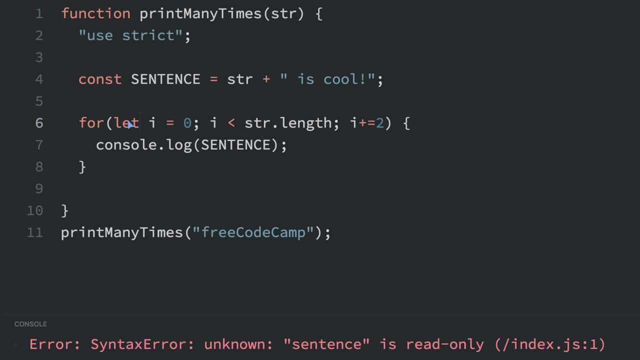 at it. we're going to change this to let because for the most part, you should only use const or let, but there are certain circumstances where you would use var And also in some other videos. in this course I'll be using var. 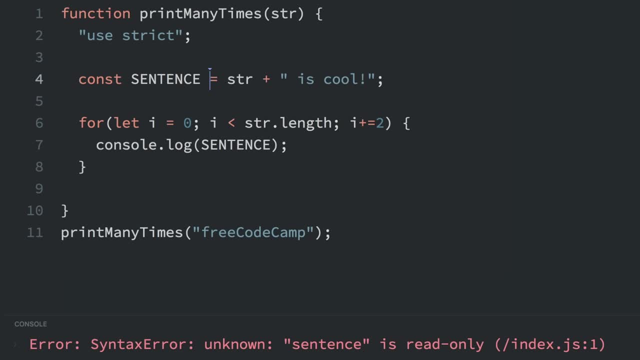 In your own code. you should mainly use const, and let let's reload this to see what happens. And it worked. free code camp is cool. Many times we can no longer say that free code camp is awesome, even though we know it actually is. 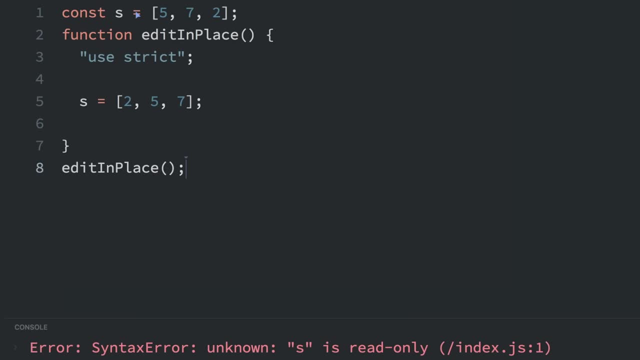 While you cannot reassign a variable declared with const, you can mutate an array. So look at this example. that's not going to work. First we declare the variable s and we assign it to an array. we declare with const, And now we're going to. 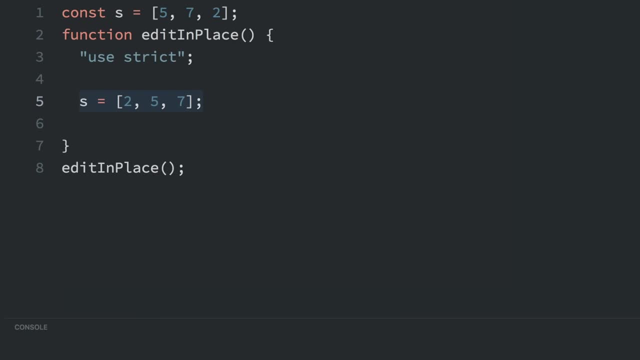 reassign the variable s here, But if we do that, we're going to get the error s is read only. However, we can update the array using bracket notation, So I'll just comment that out And using bracket notation, I'll do index. 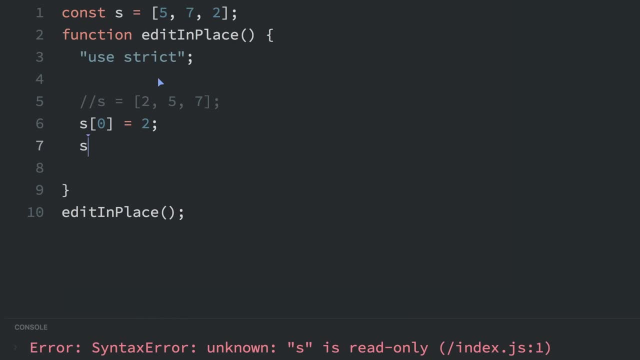 zero, I'll assign that to two. one, I'll assign that to five and then index two, I'll assign that to seven And just like that it is going to reassign the array. So if I just do a console dot log here, console dot log and put the array in there, we should. 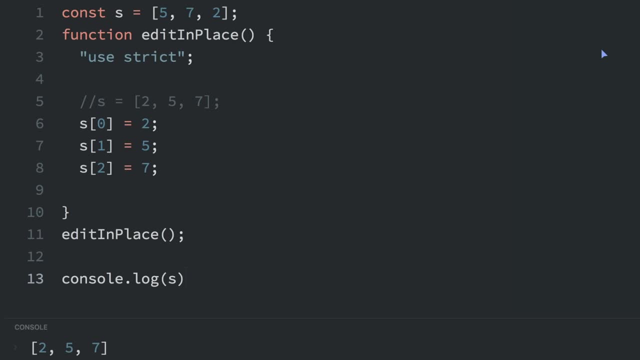 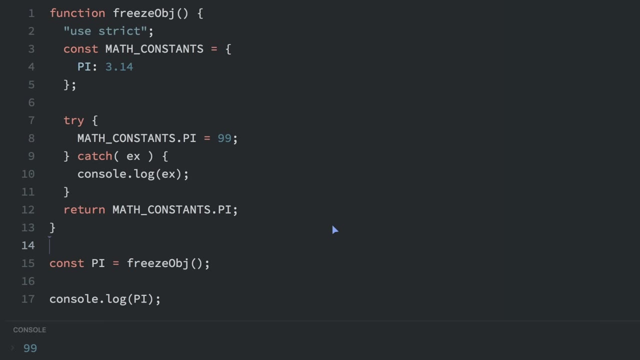 see the new array here, 257.. As seen previously, a const declaration alone doesn't really protect your data from mutation. If you have an object or an array, you can still mutate it, even if it's declared with const. There is something called object dot. 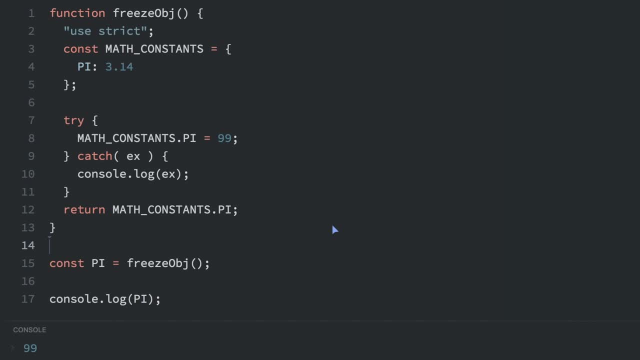 freeze that will prevent data mutation. So let me talk to you about object dot freeze. First of all, let's understand this function here. We're using this function to demonstrate object dot freeze, So it's going to create this constant- math constants- with a pie in it. This is an 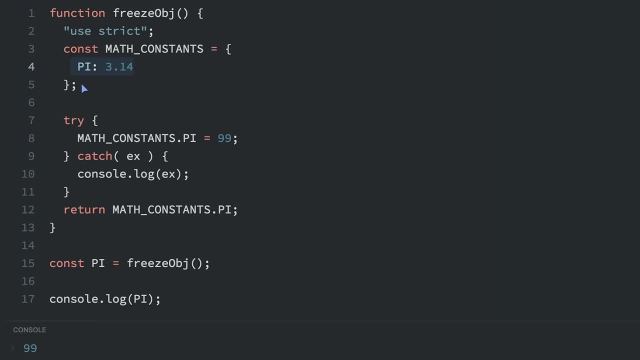 object And right now this can still be changed. So if we look down here, this is a try catch block. We'll talk about try catch blocks in more detail later, But for now you just have to know that it's going to try what's in. 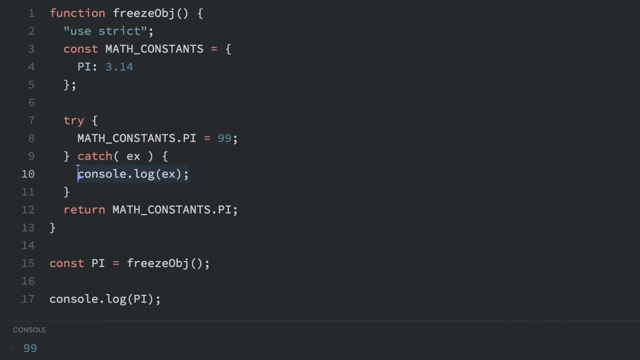 the first part of the block And if there's an error then it's going to go into the catch block part and it's going to log it out. So right now we're going to try to change math constants, dot, pi to. 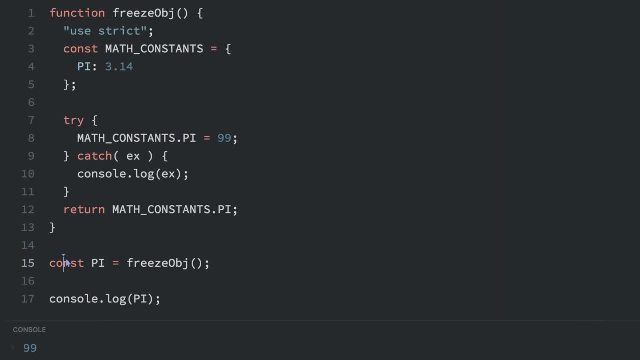 99. And if you can see, right here we're going to return the math dot constants, dot, pi, And down here we are putting into a variable called pi. So if we run this you'll see that we console dot log time is 99.. But wait a. 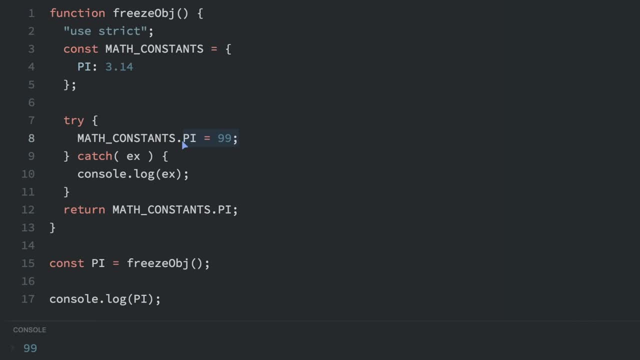 second, we don't want pi to change, Because we know that pi never changes. That's why we're going to use object dot freeze. So I'll put it right here: I'm going to do object dot freeze And then, in parentheses, I'll put the object, which is math constants. Now I frozen math. 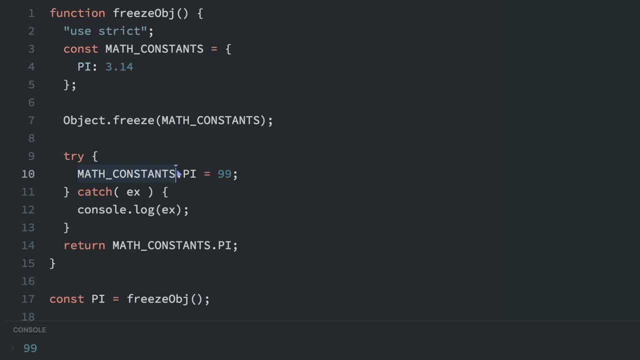 constants. So when it tries to change math constants, dot, pi here it's not going to work And it's going to go into this catch block And it's going to log out the air or the exception. So let me run that And you'll see. type air cannot assign to read. 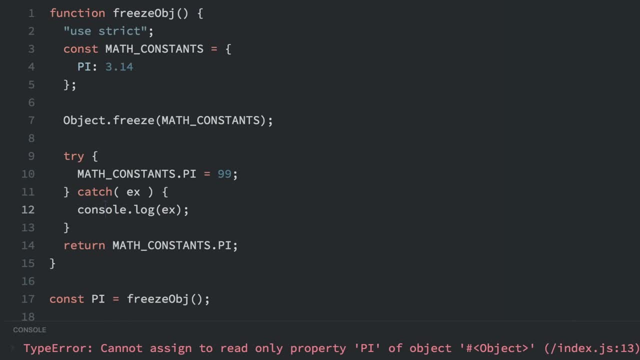 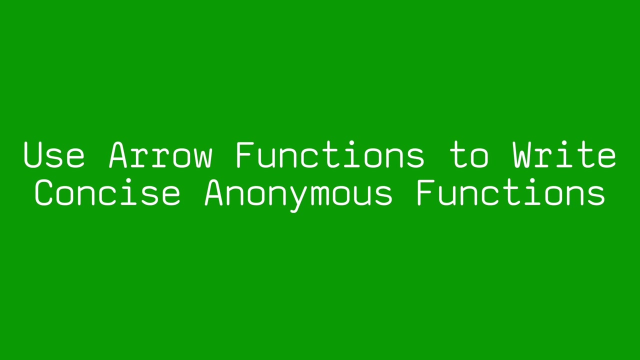 only property of pi of object. So we had an error And we can see here that pi is stays the same at 3.14.. So whenever you have an object and you don't want any of the items in the object to change, use object dot freeze. This function here is. 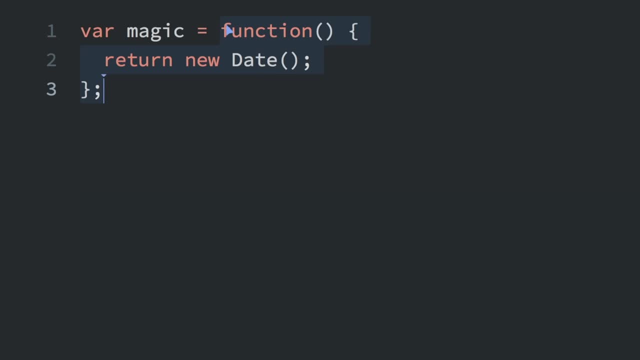 called an anonymous function. it doesn't have a name. it is assigned to this variable magic, But there's no word right before the function keyword to assign the name to the function. Whenever you have an anonymous function, you can convert it into an. 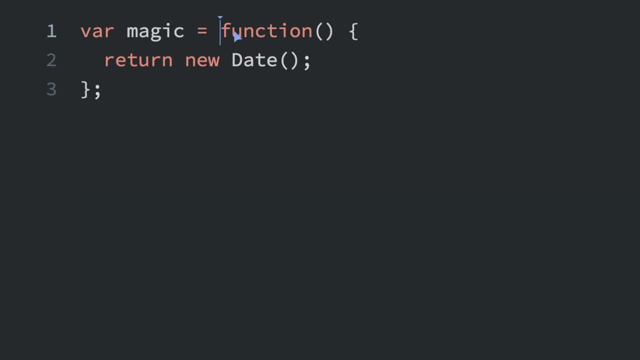 arrow function. That makes it a little quicker to write. So instead of the word function, I'm going to take that out completely and then put an arrow here. So this is the same thing, Except it's just a little quicker to write. But we can shorten this even more If we're just returning one value here, we don't even 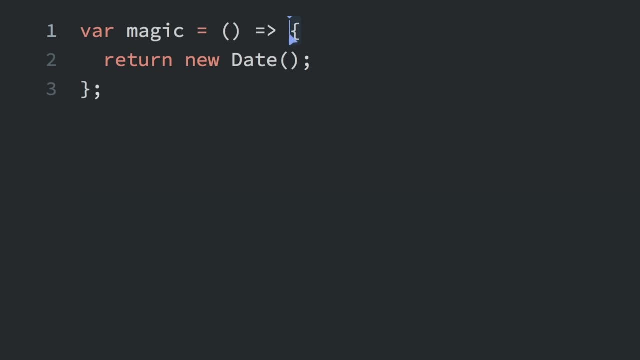 need the return keyword And we don't need the curly braces. So I can delete all this, And I can delete all this here And now. this is the full function from before, but it's just really shortened up. And to make this even nicer, we're not going to use var, I'm going 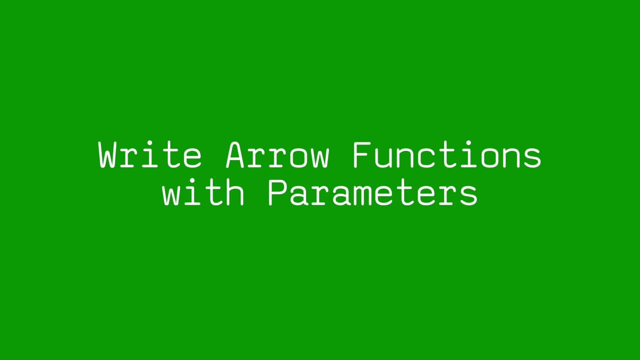 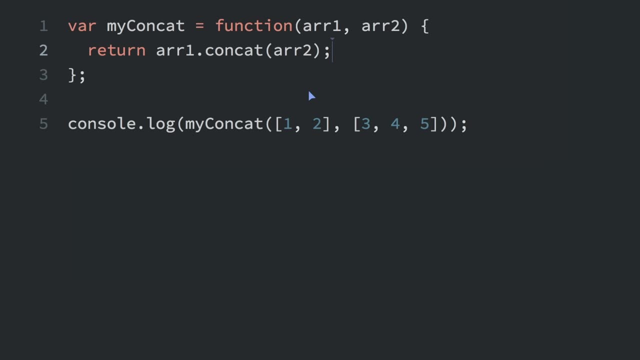 to change this to const, And so we're going to change it to const, And I'm going to change it here, And then we're going to remove this and change it to const. Just like in a normal function, you can pass arguments to arrow functions, So let me show you how to convert this function into an. 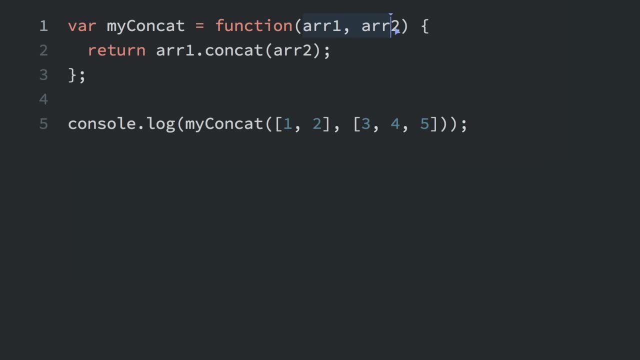 arrow function. So it's a normal function now and it has two arguments, And then it's going to concatenate the two arrays passed in. So first we'll take off the function keyword. we're going to leave these parentheses with the parameters. Now put the arrow. 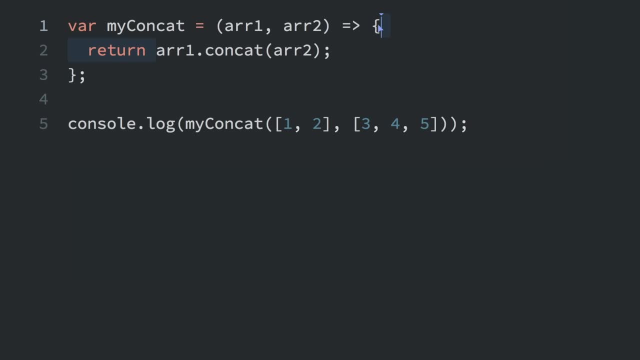 since all we're doing is returning, return this- we don't even need the return keyword and we don't need the curly braces, So I'll take that off, we'll take this off. And now we've done this. I just converted that function into an arrow. 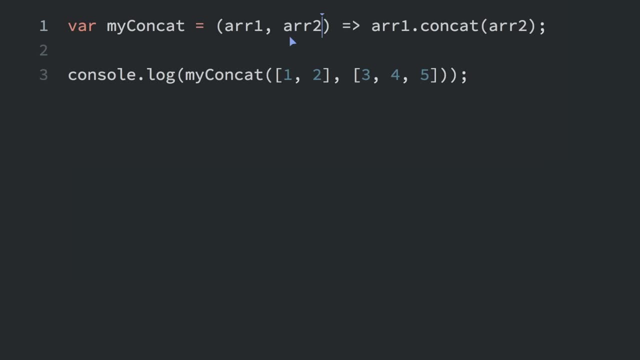 function And it has these two parameters. So we just have the parameters in parentheses, we have the arrow and then we have what's being returned right after the arrow. So if I run that, you'll see that we concatenate the two arrays that are passed in in this example And then for good. 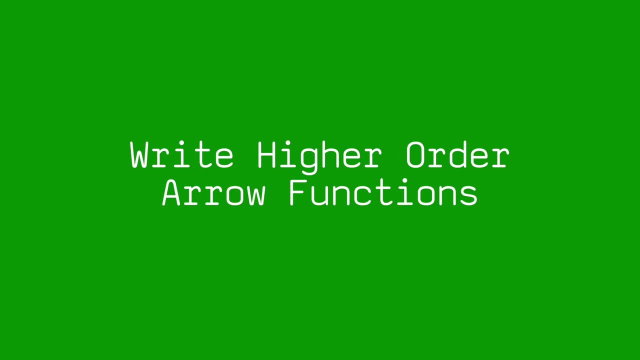 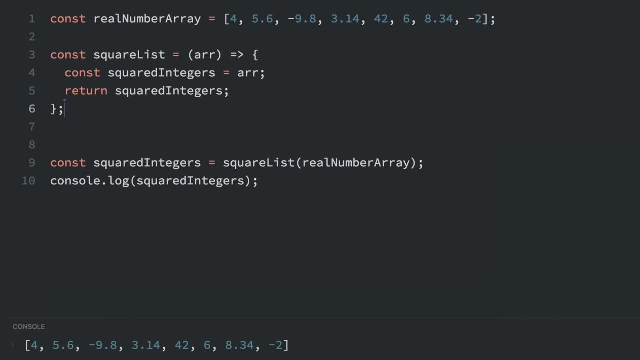 measure. we'll change this to const. arrow functions work really well with higher order functions such as map filter and reduce. I'll go into more detail at a different time about map filter and reduce, But the main thing to know is that they take functions as arguments for. 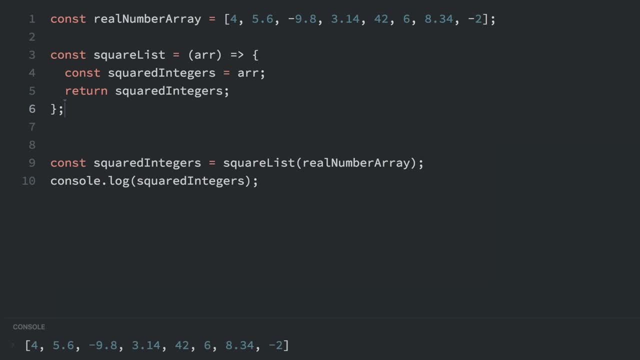 processing collections of data. Whenever one function takes another function as an argument, that's a good time for an arrow function. So what we're going to do here is we're going to update this function right here. we want to compute the square of only the positive integers in the array, So it's pass in this array. 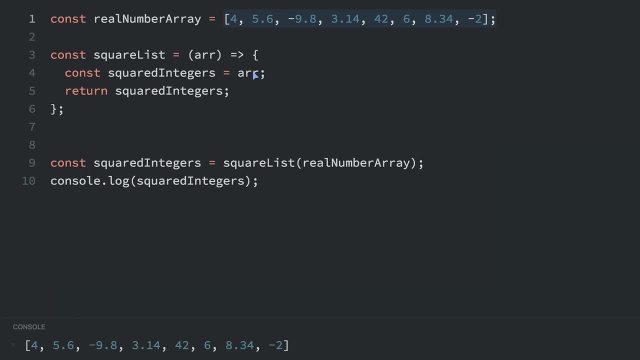 which is this: and we want to filter out everything that's not a positive integer. So I'm going to use the filter and map functions to do that, But the main thing I want you to look at is the arrow functions that I'm passing into filter and map. this line is going to be a lot more succinct. 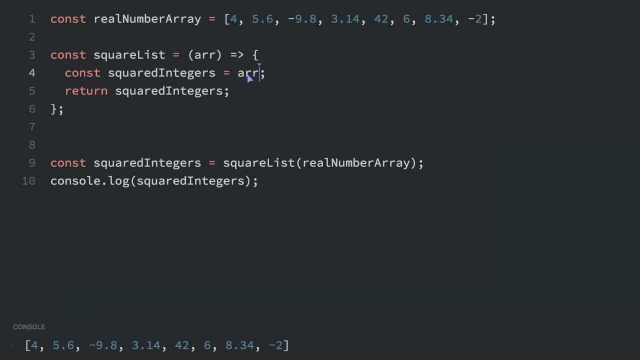 because of the arrow functions. So we have the squared integers is going to be the RR And we're going to filter this. so dot filter. Now again, I'm not really going to explain in detail what the filter function does, But that will be something for another time. Just look at this. 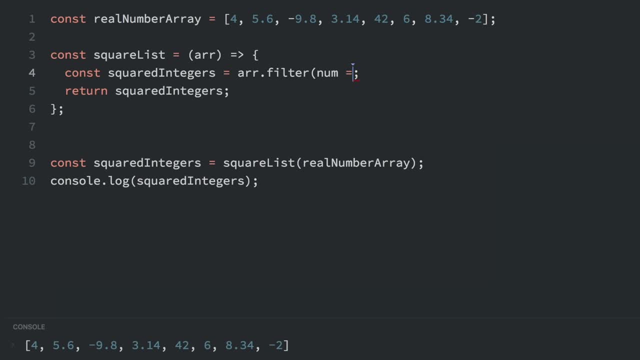 arrow function. we're going to create this arrow function by starting it just like this. Now I'm going to do a little bit more review because the wife of the arrow function is going to show you how to do that. So, as I mentioned before, I showed you that you pass in arguments and parentheses for 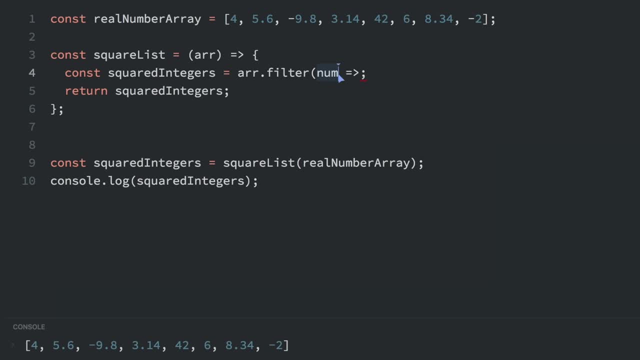 an arrow function. But if you only have a single argument like this- the number argument- you don't need parentheses around the argument. you can just put the argument and then the arrow. So this is the beginning of the arrow function, And then we'll see what's returned from the arrow function. First we 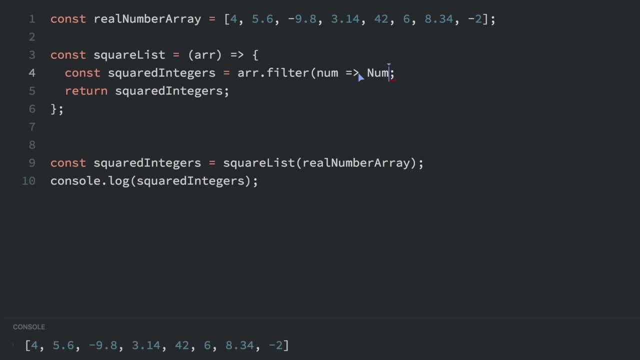 want to filter this array, So we. So we'll do. number dot is integer, And then we will pass in the number and number is more than zero. So let me complete the parentheses here Now. the result of this filter command will be an array with all the numbers that are more than zero and also integers, So that would be 442.. And 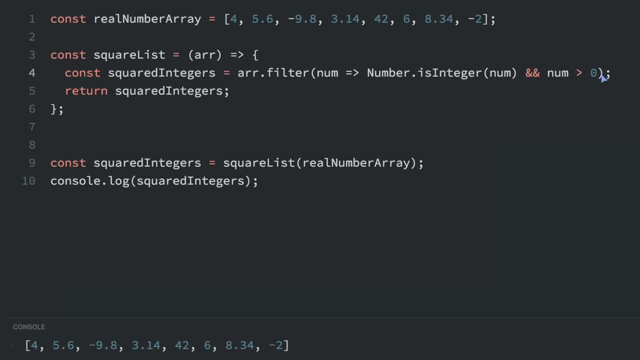 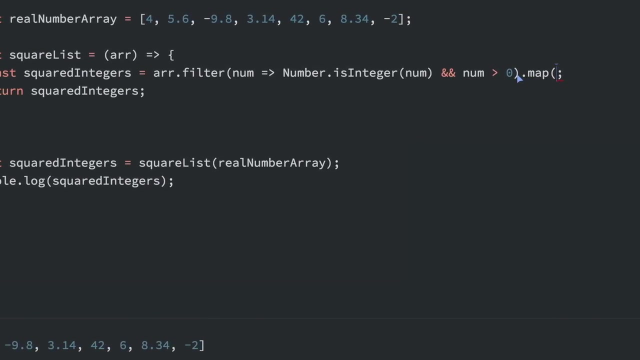 six. But after we get that new array, we want to get the square of each number in that array. So that's where we're going to use the map function. Now, the map function takes a function as its argument, But instead of writing a full function, 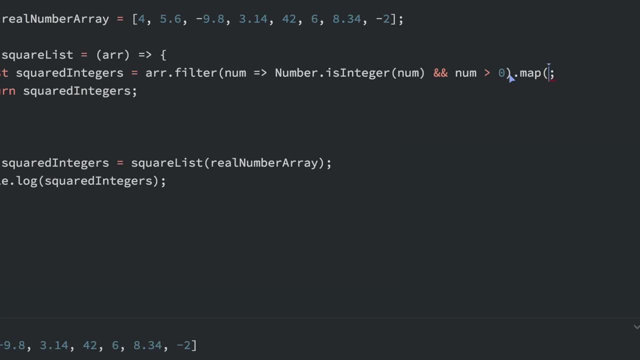 out. we can use an arrow function. So we're going to pass in x to the function And then there's gonna be an arrow function. Now x just means every element from the array that's being passed to it. So remember, the map is getting the array for 42, six. x means for every element in. 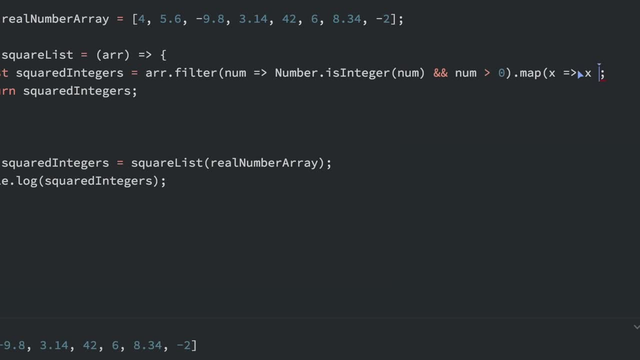 the array. this is what we're going to do to it: x times x, because it's going to be squared. Okay again, the main point of this lesson is not to understand the filter and map functions, But to see that we can put an arrow function, we can pass in an arrow function And it makes it so we can. 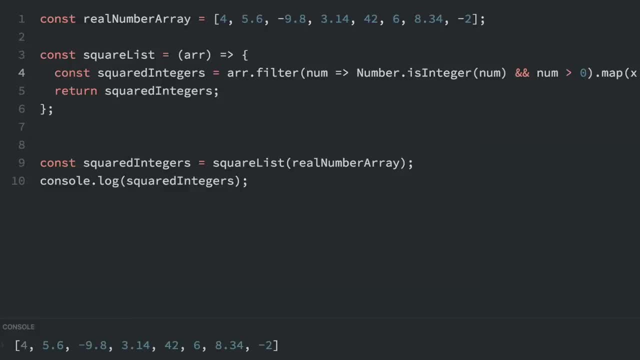 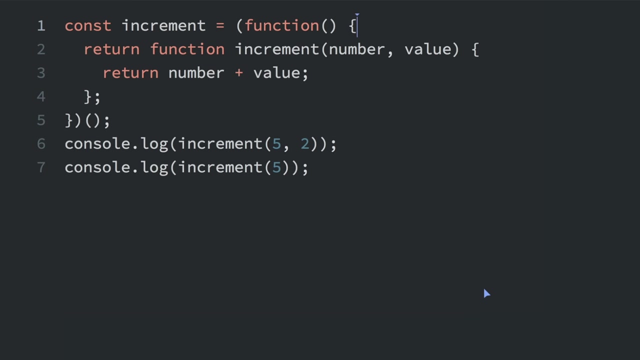 fit everything really succinctly on one line, So let's reload this and see if it works. Now we have 16, 1764 and 36.. In order to create more flexible functions, you can use default parameters. The default parameter kicks in when the argument is not specified or is. 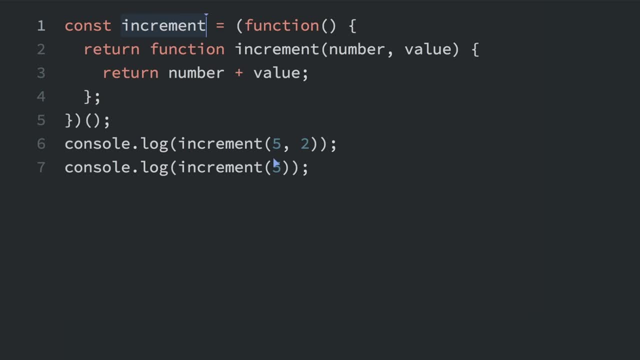 undefined. So, for instance, with this increment function, we want to change it. we want to change the increment function. So you can pass in two arguments- the five and two- to increment by two, Or you can just pass in the one argument, the five, if you want to. 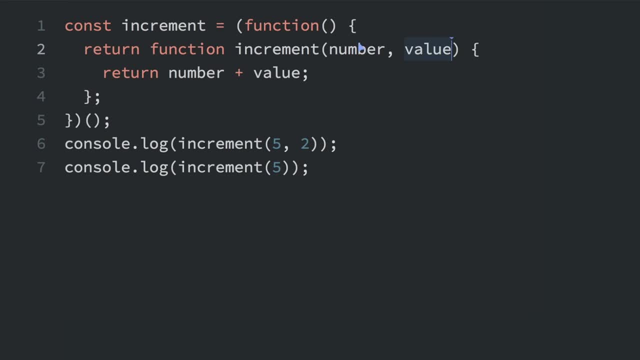 increment by one. So here are the numbers. we're passing in a number and a value, So we just have to Put: value equals one. So now, if a value isn't passed in, it will be set to one automatically. But if it is passed in, 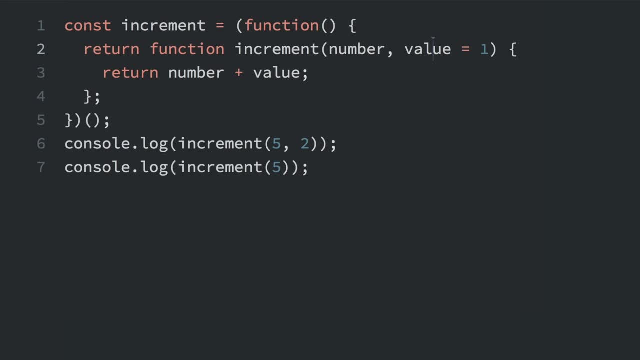 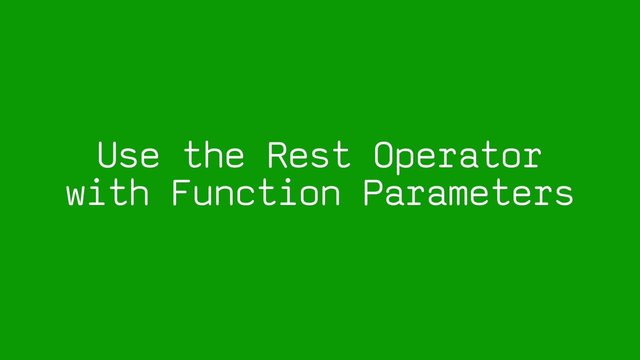 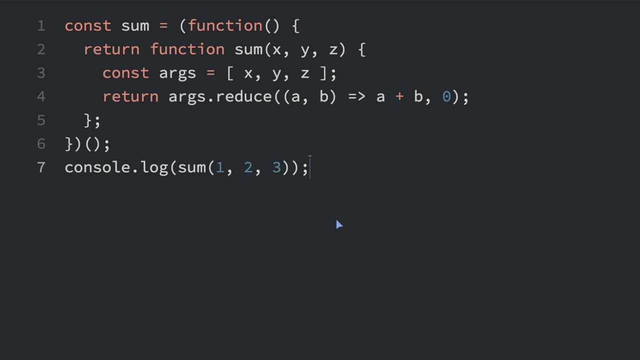 it will be set to whatever is passed in. So if we run this we can look on the console. we have seven for this first one and six for the second. The rest operator allows you to create a function that takes a variable number of arguments. The rest operator is three dots, So we have this. 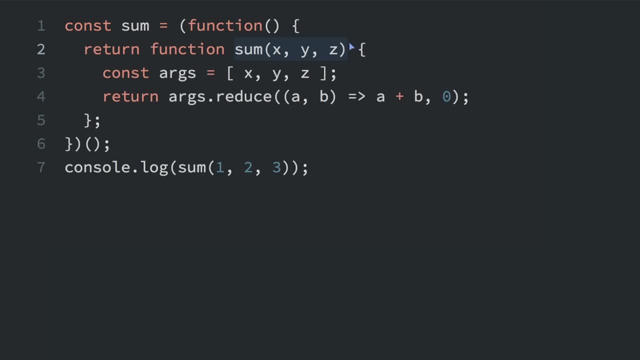 function here And it's taking three arguments- x, y and z- and it's summing them. So at first it's converting these x, y, z into an array called args, And then it's reducing them, So it's summing. 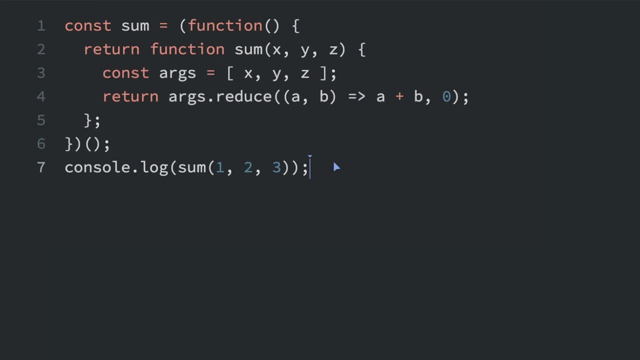 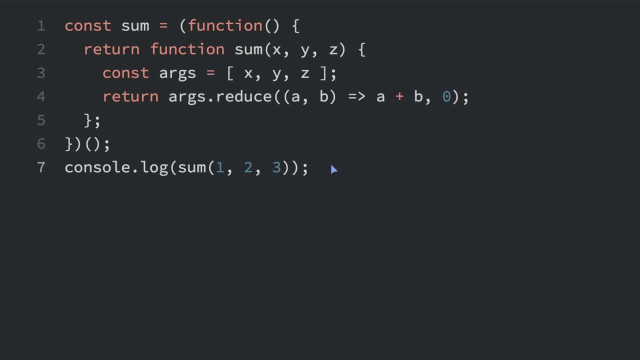 take the sum of the arguments. And then it's going to take the sum of the arguments Because one plus two plus three is six. we can change this to use the rest operator. So we're still going to pass in 123. But where it's accepted here, where we have the arguments here, x, y, z, I'm just going. 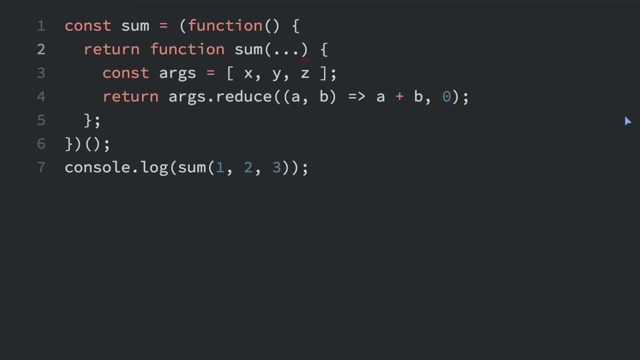 to put dot dot dot. that's the rest operator, just dot dot dot, and I'm going to put args. So with this rest operator dot dot dot, it will convert everything that's passed in into one array and the array is called args. So now we don't need this anymore And it should work the same. 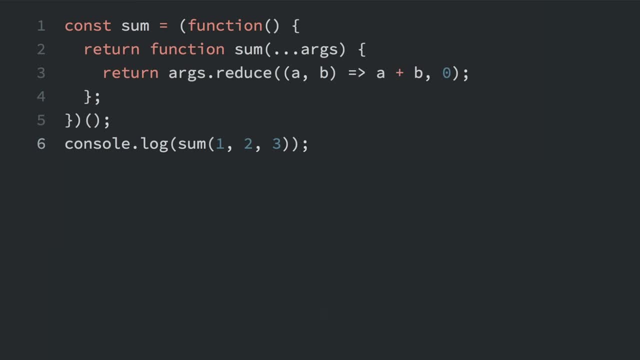 If we run this we'll get six, But we can also now add any number of numbers. So I'll put a four on the end and 10, it's going to add those numbers together. So before we can only pass in three arguments And now we can have any number of arguments. The spread of arguments. 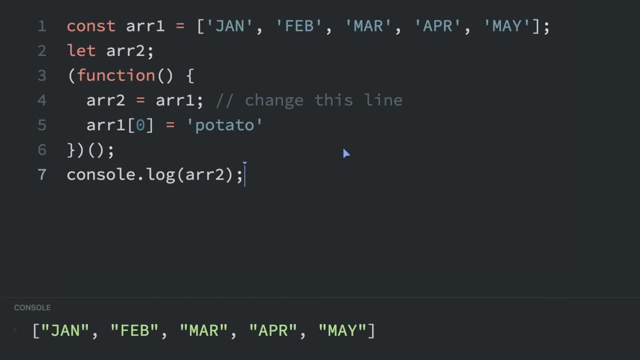 operator looks just like the rest operator- three dots- but it expands in already existing array or it spreads out an array. So it takes an array and spreads out into its individual parts. So here we have an array with some months and the spread operator can spread this array. this are one into: 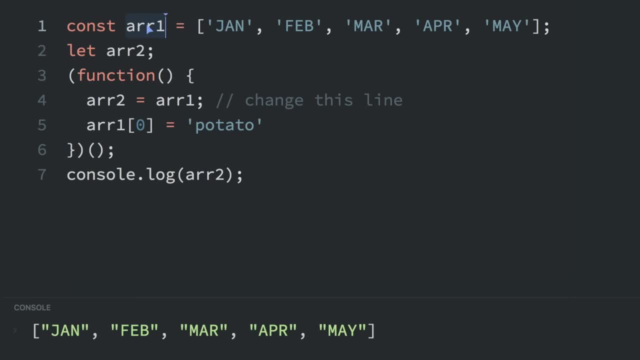 the individual months instead of the actual array here. you can only use it in an argument to a function or in an array of literal. So let's look at this. So right now we're setting array two to equal array one In this example. we're not actually copying it. 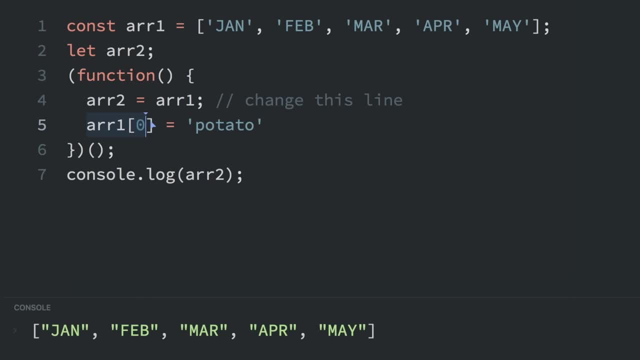 Because if we change array one, if we set the index of array one to potato and we log array two, you'll see that index zero is potato, even though we're logging array two and we only change array one because these are equal: array two and array one are the same. but what if we want array? 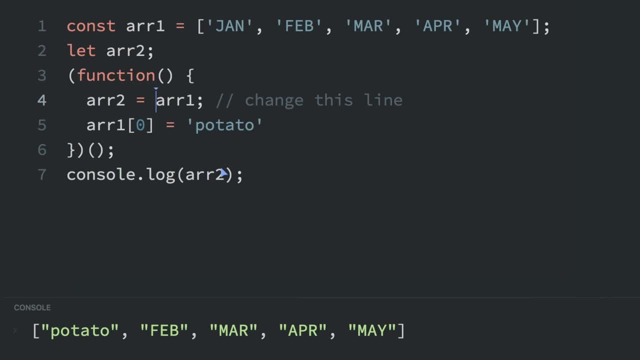 two to be a copy of array one, we can use the spread operator. Now, we can't just use the spread operator like this. that's not going to work. But if we put this inside brackets, which is an array, it will spread out the contents of array one into this new array. So we're not making array two. 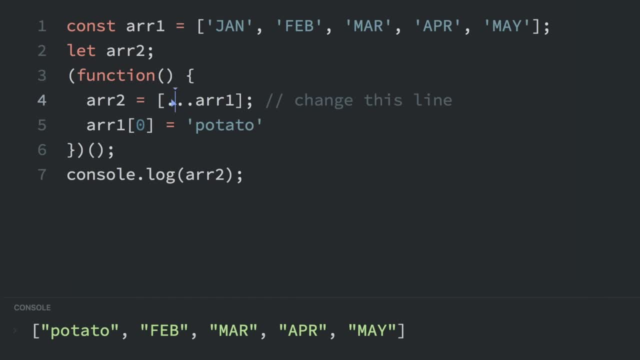 equal array one. we're we are making array two equal array one, And then we're going to create an array two. we're not making array two equal array one. we're not making array two equal array one, array to equal all of the contents of array one. So there'll be different. So if we run this again, 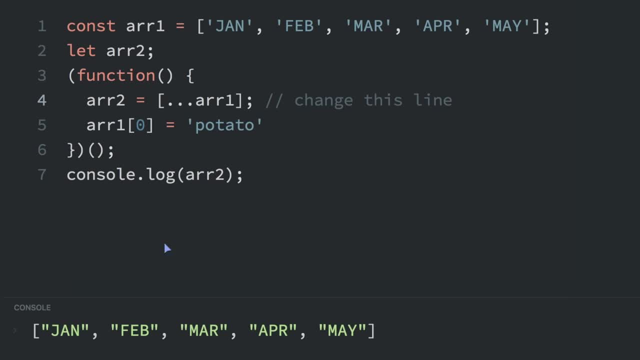 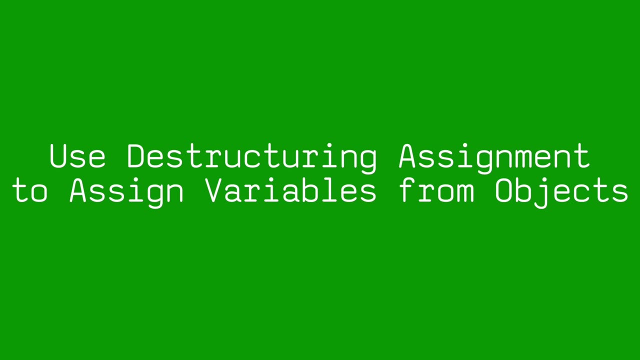 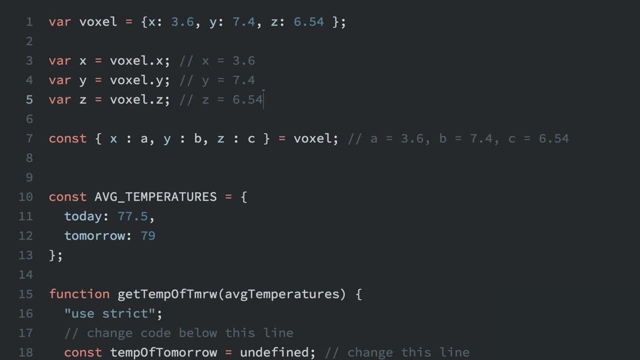 you'll see that it says January for the first element in the array instead of potato. The next few lessons will be about the structuring assignment. This is a special syntax for neatly assigning values taken directly from an object to a variable. So look at this. 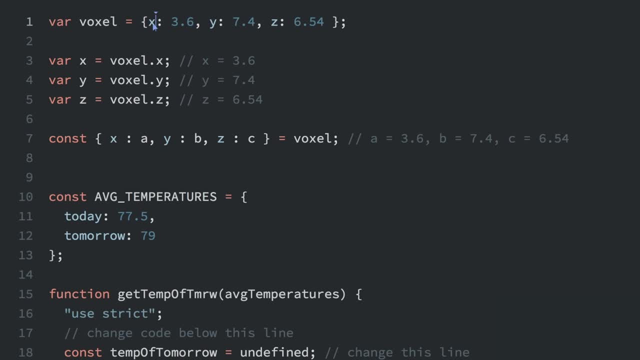 object. here we have this object with three elements. we have the x, y and z with their values, And it's all in the voxel variable. So if we want to take each individual element in this object and assign it to its own variable, this is the old way of doing it, So you could do voxel. 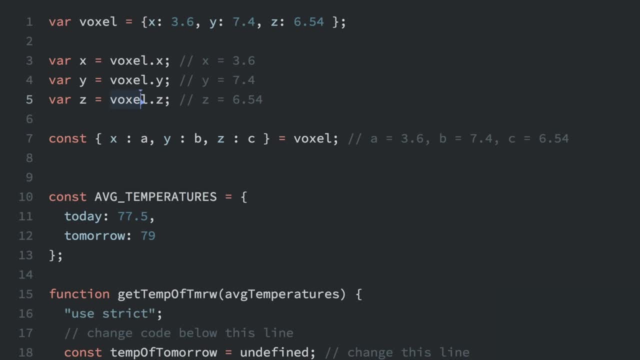 dot x: the stores x box without y stores y box without z: the store z. Now, with with destructuring, there's a simpler and quicker way to assign variables for each element in an object. So here's the destructuring syntax, right here. This time we are creating variables A, B and C and assigning 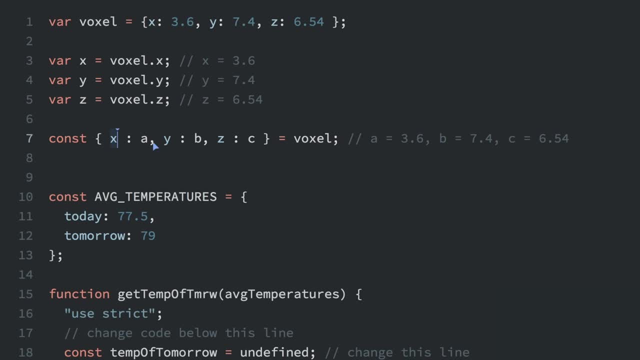 them to the values from the object x, y and z. we can see we put in curly braces here and we just say: equals the object, equals voxel. You can read it like this: get the field of x and copy into the value a. So get the field of x from the object, copy into the value. 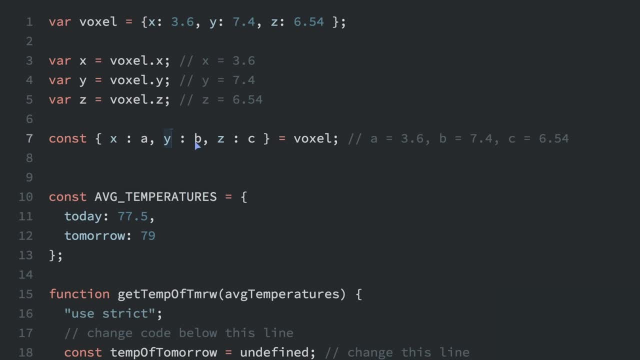 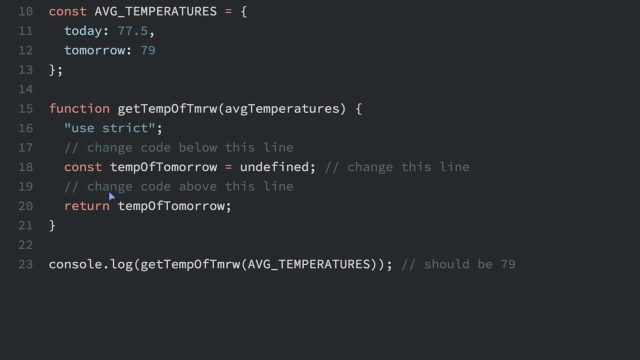 a: get the field of y from the object copy to the value B. get the field of Z: copy into the value C. So this is just a quicker way of assigning things from an object into variables. Now we're going to use destructuring to obtain the average temperature for tomorrow from the input. object: average temperatures. So we have average temperatures, app values and score. We call this variable And we're going to make a shorescale from the object and we're going to muster it up And then on the Y axis we're going to get 0. And the company will have an inverseDIY으로 and 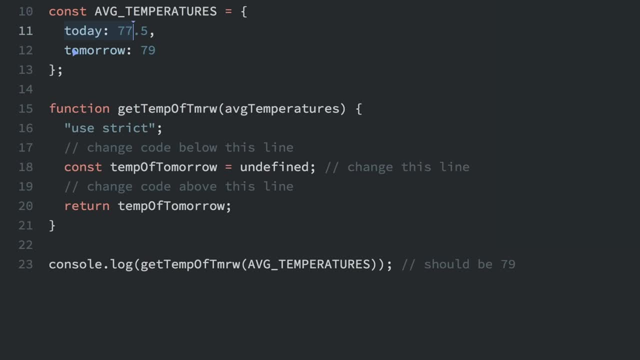 then we're going to hash out these values on the mod controller, So we're going to copy it into the value Plummer. we have average temperatures. it has today and tomorrow's temperatures, and then the average temperature is inputted into this function here. so i'm going to change this line here. 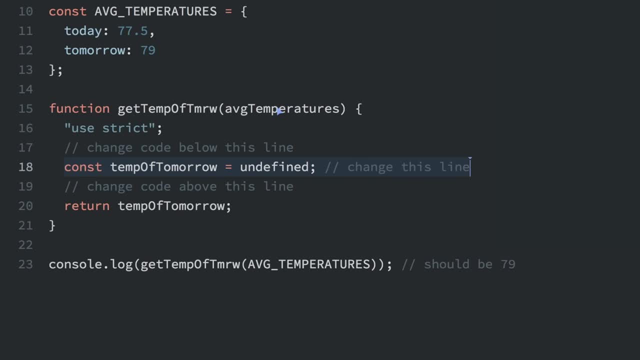 to use destructuring and destructure the average temperatures object here. that's passed into this function. so first i'm just going to put the average temperatures variable here and then on this side of the equal sign i'm going to have to use the destructuring. so i'll put the curly braces. 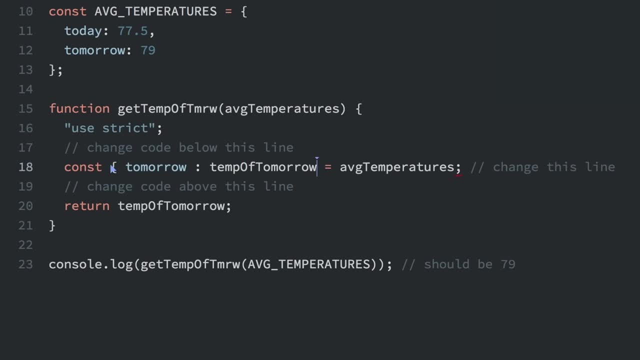 and we'll put tomorrow in the colon and then the other curly brace. so this is saying: get the tomorrow field from the average temperatures object and assign it to the temp of tomorrow variable. so if we run this we should see it says 79 in the console because we got the temp of tomorrow variable. we return temp of. 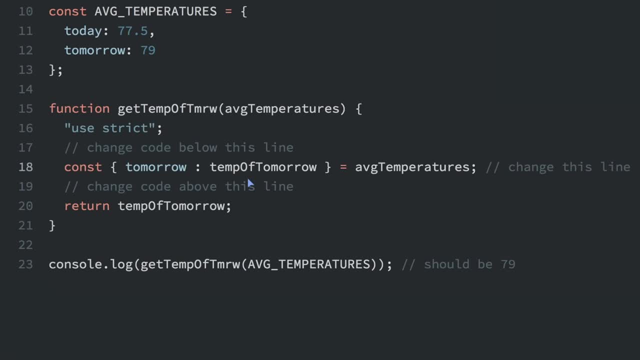 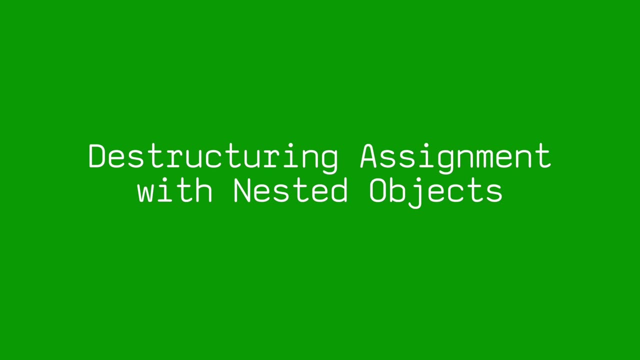 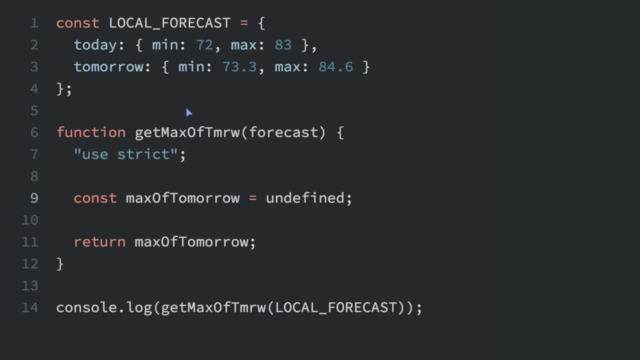 tomorrow and it was logged right here. so we successfully used the structuring to get the tomorrow variable out of average temperatures. we can also use the structuring assignment to assign variables from nested objects. we have this nested object right here, the local forecast. we have some nested objects, So we have the forecast from today and the forecast from. 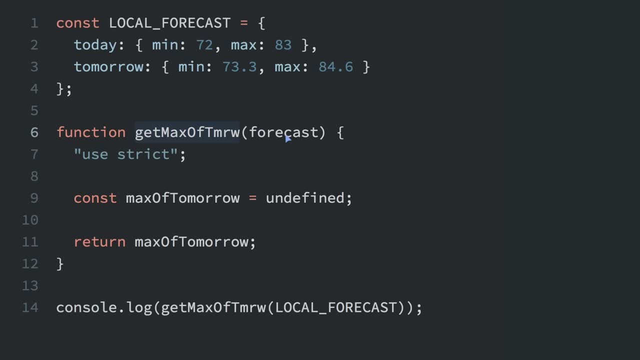 tomorrow. So here we have get max of tomorrow where we're going to pass in the forecast, And here we can see the local forecast becomes the forecast variable And we're trying to figure out the max of tomorrow. So we are going to use destructuring to figure that out. So it's going. 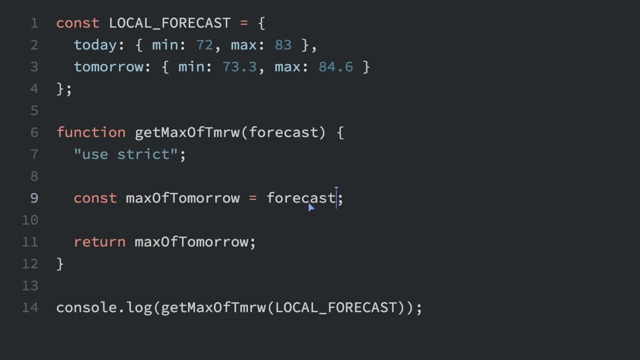 to equal forecast And remember that that is a nested object. So here when you're destructuring, you're always going to use the curly braces And we are first going to get tomorrow And on the other side of the colon we're going to have some more curly braces because it's nested. So we need 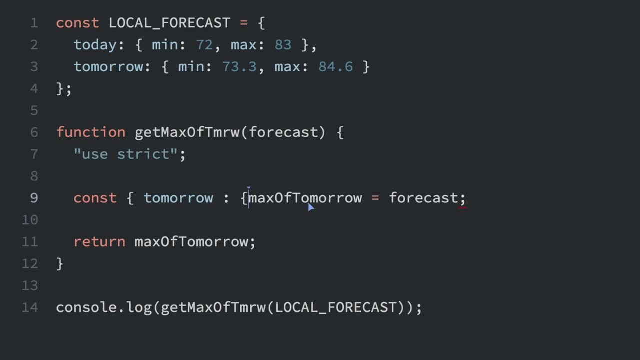 to go inside of the tomorrow object and we need the max. So we'll do max. And then we have the colon And max of tomorrow. Now we need two sets of squiggly braces here, So we have this one and this one, And so we've destructured two times And the variable is max of tomorrow. So we've set the. 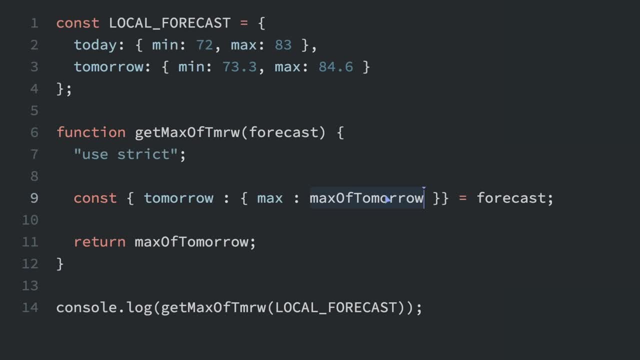 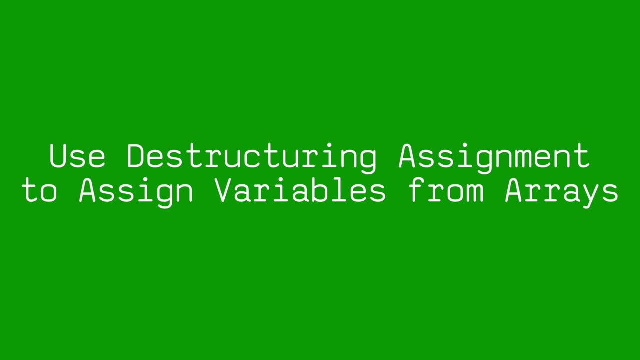 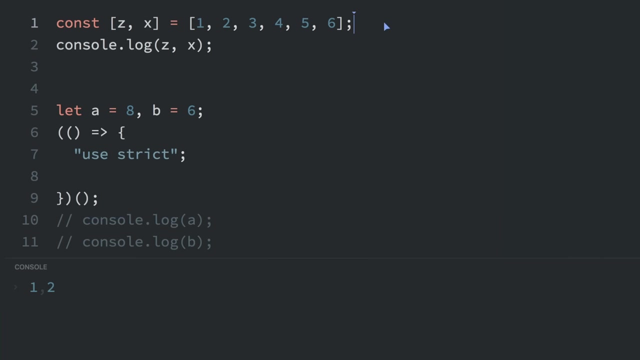 max that was inside tomorrow to max of tomorrow. So if I run this you'll see it's 84.6.. And you can use these structuring assignment to assign variables from arrays. Look at this example here. So we have this array of 123456.. And we're assigning the variable z and x to the first two. 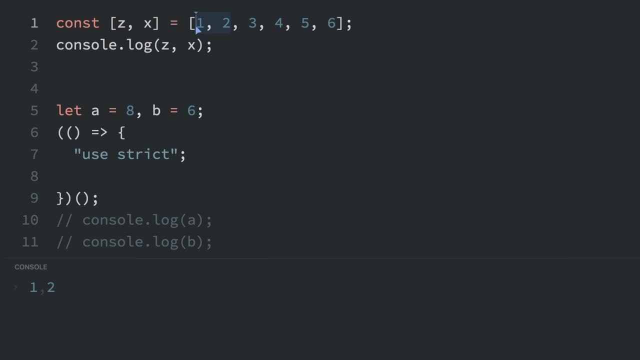 numbers of the array one and two. The difference between destructuring from arrays and destructuring from objects is that you cannot specify which element from the array to go into a variable. It's just goes in order. However, if we wanted number four to be go into a variable, we could just do. 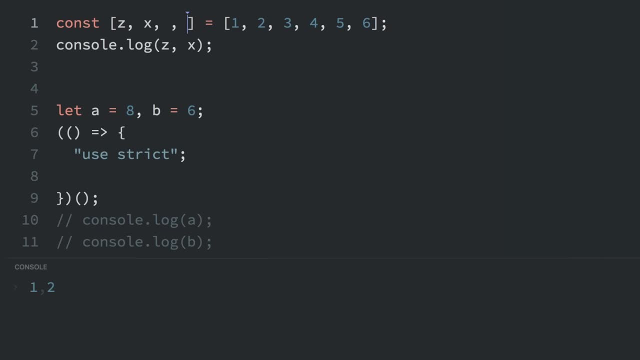 like this: we would just add some commas. So we put a comma with nothing in it, like that, two commas in a row, And I'll put a y here. So now we have the first element, the second element, we skip the third element and then we have the fourth element. So if I console dot log z, x and y, we should see. 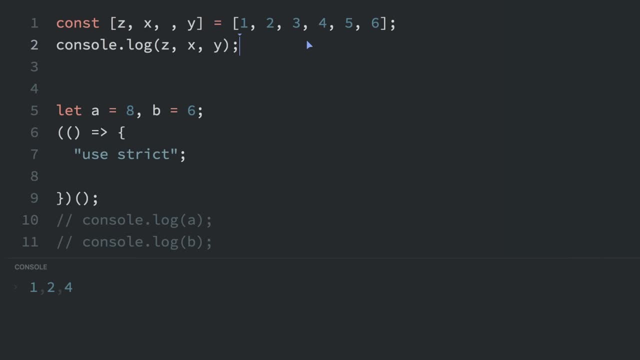 one, two and four. Here's another thing you can do. you can use destructuring of arrays to switch the places of variables. let me uncomment out these, And what I'm going to do is use destructuring to switch the places of a and b. So it'll be like this: I'll say a, b and I'll say equals. 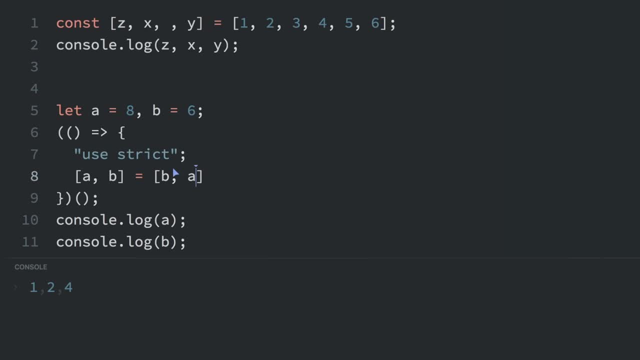 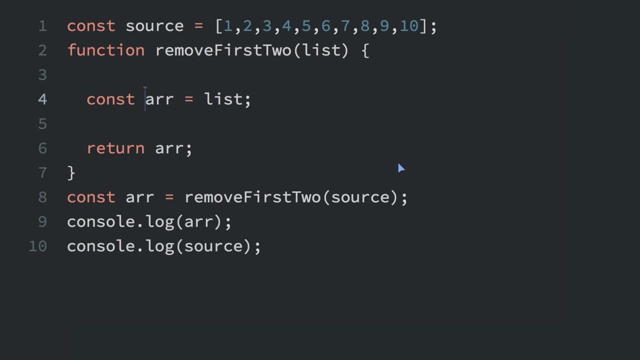 b, a. So now it's just taking this and switching the places. So instead of a being eight and b equals six, it's now going to log out six and eight. So let's see, Yep, it worked. We can use destructuring assignment with the rest operator to reassign array elements. we can see in: 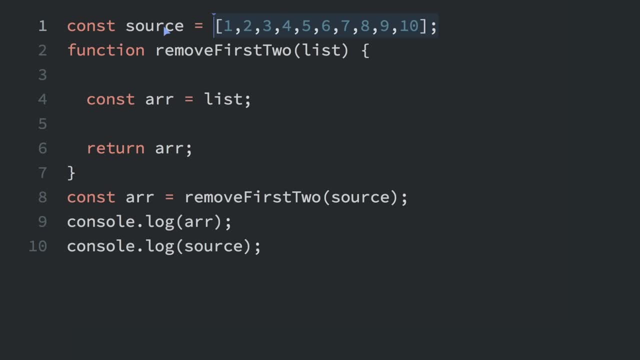 this example: we have this array, the digits one through 10, and the array, and we have this remove first to function. we're calling it here and we're passing in the source. that's the source array and it becomes the list. So we want to return the array with the first two elements. 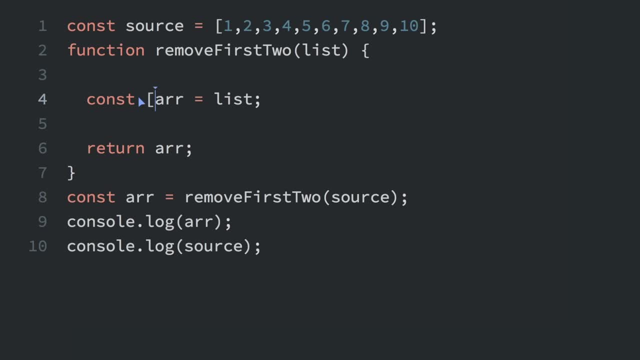 removed. So let's use the rest operator inside an array here. So we'll use the rest operator, the three little dots, And to remove the first two I just have to put two commas here with nothing in between them. It's saying: do nothing for the first element, do nothing for the second element, everything else. 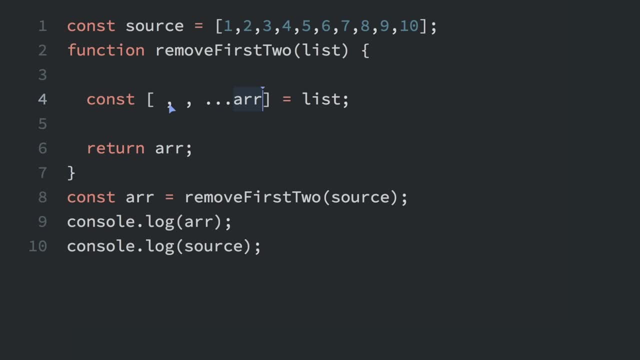 put into the our variable, we could have assigned the first two numbers in the array to two other variables. So I could do a, b, and then a would be one, B would be two And then our would be an array of 3456789, 10.. But right now we just need to return the array with the first two elements. 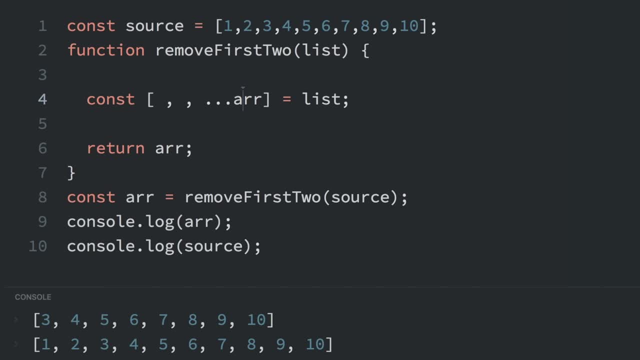 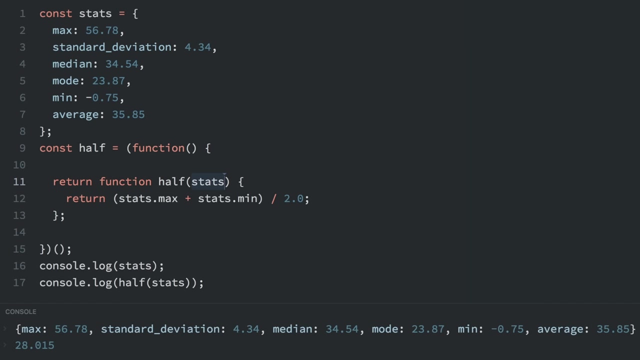 missing. If I run that, you'll see that we did that. If you look in the console, we've logged the array and the first two elements are missing And then we have the original array down here. You can use the structuring assignment to pass an object as a functions parameter. Let me show. 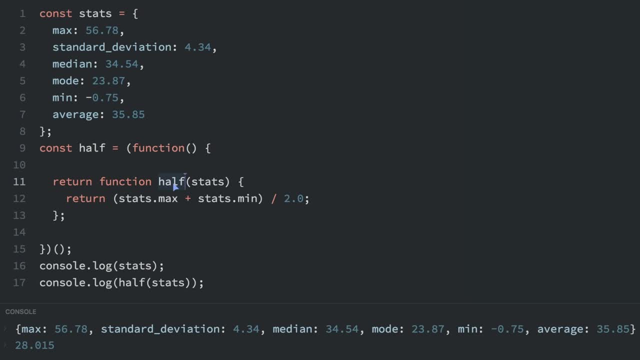 you what I mean. Right now we have this half function and it's getting the stats argument. So the stats is being passed when it's called down here And it's passing in this whole object, so this whole stats object. but you can see within this, 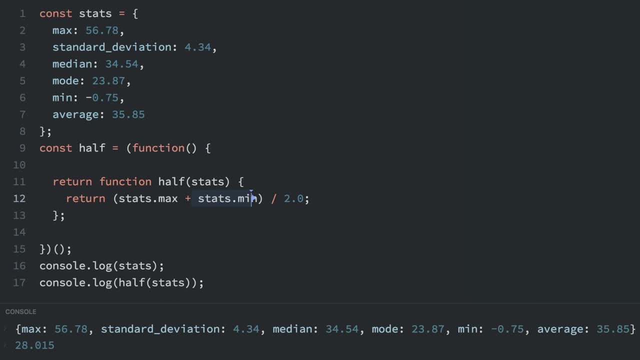 function. we're only using stats dot max and stats dot min. So instead of passing the entire stats into this function, we can just pass in what we need. So this is what we're going to do. I'm going to put in some curly braces here and just put Max and men. So now, when stats are in the 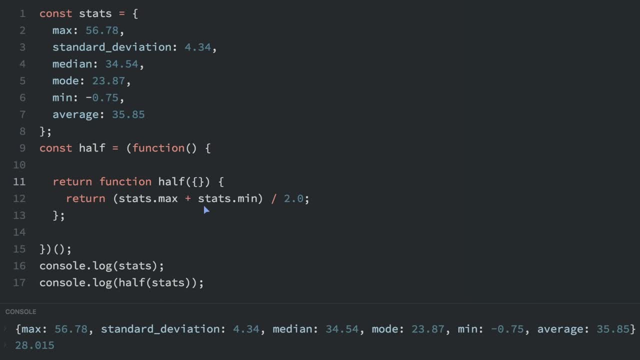 array. what I'm going to do is pass this function in a statement. I'm going to say it's fun, And right now we're giving him a new class from the original array. let's resent vá nap times S long. These are the nice things that happen when we're podem as a dimension of. we give him a duration. 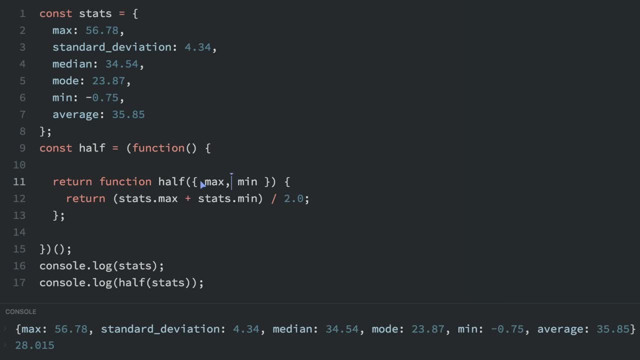 All right, guys, here's a different statement. Let's see if we can get rid of the particular array. So now, when stats get passed in, it's destructured into just the max and min variables, and the max and min from the function gets passed in. So now, instead of doing stats dot max, we can just do max. 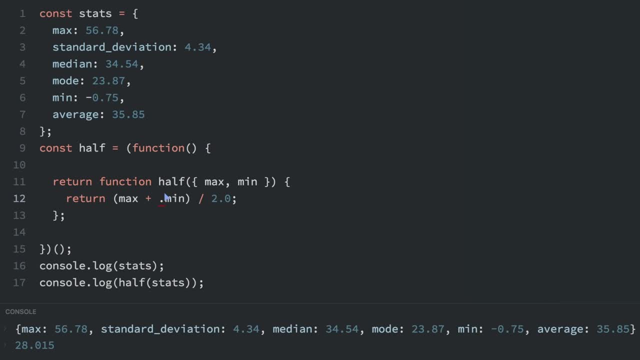 instead of stats dot min. we can do men. So if we reload that, it's going to work exactly like it did before, But now we only pass in what we need. This is commonly used with API calls. When you are getting information from an AJAX request or an API request, it will often have a lot more information. 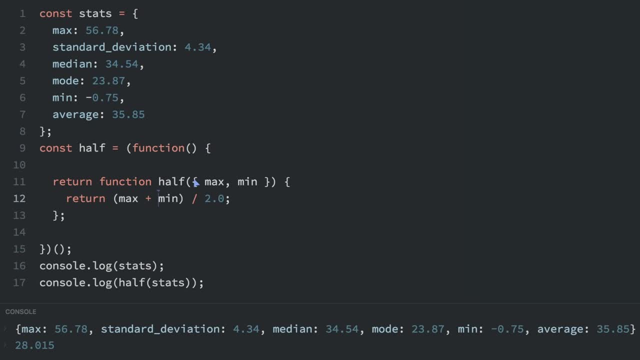 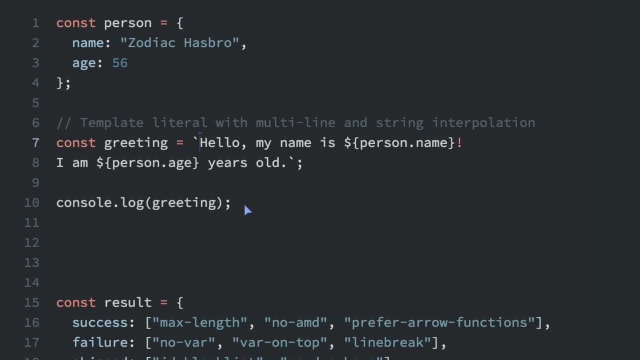 than what you need, And you can use destructuring to get it down to what we actually want to work with. Template literals are a special type of string that makes creating complex strings easier. You make them with this backtick. So here's an example of a template literal- right here. 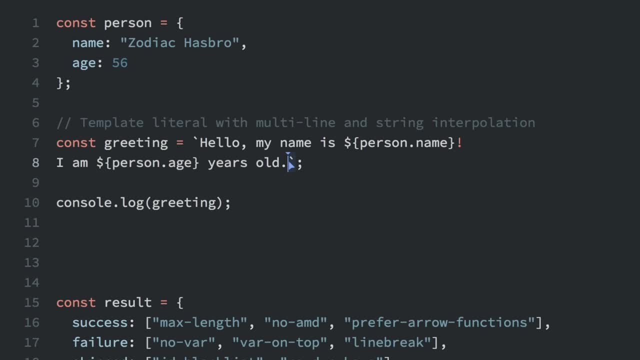 we have the beginning backtick and we have the ending backtick. this would be in place of using a quotation, a single or double quotation mark. A few advantages of using these template literals, these backticks instead of quotation marks, are one: you can make multi line strings. 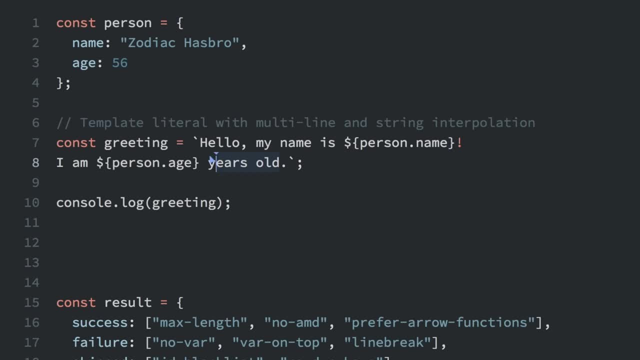 you can see this has two lines. here's the first line And here's the second line. And if we log the greeting, it's going to put the new line right in there. Another thing is you can add, quote single or double quotation marks right in the string and you don't have 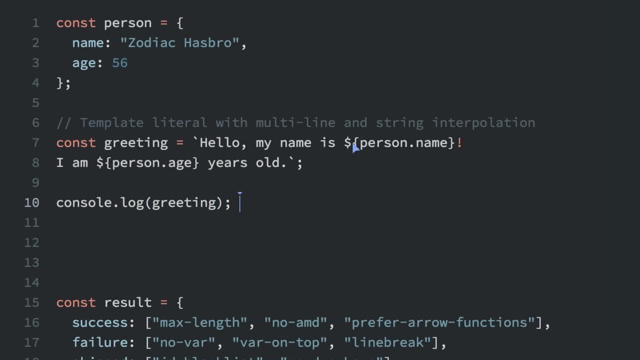 to escape them. The third thing is you can put variables right in the string. So if we see this, see the dollar sign, and then we have these curly braces, And so anything in between these curly braces that start with the dollar sign is JavaScript, And then we have these curly braces. 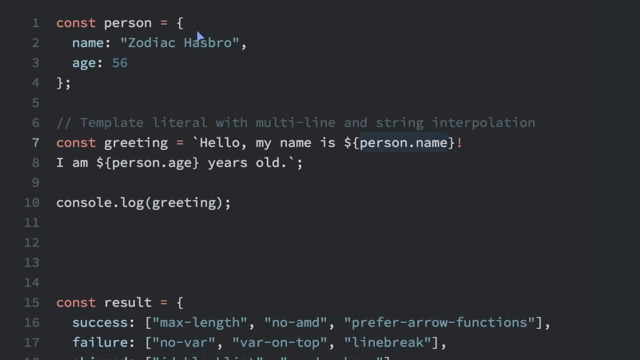 So right now we just have this variable person dot name which gets the name from up here, And then here we have person that age which gets the age from right there. So it makes things easier that you can put variables right in the strings. So if we run that you'll see. Hello, my name is. 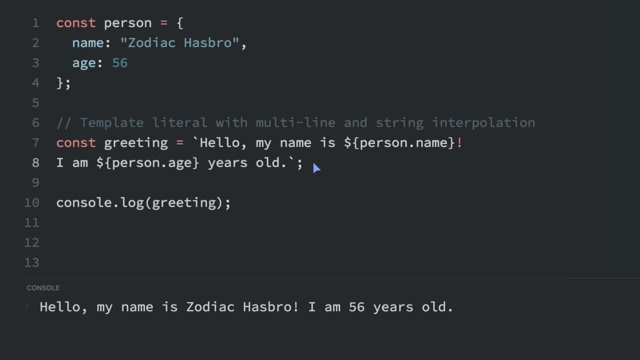 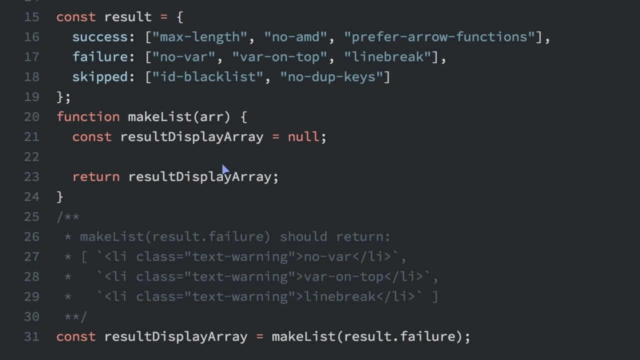 Zodiac Hasbro. I am 56 years old And normally it would actually also be printed with a new line. But with this exact code, editor and console doesn't show the new line, So there's gonna be a coding challenge that we're going to do right down here. we have this make. 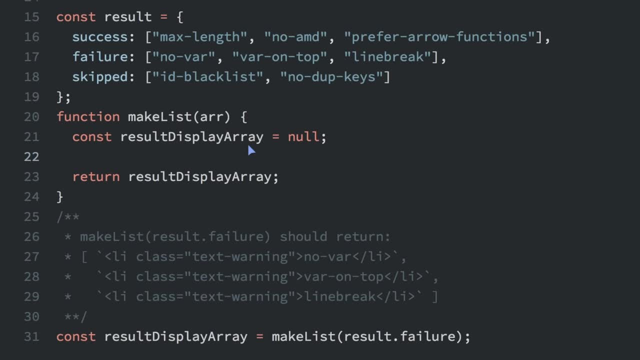 list function And we want it to create a list based on the array that's passed in. So when we call make lists, we pass in result that failure. well, here's the result. result that failure is this array here, And we want it to return an array that looks like this: Each element in the array is: 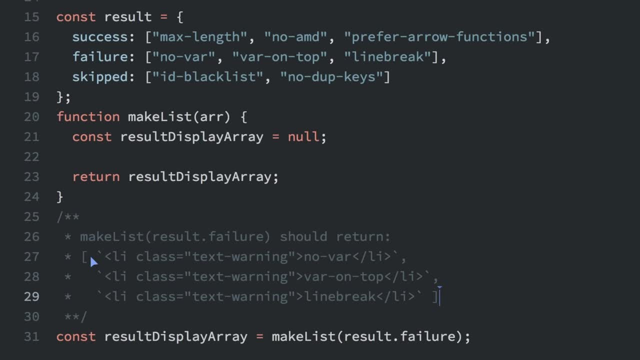 a template literal That has some HTML in it And then it also has this no var, var on top and line break. that comes right from this array that's passed in. So let's use template literal So create that. So, instead of setting this to equal null, I'm going to start this off to be an empty array. Now there's many. 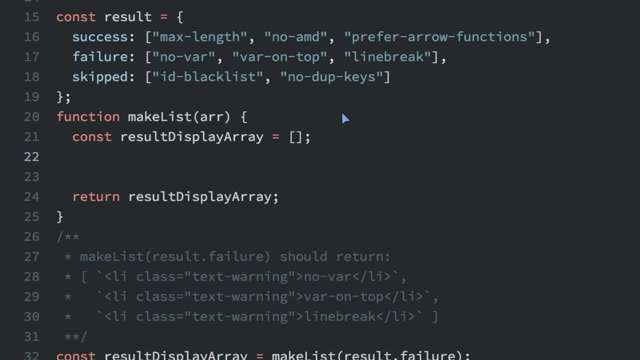 ways to do this, but I'm going to use the classic for loop. So we'll do four And then we're going to create an array And hopefully you remember how to make a for loop. we'll do. let i equal zero While. 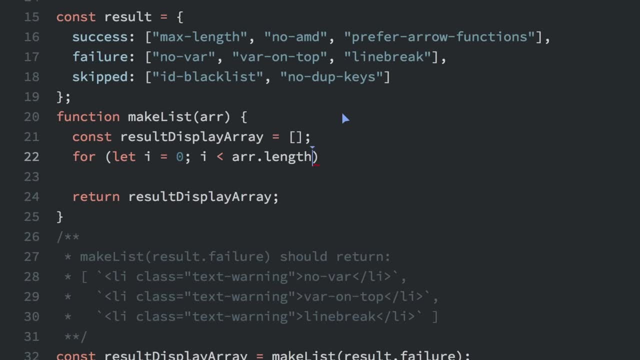 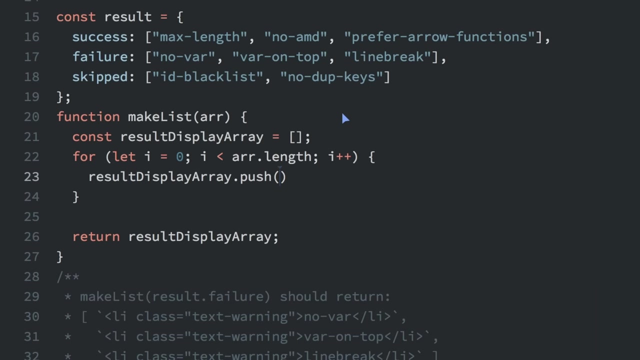 i is less than r dot length, And then at the end we will increment I. So inside this for loop we'll do result display, array, dot push. And then here's where I'm going to use the template: literal put a. 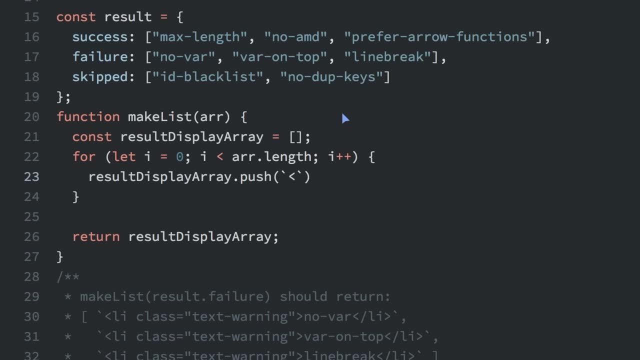 back tick. I'll put this HTML code here: li class equals text warning. And now this next part is going to be a variable because it changes for each array element here. So I'm going to do dollar sign and then the curly braces, And now I can just do our, and then at index, I now in the curly brace and then I can. 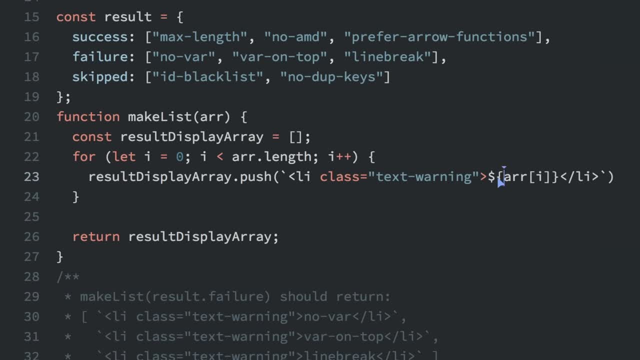 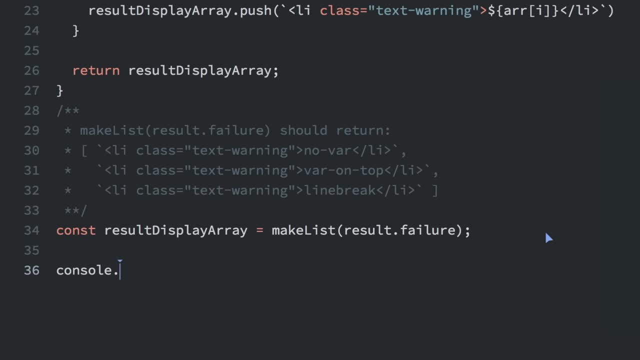 just put the slash Li: Okay. And if we console dot log this out because we just finished that video console dot log result to display array, the array looks just like it's supposed to be. if you look in the consolelog result, the array looks just like it's supposed to be. if you look in the consolelog. 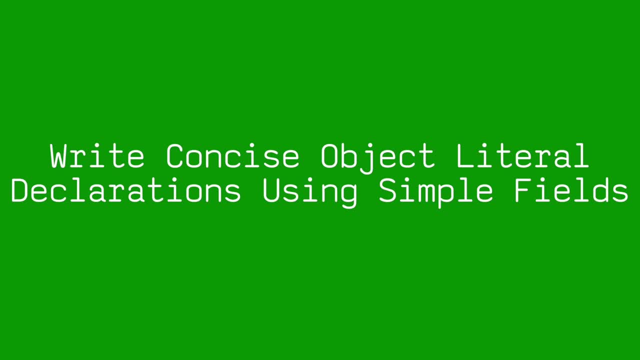 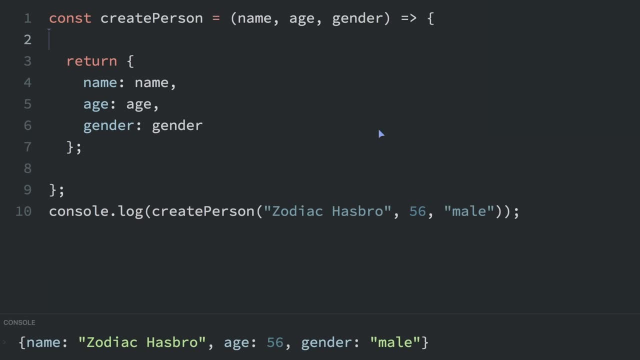 result to display array. the array looks just like it's supposed to be. if you look in the consolelog console it returns correctly. Yes, six added some nice support for easily defining object literals. If we look at this function here, this function is an arrow function. it takes in three variables: name, age and gender- And it's 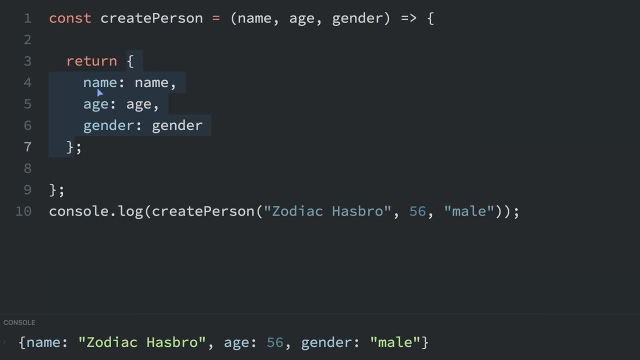 going to return an object And the object is going to have a series of key value pairs where the key is the name, age and gender, And the values are the past in variable names, the past in names, age and gender. So if you look in the console you can see what this currently does. We did the create person. 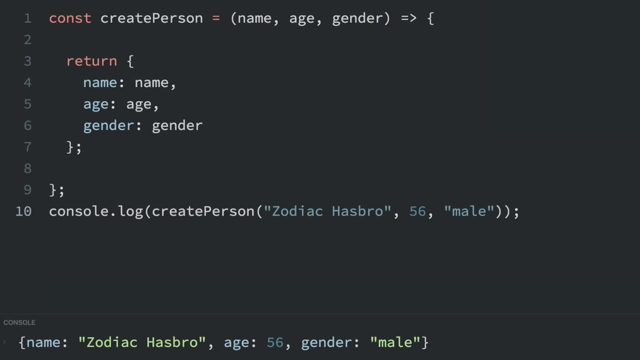 we pass a name, age and gender And you can see in the console. the object is name and Zodiac Hasbro, age 56. gender: male. So you can see there's some repetition. we're repeating name, name, age, age. 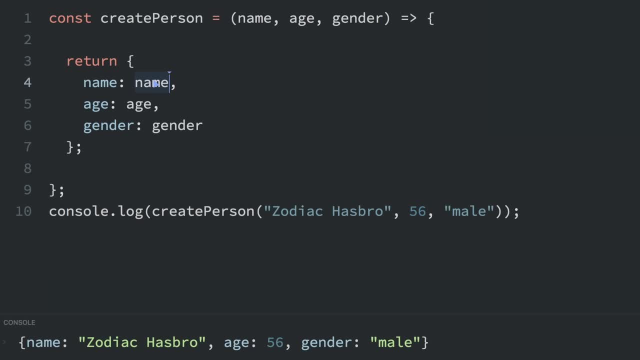 gender, gender. Now the first name- age, gender and gender, And then the second name- age, age, gender- is the key And the second name is the value. But there's a way to just make this simpler, If you. 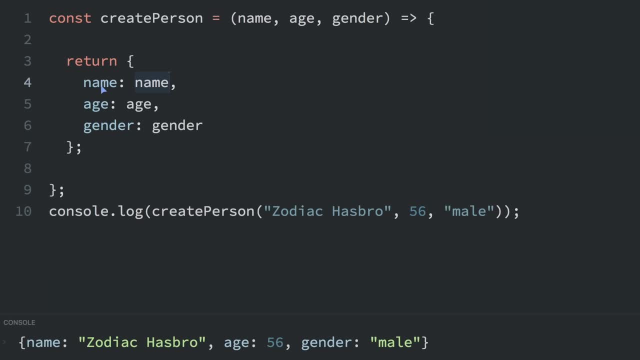 know that you want to create an object with the, where the key is the name of the variable And the value is the value of the variable. There's an easier way to do it. we can actually delete this whole thing here, And this is how we're going to do do it. We'll just do name age under JavaScript. 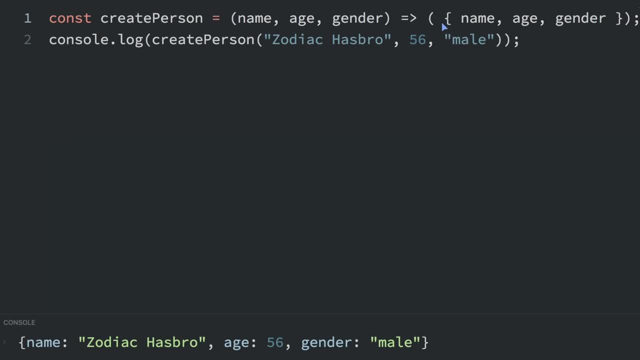 knows that it's going to return its value. As soon as we enter this debug into our clause, we'll actually we're going to see Now, with that the value is lại a value, or it's an такая contest roamed with a value, of a value that 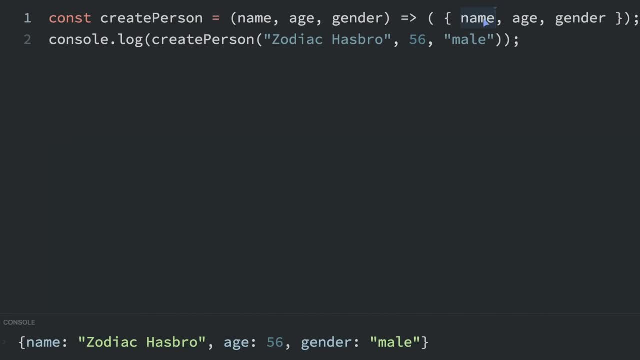 we're not able to exactly. i've got a. we're just gonna touch back and we're going to in and check that out. change a a little bit And you can actually see how it works, because this is what we're hoping thing. return this object and it's going to have three key value pairs: the name, age and gender. So if 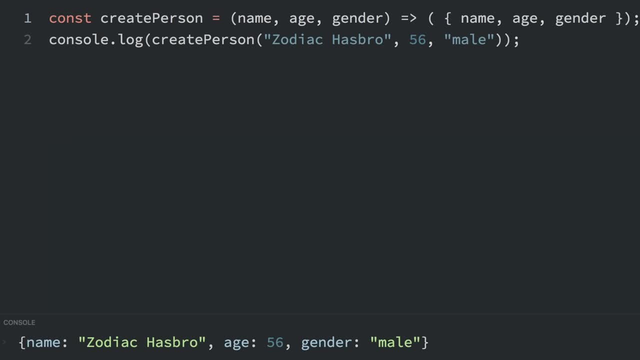 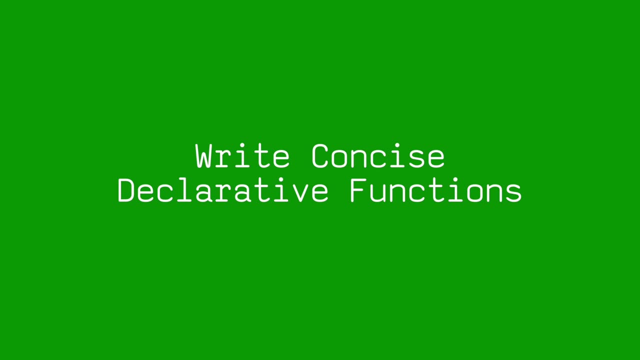 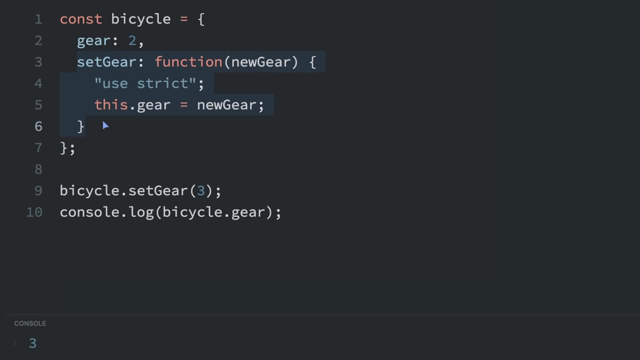 I reload this. you'll see in the console it looks exactly the same, because this code does the same thing that the previous code did: An object can contain a function. This is the long way to put a function within an object. But there is a simpler way. we have the set gear function. But 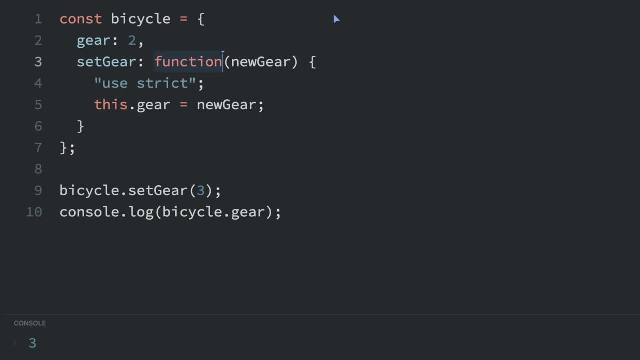 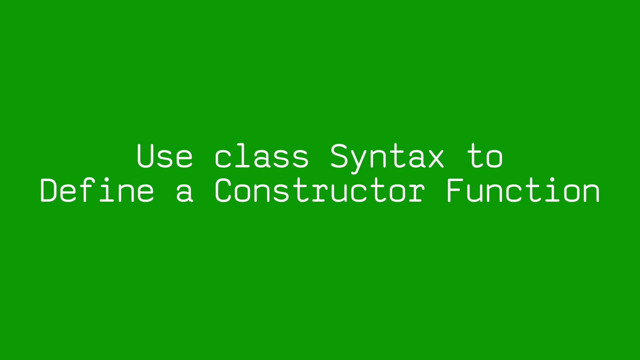 instead of using the function keyword and this colon, we can just delete all that. And now this is the new way. If I load this again, you'll see three in the console, just like it was before, because we've been able to set the gear using that function. Yes, six provides a syntax to: 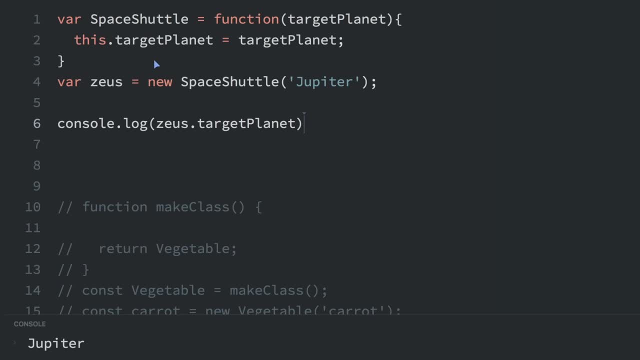 help create objects using the function key, And that's what we're going to do here. We're going to use the class keyword. So here's the older way to create an object. It's with the, the new keyword. we can instantiate an object using this new keyword And we're instantiating the space. 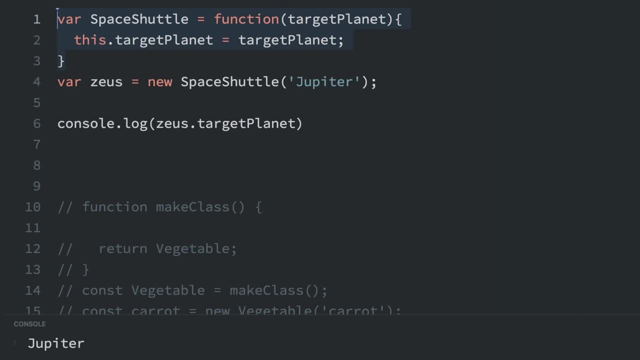 shuttle object. we have to have this constructor function up here. So we use this to construct the object where we pass in the target planet Jupiter and we set the target plan to this dot target planet. Once we create the new object, we're going to use the class keyword And we're going to use 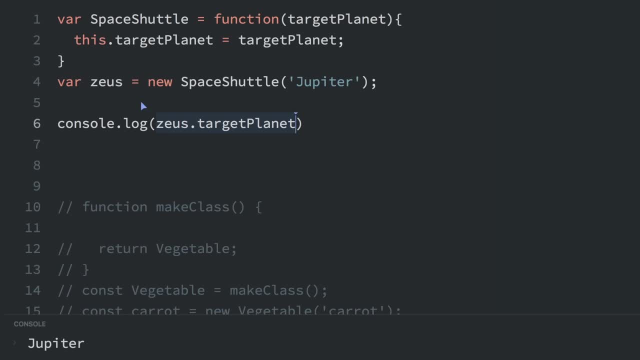 an object like this that allows us to do Zeus dot target planet. So Zeus dot target planet, which we set to Jupiter, Jupiter. So in the console you can see Jupiter. the class syntax replaces the constructor function creation, So I delete that. we're going to use the class syntax, So I'll do a. 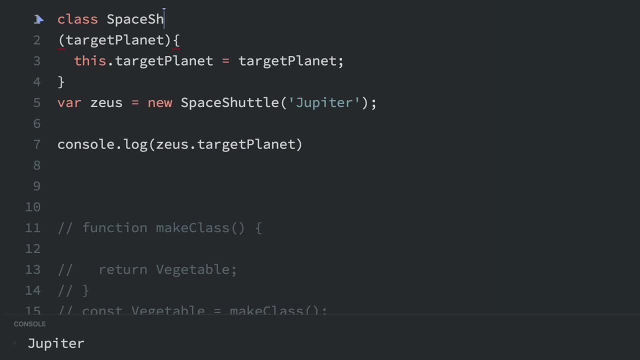 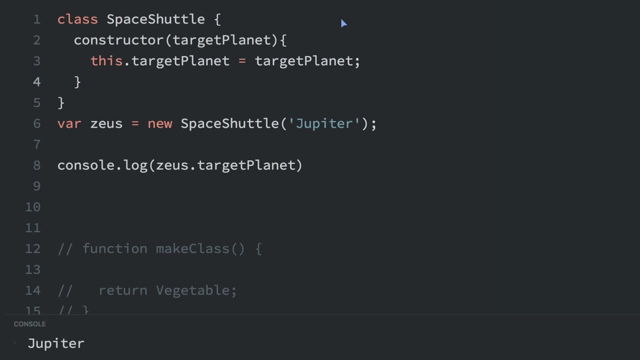 class space shuttle, And then we have the curly brace here, And so inside here we have a construct structure, So do constructor, target planet, And then that's all we just have to put in the curly brace, And this works exactly the same as before, using the class keyword and this constructor. So 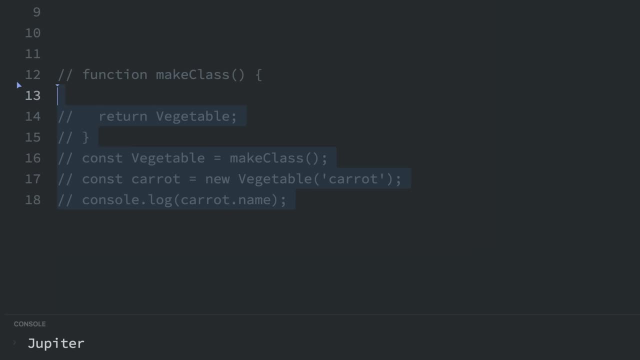 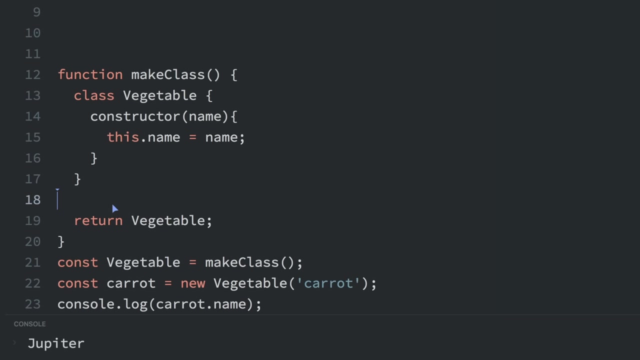 down here we are going to do the same thing for a vegetable class. So for the vegetable class we'll have class, That's the bo, And we're going to have a constructor with the name. this dot name equals name. So now that we have this, we can set this vegetable to make class, which will return. 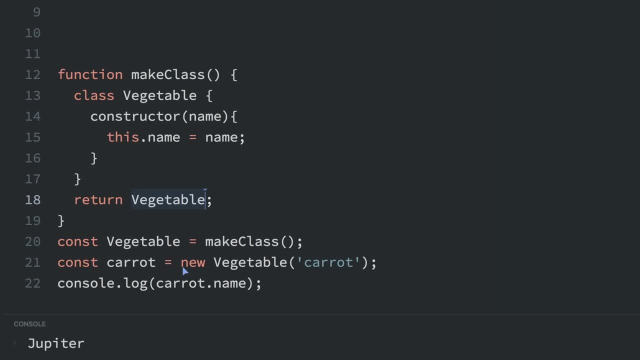 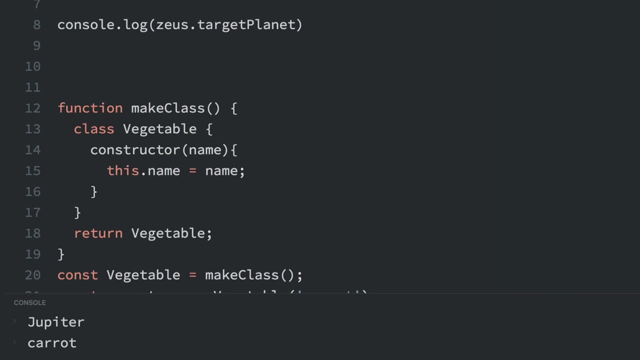 a vegetable class. So that's up here And then when we do new vegetable and passing carrot, this care will go into here and it'll get set as this dot state name. So when we console that log caret, that name, we should get caret With a class object. 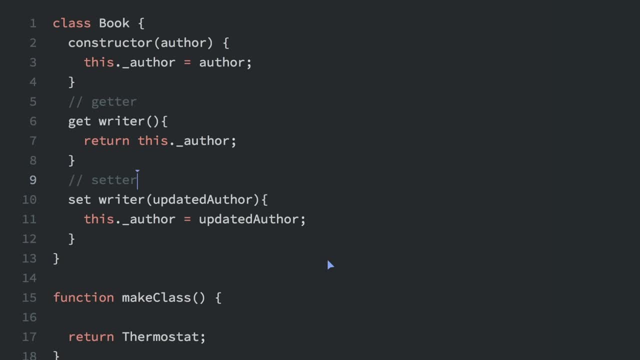 you often want to obtain values from the object and set a value of a property within an object. These are often called getters and setters. So in this class object we have the constructor, which we already talked about. we also have a getter and setter to get and set the writer. 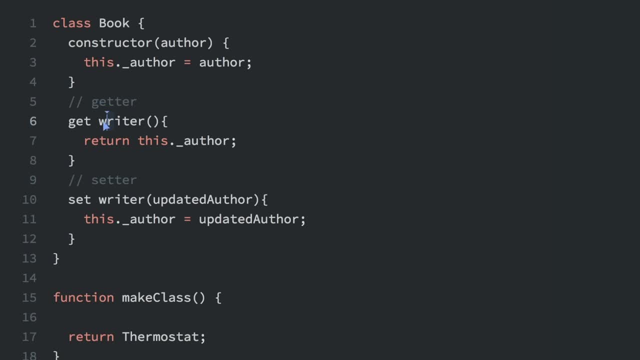 so we can get the writer and we can set the writer. getter functions are meant to simply return or get the value of an object's private variable to the user without the user directly accessing the private variable. So the private variable is this underscore author that gets set. 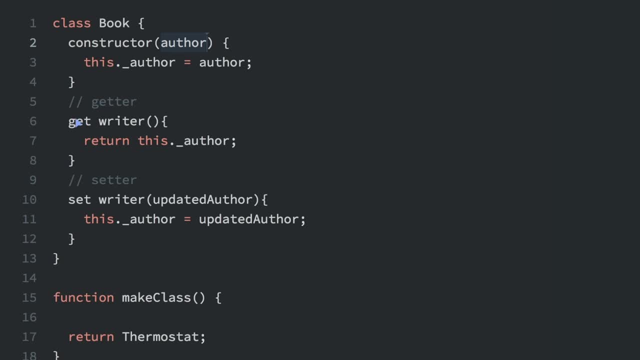 when you construct the object And then when we do get writer, it's going to return the return. this dot underscore author. So you never actually interact directly with this variable, But it's going to get the writer, which is the author here. And when you're setting 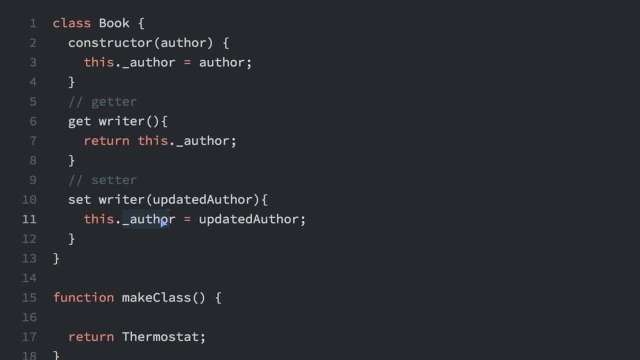 it's the same, So you're never interacting with the underscore author, But you can set that with the writer setter. this change could invoke calculations or even even overriding the previous value completely, So you can have any number of code lines in this setter. 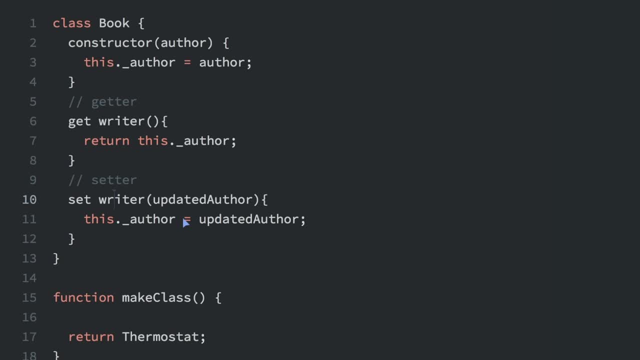 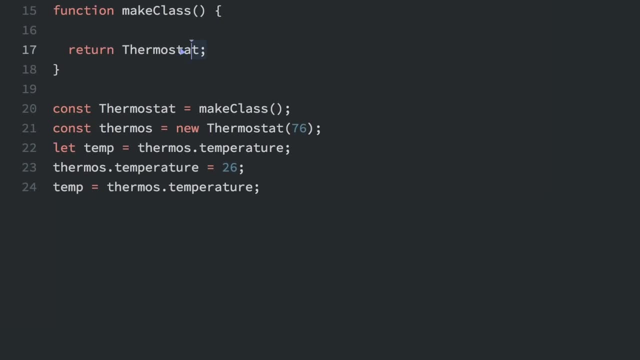 to ultimately maybe do different calculations before you set it or a calculation before you get the property. So what we're going to do is make our own getter and setter for the thermostat class. we're going to create a thermostat class and we're going to have a getter and setter. So here's. 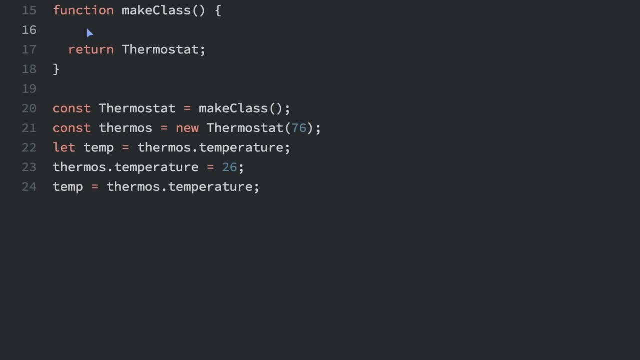 the thing about this challenge is that when we construct the class, it's going to accept Fahrenheit temperature, but we're going to create a getter and setter in the class to obtain the temperature in Celsius, So it's going to have to do the calculation. 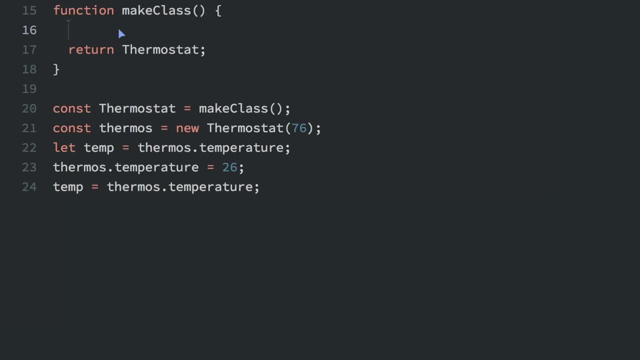 right within the class. So let's do that. we're going to do a class of thermostat And in this class we need the constructor. But when you first create the thermostat, you're going to pass in a temperature And remember this is going to be Fahrenheit. Now, within this constructor, 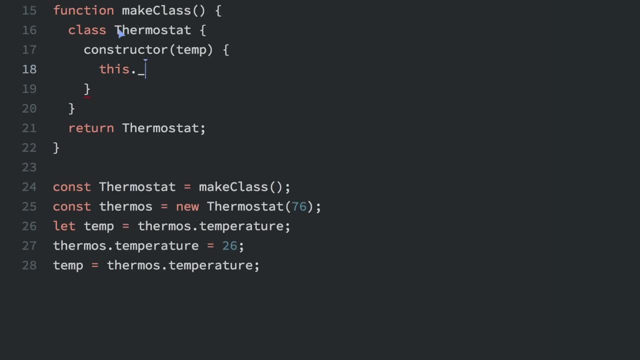 we're going to set a private variable, this dot, underscore temp. So the word this just means that this variable is only accessible within this class here And the underscore temp. whenever you start a variable with an underscore, that's going to generally signify that it's a private variable, that you're not supposed to access it outside of that scope, or 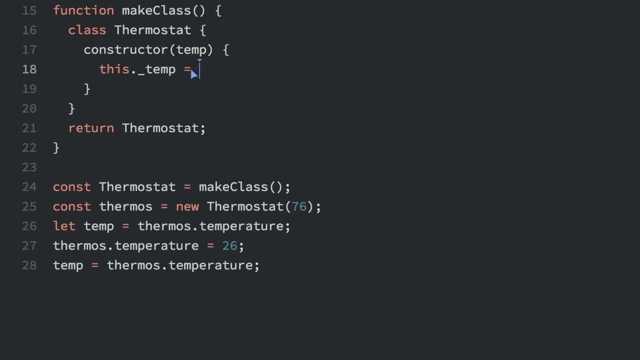 outside of that class. So we're going to set the temp And we're not going to just put this underscore. temp equals temp, because it's passed in as Fahrenheit and we want to convert it to Celsius. I just happen to have the equation for Celsius, So 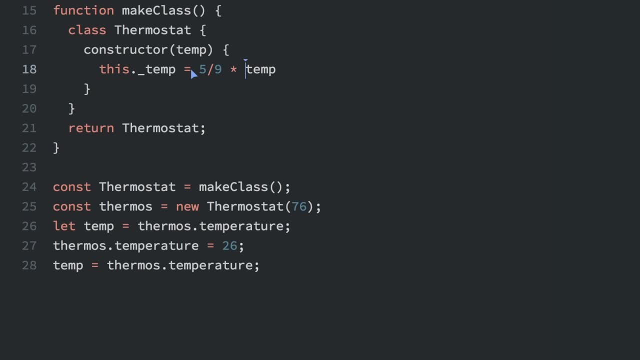 it's five, over nine times and then we'll temp minus 32.. So now we can create the getter and setter. So we'll forget or we'll do get temperature And we're just going to return this dot underscore temp, which now it's in Celsius, because we're storing the value in Celsius, even though the 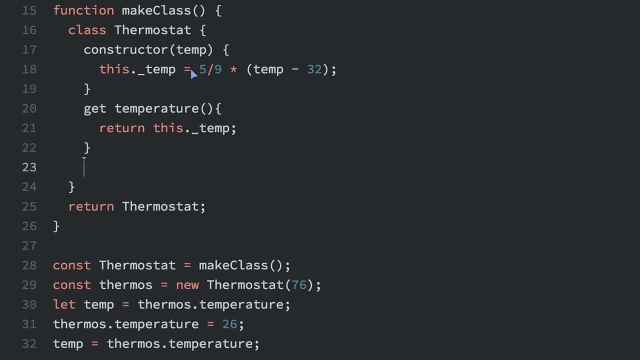 thermostat is created in Fahrenheit, So with the setter it's going to be the same set temperature, updated temp And it's now going to still be in Celsius. So this dot temp equals updated temp. So let's look at the code. 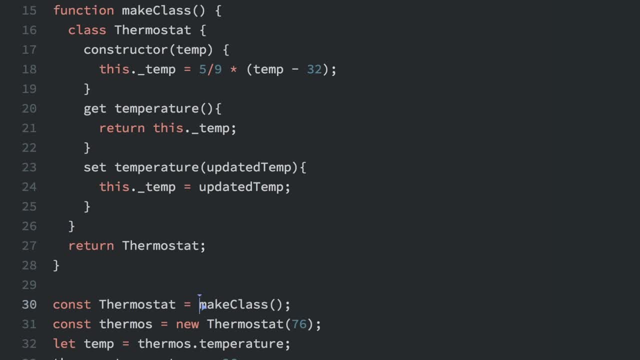 Okay. so I'm going to re-show that down here in a minute how we're using it. So the cons thermostat equals make class, this make class function is going to return this thermostat object here, And then we're going to do a const thermos equals new thermostat. So when you're instantiating an object, you always use the new keyword new. 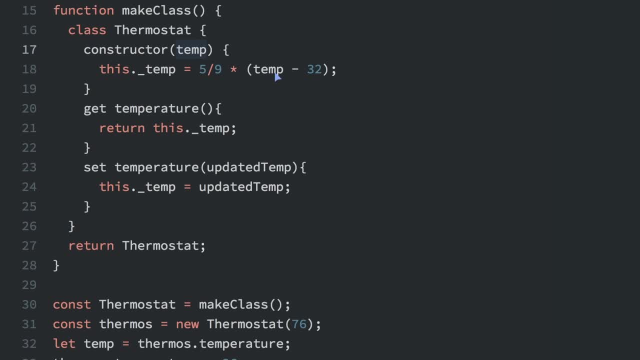 thermostat. That's this, and we're passing in 76, that goes into the constructor, the temp, And so we do this calculation to convert that Fahrenheit to the Celsius and the m el, We use a弟α manufacturer as a plus sign. we move thecka ness and output sparte in 우ic factors equal viendo. 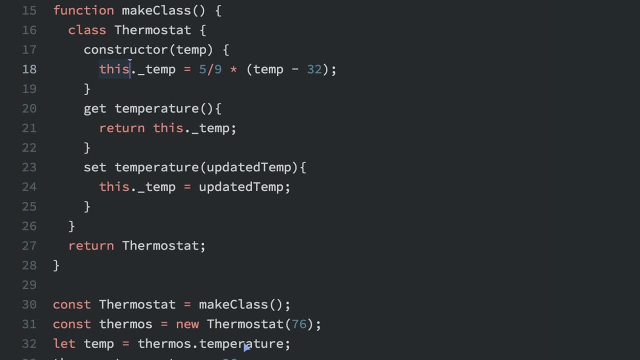 Fahrenheit tota电iques to the Celsius in this local variable here And then let temp equals thermos dot temperature. So thermos dot temperature is going to use the getter get temperature and it's going to return this dot underscore temp. So a key thing to look at is that there are no parentheses after this. 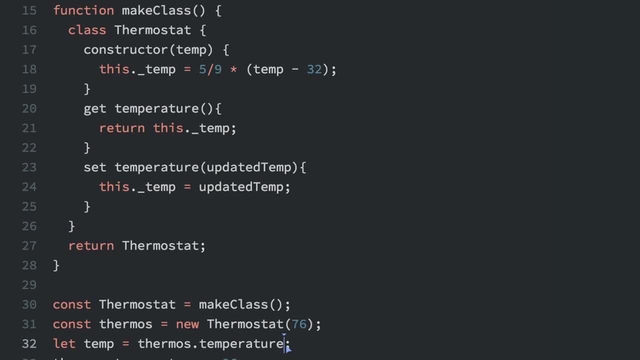 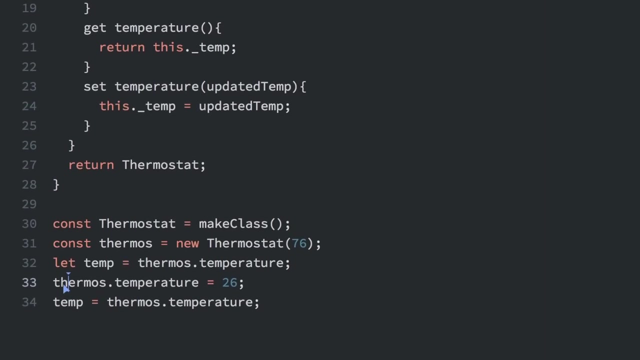 So generally, if there's, if something is a function, you would see parentheses after the function name. But if it's a variable or property name, it's going to not have parentheses. So getters and setters are access similar to properties And then we can use the setter here. 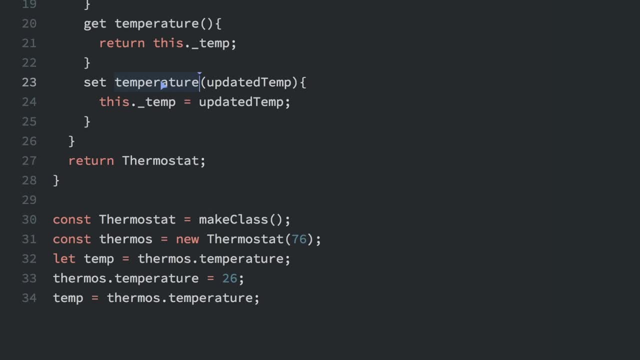 thermos dot temperature equals 26.. And then it sets it with the updated temperature And now we can say temp equals thermos dot temperature And if we do a console dot log here we can do that with the temp And it should have the new temperature. 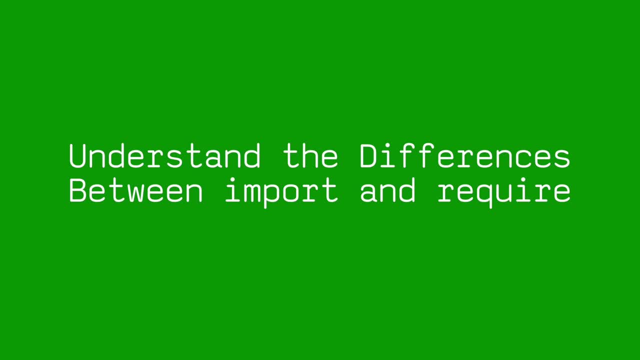 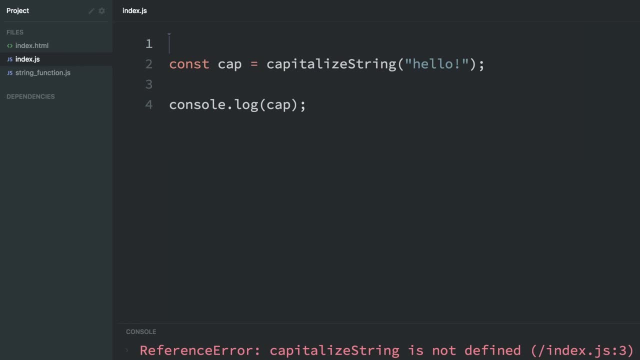 By load that 26.. In the past people would use the require function to import functions and code from other files, But now we have import and export. you can export code in one file and then import it in another file. It also allows you to only import certain functions from a file or 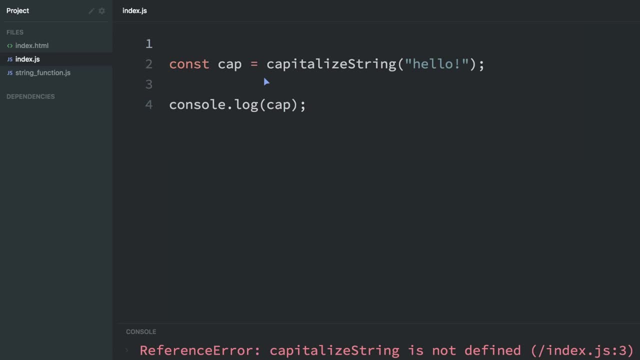 certain variables. Let me show you how it works. So in this file we have this case. you have adleized string function where we're passing in the string hello, and we want it to log out the capitalized strings. But right now it just has an error because there is no capitalized. 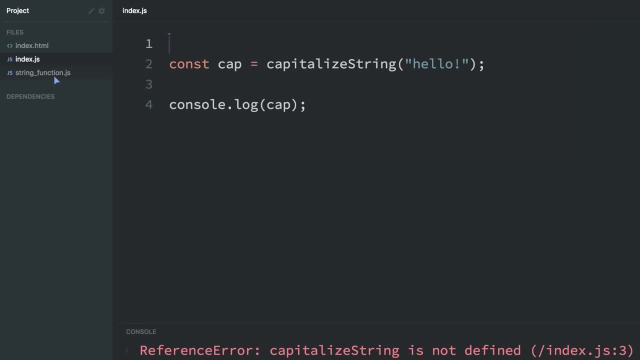 string function in this file. However, in this other file we do have a capitalized string function. In this string function, dot jse, we have export- this is the export statement I was talking about- And then it's exporting this function. It's actually a variable capitalized. 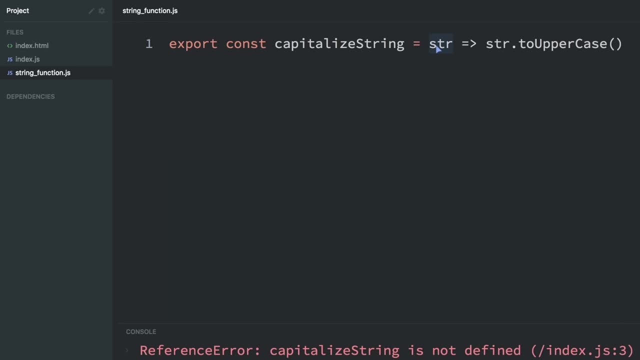 string function dot conveniter, And you can see here that we have alternate、 and that means string that's set to equal a function. This is a an arrow function where we pass in a string and then we return the string dot to uppercase. Now, to uppercase is just a string function. that. 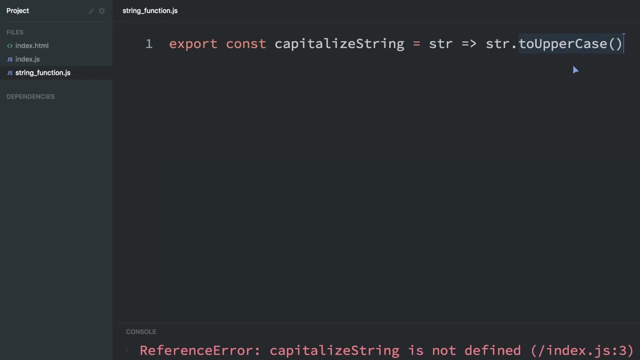 makes every letter uppercase. So we can import this in our other file. So let's go back to our other file And I will import And with the import statements you're going to use curly braces And then I'll put capitalize string And then we have to say what we're importing it from. we want to. 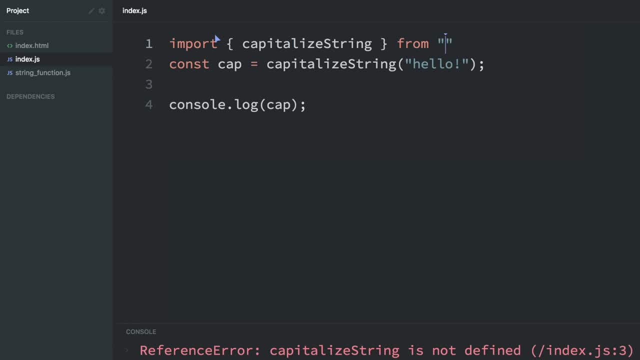 import it from, And this is where I put the file name. Now, normally you're gonna start with a dot slash, which just means the current directory, and I'll type in the file name string function. now the file name is a dot j s after it, but that's assumed, So you don't have to put dot j s. 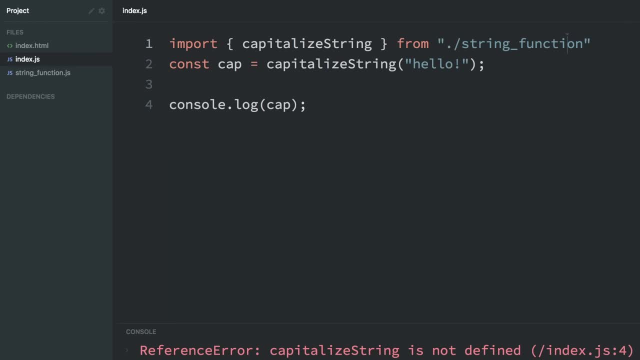 you can just put the file name without the extension. So if I run this you can see Hello and all capital letters is successfully imported. this function from the other file And we used it in this file. I talked a little bit about export in the last lesson, But now I'm going to go into 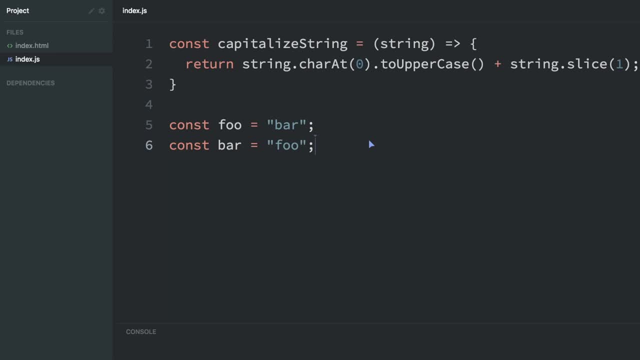 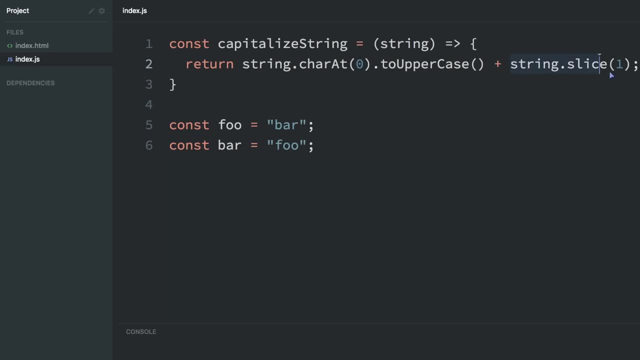 it actually just capitalizes the first letter of the string and then leaves the rest of the string lowercase. And before I showed you you can just put export right before here. but we can export a different way, So I'll do export And then, in curly braces, capitalize, capitalize. 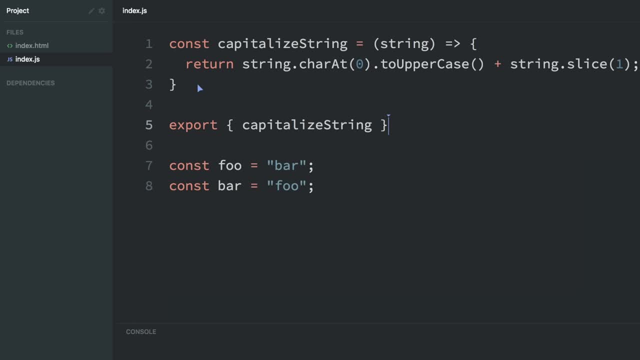 string. And so now we just export this function. And to export a variable like this, we have const equals bar, const bar equals foo. To export these variables you just type in export, like both before. So now in this file we're exporting this. 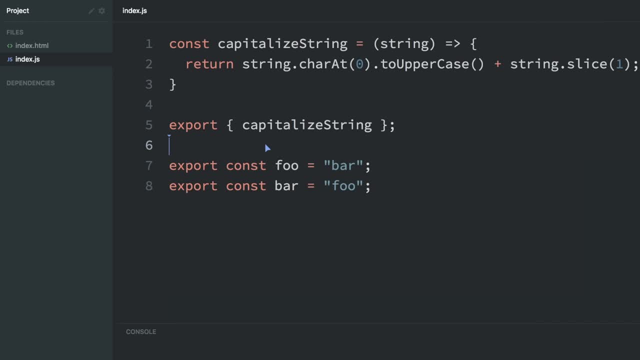 function and these two variables, and then we could import them into another file. If a file exports multiple different things, you can import each things individually or you can import everything. So let me show you how you would import everything from a file. 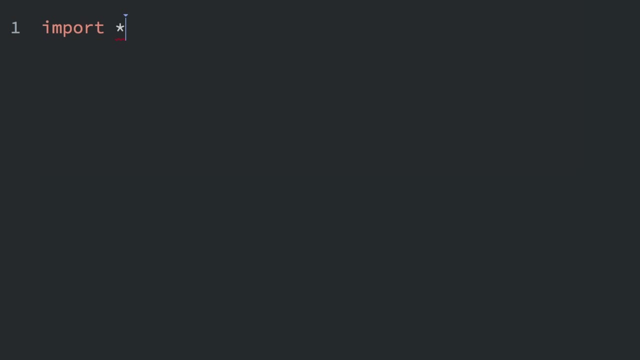 it's just import, And then you're gonna put an asterisk or a star, And then you're gonna put as, import as, and then you have to create an object to store everything in. So I'm going to import stuff from a file called capitalized strings. So I'm going to call this capitalize. 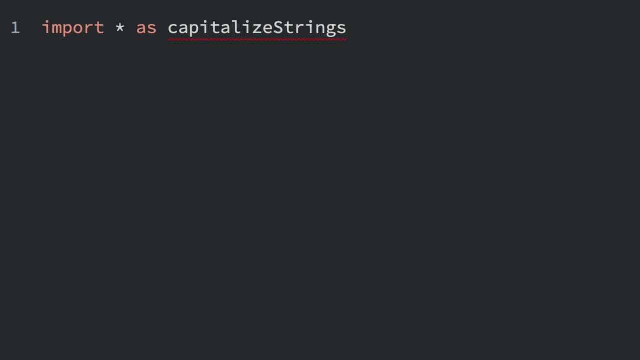 strings. So this could really be anything. I'm creating an object with this, And then I'm going to say what I'm importing it from, from, and then I just put the file name. In this case it's just going to be capitalized strings. Sometimes you would have to put a dot slash if it's in the same. 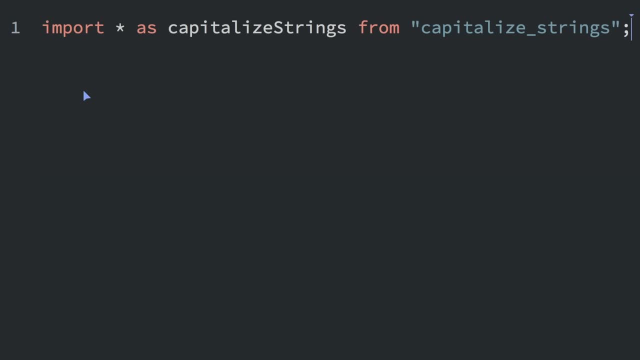 directory there And then I'll make sure to put a semicolon at the end. So if you're importing everything, you always start off with import star as, and then this can be anything. it can be any object name that you create and then gonna put from an enemy. put the file name in.